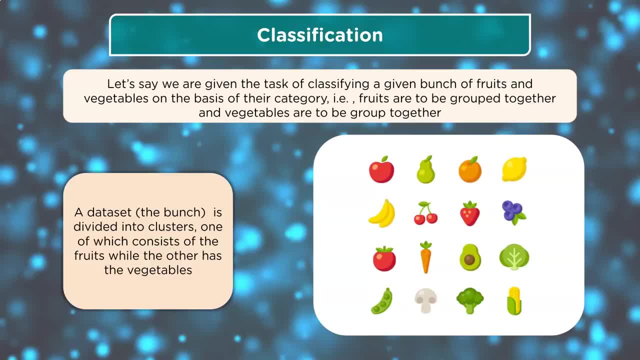 data. When we talk about breast cancer, can we sort out in images to see what is malignant and what is benign? Very popular one. Can you classify flowers? The iris data set Certainly in wildlife. can you classify different animals and track where they're going? Classification is really. 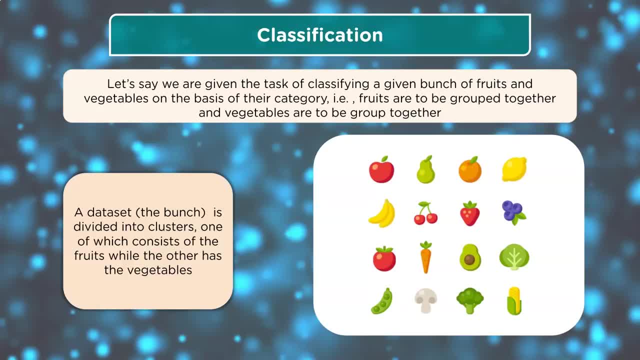 the bottom starting point or the baseline for a lot of machine learning and setting it up and trying to figure out how we're going to break the data up so we can use it in a way that is beneficial. So here the fruits and the vegetables are grouped into clusters and each cluster has a specific 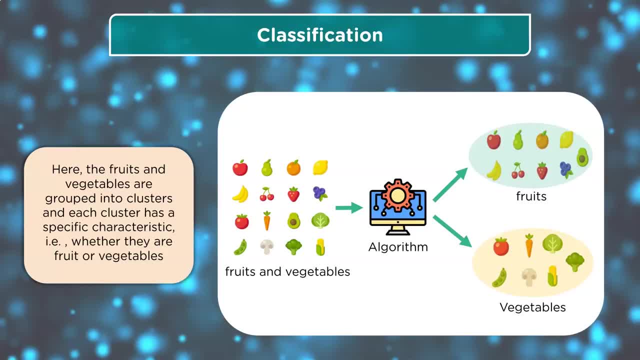 characteristic, ie whether they are a fruit or a vegetable. And you can see, we have a pile of fruits and vegetables. We feed it into the algorithm and the algorithm separates them out and you have fruits and vegetables. So some important terminologies before we dig into how it sorts them out and what that all. 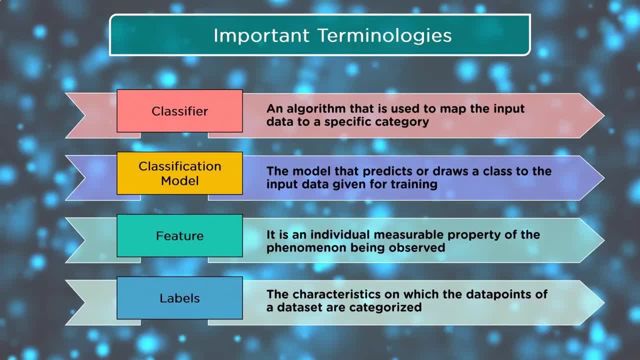 means, When we look at the terminologies, you have a classifier. That's the algorithm that is used to map the input data to a specific category. The classification model: the model that predicts or draws a class to the input data given for training Feature. it is an individual measurable property of the phenomena being observed And 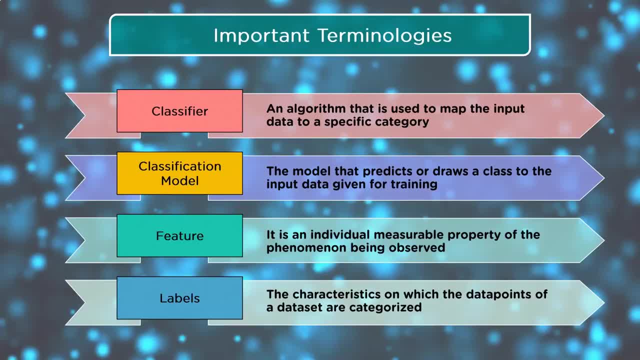 labels the characteristics on which the data points of a data set are categorized. The classifier and the classification model go together. A lot of times the classifier is part of the classification model And then you choose which classifier you use after you choose which model you're using Where features are. 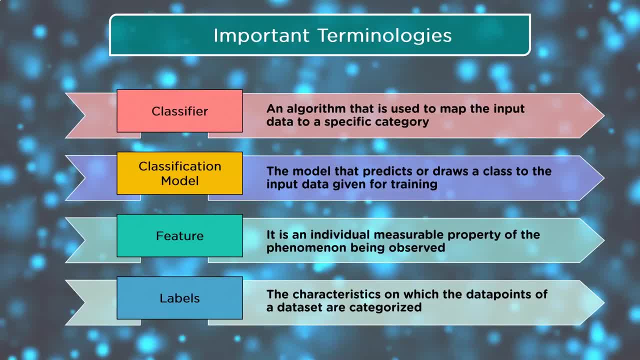 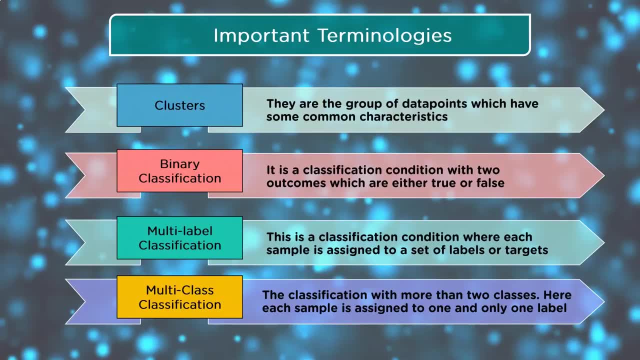 that go in, Labels are that go out. So your classifier model's right in the middle of that. That's that little black box. we were just talking about Clusters. they are a group of data points which have some common characteristics: Binary classification. 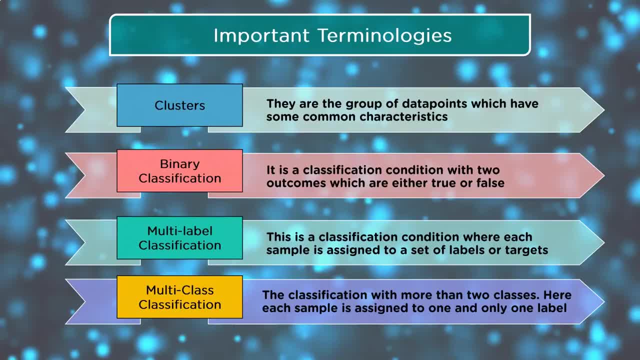 It is a classification condition with two outcomes, which are either true or false. Multilabel classification: this is a classification condition where each sample is assigned to a set of labels or targets. Multiclass classification: The classification with more than two classes, Here each sample. 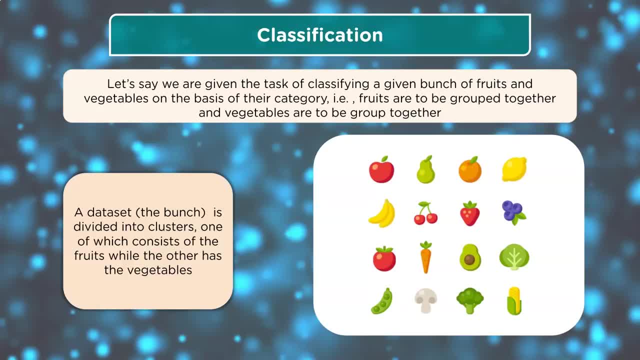 the bottom starting point or the baseline for a lot of machine learning and setting it up and trying to figure out how we're going to break the data up so we can use it in a way that is useful. So here the fruits and the vegetables are grouped into clusters and each cluster has a specific 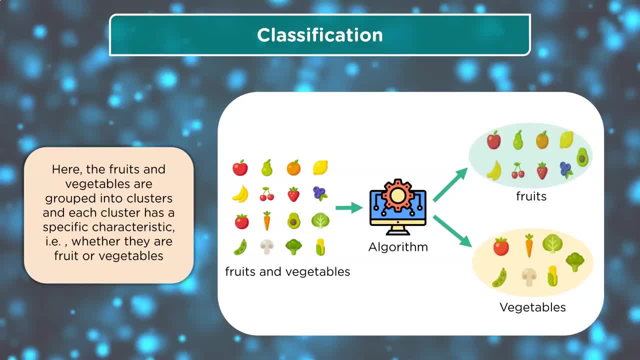 characteristic, ie whether they are a fruit or a vegetable. And you can see, we have a pile of fruits and vegetables. We feed it into the algorithm and the algorithm separates them out and you have fruits and vegetables. So some important terminologies before we dig into how it sorts them out and what that all means. 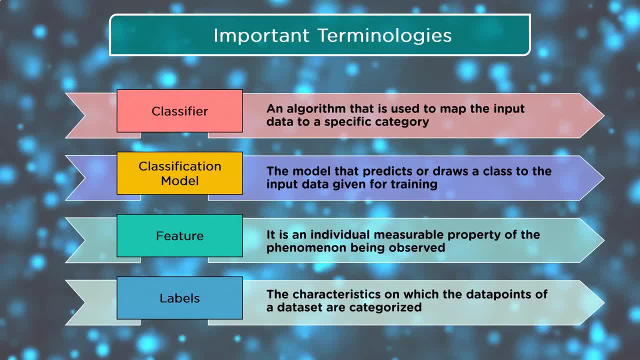 When we look at the terminologies, you have a classifier. That's the algorithm that is used to map the input data to a specific category. The classification model: The model that predicts or draws a class to the input data given for training Feature. It is an individual, measurable property of the phenomena being observed. 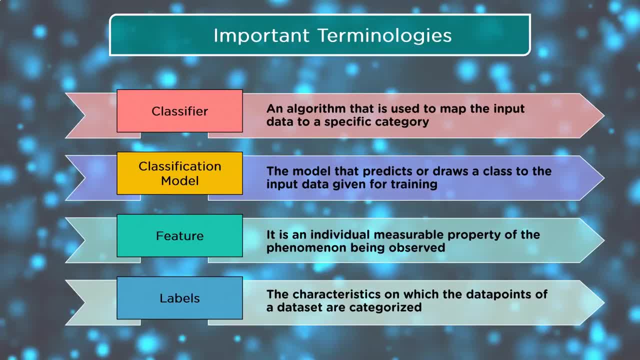 And labels The characteristics on which the data points of a data set are categorized. The classifier and the classification model go together. A lot of times the classifier is part of the classification model And then you choose which classifier you use after you choose which model you're using. 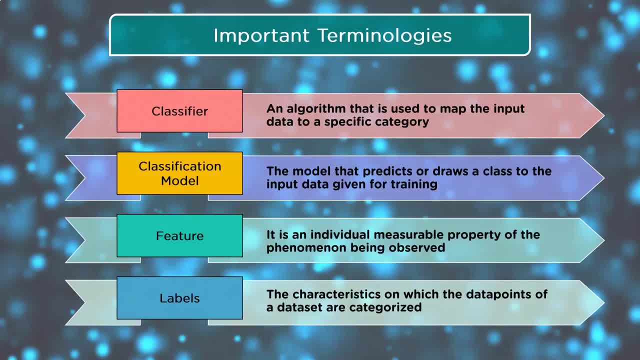 Where features are what you're using. The classifier is what you're using. Where features are what you're using. Where features are what you're using. What goes in Labels are what comes out. So your classifier model is right in the middle of that. 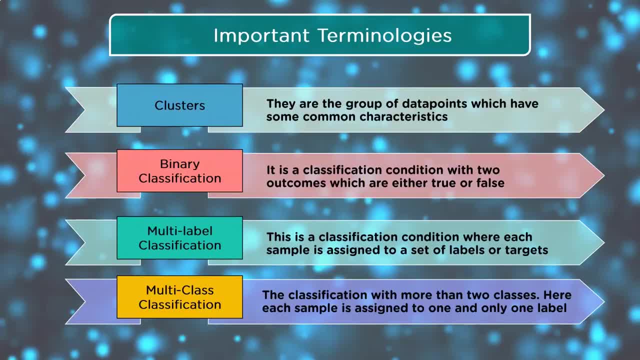 That's that little black box we were just talking about Clusters. They are a group of data points which have some common characteristics. Binary classification: It is a classification condition with two outcomes, which are either true or false. Multi-label classification: This is a classification condition where each sample is assigned to a set of labels or targets. 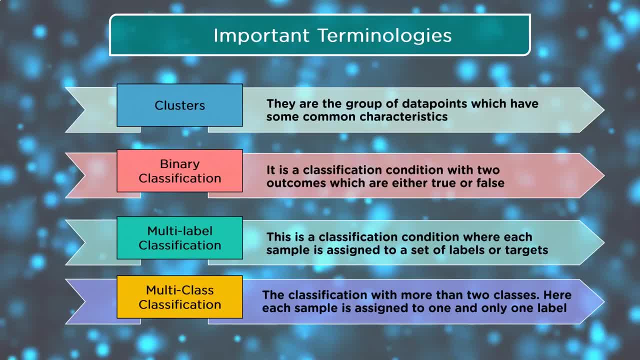 Class classification: The classification with more than two classes. Here each sample is assigned to one and only one label. When we look at this group of terminologies, a few important things to notice, Going from the top clusters. When we cluster data together, we don't necessarily have to have an end goal. 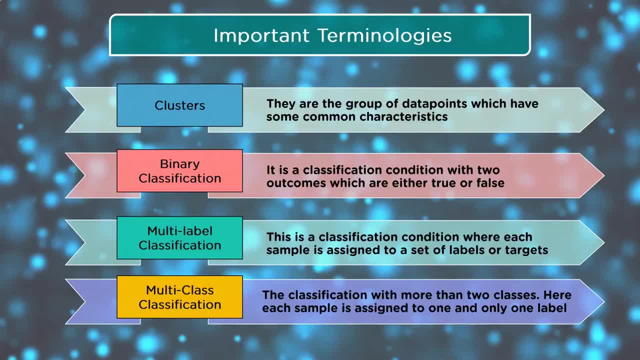 We just want to know what features cluster together. These features, then, are mapped to the outcome we want. In many cases, the first step might not even care about the outcome, only about what data connects with other data, And there's a lot of clustering algorithms out there that do just the clustering part. 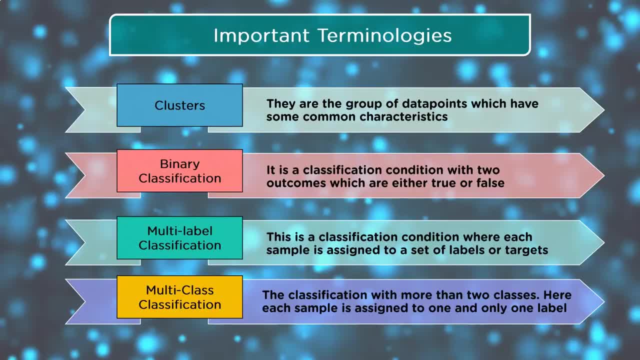 is assigned to one and only one label. When we look at this group of terminologies, a few important things to notice Going from the top clusters. when we cluster data together, we don't necessarily have to have an end goal. We just want to know what features cluster together. These features, then, are mapped. 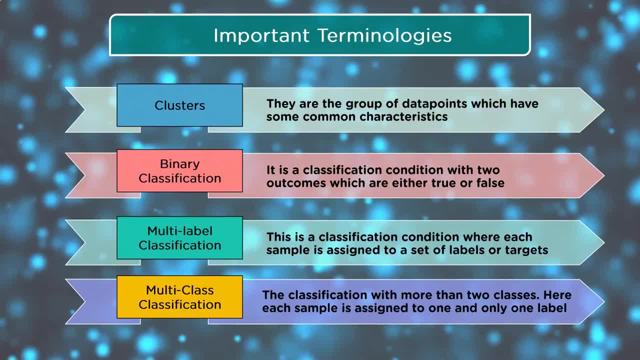 to the outcome we want. In many cases, the first step might not even care about the outcome, only about what data connects with other data, And there's a lot of clustering algorithms out there that do just the clustering part. Binary classification: It is a classification condition with two outcomes, which are: 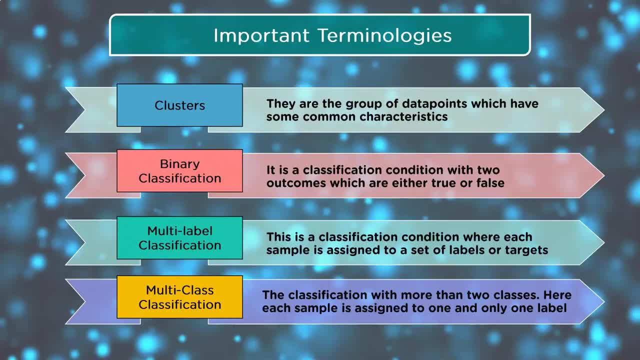 either true or false We're talking. usually it's a. it's either a cat or it's not a cat. It's either a dog or it's not a dog. That's the kind of thing we talk about, binary classification, And then that goes into multi-label classification. Think of label as you can. 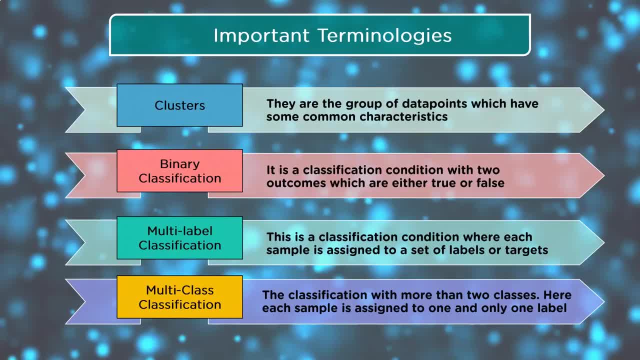 have an object that is brown. You can have an object that is labeled as a dog, So it has a number of different labels. That's very different than a multi-class classification, where each one's a binary: You can either be a cat or a dog. You 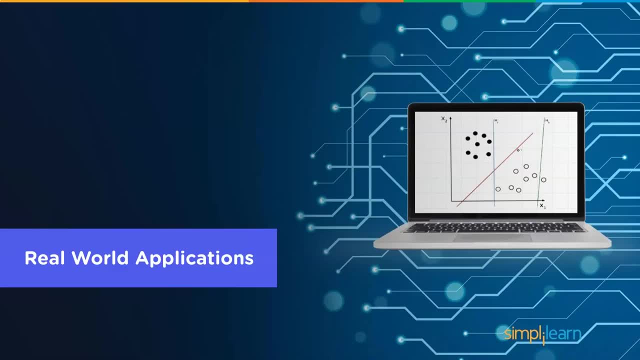 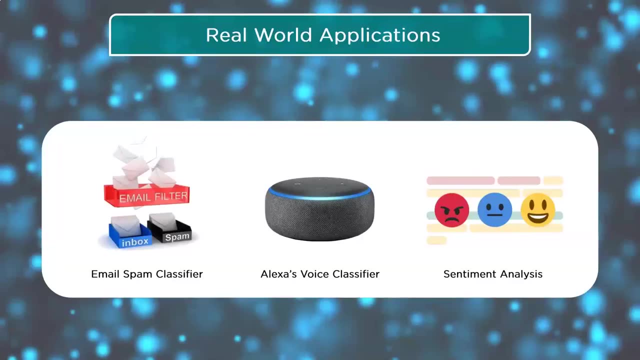 can't be both a cat and a dog- Real-world applications. So to make sense of this, of course the challenge is always in the details- is to understand how we apply this in the real world. So in real-world applications, we use this all the time. We have email spam classifier, So you have your email. 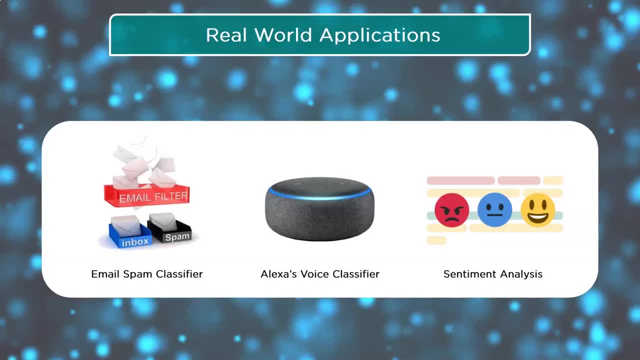 inbox coming in. It goes through the email filter that we usually don't see in the background And it goes. this is either valid email or it's a spam And it puts it in the spam filter if that's what it thinks it is Alexa's voice. 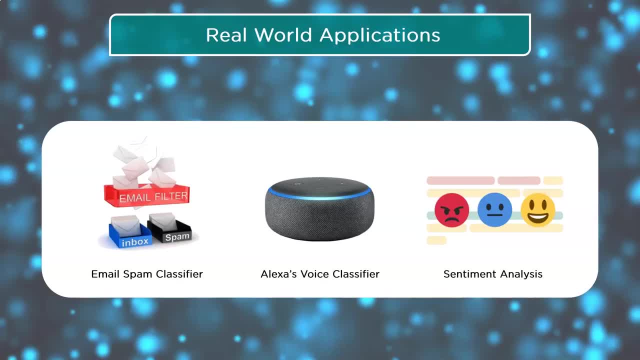 classifier: Google Voice, Any of the voice classifiers. they're looking for points, So they try to group words together And then they try to find those groups of words trigger a classifier. So it might be that the classifier is to open your tasks program or open your 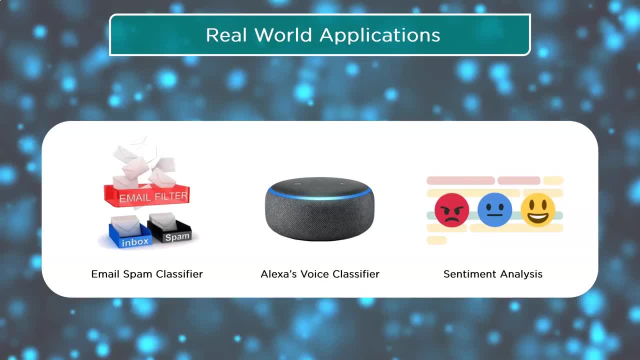 text program so that you can start sending a text. Sentimental sentiment analysis is really big When we're tracking products. we're tracking marketing. trying to understand whether something is liked or disliked is huge. That's like one of the biggest driving forces in sales nowadays And you almost have to have these. 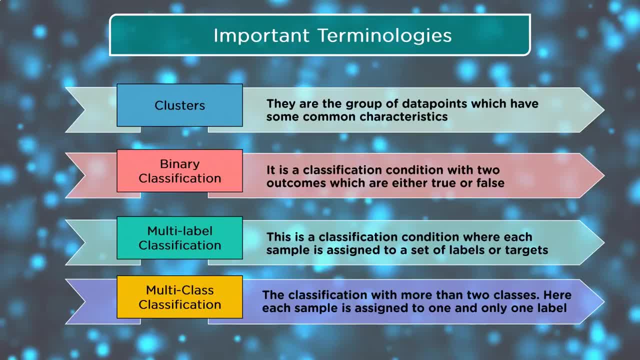 Binary classification. It is a classification condition with two outcomes, which are either true or false We're talking. usually it's either a cat or it's not a cat. It's either a dog or it's not a dog. That's the kind of thing we talk about, binary classification. 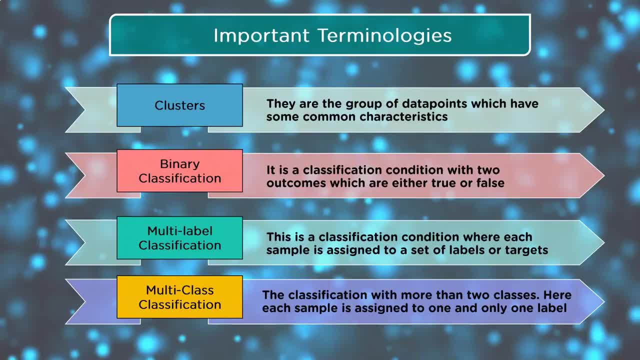 And that goes into multi-label classification. Think of label, as you can have an object that is brown, You can have an object that is labeled as a dog, So it has a number of different labels. That's very different than a multi-class classification where each one's a binary. 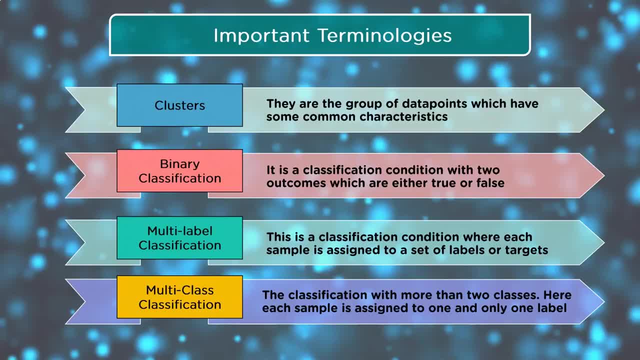 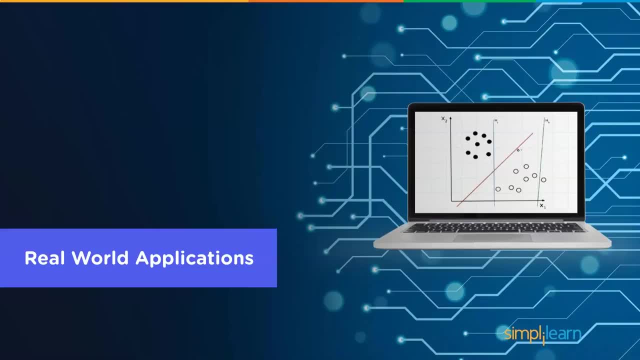 You can either be a cat or a dog. You can't be both a cat and a dog. Real world applications. So to make sense of this, of course the challenge is always in the details. Just to understand how we apply this In the real world. 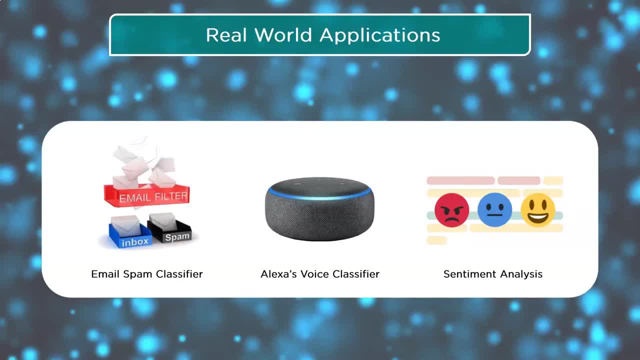 So in real world applications we use this all the time. We have email spam classifier, So you have your email inbox coming in. It goes through the email filter that we usually don't see in the background And it goes: this is either valid email or it's a spam. 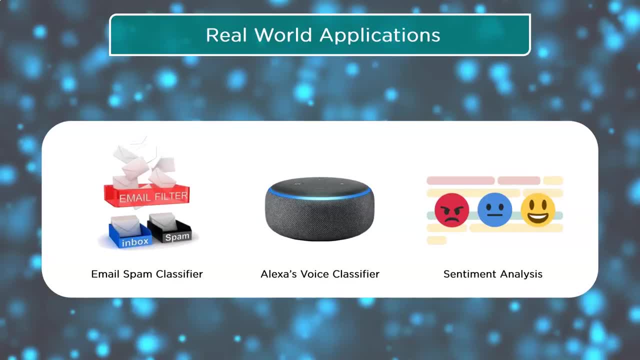 And it puts it in the spam filter, if that's what it thinks it is. Alexa's voice classifier, Google Voice- Any of the voice classifiers? they're looking for points, So they try to group words together And then they try to find those groups of words trigger a classifier. 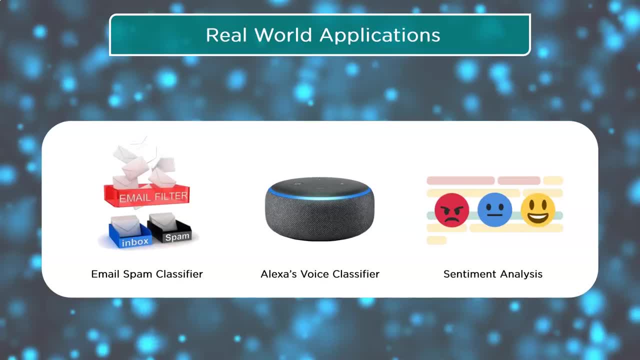 So it might be that the classifier is to open your tasks program Or open your text program so that you can start sending a text. Sentiment analysis is really big When we're tracking products, we're tracking marketing. Trying to understand whether something is liked or disliked is huge. 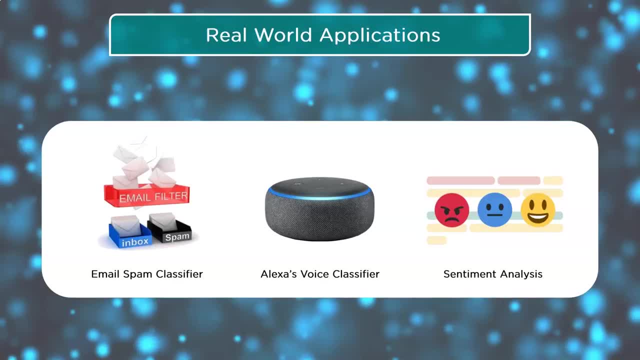 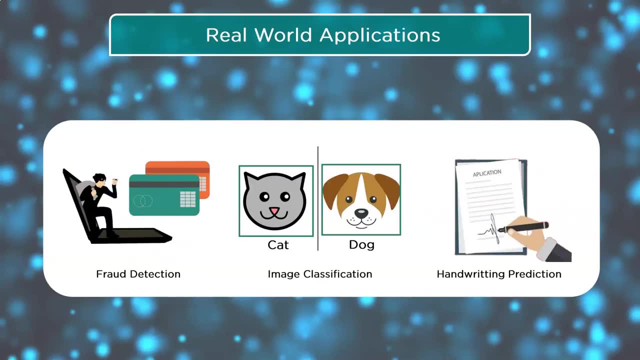 That's like one of the biggest driving forces in sales nowadays And you almost have to have these different filters going on. if you're running a large business of any kind Fraud detection- You can think of banks. They find different things on your bank statement. 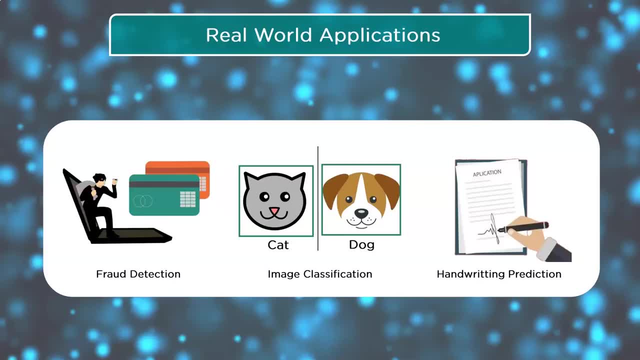 And they detect that there's something going on there. They have algorithms for tracking the logs on computers. They start finding weird logs on computers. They might find a hacker. I mentioned cat and dog, So here's our image classification. We have a neighbor who runs an outdoor webcam. 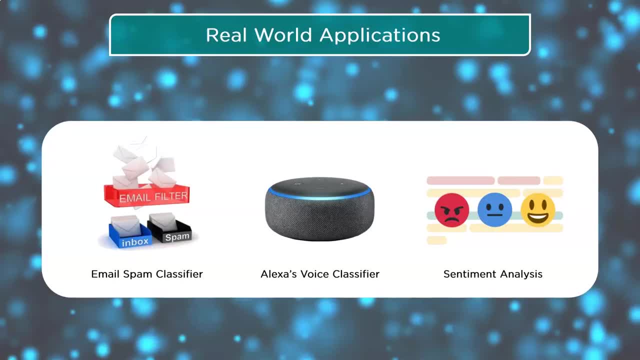 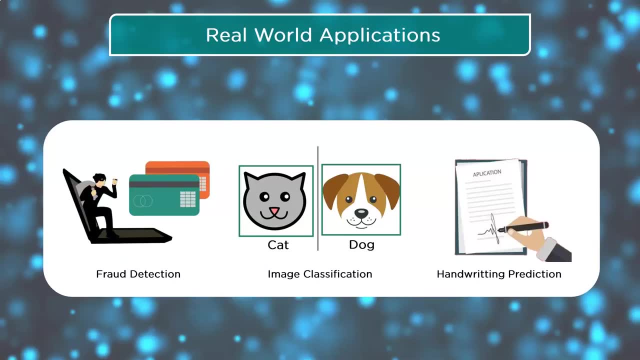 different filters going on. if you're running a large business of any kind Fraud detection, You can think of banks. They find different things on your bank statement and they detect that there's something going on there. They have algorithms for tracking the logs on computers. They start finding weird logs. 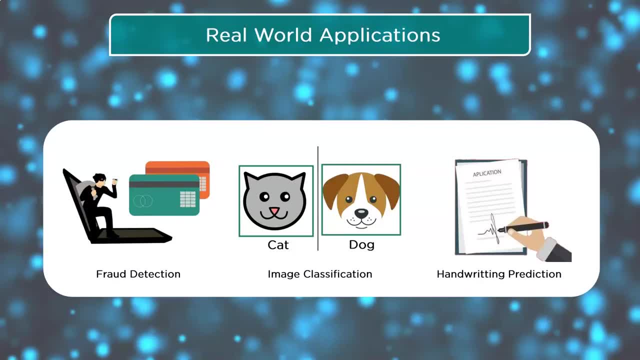 on computers They might find a hacker. I mentioned cat and dog, So here's our image classification. We have a neighbor who runs an outdoor webcam And we like to have it come up with the classification when the wild animals in our area are out like foxes. We actually have a mountain lion that lives in the area. 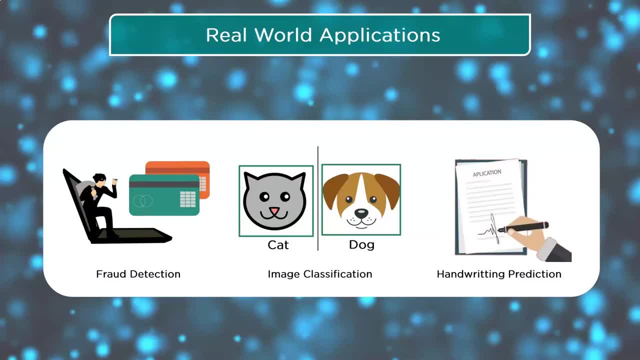 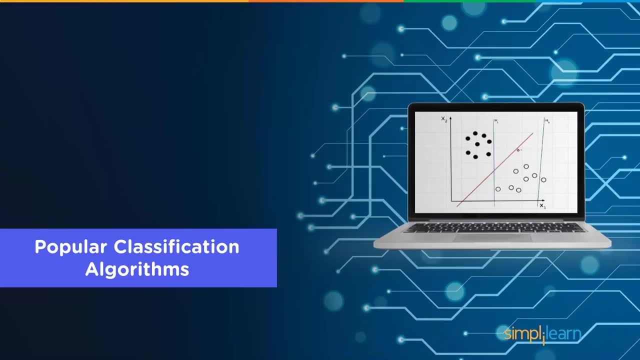 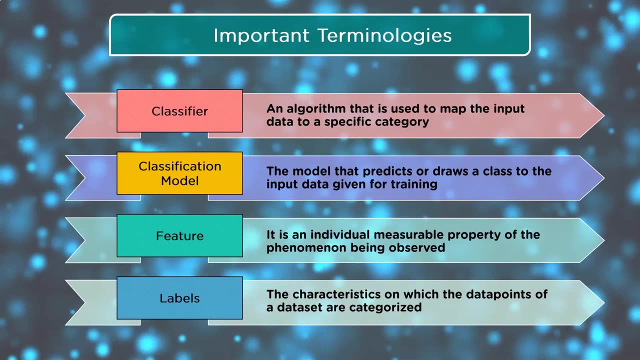 So it's nice to know when he's here. So let's go ahead and roll our sleeves up and take a look at some popular classification algorithms. Before we look at the algorithms, let's go back and take a look at our definitions. We have a classifier and a classification model, So 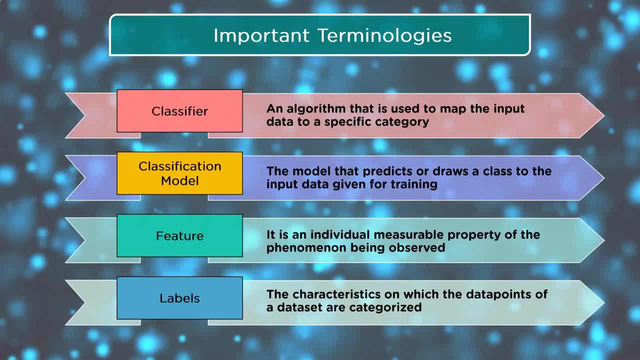 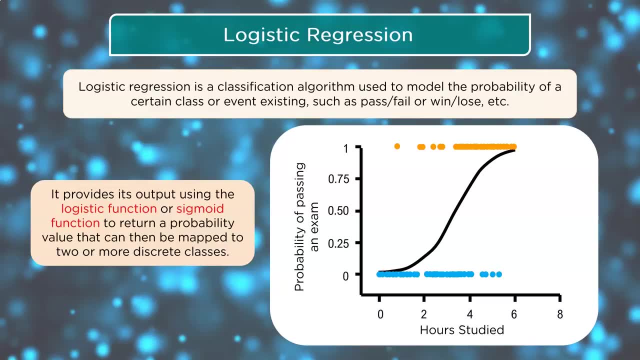 we're looking at the classifier, an algorithm that is used to map the input data to a specific category. One of those algorithms is a logistic regression. The logistic regression is a classification algorithm used to model the probability of a certain class or event existing, such as pass, fail or win, lose, etc. It provides its output using 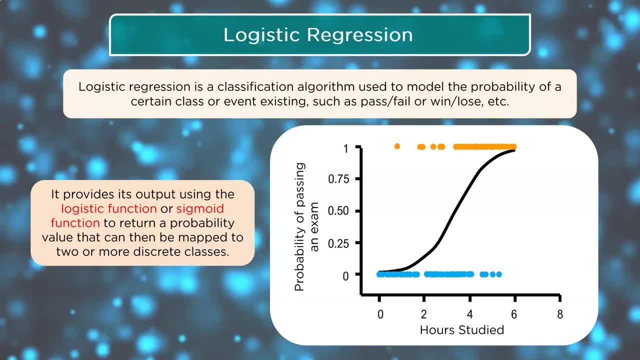 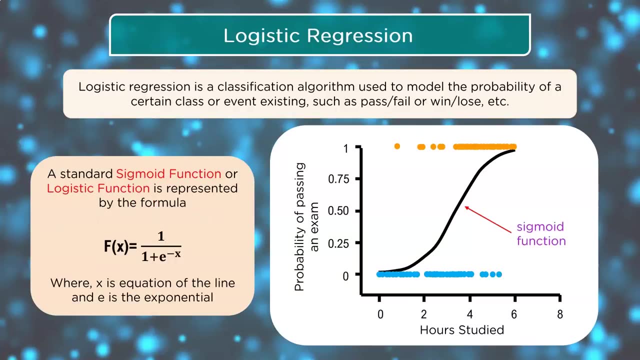 the logistic function or sigmoid function to return the probability value. that can then be mapped to two or more discrete classes. A sigmoid function is an activation function that fits the variable and limits the output to a range between zero and 1.. A standard sigmoid function or logistic function 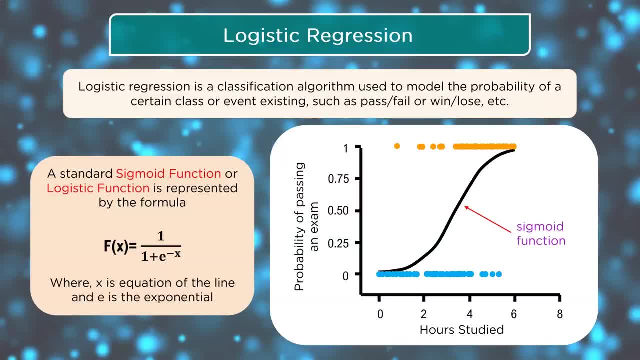 function is represented by the formula: fx equals 1 over 1 plus e to the minus x, where x is the equation of the line and e is the exponential. Just taking a quick look at this, you can think of this as being a point of uncertainty, and so, as we get closer and closer to the middle of the line, 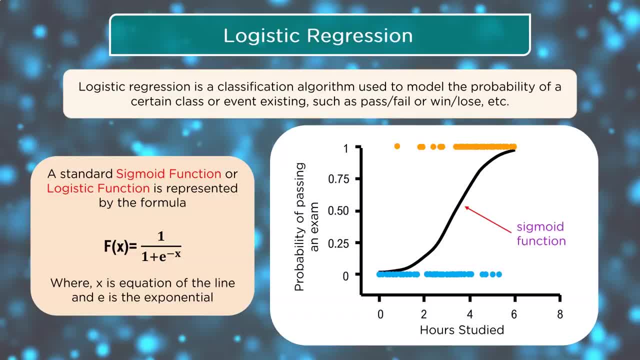 it's either activated or not, and we want to make that just shoot way up so you'll see a lot of the activation formulas kind of have this nice s-curve where it approaches 1 and approaches 0 and based on that there's only a small region of error, and so you can see in the sigmoid logistic function. 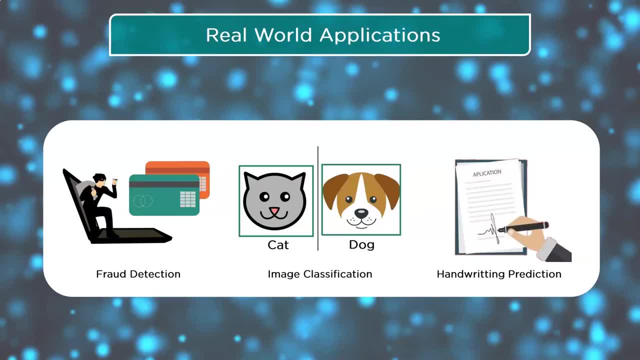 And we like to have it come up with a classification when the wild animals in our area are out Like foxes. We actually have a mountain lion that lives in the area, So it's nice to know when he's here. Handwriting prediction. 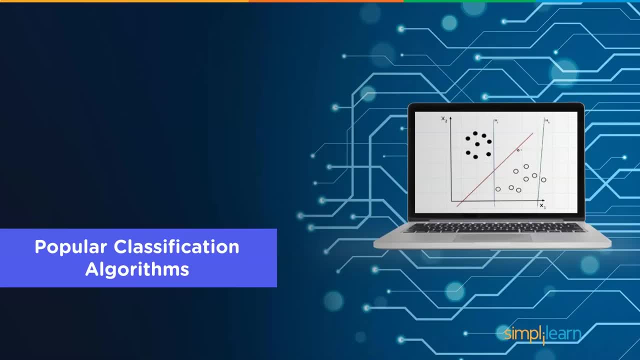 Classifying A, B, C, D and then classifying words to go with that. So let's go ahead and roll our sleeves up and take a look at some popular classification algorithms. Before we look at the algorithms, let's go back and take a look at our definitions. 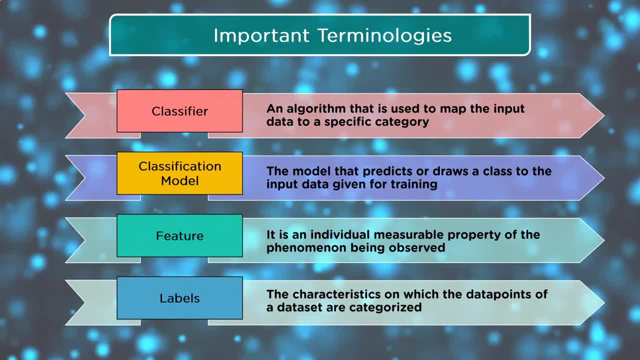 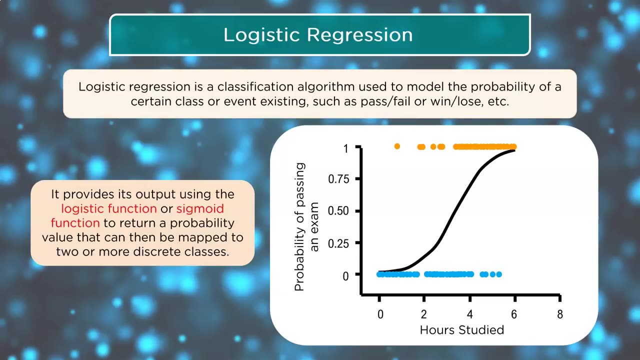 We have a classifier and a classification model. So we're looking at the classifier, An algorithm that is used to map the input data to a specific category. One of those algorithms is a logistic regression. The logistic regression is a classification algorithm used to model the probability of a certain class or event existing, such as pass, fail or win, lose, etc. 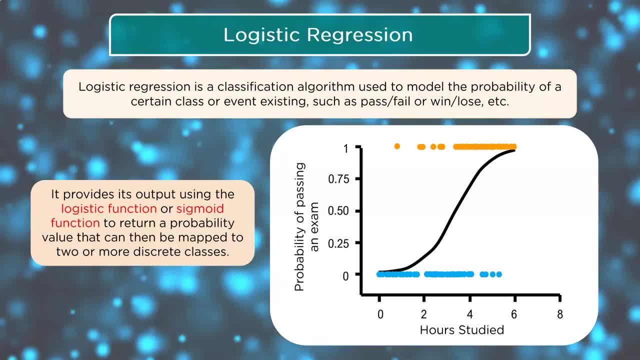 It provides its output using the logistic function or sigmoid function to return the probability value that can then be mapped to two or more discrete classes. A sigmoid function is an activation function that fits the variable and limits the output to a range between 0 and 1.. 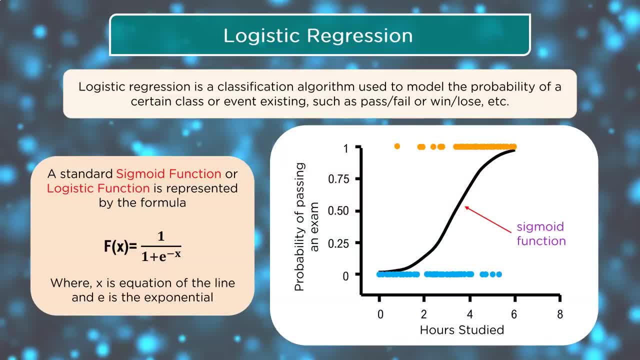 The standard sigmoid function or logistic function is represented by the formula: fx equals 1 over 1 plus e to the minus x, Where x is the equation of the line and e is the exponential. Just taking a quick look at this, You can think of this as being a point of uncertainty. 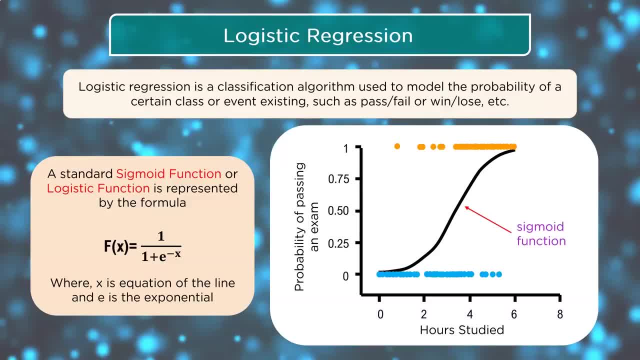 And so as we get closer and closer to the middle of the line, it's either activated or not, And we want to make that just shoot way up, So you'll see a lot of the activation of the line. The activation formula is kind of have this nice s-curve where it approaches 1 and approaches 0.. 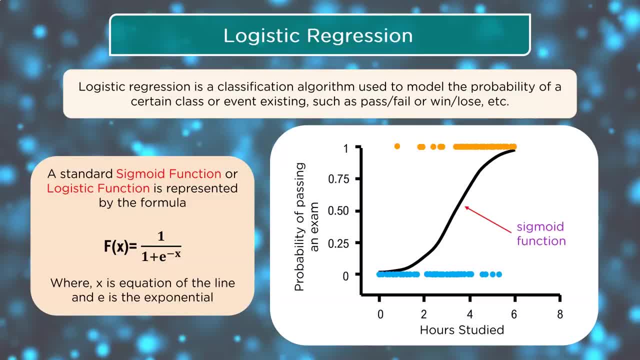 And based on that there's only a small region of error. And so you can see in the sigmoid logistic function the 1 over 1 plus e, minus x to the minus x. You can see it frames that nice s-curve. 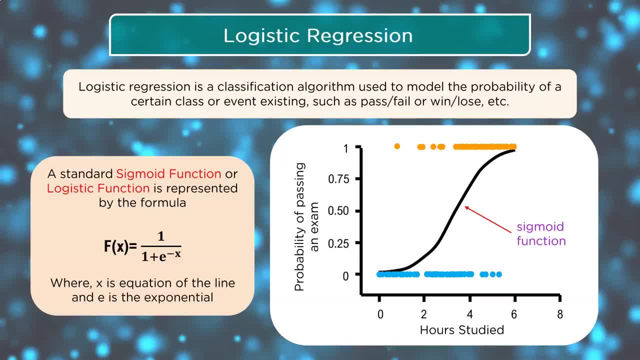 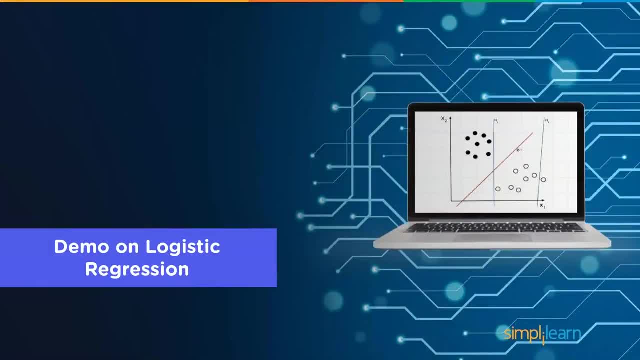 We also can use a tangent variation. There's a lot of other different models here. as far as the actual algorithm, This is the most commonly used one. Let's go ahead and roll up our sleeves And take a look at a demo. This is going to use a logistic regression. 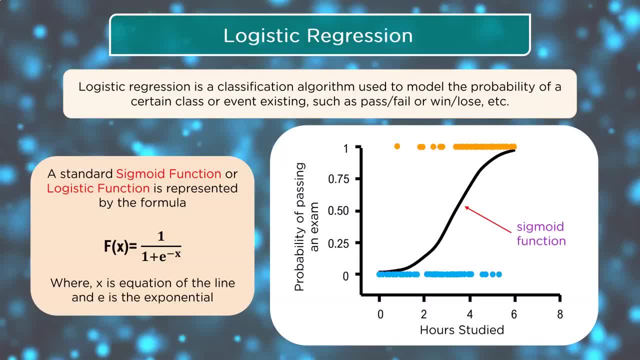 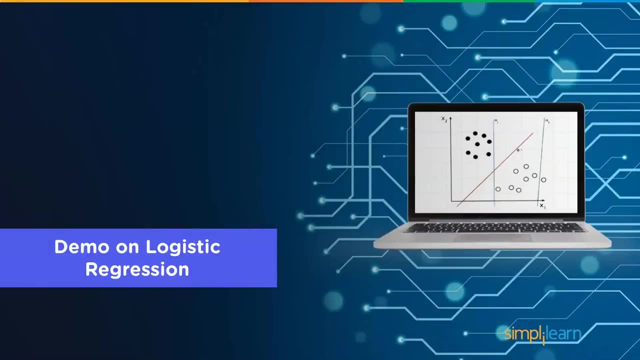 the 1 over 1 plus e minus x to the minus x. you can see a famous, that nice s-curve. we also can use a tangent variation. there's a lot of other different models here. as far as the actual algorithm, This is the most commonly used one. Let's go ahead and roll up our sleeves and take 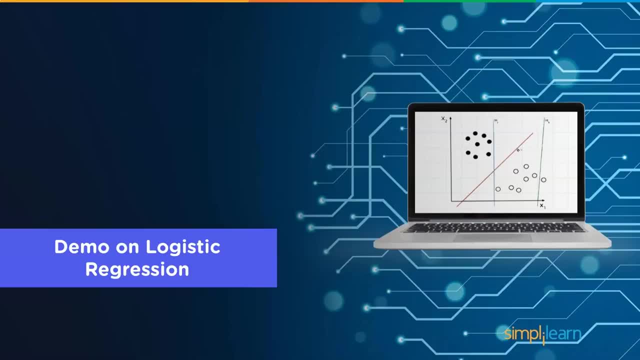 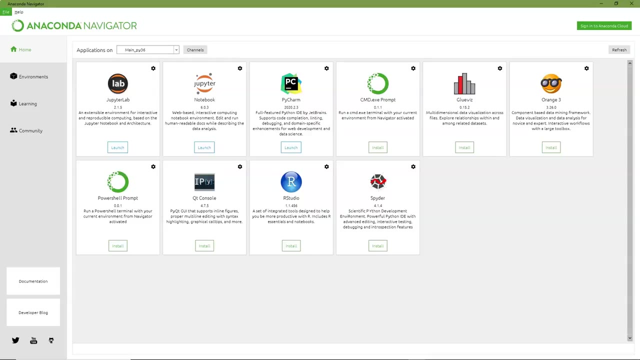 a look at a demonstration. This is a demo that is going to use a logistic regression. so we're going to have the activation formula and the model, because you have to have, you have to have both. For this we will go into our Jupyter notebook Now. I personally use the anaconda navigator to open up the Jupyter notebook to set. 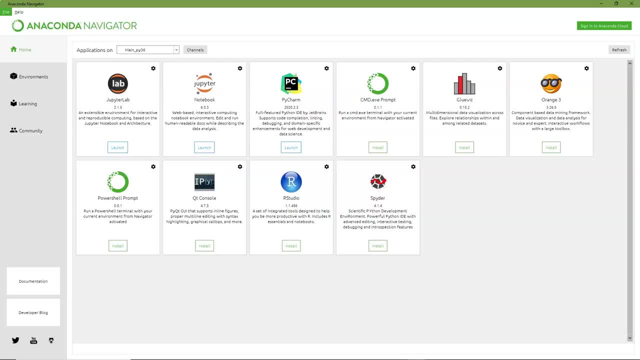 up my IDE as a web-based. It's got some advantages that it's very easy to display in, but it also has some disadvantages in that if you're trying to do multi threads and multi processing you start running into a lot of problems. So I'm going to go ahead and jump to single git issues with python and then I jump to Pycharm. 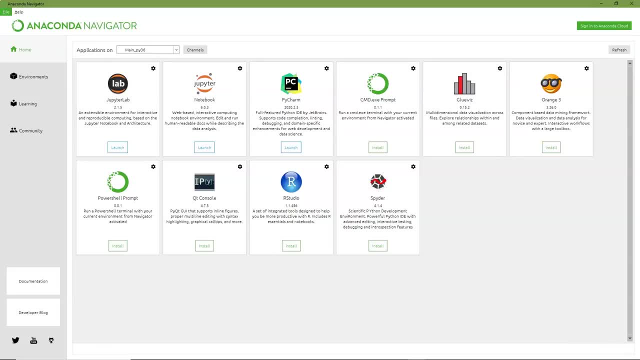 Really depends on whatever IDE you want. Just make sure you've installed numpy and the sklearn modules into your python, in whatever environment you're working in, so that you'll have access to that for this demo. Now the team in the back has prepared my code for me, which I'll start bringing. 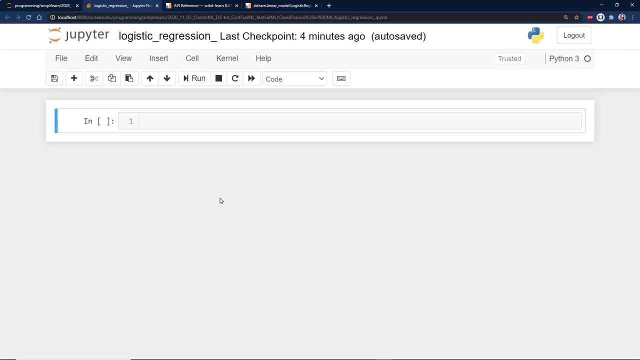 in one section at a time so we can go through it Before we do that. it's always nice to actually see where this information is coming from and what we're working with. So the first part is we're going to import our packages, which you need to install into your. 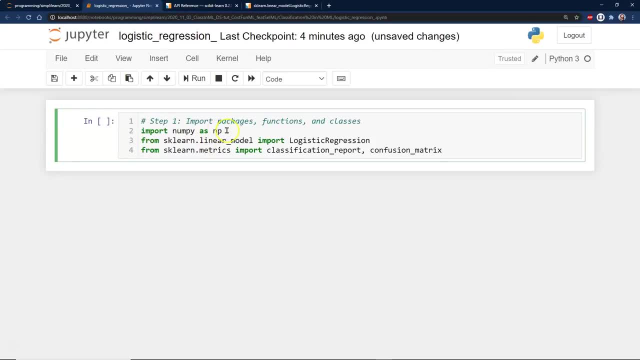 python and that's going to be your numpy. We usually use numpy as in p. and then from sklearn, the learn model, we're going to use a logistic regression and from sklearn metrics we're going to import the classification report, confusion, matrix, And if we go ahead and open up the 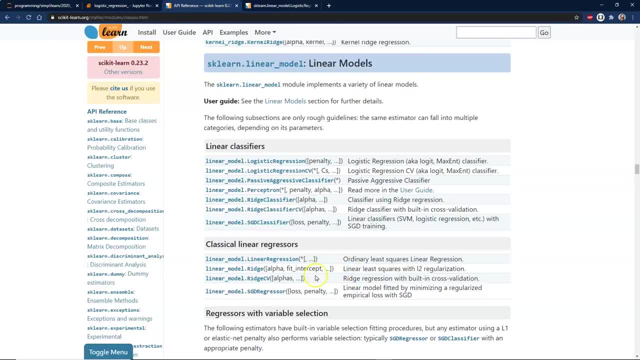 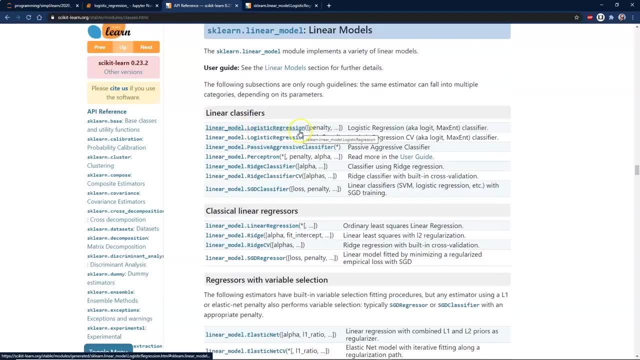 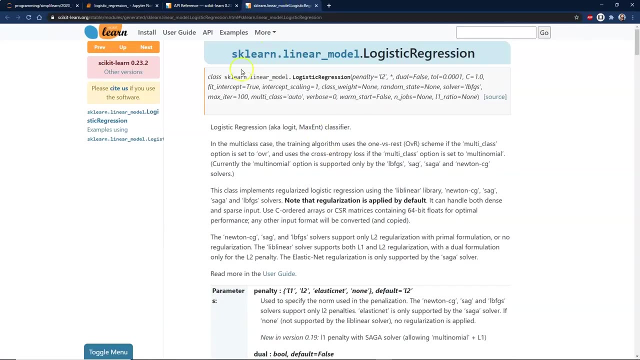 scikit-learnorg and go under their API, you can see all the different features and models they have. And we're looking at the linear model, logistic regression, one of the more common classifiers out there, And if we go ahead and go into that and dig a little deeper, you'll see here where they. 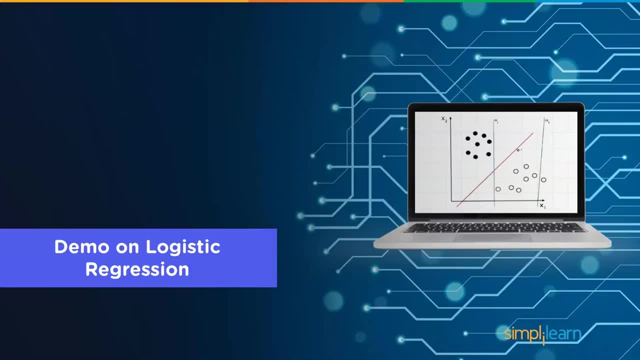 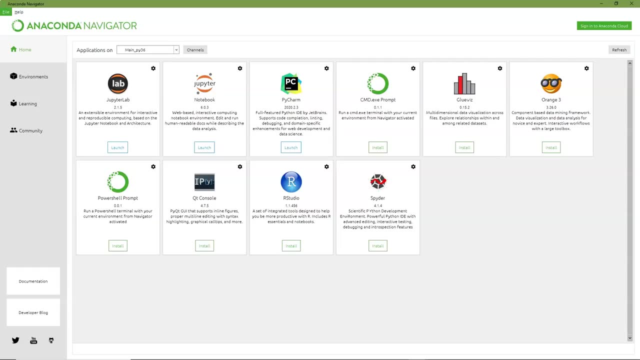 So we're going to have the activation formula and the model, Because you have to have both. For this we will go into our Jupyter notebook Now. I personally use the Anaconda Navigator to open up the Jupyter notebook to set up my IDE as a web-based. 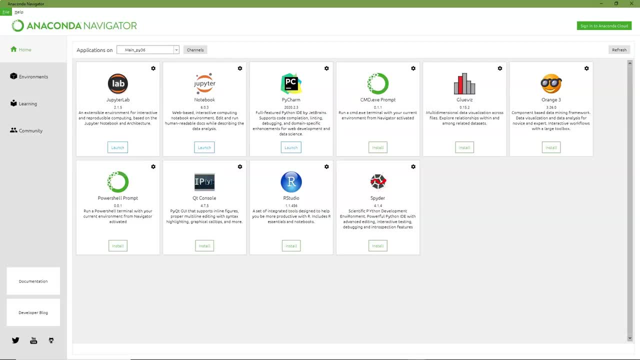 It's got some advantages that it's very easy to display in, But it also has some disadvantages in that if you're trying to do multi-threads and multi-processing, you start running into some problems. For example, I run into some single-git issues with Python. 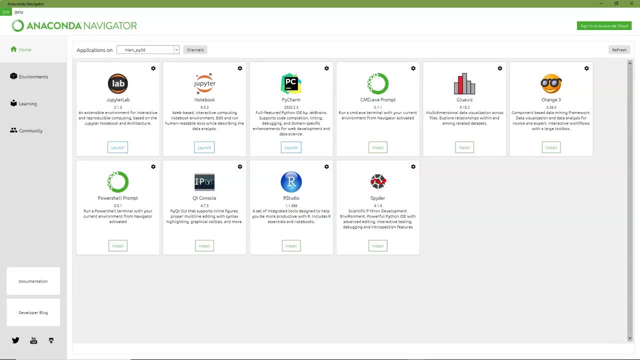 And then I jump to PyCharm. It really depends on whatever IDE you want. Just make sure you've installed numpy and the sklearn modules into your Python in whatever environment you're working in, so that you'll have access to that for this demo. 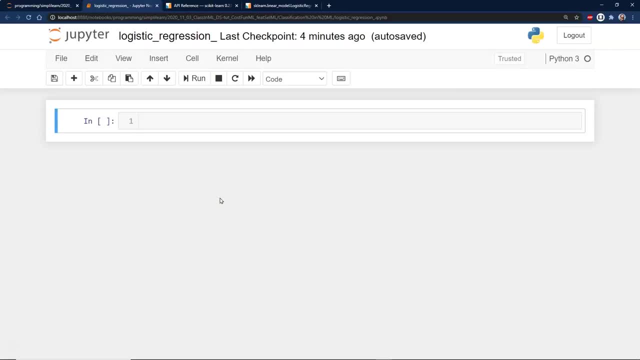 Now the team in the back has prepared my code for me, which I'll start bringing in one section at a time so we can go through it Before we do that. it's always nice to actually see where this information is coming from and what we're working with. 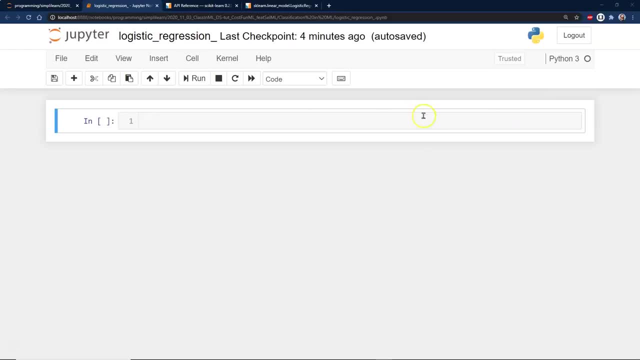 So the first part is we're going to import our packages which you need to install into your Python, And that's going to be your numpy. We usually use numpy as in P, And then from sklearn, the learn model, we're going to use a logistic regression. 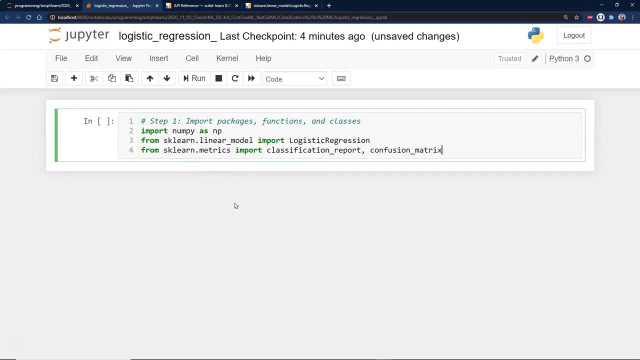 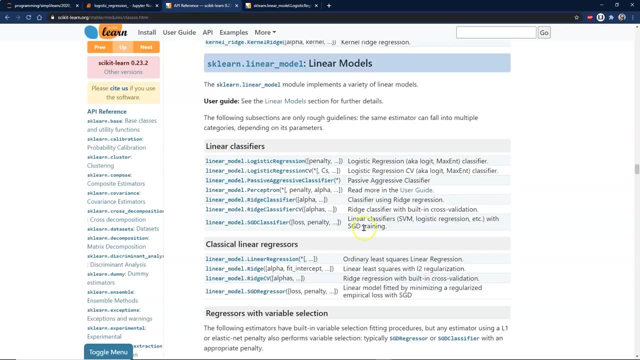 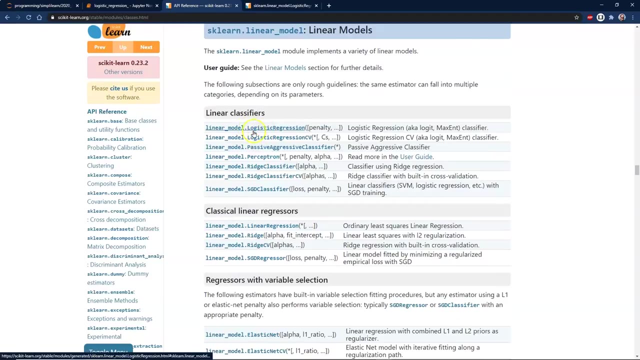 And from sklearn metrics we're going to import the classification report, confusion matrix, And if we go ahead and open up the scikit-learnorg and go under their API, you can see all the different features and models they have And we're looking at the linear model, logistic regression. 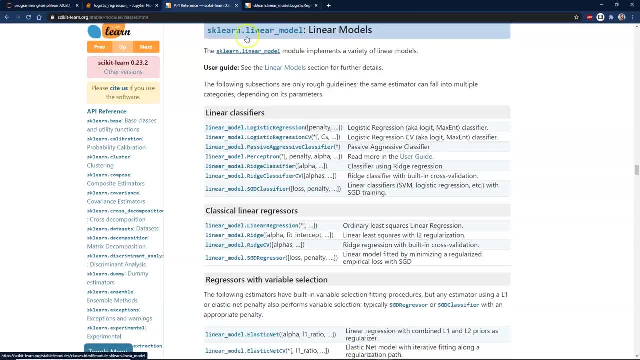 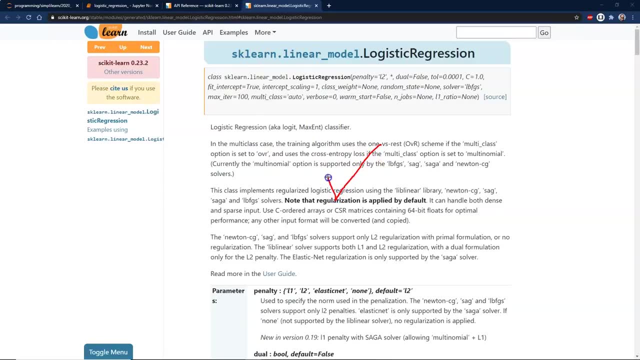 one of the more common classifiers out there And if we go ahead and go into that and dig a little deeper, you'll see here where they have the different settings. It even says right here: note: the regularization is applied by default. So by default that is the activation formula being used. 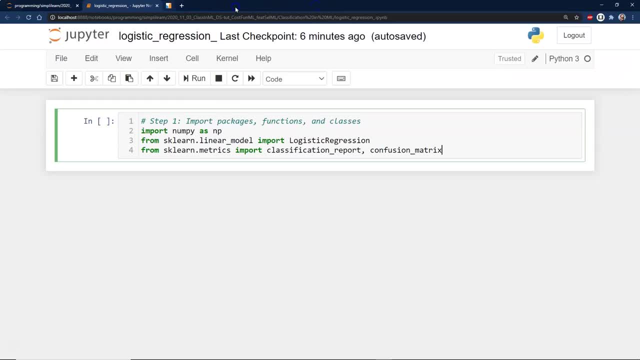 Now we're not going to spend. we might come back to this. look at some of the other models, because it's always good to see what you're working with, But let's go ahead and jump back in here And we have our imports. 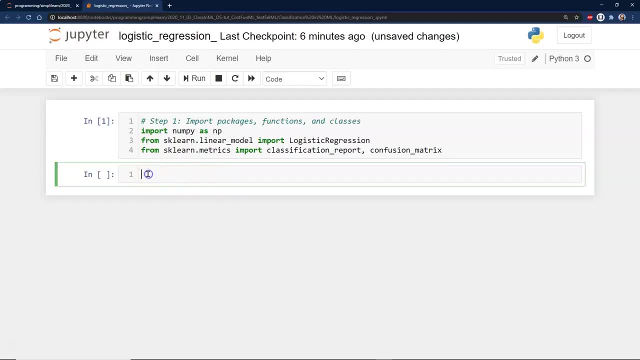 We're going to go ahead and run those. So these are now available to us as we go through our Jupyter notebook script And they put together a little piece of data for us. This is simply going through 0 to 1.. Actually, let's go ahead and print this out over here. 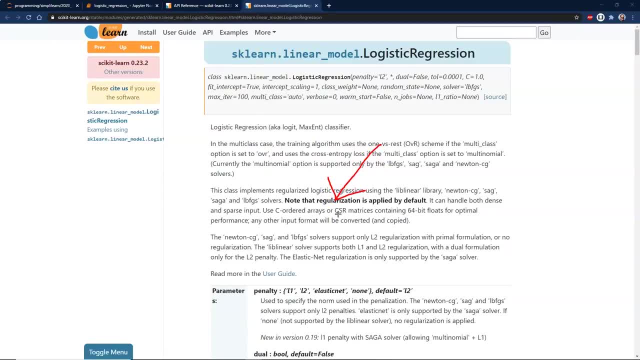 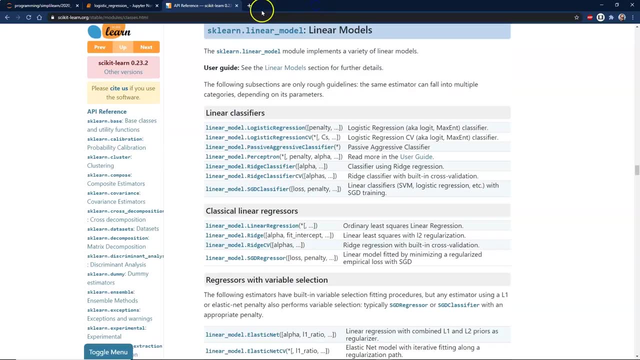 have the different settings. It even says right here: note: the regularization is applied by default. So by default, that is the activation formula being used. Now we're not going to spend. we might come back to this. look at some of the other models, because it's always good to see what you're. 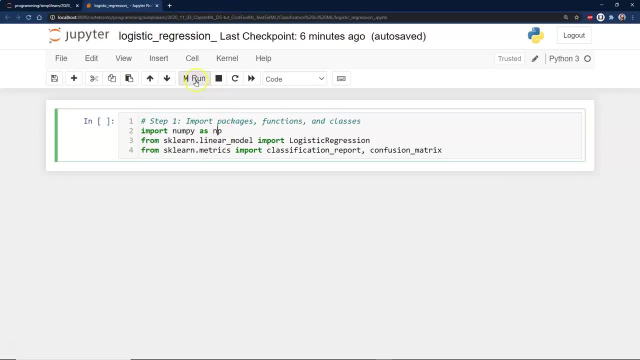 working with. But let's go ahead and jump back in here and we have our imports we're going to go through. So these are now available to us as we go through our Jupyter notebook script And they put together a little piece of data for us. This is simply going through 0 to 1.. Actually, let's go. 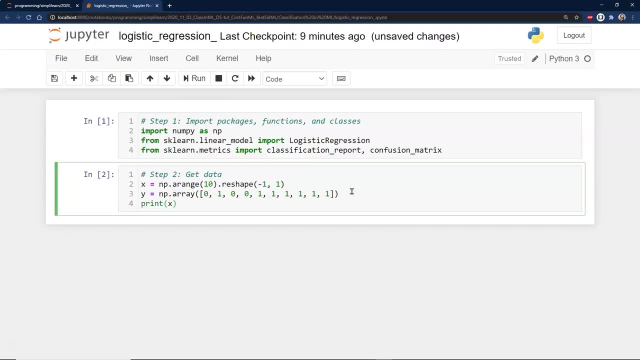 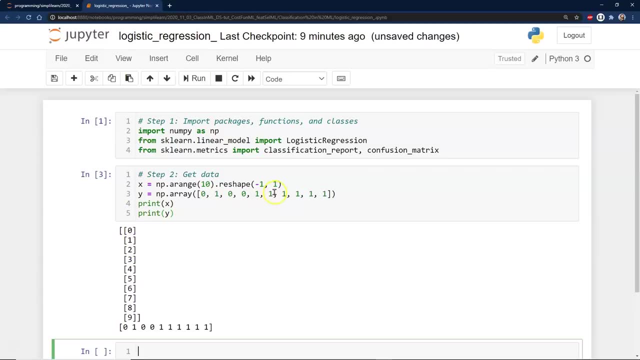 ahead and print this out over here. We'll go ahead and print x just so you can see what we're actually looking for, And when we run this you can see that we have our x is 0, 1, 2 through 9.. We reshaped it. 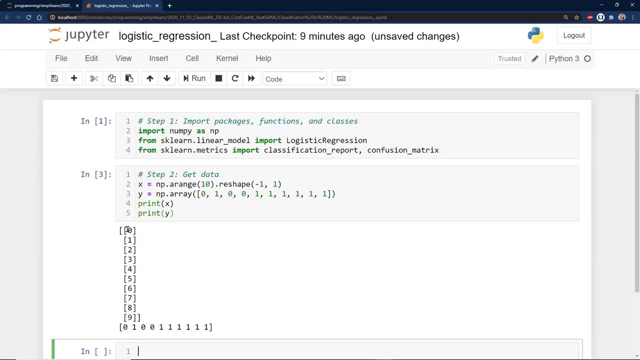 The reason for this is just looking for a row of data. Usually we have multiple features. We just have the one feature, which happens to be 0 through 9.. So we're going to go ahead and print this out over here And then we have our 10 answers right down here: 0 1 0, 0, 1 1, 1, 1, 1, 1.. You can bring in a lot. 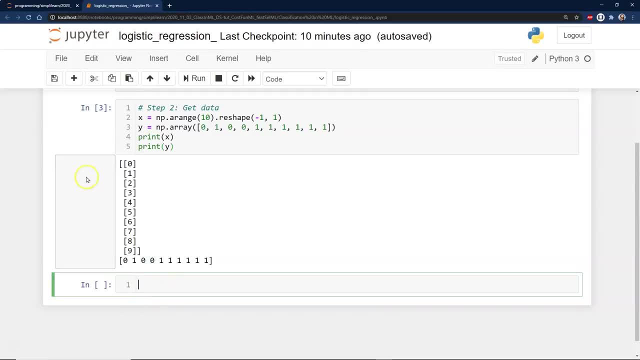 of different data, depending on what you're working with. You can make your own, You can. instead of having this as just a single, you could actually have like multiple features in here, But we just have the one feature for this particular demo, And this is really where all the magic happens, right? 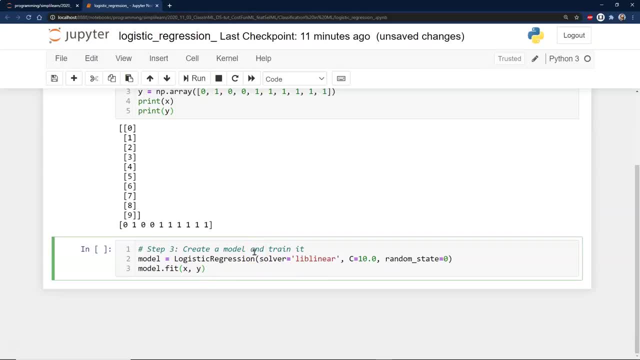 here And I told you it's like a black box. That's the part that is kind of hard to follow, And so if we have our model- we talked about the model right there- and then we went ahead and set it for library linear. As I showed you earlier, that's actually default, so it's not that important. Random state. 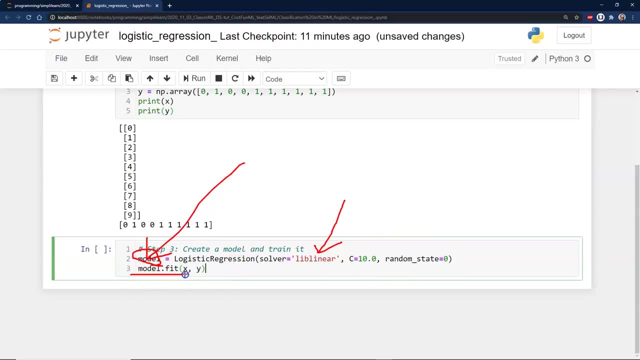 equals zero. This stuff you don't worry too much about And then with the scikit learn, you'll see the model fit. This is very common to scikit. They use similar stuff in a lot of other different packages, But you'll see that that's very common. You have to fit your data And that means we're. 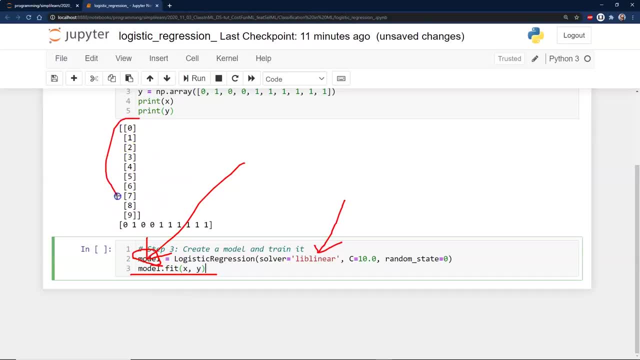 just taking the data and we're fitting it in the model And then we're going to go ahead and print something, Our x right here, which is our features. That's our x And here's y. These are the labels we're looking for. So, before we were looking at, is it fraud, Is it not? Is it cat? Is it not That? 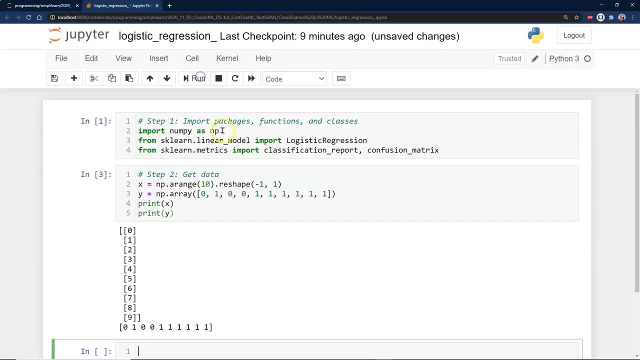 We'll go ahead and print x, just so you can see what we're actually looking for And when we run this, you can see that we have our x is 0,, 1,, 2 through 9.. We reshaped it. 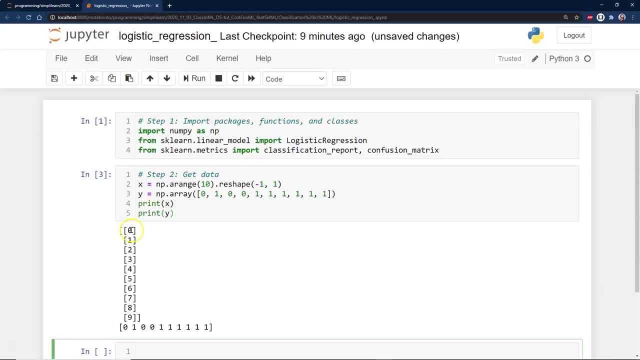 The reason for this is just looking for a row of data. Usually we have multiple features. We just have the one feature, which happens to be 0 through 9.. And then we have our 10 answers right down here: 0, 1, 0, 0, 1, 1, 1, 1, 1, 1.. 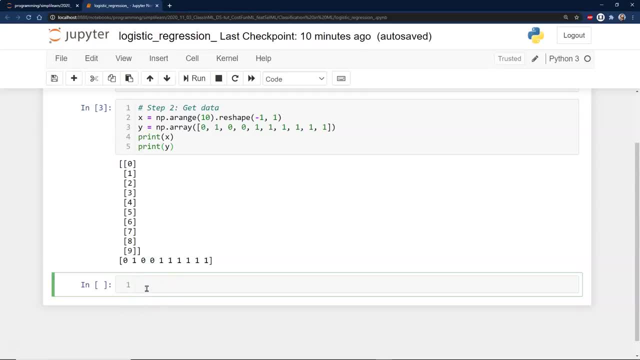 You can bring in a lot of different data depending on what you're working with. You can make your own, You can, instead of having this as just a single. you could actually have like multiple features in here, But we just have the one feature for this particular demo. 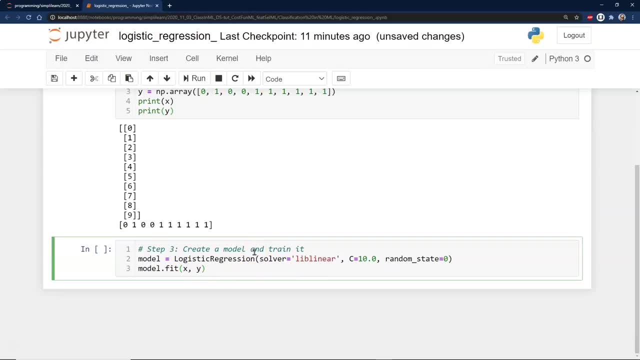 And this is really where all the magic happens, right here, And I told you it's like a black box. That's the part that is is is. It's kind of hard to follow, And so if you look right here, we have our model. 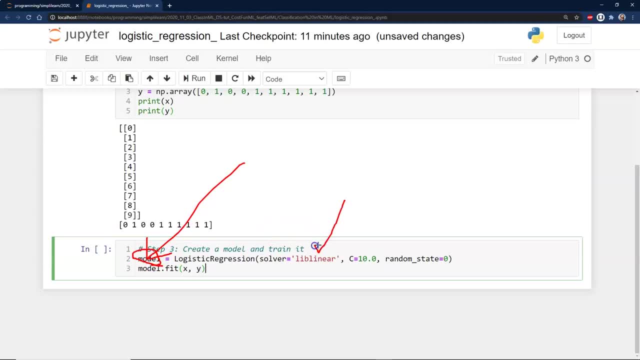 We talked about the model right there And then we went ahead and set it for library linear. As I showed you earlier, that's actually default, So it's not that important. Random state equals 0. This stuff you don't worry too much about. 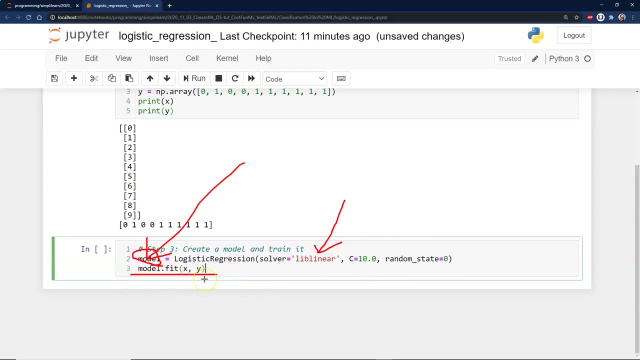 And then with the scikit learn, you'll see the model fit. This is very common to scikit. They use similar stuff in a lot of other different packages, But you'll you'll see that that's very common And you have to fit your data. 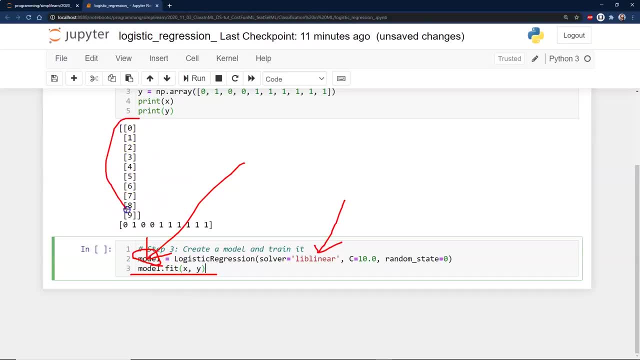 And that means we're just taking the data and we're fitting our x right here, which is our features. That's our x And here's y. These are the labels we're looking for, So before we were looking at, is it fraud? 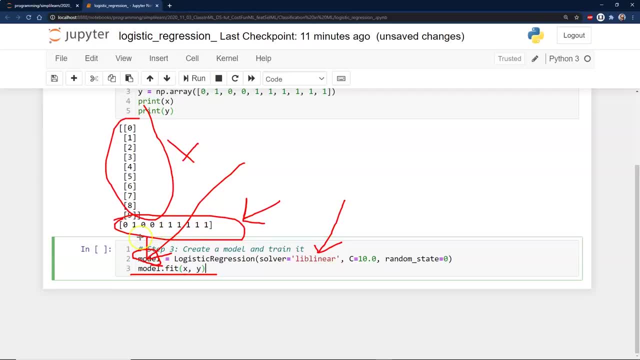 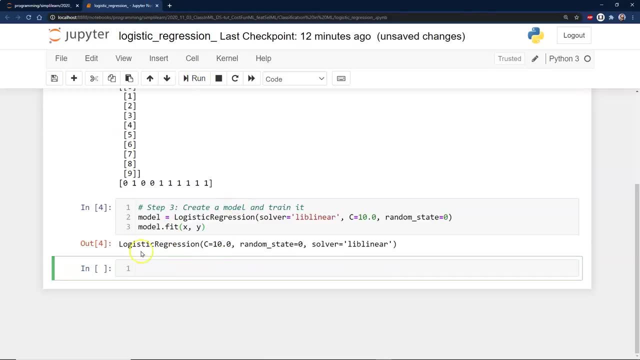 Is it not? Is it cat? Is it not That kind of thing? And this is looking at 01.. So we want to have a binary set up on this And we'll go ahead and run this. You can see right here. it just tells us what we loaded it with as our defaults. 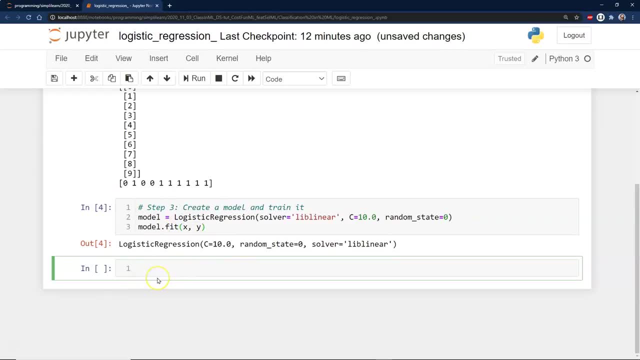 And you can see that this model has now been created And we've now fit our data to it. And then comes the fun part. You work really hard to clean your data, to bake it and cook it. There's all kinds of- I don't know why they go with the cooking terms. as far as how we get this data formatted, 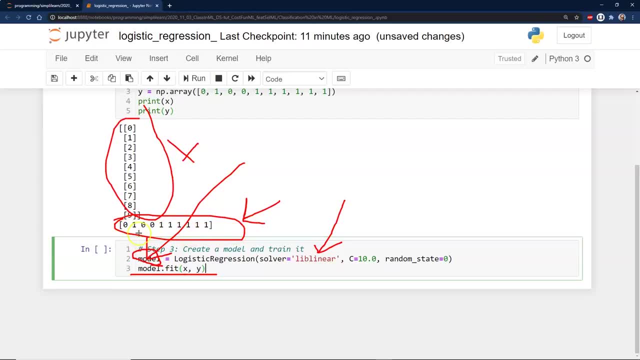 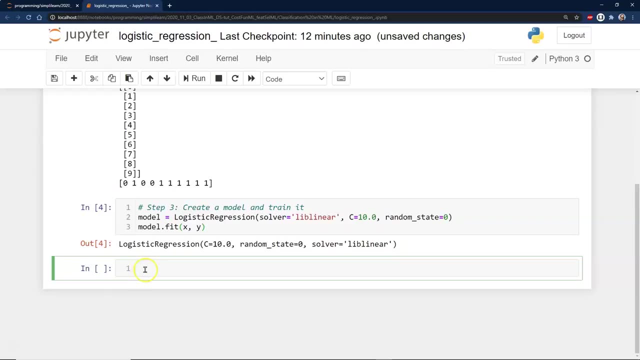 kind of thing, And this is looking at zero ones. We want to have a binary set up on this And we'll go ahead and run this. You can see right here. it just tells us what we loaded it with as our defaults And that this model has now been created And we've now fit our data to it. 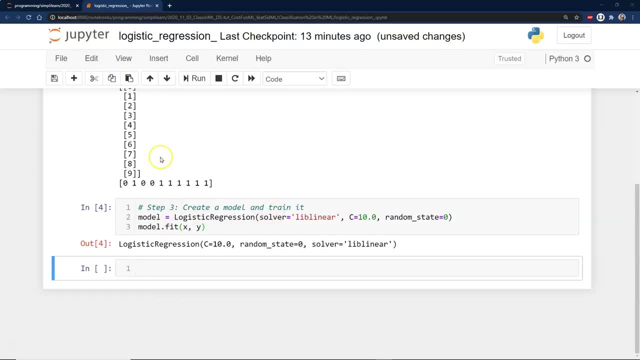 And then comes the next step: We're going to go ahead and print this, And then we're going to go ahead and put our data onto it And, as you can see, throughout this you see almost every single piece of this plugin, And I'm not saying that it's not all great big groups of stuff. 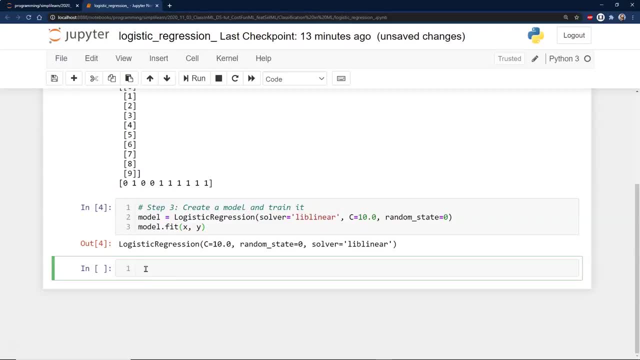 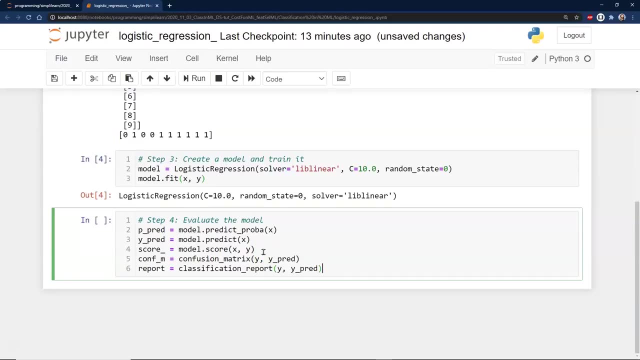 All I'm saying is that you don't have to worry about that. beta names in theウ. We need the eyelet heap value right there, Because you know if you don't want to have something walking over here at all. But we're going to pop it on here and I'll show you how it's going to. 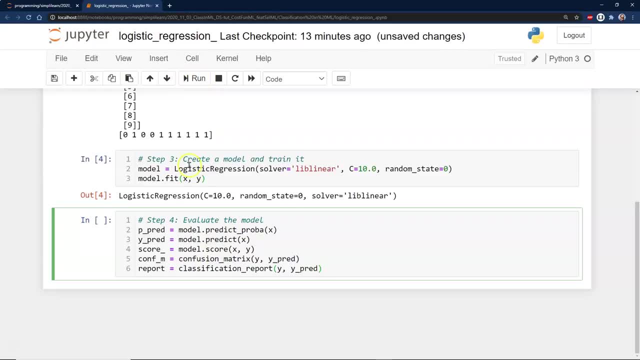 work. It's going to come automatically and we're going to overwrap or change the environment that we're庚 to something else. I mentioned tangent. that's one of the other common ones that's commonly used with language. for some reason, the tangent, even though it 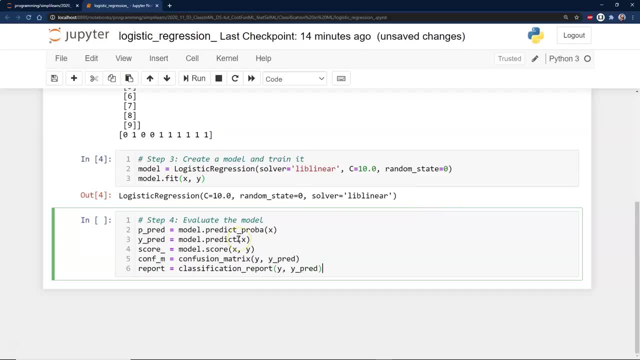 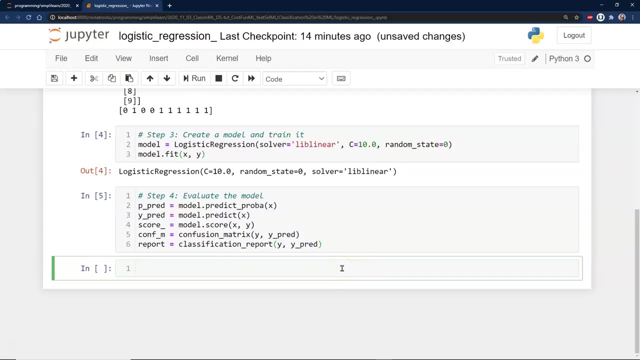 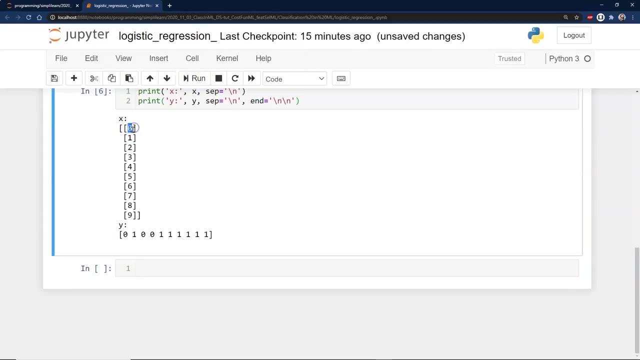 looks almost to be identical to the one we're using with the sigmoid function it. for some reason it activates better with language, even though it's a very small shift in the actual math behind it. we already looked at the data early, but we're going to look at it again. just you can see, we look at, we have our rows of. 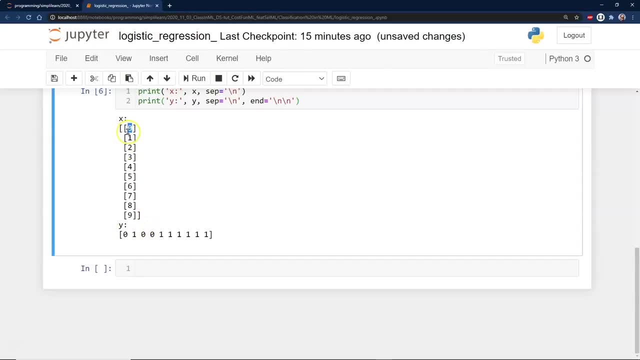 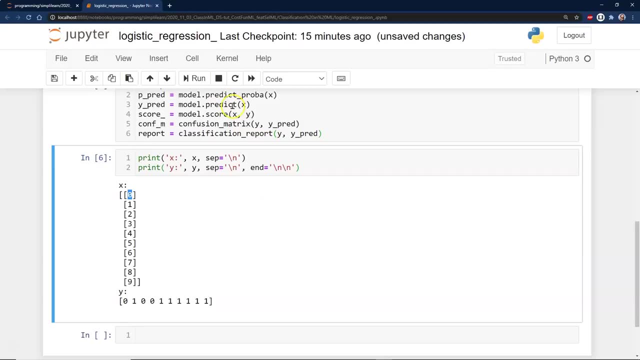 zero one row. it only has one entity and we have our output that matches these rows, and these do have to match. you'll get an error if you put in something with a different shape. so if you have ten rows of data and nine answers, it's gonna give you an error because you need to have ten answers for it. a lot of. 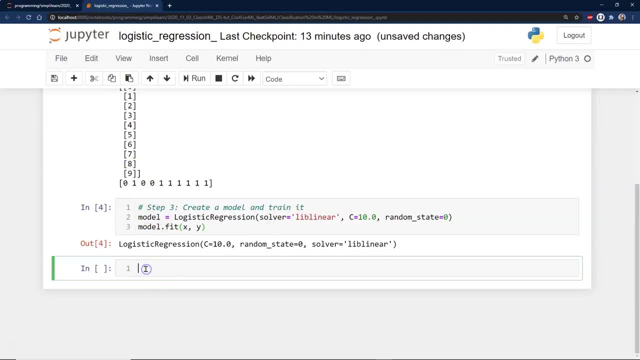 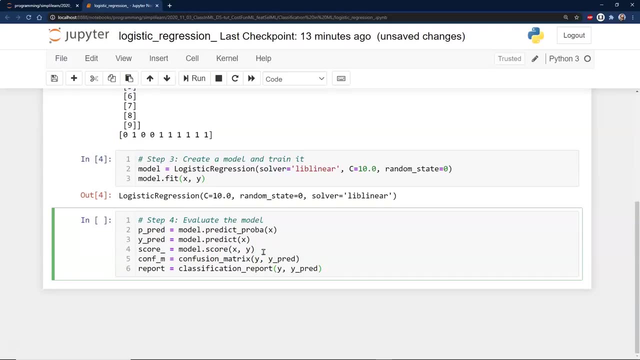 Then you go through and you pick your model, You pick your solver And you have to test it to see, hey, which one's going to be best. And so we want to go ahead and evaluate the model, And you do. this is that, once you've figured out which one is going to work the best for you, 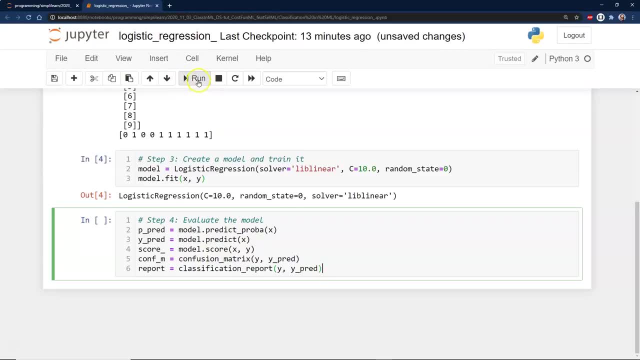 you evaluate it so you can compare it to your last model And you can either update it to create a new one or maybe change the solver to something else. I mentioned tangent. That's one of the other common ones that's commonly used with language. 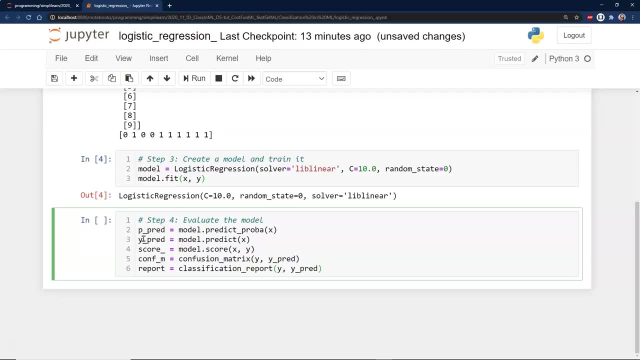 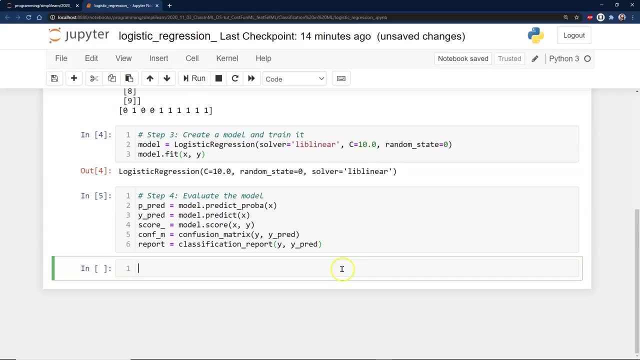 For some reason the tangent, even though it looks almost to me identical to the one we're using with the sigmoid function. for some reason it activates better with language, even though it's a very small shift in the actual math behind it. 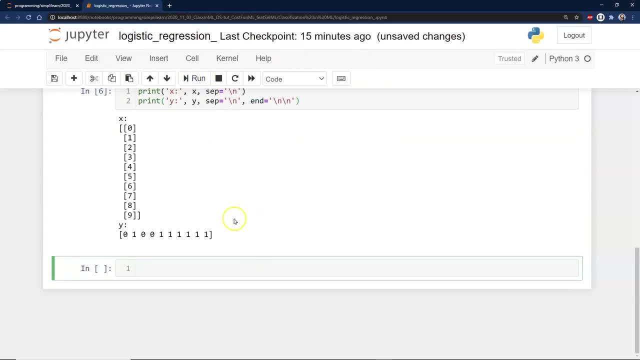 We already looked at the data early, But we're going to look at it again, Just so you can see what's going on. So we look at. we have our rows of 0, 1.. The row only has one entity. 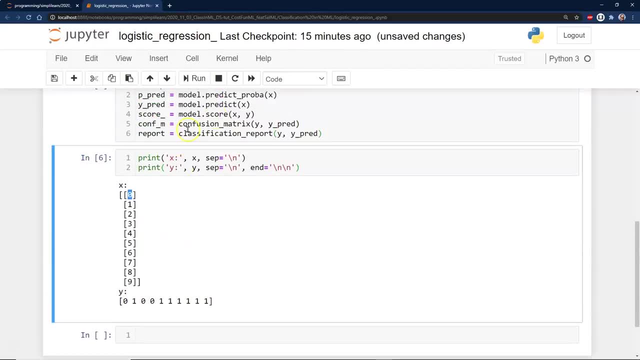 And we have our output that matches these rows, And these do have to match. You'll get an error if you put in something with a different shape. So if you have 10 rows of data and 9 answers, it's going to give you an error because you need to have 10 answers for it. 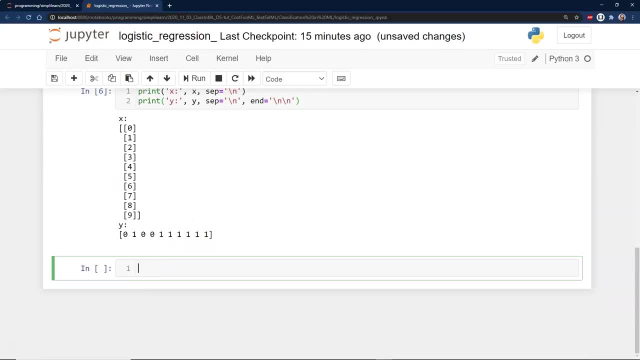 A lot of times you separate this too when you're doing larger models, But for this we're just going to take a quick look at that. The first thing we want to start looking at is the intercept, One of the features inside our linear regression model. 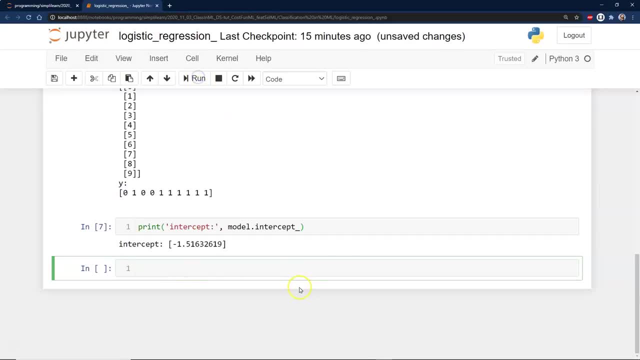 We'll go ahead and run that and print it. You'll see here we have an intercept of minus 1.516.. And if we're going to look at the intercept, we should also look at our coefficients. And if you run that you'll see that we get. our coefficient is the 0.7035.. 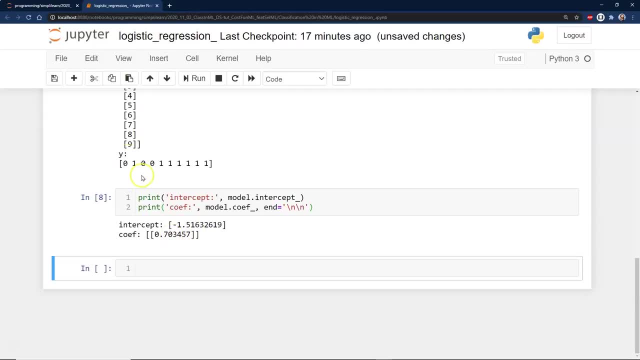 You can just think of this as your Euclidean geometry for a very basic model like this, where it intercepts the y at some point And we have a coefficient multiplying by it. A little more complicated in the back, But that is just this simple model with just the one feature in there. 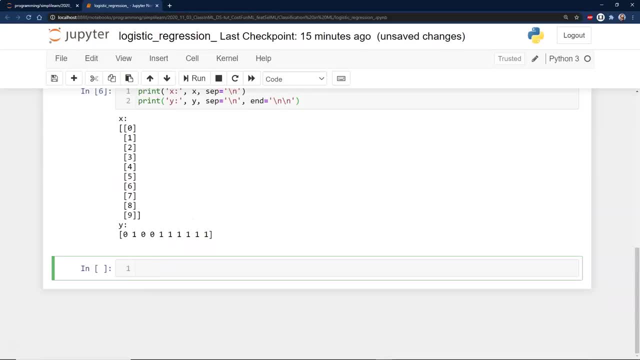 times you separate this too when you're doing larger models, but for this we're just going to take a quick look at that. the first thing we want to start looking at is the intercept, one of the features inside our linear regression model. we'll go ahead and run that in. 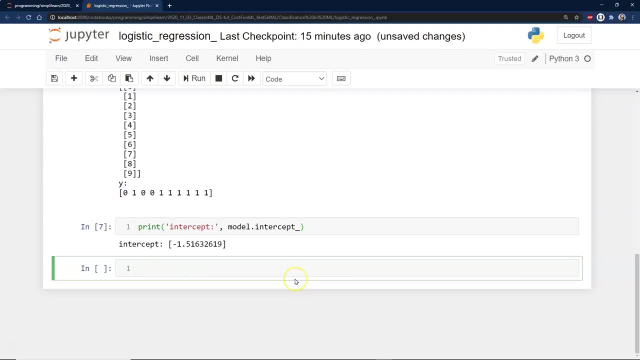 print it, you'll see. here we have an intercept of minus 1.516 and if we're gonna look at the intercept, we should also look at our coefficients. and if you run that, you'll see that we get a little, we get the. our coefficient is the point. 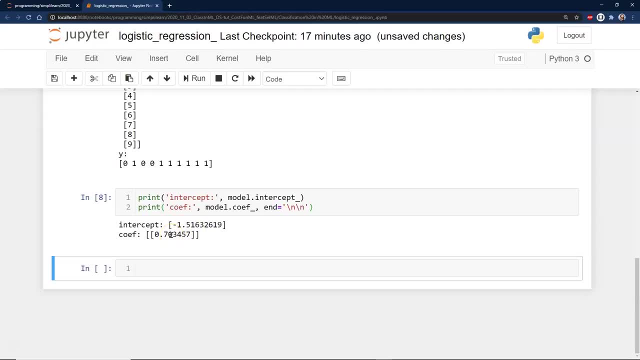 seven, oh three, five. you can just think of this as your Euclidean geometry for very basic model like this, where it intercepts the Y at some point and we have a coefficient multiplying by it. a little more complicated in the back end, but that is the gist of this simple model. 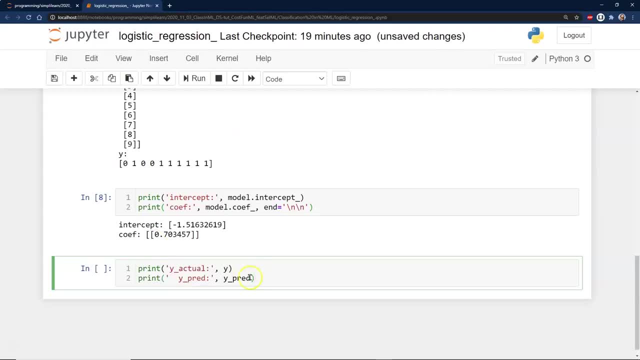 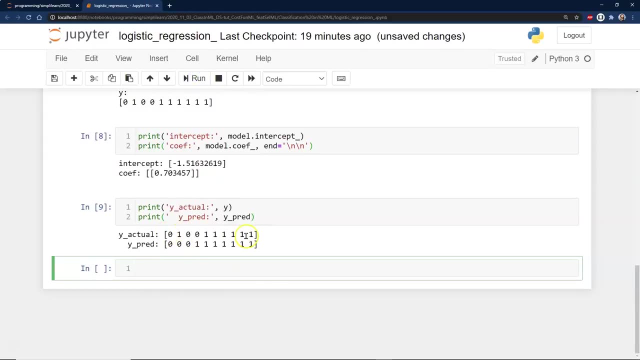 which is the one feature in there, and we'll go ahead and hope reprint the Y because I want to put them on top of each other with the Y predict, and so these were the Y values we put in and this is the Y predict we had coming out. 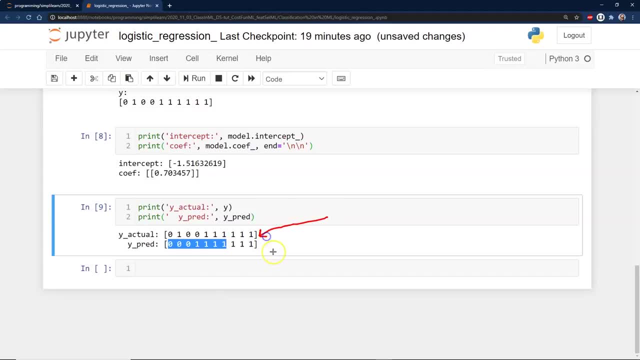 and you can see here we go, there's the Y actual and there's what the prediction comes in. now, keep in mind that we used the actual, complete data as part of our training. that is, if you're doing a real model of a big stopper right there, because you can't really see how good it did unless 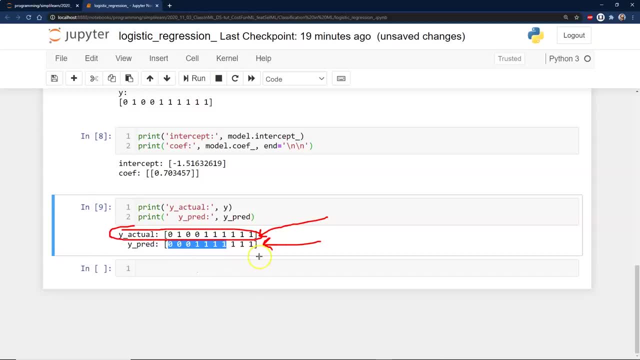 you split some data off to test it on. this is the first step. is you want to see how your model actually test on the data you trained it with and you can see here. there is this point right here where it has it wrong, and this point right here where it also has it wrong and it makes sense because we're going. 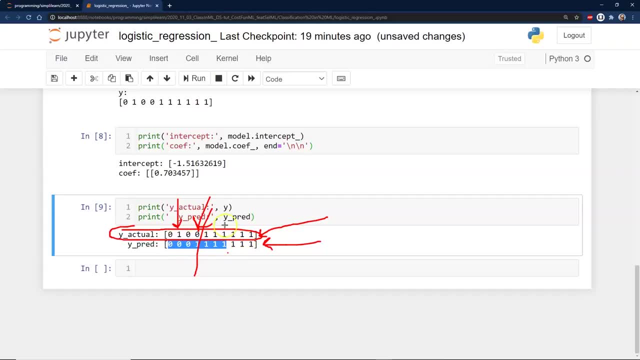 our input is zero, one through zero through nine- and it has to break it somewhere and this is where the break is. so it says this: half the data is gonna be zero, because that's what it looked like to me if I was looking at it without an algorithm, and this data is probably going to be one, and I didn't. I forgot to. 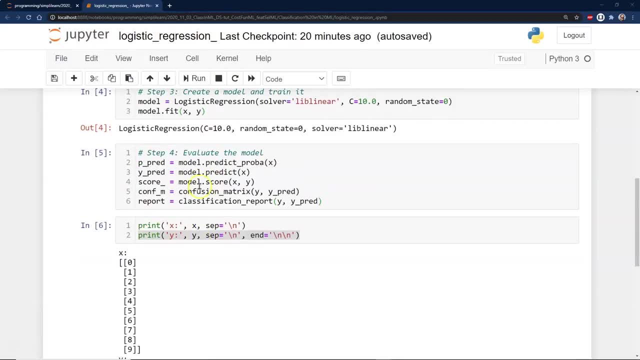 point this out. so let's go back up here. I just kind of glanced over this window here. we did a lot of stuff. let's go back and just take a look at that. what was done here is we ran a prediction, so this is where our predict comes in- is our 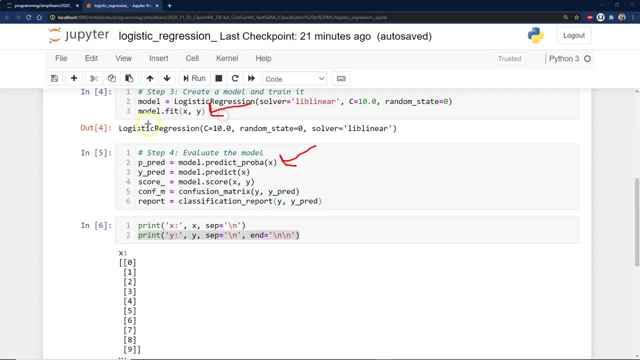 model dot predict. so we had a model fit. we created the model, we programmed it to give us the right answer. now we go ahead and predict what we think it's going to be. there's our model that predict probability of X, and then we have our Y predict, which is very similar, but this: 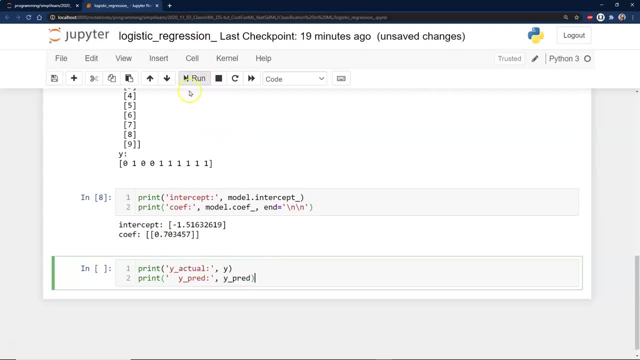 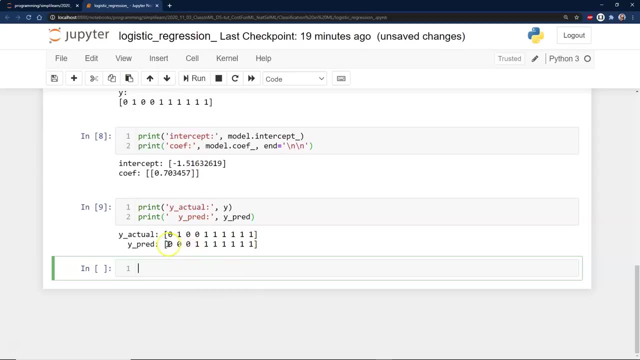 And we'll go ahead and we'll reprint the y because I want to put them on top of each other with the y predict, And so these were the y values we put in And this is the y predict we had coming out. And you can see, here we go. 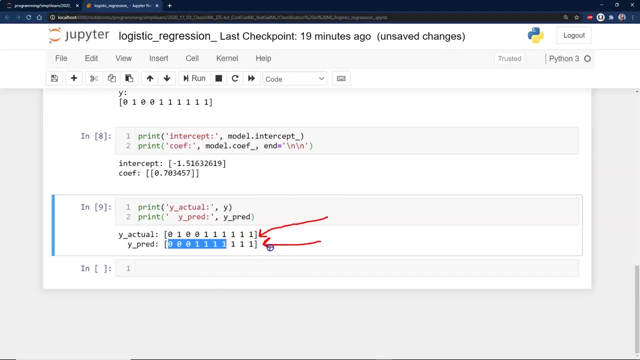 There's the y actual And there's what the prediction comes in. Now keep in mind that we used the actual, complete data As part of our training. That is, if you're doing a real model, a big stopper right there, because you can't really see how good it did unless you split some data off to test it on. 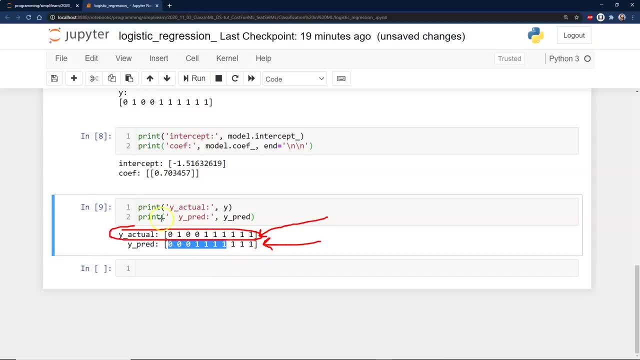 This is the first step- is you want to see how your model actually tests on the data you trained it with And you can see here- there is this point right here where it has it wrong And this point right here where it also has it wrong. 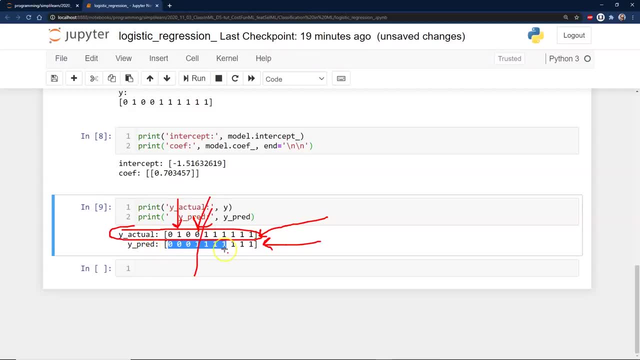 And it makes sense because we're going, our input is 0 through 9.. And it has to break it somewhere And this is where the break is. So it says this: half the data is going to be 0, because that's what it looked like to me if I was looking at it without an algorithm. 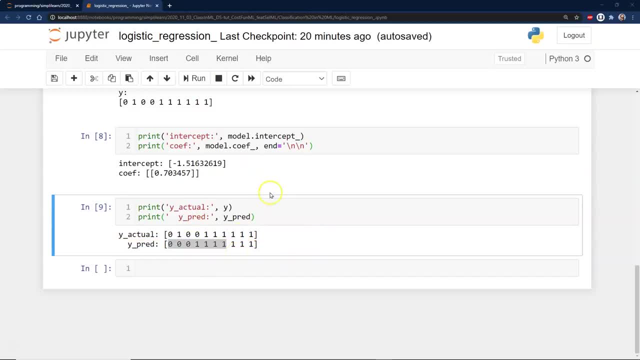 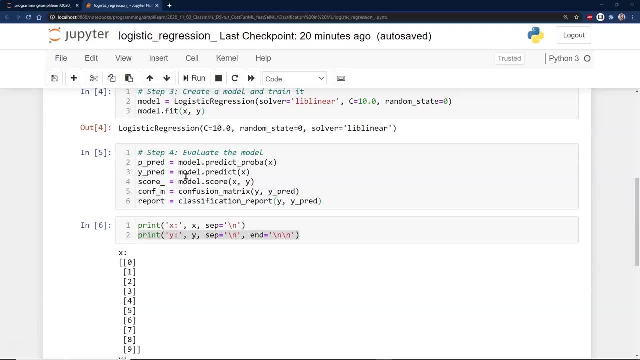 And this data is probably going to be 1.. And I forgot to point this out. So let's go back up here. I just kind of glanced over this window here where we did a lot of stuff. Let's go back and just take a look at that. 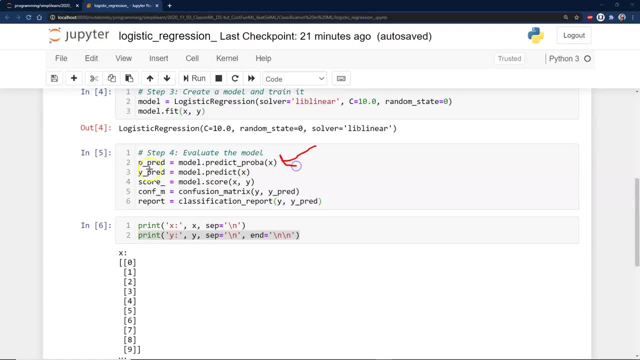 What was done here is we ran a prediction, So this is where our predict comes in, is our modelpredict. So we had a model fit. We created the model, We programmed it to give us the right answer. Now we go ahead and predict what we think it's going to be. 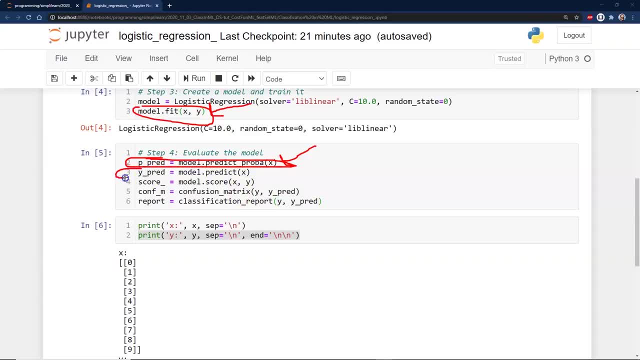 There's our modelpredict- probability of x- And then we have our ypredict, which is very similar, but this has to do more with the probability numbers. So, if you remember, down below we had the setup where we're looking at that sigmoid function. That's what this is returning. 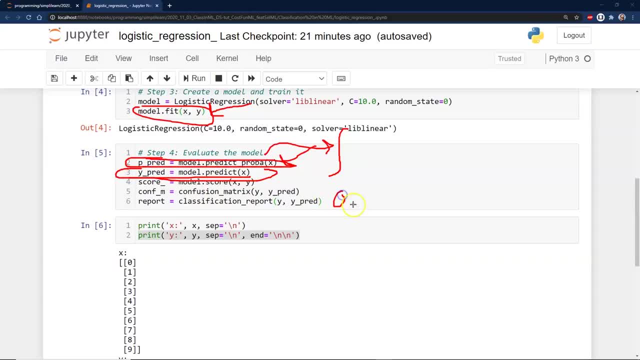 And the ypredict is returning a 0 or a 1.. And then we have our confusion matrix- We'll look at that- And we have our report, which just basically compares our y to our ypredict, which we just did. It's kind of nice. 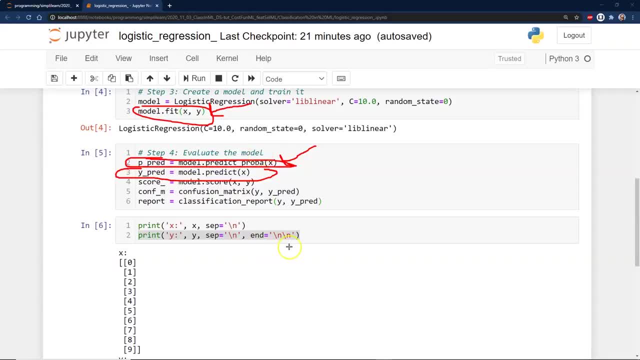 is has to do more with the probability numbers. so, if you remember, down below we had the setup where we're looking at that sigmoid function. that's what this is returning and the Y predict is returning a zero or a one. and then we have our confusion matrix. we'll look at that and we have our report, which just 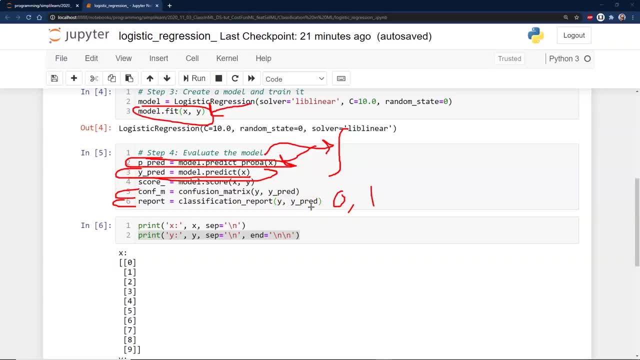 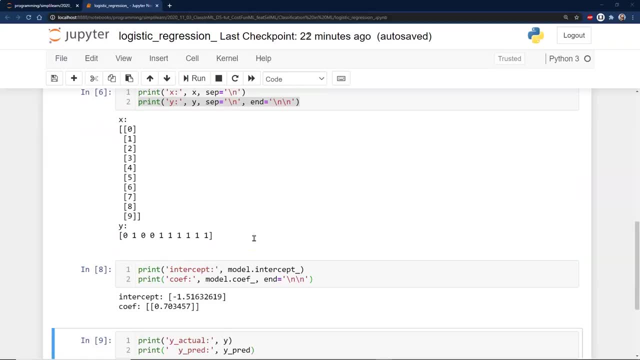 compares our Y to our Y predict, which we just did. it's kind of nice- a simple data, so it's really easy to see what we're doing. that's why we do is use the simple data. this can get really complicated when you have a lot of different. 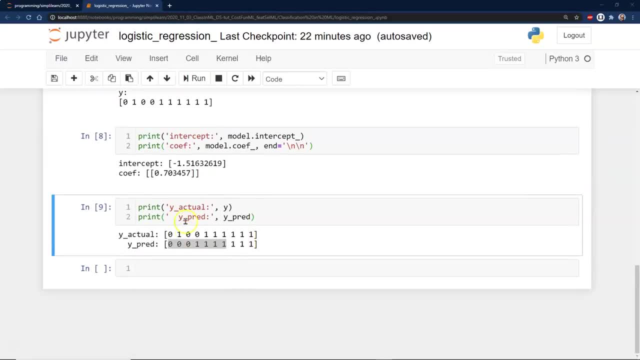 features and things going on and splits. so here we go. we've had our. I printed out our actual and our prediction. so this is the actual data, this is what the predict ran, and then we're go ahead and do. we're gonna print out the confusion matrix. we were just talking about that. this is great if you have a lot of data. to luck with the data. 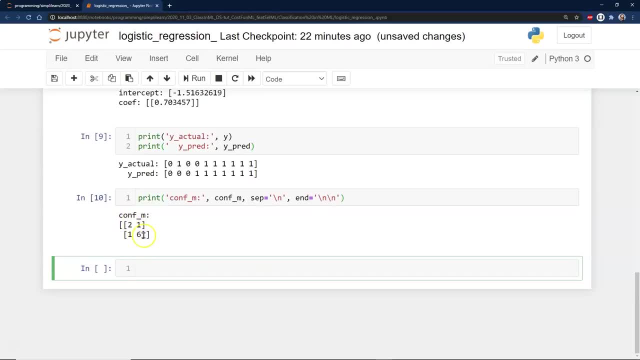 at. but you can see right here a confusion matrix says: if you remember from the confusion matrix, we have the two. this is two, correct, one, two. and it's been a while since I looked at a confusion matrix. there's the two and then we have this one which is our six. that's where the six comes from, and then 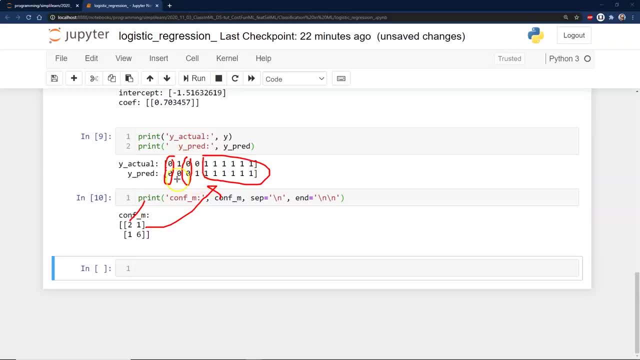 we have this one, which is the one false, this is the two one. so we have this one here and this one here which is misclassified. this really depends on what data you're working with as to what sure is important. you might be looking at this model and if this model, this confusion matrix, comes up and says that 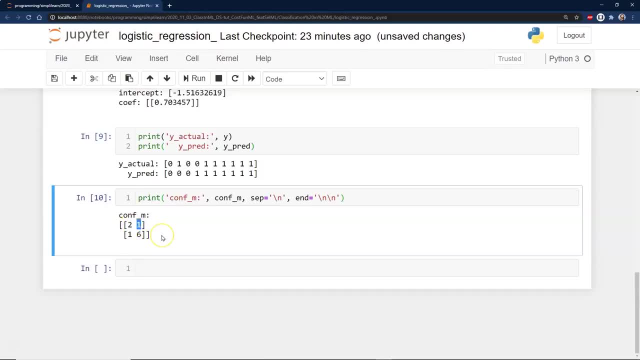 you've misclassified even one person as being non malignant cancer. that's a bad model. I wouldn't want that classification. I'd want this number to be zero. I wouldn't care if this false positive was a zero. I wouldn't care if this false positive was a zero. I wouldn't care if. 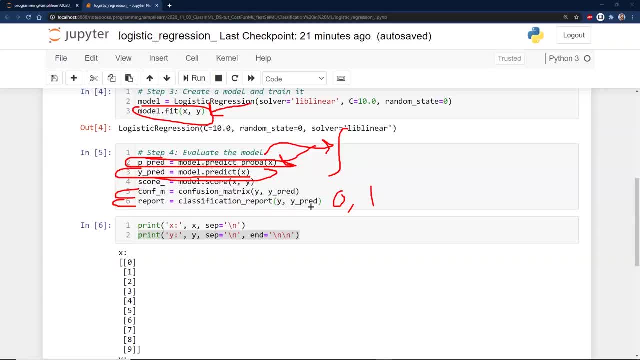 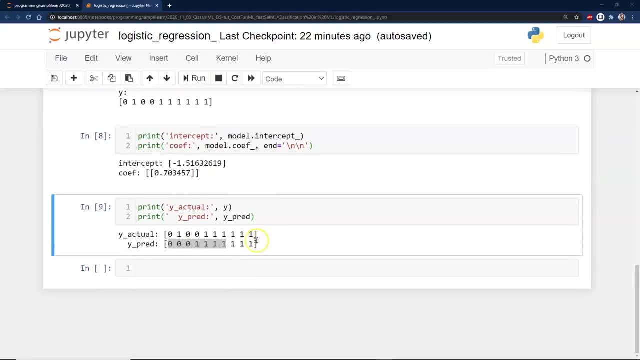 It's simple data so it's really easy to see what we're doing. That's why we use the simple data. This can get really complicated when you have a lot of different features and things going on and splits. So here we go. I printed out our actual and our prediction. 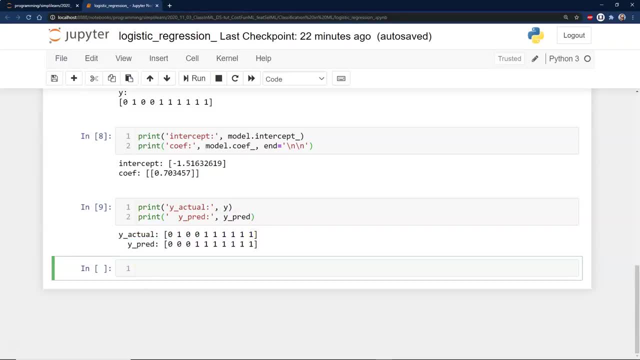 So this is the actual data, This is what the predict ran, And then we're going to go ahead and print out the confusion matrix. We were just talking about that. This is great if you have a lot of data to look at, But you can see right here: our confusion matrix says: if you remember, from the confusion matrix we have the 2.. 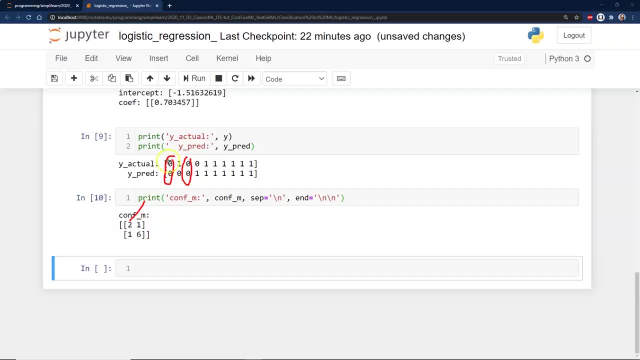 This is 2, correct 1, 2. And it's been a while since I looked at a confusion matrix. There's the 2. And then we have this one which is our 6. That's where the 6 comes from. 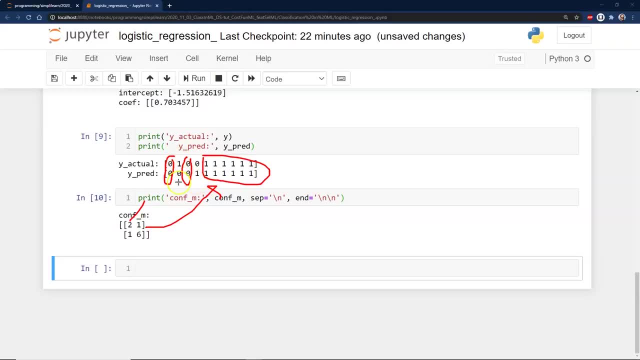 And then we have this one, which is the 1.. This is the 1 false. This is the 2 ones. So we have this one here and this one here which is misclassified. This really depends on what data you're working with as to what is important. 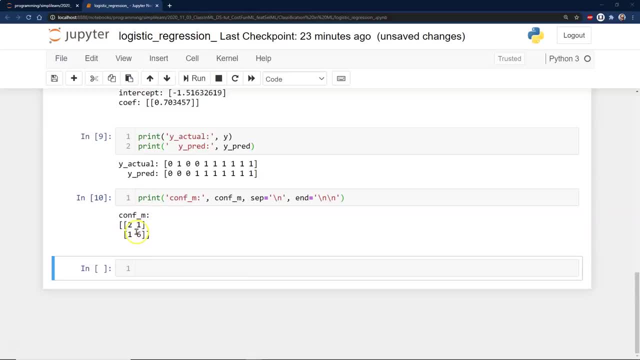 You might be looking at this model And if this confusion matrix comes up and says that you misclassified even one person as being nonmalignant cancer, that's a bad model. I wouldn't want that classification. I'd want this number to be 0.. 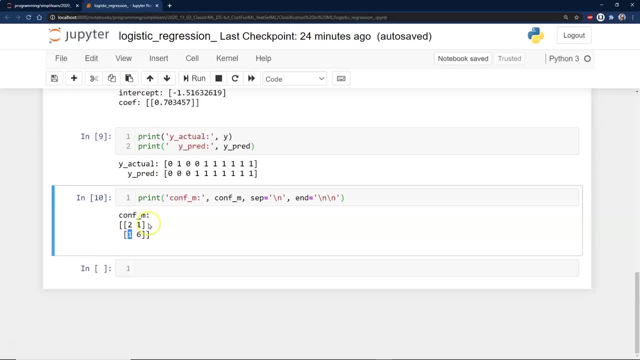 I wouldn't care if this false positive was off by a little bit more long, as I knew that I was correct on the important factor that I don't have cancer. So you can see that this confusion matrix really aims you in the right direction of what you need to change in your model, how you need to adjust it. 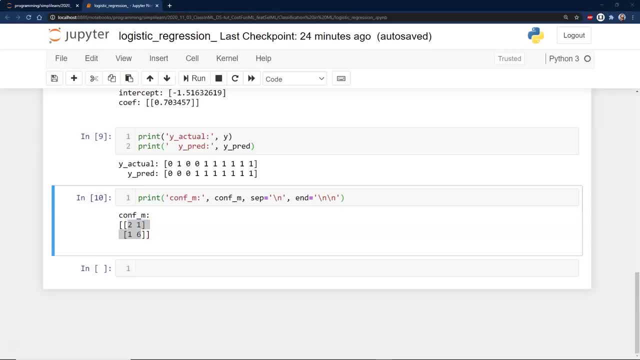 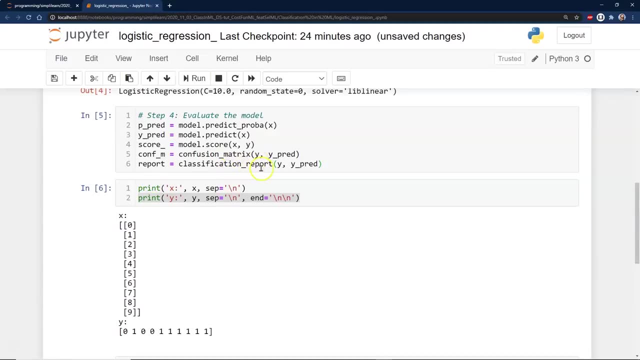 And then there's, of course, a report. Reports are always nice. If you notice, we generated a report earlier. We'll go and just print the report up And you can remember: this is our report. It's a classification report. Y, Y predict. 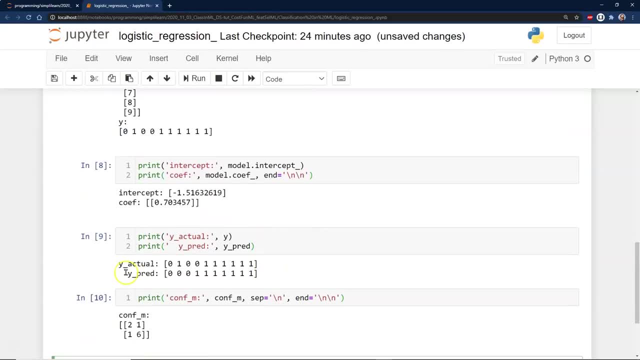 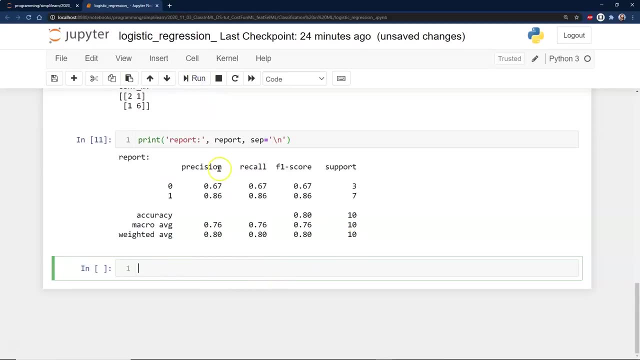 So we're just putting in our two values, Basically what we did here visually with our actual and our predicted value, And we'll go ahead and run the report And you can see it has the precision, the recall, your F1 score, your support. 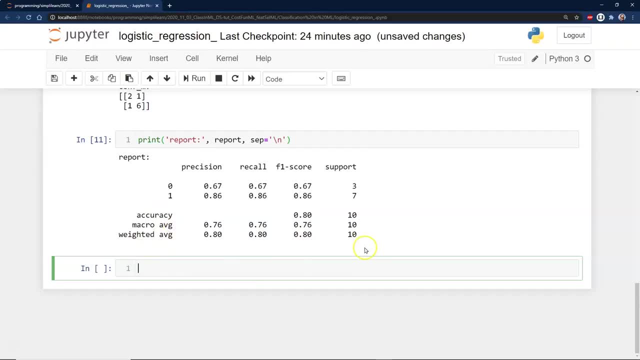 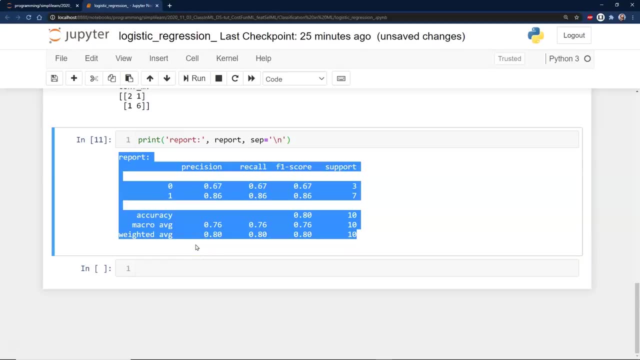 Translated into accuracy: macro average and weighted average, So it has all the numbers. A lot of times, when working with clients or with the shareholders in the company, this is really where you start, Because it has a lot of data And they can just kind of stare at it and try to figure it out. 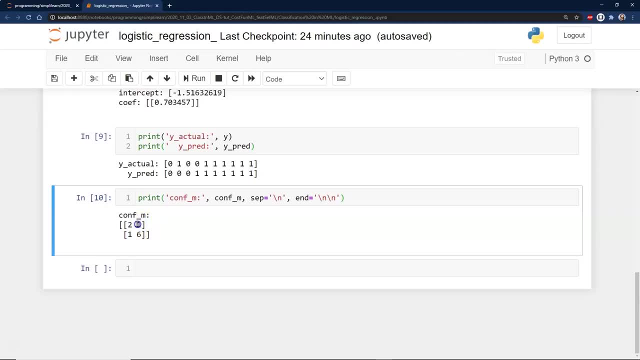 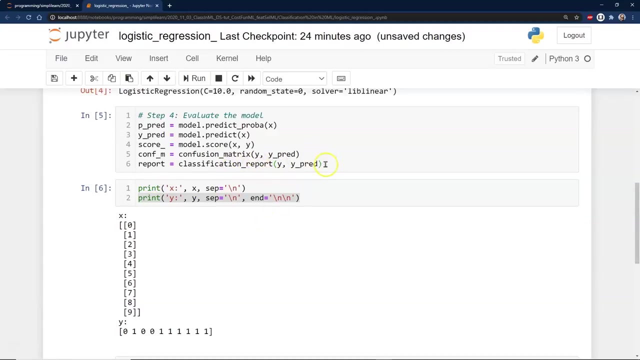 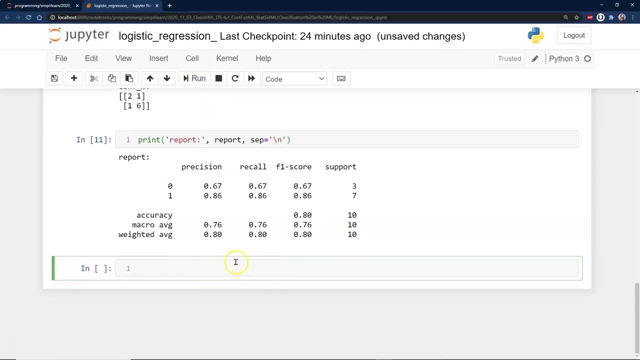 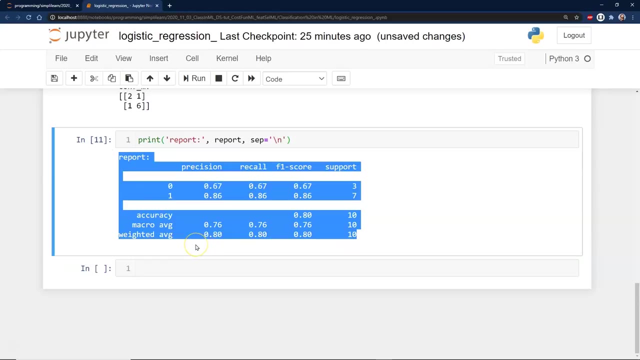 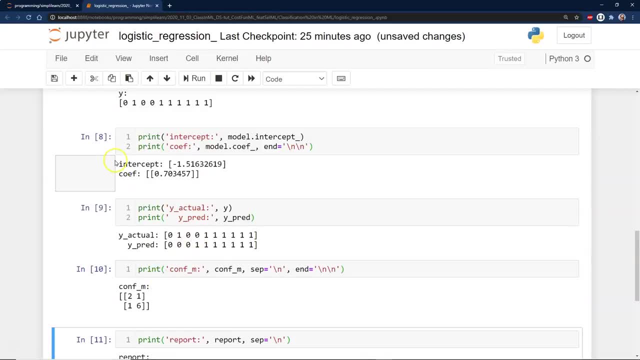 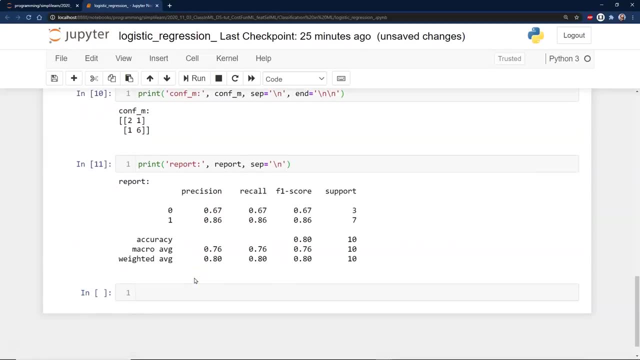 confusion matrix- I almost do this in reverse- as to what they show. I would never show your shareholders the intercept of the coefficient. That's for your internal team only working on machine language. But the confusion matrix and the report are very important. Those are the two. 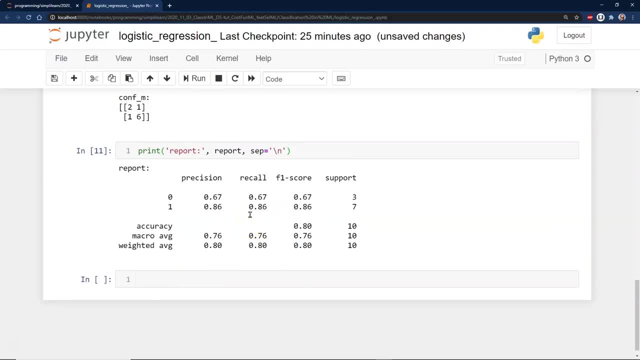 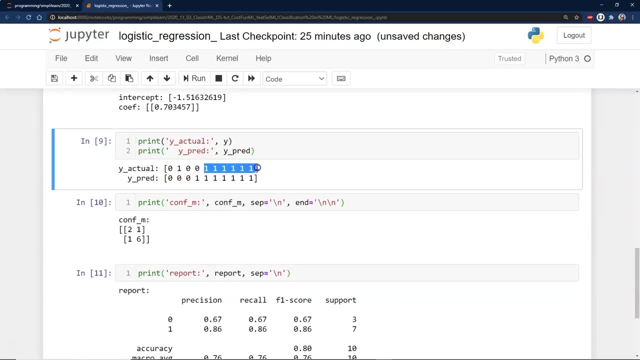 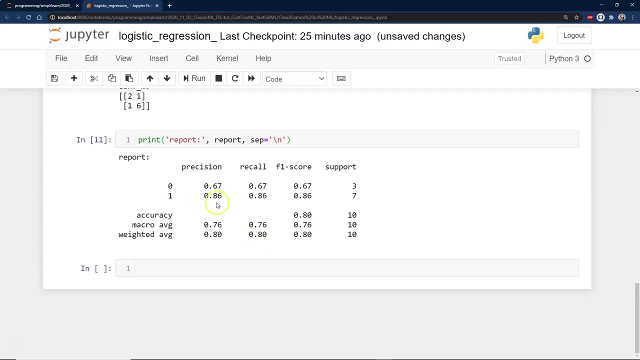 things you really want to be able to show. on these, And you can see here, we did a decent job of classifying the data, managed to get a significant portion of it correct. We had our accuracy here as a 0.80 F1 score, that kind of thing. So you know it's a pretty accurate model, Of course. 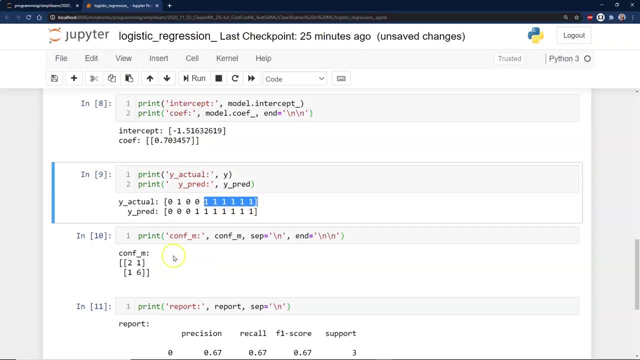 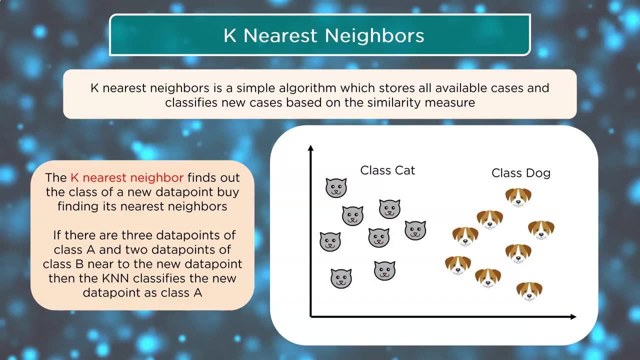 this is pretty goofy because it's a very simple model and it's just splitting the model between ones and zeros. So that was our demo of the logistic regression on there. Let's go and take a look at k-nearest neighbors. This one is another very highly used and important algorithm to 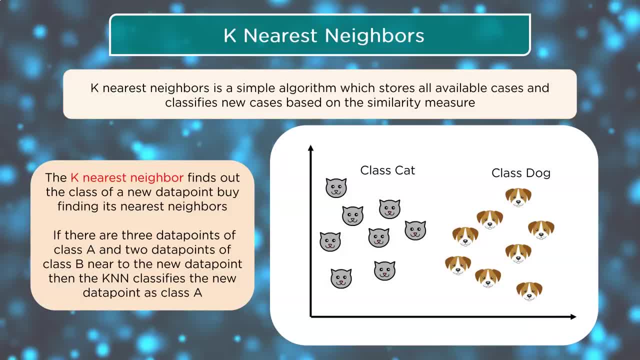 understand k-nearest neighbors is a simple algorithm which stores all of the data that we have, And it's a simple algorithm that stores all of the data that we have. And it's a simple algorithm that stores all of the data that we have, And it's a simple. 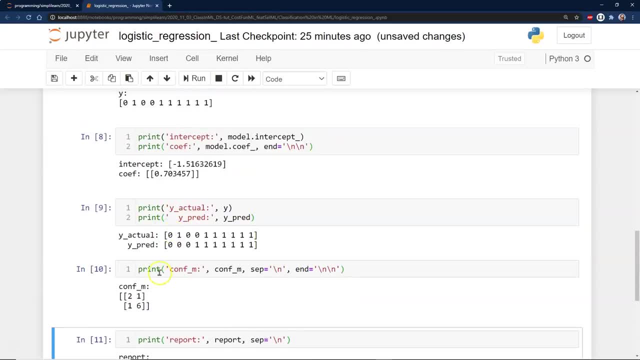 And then you start bringing in like the confusion matrix- I almost do this in reverse- as to what they show. I would never show your shareholders the intercept of the coefficient, That's for your internal team only working on machine language. But the confusion matrix and the report are very important. 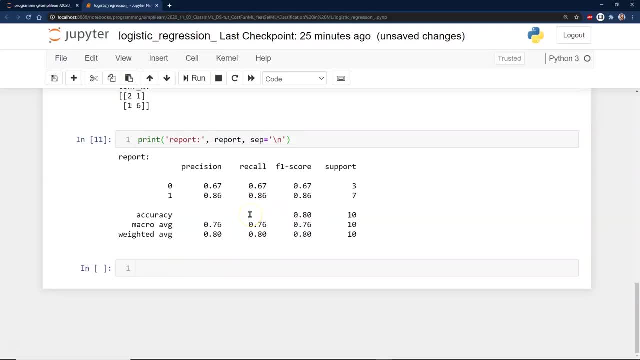 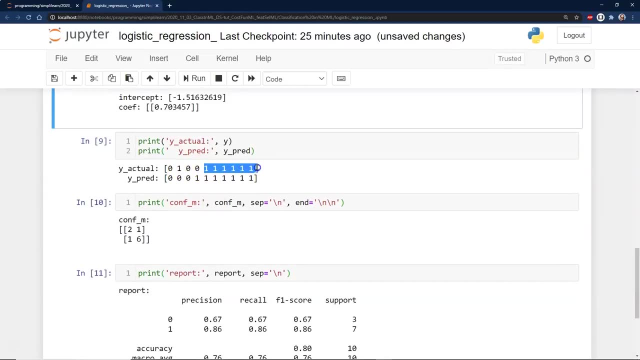 Those are the two things you really want to be able to show on these, And you can see here we did a decent job of classifying the data, Managed to get a significant portion of it correct. We had our accuracy here as a .80 F1 score. 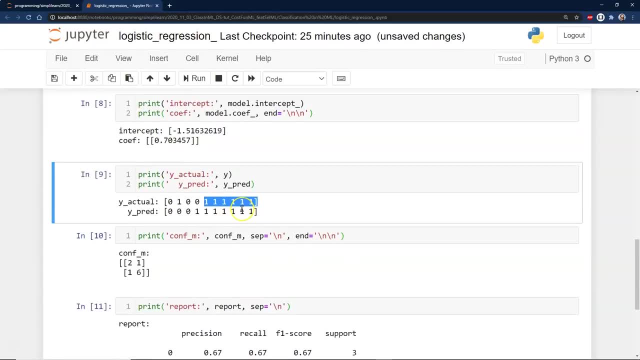 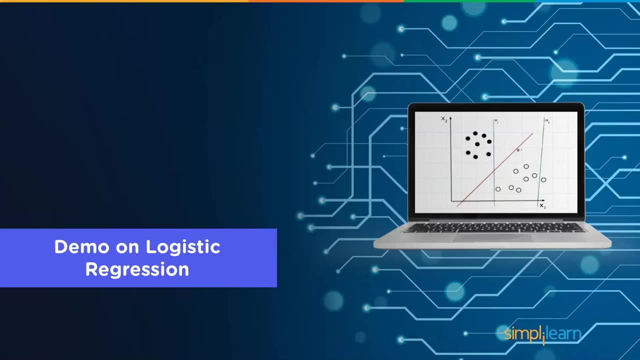 That kind of thing. So it's a pretty accurate model. Of course, this is pretty goofy because it's a very simple model And it's just splitting the model between 1s and 0s. So that was our demo of the logistic regression on there. 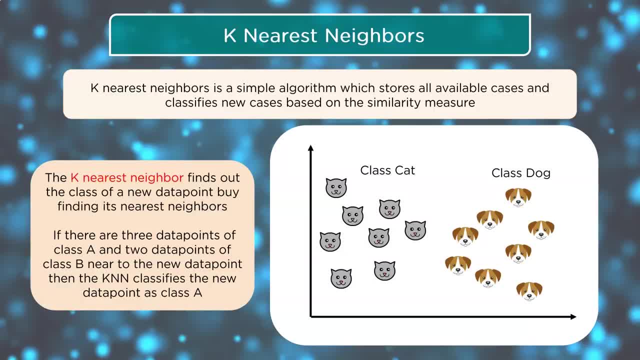 Let's go ahead and take a look at k nearest neighbors. This one is another very highly used And important algorithm. to understand K nearest neighbors is a simple algorithm which stores all available cases And classifies new cases based on the similarity measure. 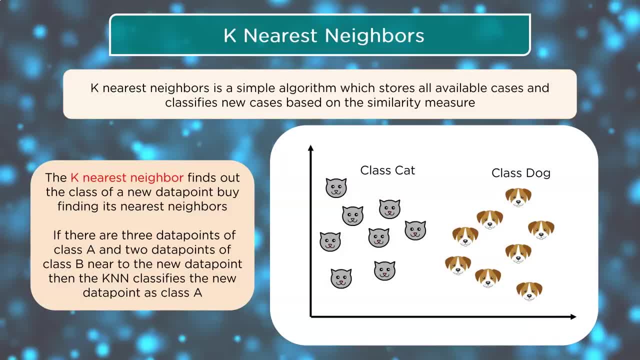 The k nearest neighbor finds out the class of the new data point By finding its nearest neighbors. If there are three data points of class A and two data points of class B Near to the new data point, Then the KNN classifies the new data point as class A. 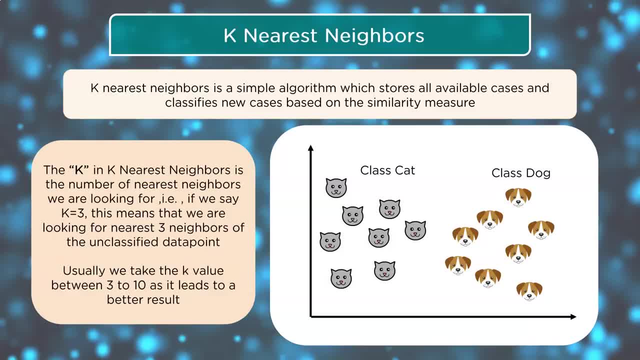 The k in k nearest neighbors is the number of nearest neighbors We are looking for. Ie if we say k equals 3. This means that we are looking for nearest three neighbors of unclassified data point. Usually we take the k value between 3 to 10.. 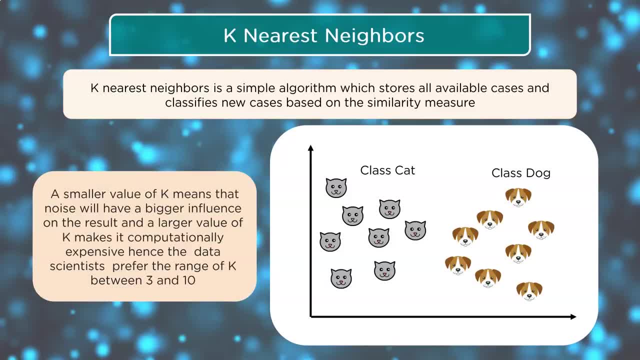 As it leads to a better result. A smaller value of k means that noise will have a bigger influence on the result, And a larger value of k makes it computationally expensive. Hence the data scientists prefer the range of k between 3 and 10.. 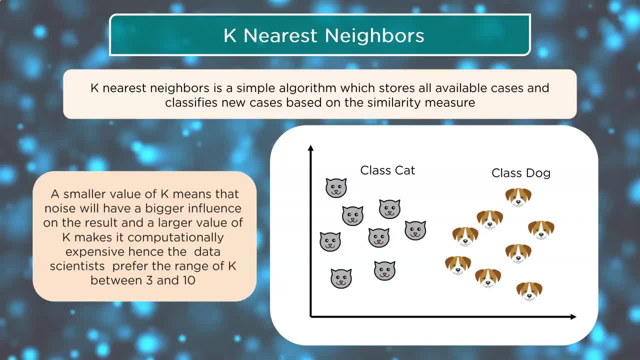 When we talk about noise. Remember, the data we just looked at was 0, 1, 1, 0, 0. It had some values where it cut it and said: everything to the right is a 1.. Everything to the left is a 0. 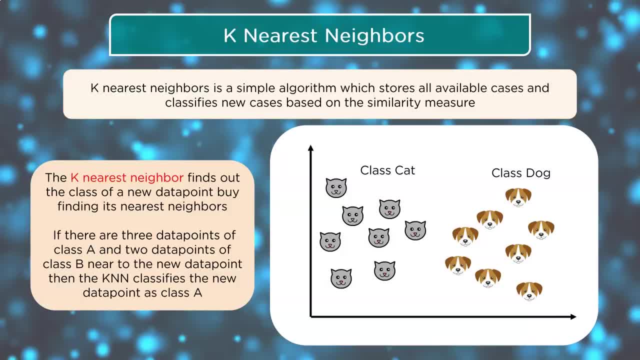 algorithm that stores all of the data that we have And it's a simple algorithm that stores all available cases and classifies new cases based on the similarity measure. The k-nearest neighbor finds out the class of the new data point by finding its nearest neighbors If there are three. 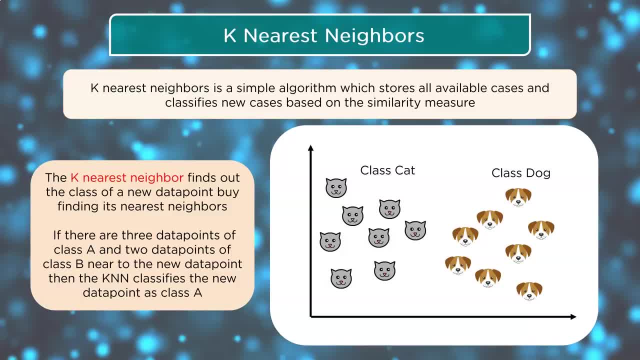 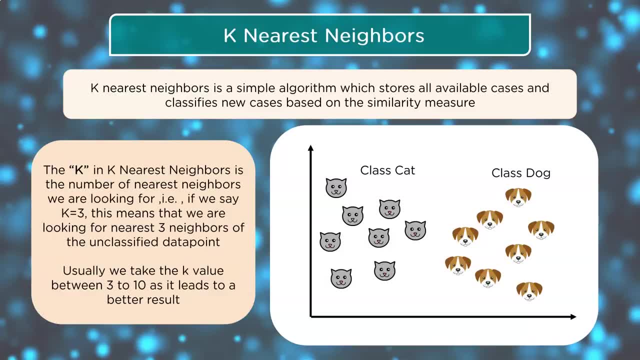 data points of class A and two data points of class B near to the new data point. then the K and N classifies the new data point as class A. The K and k-nearest neighbors is the number of nearest neighbors we are looking for. ie, if we say K equals 3, this means that we are looking for. 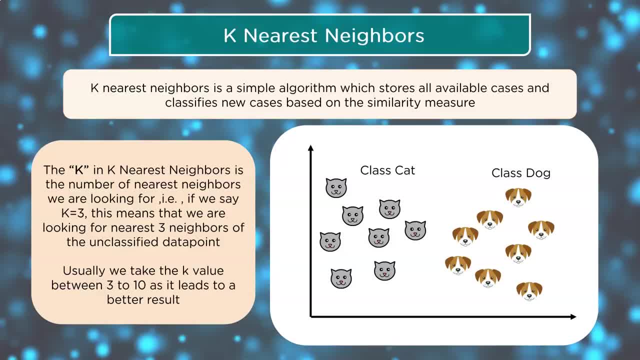 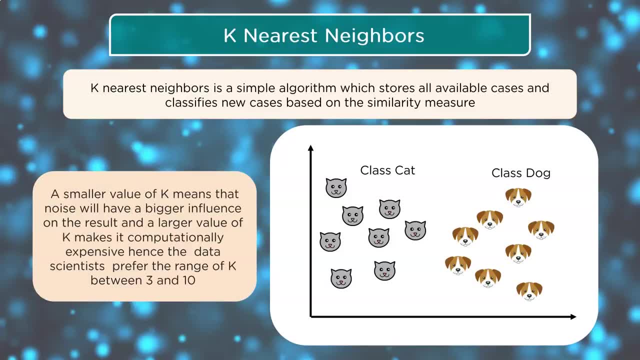 nearest neighbors And we're looking for the number of nearest neighbors And we're looking neighbors of unclassified data point. Usually we take the k value between 3 to 10, as it leads to a better result. A smaller value of k means that noise will have a bigger influence on the result. 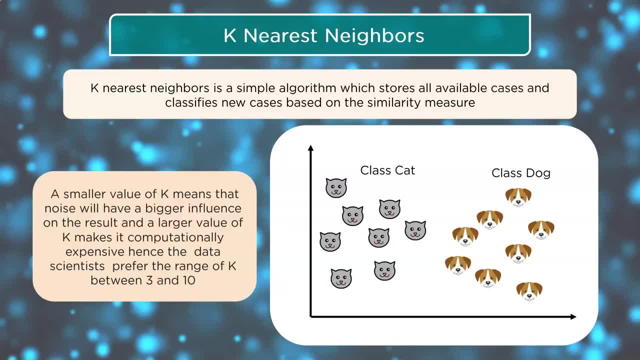 and a larger value of k makes it computationally expensive. Hence the data scientists prefer the range of k between 3 and 10.. When we talk about noise, you remember the data we just looked at was 0,, 1,, 1,, 0, 0. It had some values where it cut it and said: everything to the right is a 1,. 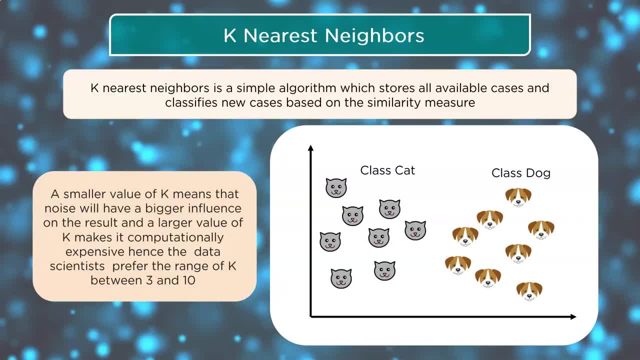 everything to the left is a 0,, but it had some 1s and 0s mixed in there. That's called noise. That's what they're talking about, is? there's some things that are right in the middle in the classification, which makes it very hard to classify, So suppose we were trying to find the class for a new point. 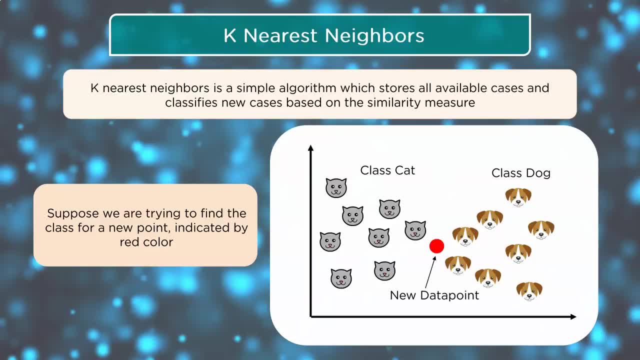 indicated by the red color and you can see it's kind of right between the cat, right between the dogs. Let k equal 3, so we are finding the red color. Let k equal 3, so we are finding the red color. Let k equal 3, so we are finding. 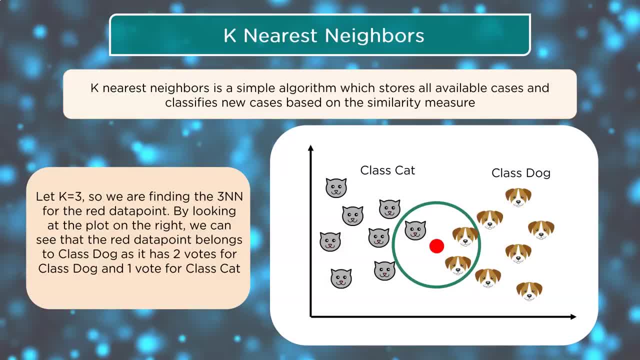 the 3nn for the red data point. By looking at the plot on the right, we can see that the red data point belongs to the class dogs, as it has two votes for class dog and one vote for class cat. And if you ask the question, well, what are you measuring the distance? What is that distance? 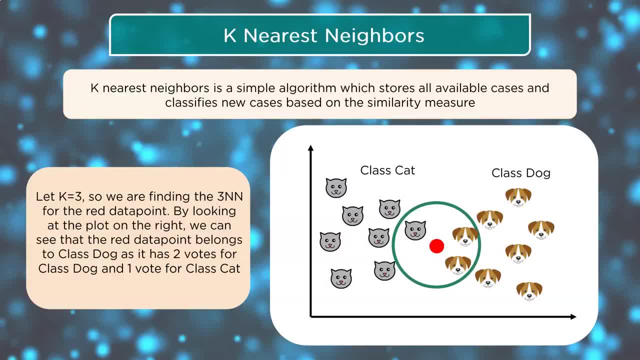 It could be the measurements of the ears, whether they're pointed or floppy. That might be. one of the features you're looking at is how floppy the ears are. Another one might be the whiskers versus the nose, And then you take those measurements and, using one of the most common things in k-means, measurement is 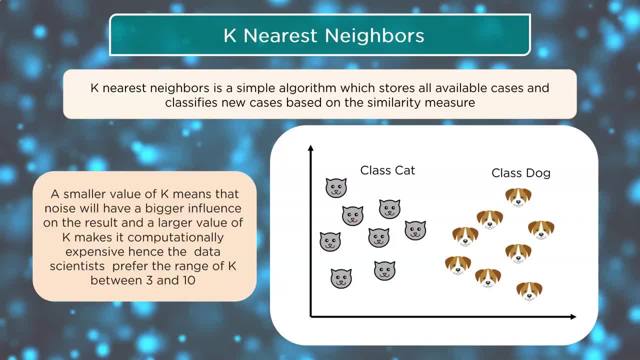 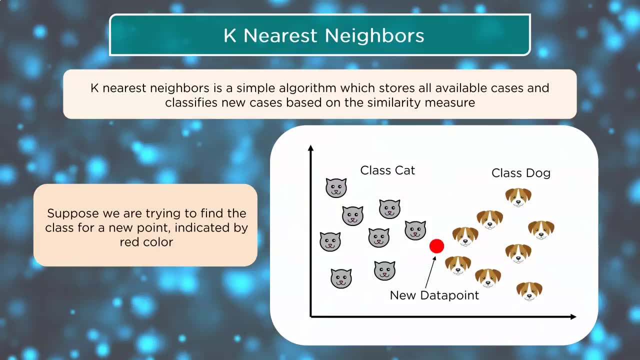 But it had some 1's and 0's mixed in there. That's called noise. That's what they are talking about. There are some things that are right in the middle in the classification Which makes it very hard to classify, So suppose we are trying to find the class for a new point. 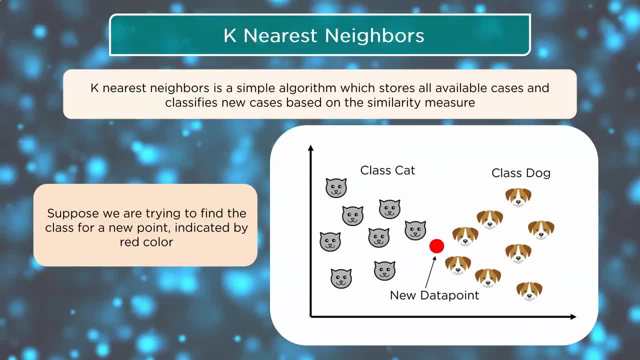 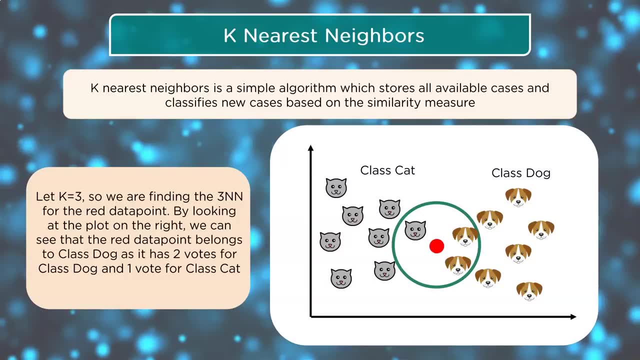 Indicated by the red color And you can see it's kind of right between the cat and right between the dogs. Let k equal 3.. So we are finding the 3nn for the red data point By looking at the plot on the right. 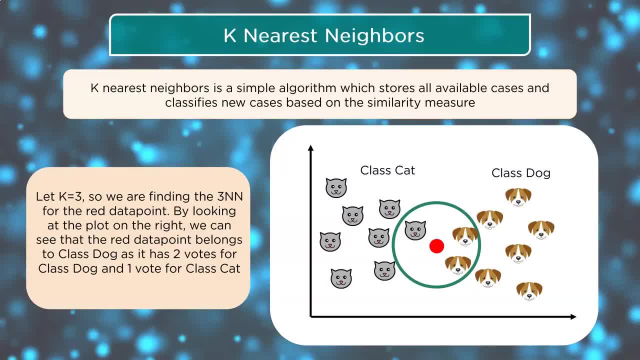 We can see that the red data point belongs to the class dogs, As it has 2 votes for class dog and 1 vote for class cat. And if you ask the question, Well, what are you measuring the distance? What is that distance? 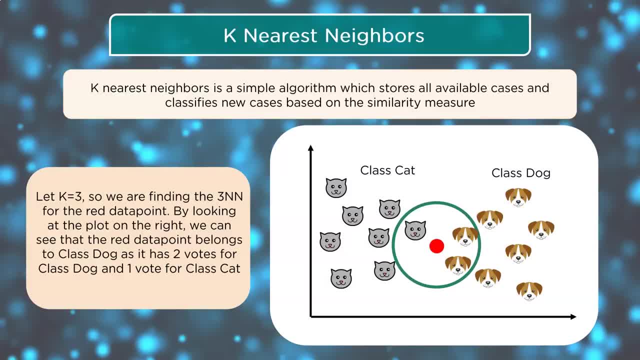 It could be the measurements of the ears, Whether they are pointed or floppy. That might be. one of the features you are looking at Is how floppy the ears are. Another one might be the whiskers versus the nose, And then you take those measurements. 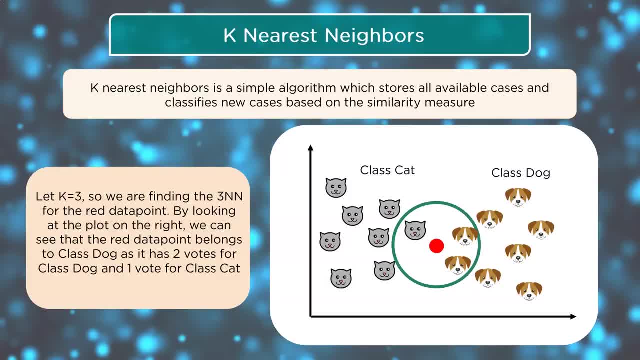 And using one of the most common things- And k means measurement- is the Euclidean geometry, You can figure out the distance between those points. There is a lot of different algorithms for that, But you can think about it that you do have to have some kind of solid data to measure. 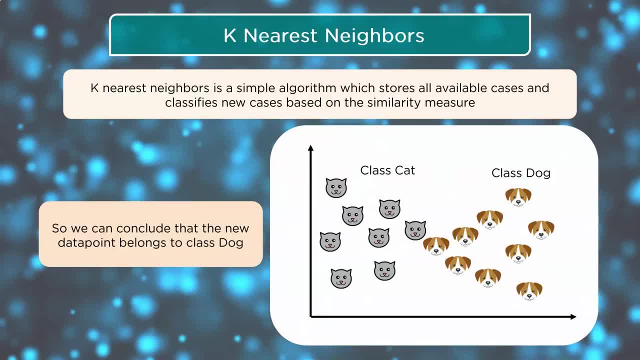 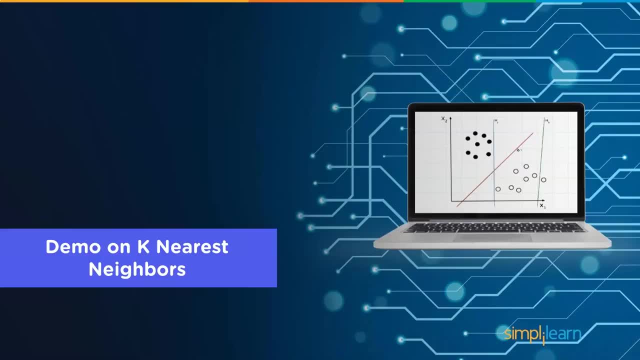 And so we can conclude that the new data point belongs to the class dog. So let's go ahead and see what this looks like in code And do a demo on the k nearest neighbor, And we will go right back into our Jupyter notebook. 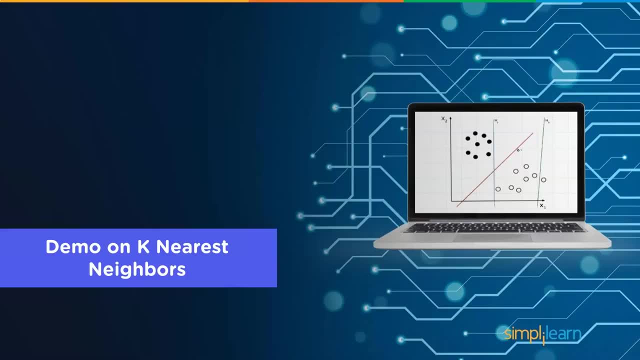 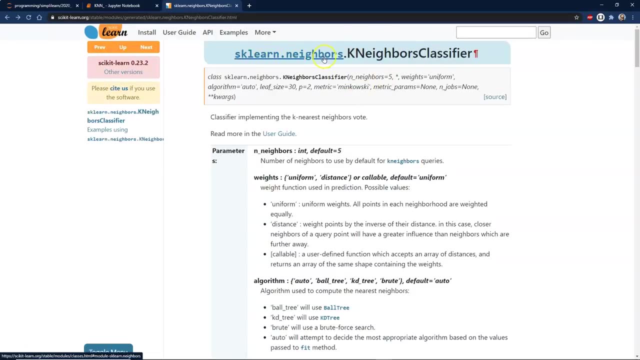 And open up a new Python programming script page. Of course, once we are in here, We will want to look at the scikit-learn. I did just a quick search for skneighborsknneighborsclassifier. This actually is the older version. 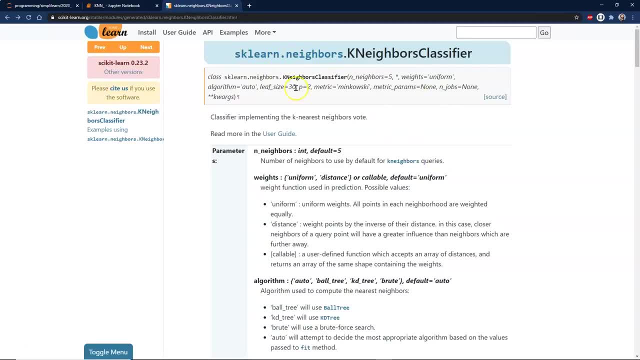 0.023 is the one we want And you will see here that we have all their defaults In neighbors equals 5.. At defaults, we were talking about that between 3 and 10. There is different ways to work with that. 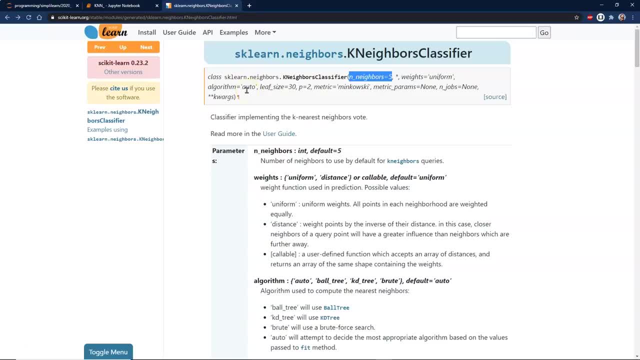 You can weigh it. There is an algorithm based on it. I mentioned Euclidean geometry, Finding the distance. There is other algorithms for figuring out what that distance is And how to weight those, And there is a lot of other parameters you can adjust. 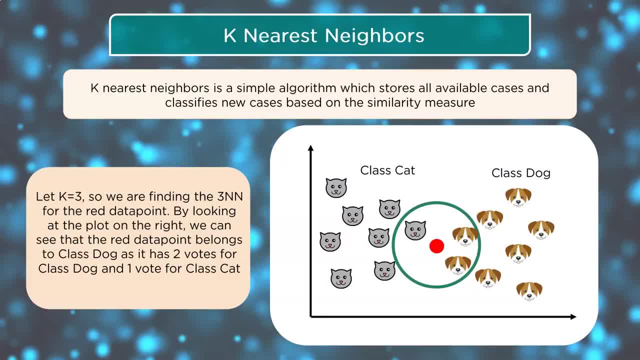 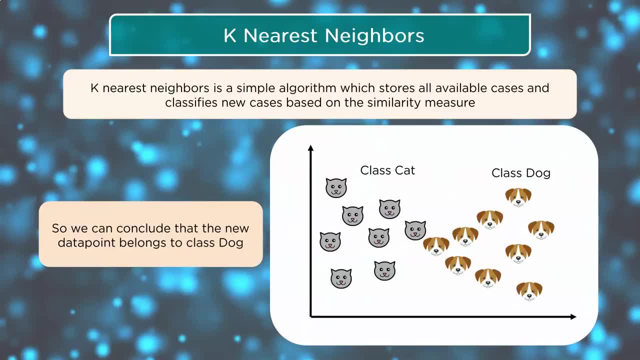 the Euclidean geometry, you can figure out the distance between those points. There's a lot of different algorithms for that, But you can think about it that you do have to have some kind of solid data to measure, And so we can conclude that the new data point belongs to the class dog. So 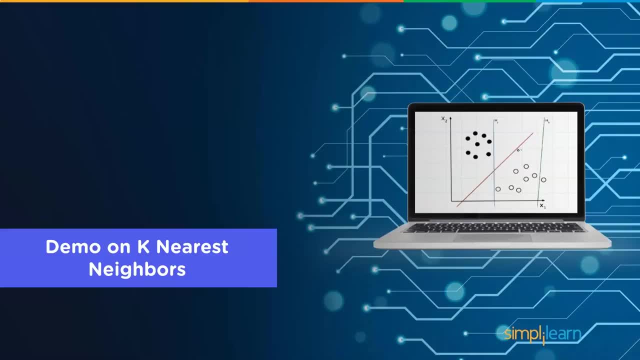 let's go ahead and see what this looks like in code and do a demo on the k nearest neighbors in here, And we'll go right back into our Jupyter notebook and open up a new Python programming script page, Of course, once we're in. 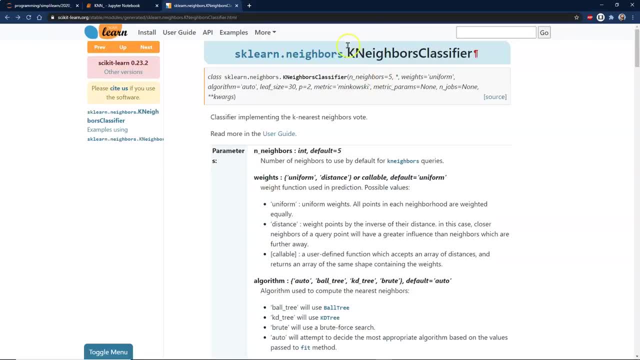 here. we'll want to look at the scikit-learn. I did just a quick search for SK neighbors, KN neighbors classifier. This actually is the older version. 0.023 is the one we want And you'll see here that we have all their defaults in neighbors equals five At defaults we were talking about. 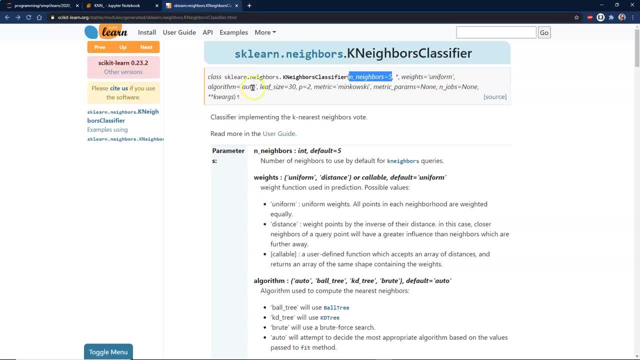 that between three and 10.. There's different ways to weigh it. There's an algorithm based on it. I mentioned Euclidean geometry, finding the distance. There's other algorithms for figuring out what that distance is and how to weight those, And there's a lot of other parameters you can. 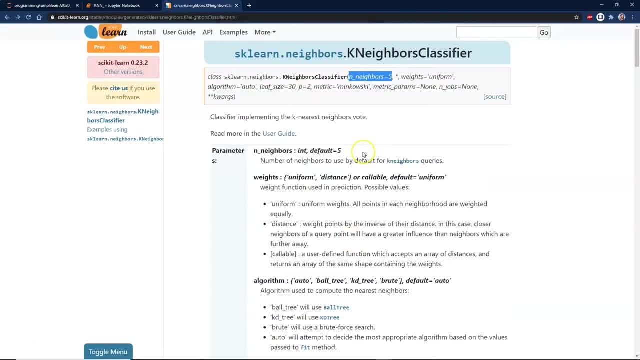 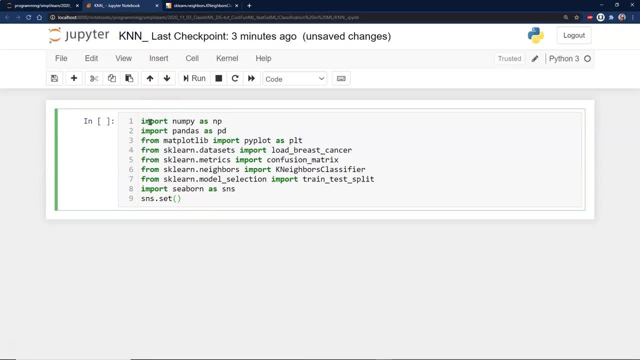 adjust. For the most part, the K means basic setup is a good place to start and just let the defaults go. We might play with some of those. We'll see what the guys in the back did And from here we're going to import numpy. We're going to use pandas If you haven't been running pandas. 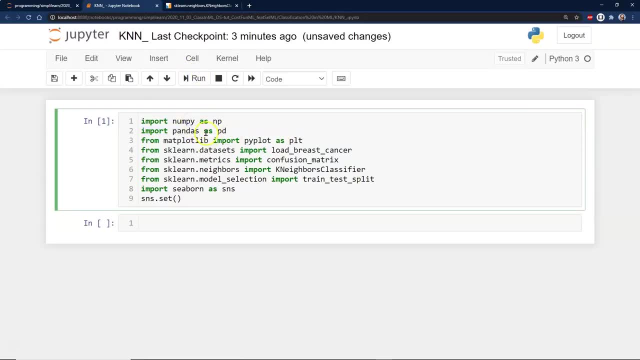 pandas is our data frame which sits on top of numpies. Numpies is our number array. Pandas is our data frame. Matplot library, because we're going to plot some graphs. Everybody likes some pretty pictures. It makes it a lot easier to see what's. 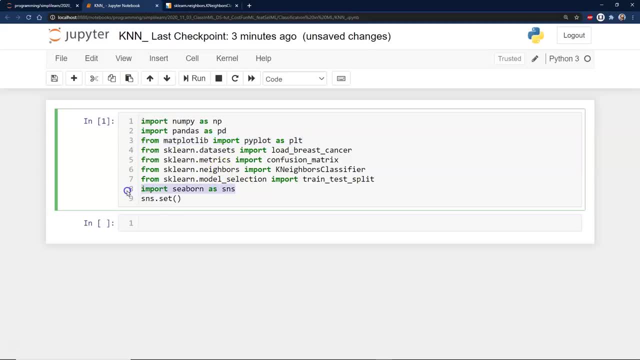 going on when you have a nice display- And that's also what the seaborn is in here in the setup that sits on top of the matplot library. The ones we really want to look at right here are what we're bringing in from sklearn, These ones right here. So from sklearn we're going to load. I mentioned 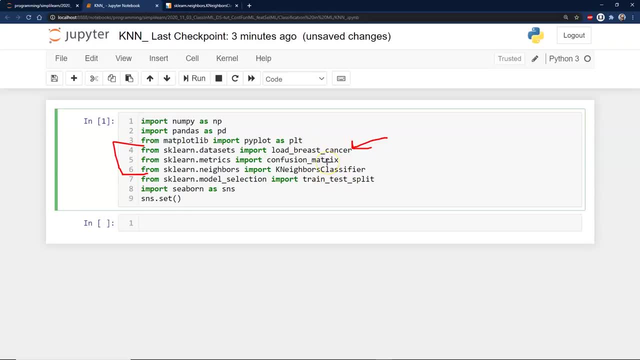 the breast cancer. That's going to be the breast cancer And then we're going to load the breast cancer. It's a very popular one because it has, I believe it's- 36 measurements. So there's 36 features, And unless you're a expert, you're not going to know what any of those features really. 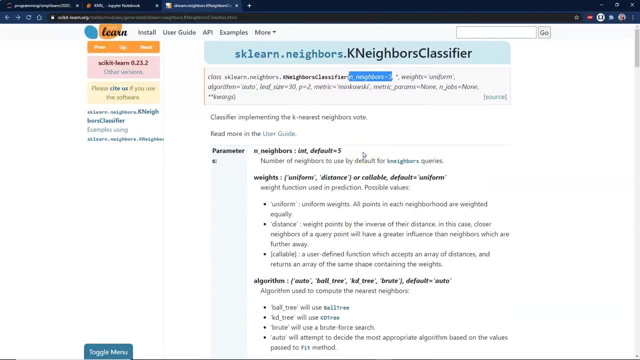 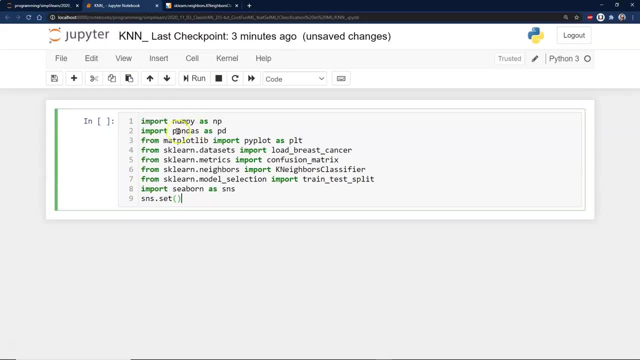 For the most part, the kmeans basic setup is a good place to start. Just let the defaults go. We might play with some of those. We will see what the guys in the back did, And from here we are going to import numpy. 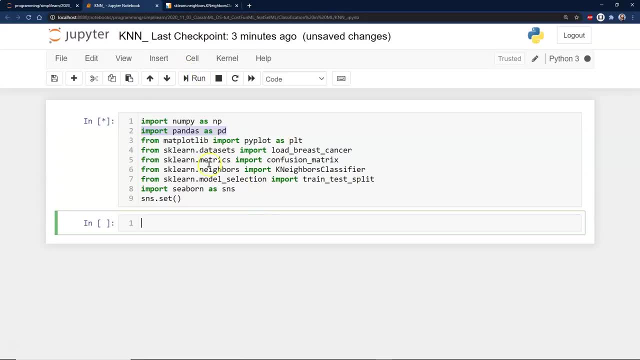 We are going to use pandas, If you haven't been running pandas. Pandas is our data frame which sits on top of numpy. Numpy is our number array. Pandas is our data frame Matplot library, because we are going to plot some graphs. 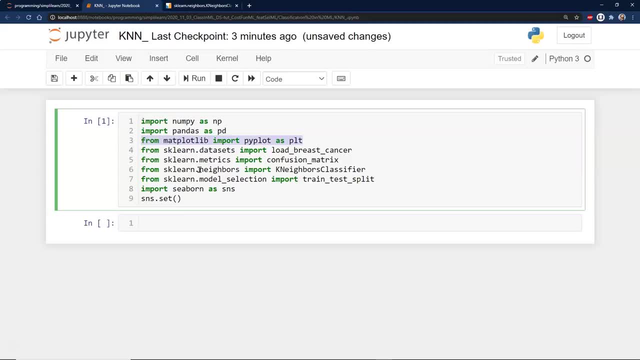 Everybody likes some pretty pictures. It makes it a lot easier to see what is going on when you have a nice display, And that is also what the seaborn is in here in the setup that sits on top of the matplot library. The ones we really want to look at right here are what we are bringing in from sklearn. 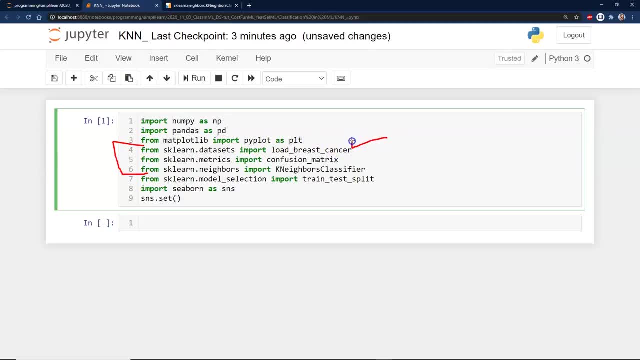 These ones right here. So from sklearn we are going to load. I mentioned the breast cancer. That is a very popular one because it has, I believe it is 36 measurements. So there is 36 features and unless you are an expert you are not going to know what any of those features really mean. 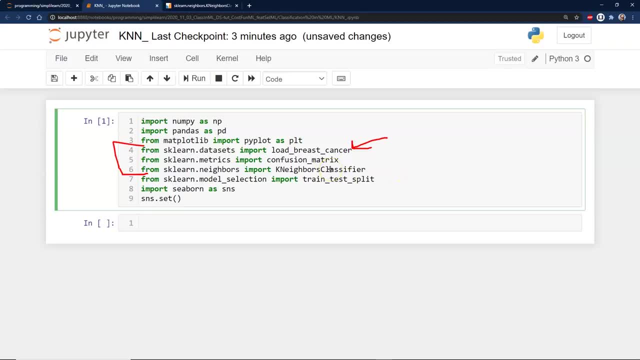 You can sort of guess. But there are special measurements they take up when they take an image And of course our confusion matrix so that we can take a look and see what the data looks like And how good we did. And then we have our kn at neighbors class. 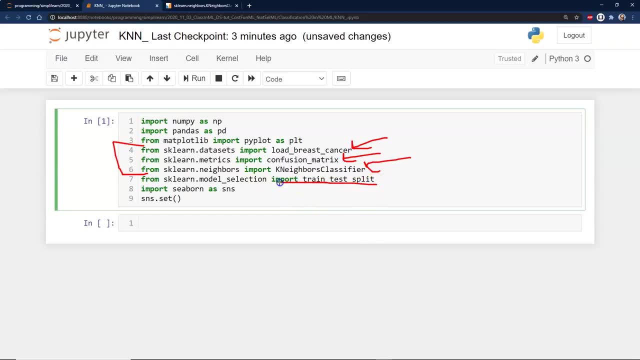 And then I mentioned that whenever you do training and testing, you want to split the data up. You don't want to train the data and then test it on the same data. That just tells you how good your training model is. It doesn't tell you whether it actually works on unknown data. 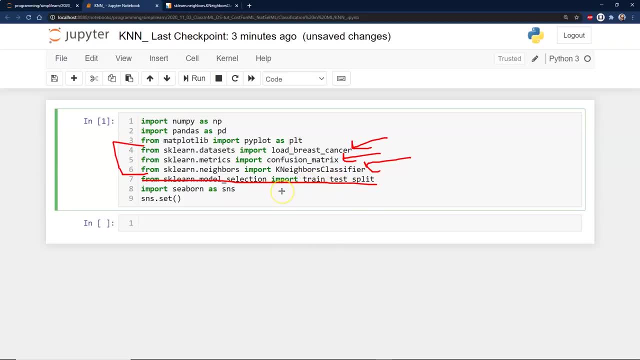 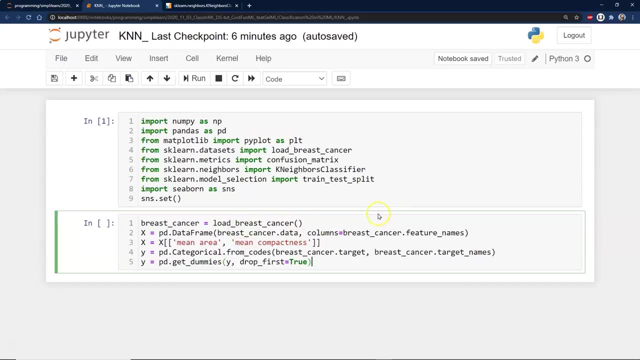 And so this just splits it off so that we can train it, And then we can take a look at data we don't have in there and see how good it did, And we will go ahead and load our data up. So here is our setup on that. 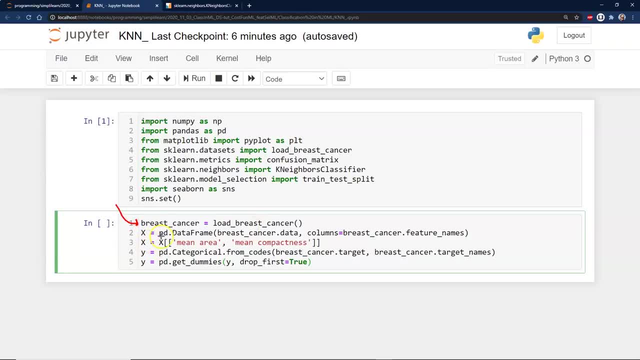 There we go. So we are going to go ahead and load the data up. We have our x value And that is going to come from our breast cancer dot data And column breast cancer feature names. So there is our actual, all our different features. 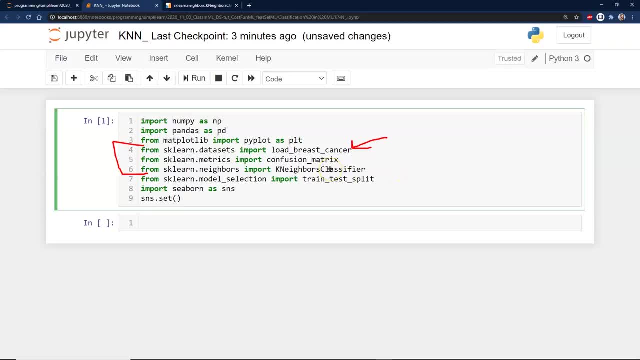 mean You can sort of guess. but there are special measurements they take up when they take an image And of course our confusion matrix so that we can take a look and see what the data looks like and how good we did. And then we have our KN at neighbor's classifier on here. And then I mentioned 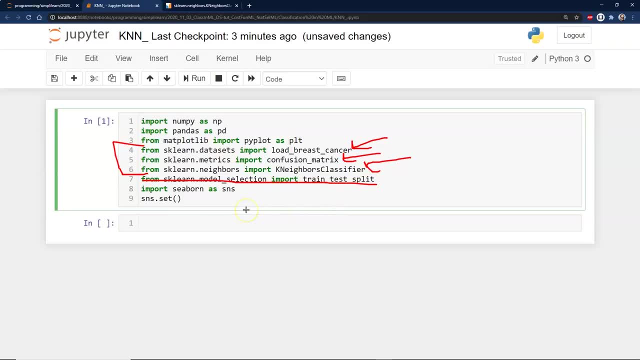 that we're going to do training and testing. You want to split the data up. You don't want to train the data and then test it on the same data. That just tells you how good your training model is. It doesn't tell you whether it actually works on unknown data, And so this just splits it off. so 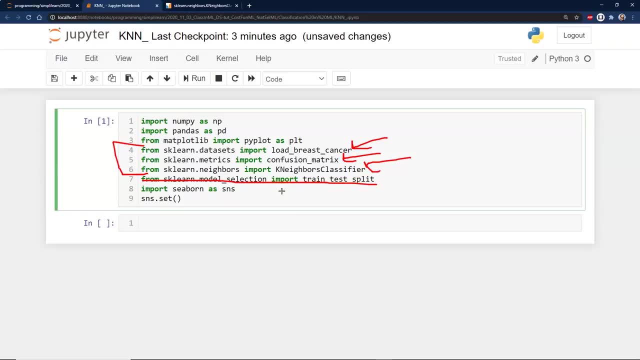 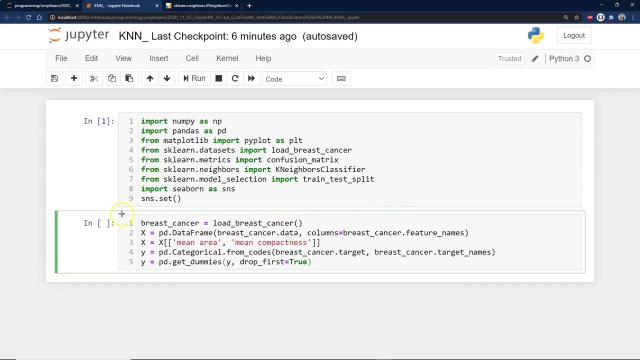 that we can train it, And then we can take a look at data we don't have in there and see how good it did, And we'll go ahead and load our data up. So here's our setup on that. Oops, there we go, So. 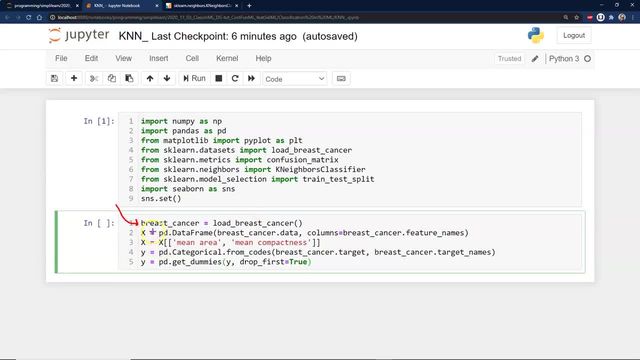 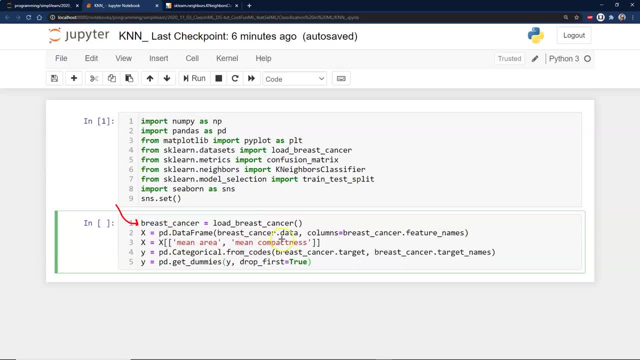 X value And that's going to come from our breast cancer dot data and column breast cancer feature names. So there's our actual, all our different features. We'll print that out here in a second And then we have our mean area, mean compactness. So I guess we're going to take the data and we're 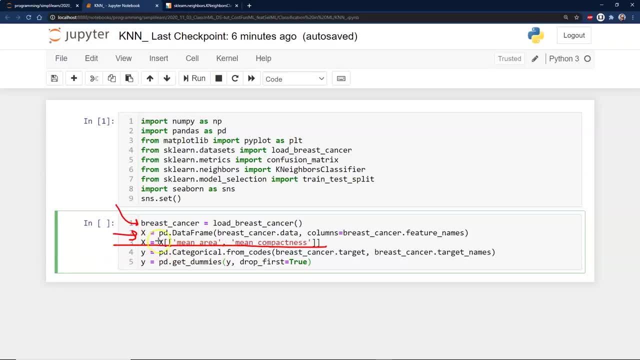 only going to use a couple of the columns. This just makes it easier to read. Of course, when you actually were going to do this, you'd want to use all your columns. And then we have our Y, and this is simply whether it's either malignant or benign. And then we want to go ahead and drop. 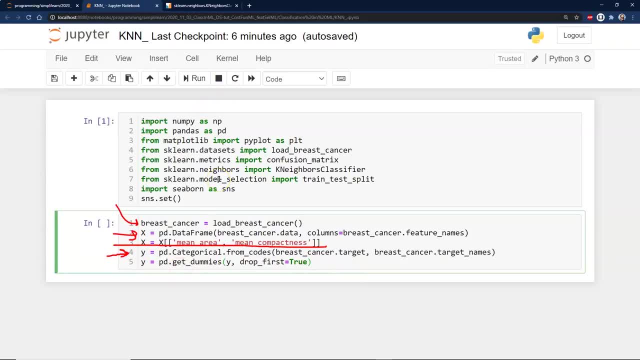 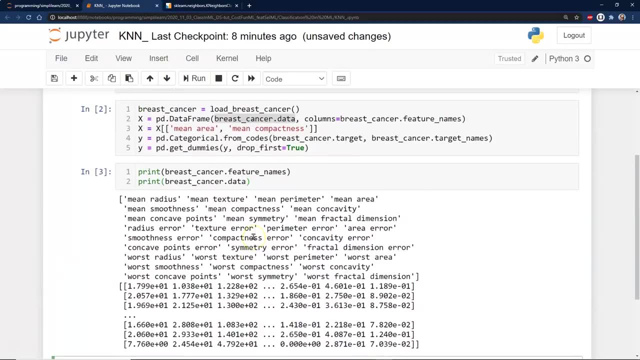 the first line because that's how it came in on there And we'll go ahead. let's just take a look at this a little closer here. Let's go and run this real quick And just because I like to see my data before I run it, we can look at this and we can look at the original features, Remember. 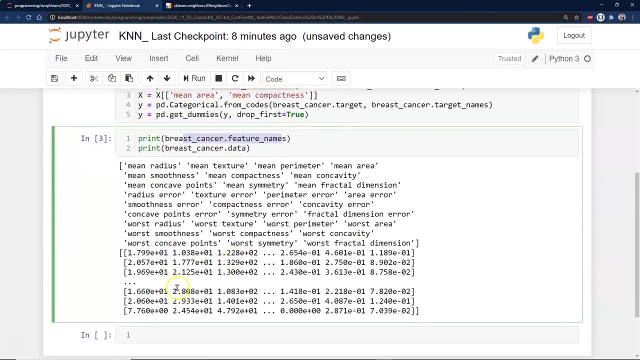 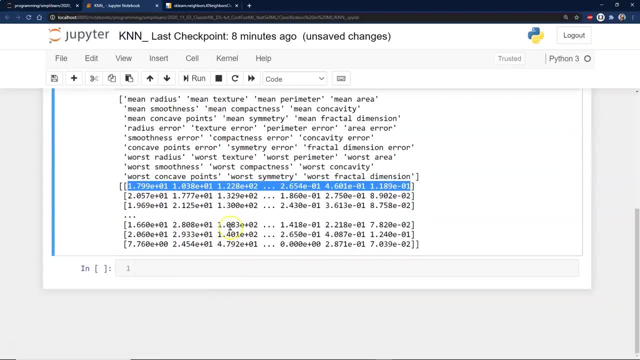 we're only going to use two features off of here just to make it a little easier to follow. And here's the actual data And you can see that this is just this massive stream of data coming in here. It's going to just skip around because there's so much in there. 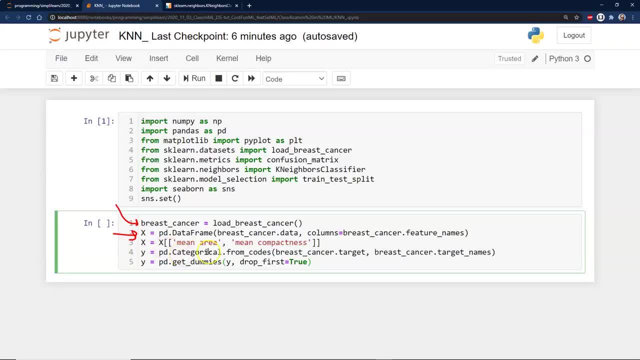 We will print that out here in a second And then we have our mean area, mean compactness. So I guess we are going to take the data and we are only going to use a couple of the columns. This just makes it easier to read. 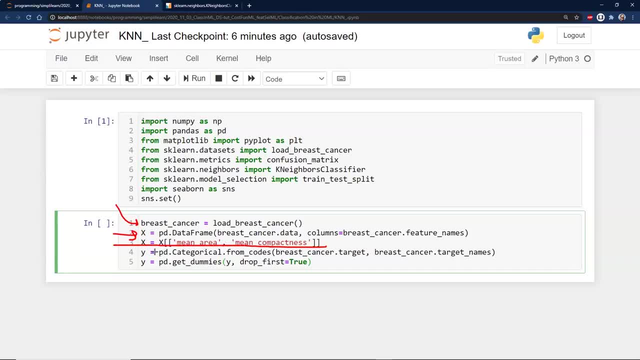 Of course, when you actually were going to do this, you would want to use all your columns. And then we have our y, And this is simply whether it is either malignant or benign. And then we want to go ahead and drop the first line, because that is how it came in on there. 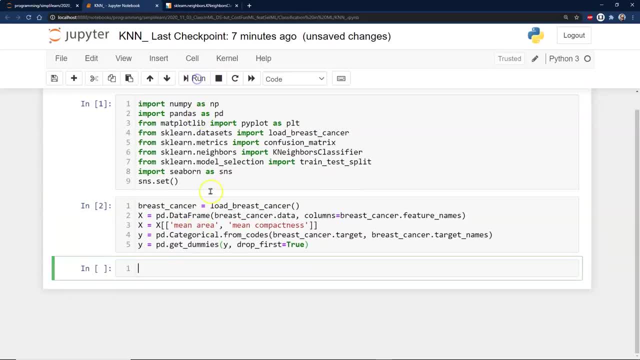 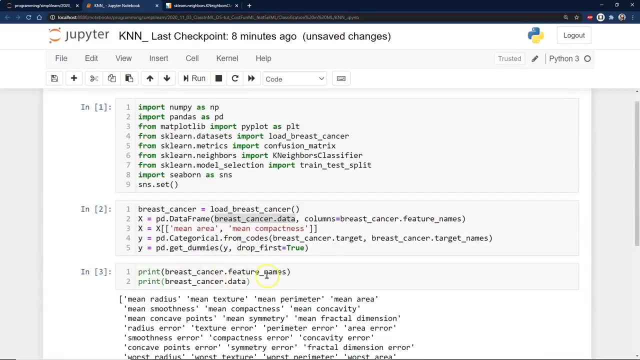 And we will go ahead. Let's just take a look at this a little closer here. Let's go ahead and run this real quick And just because I like to see my data before I run it, We can look at this and we can look at the original features. 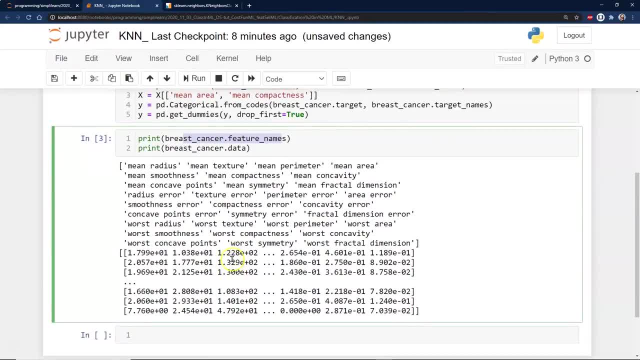 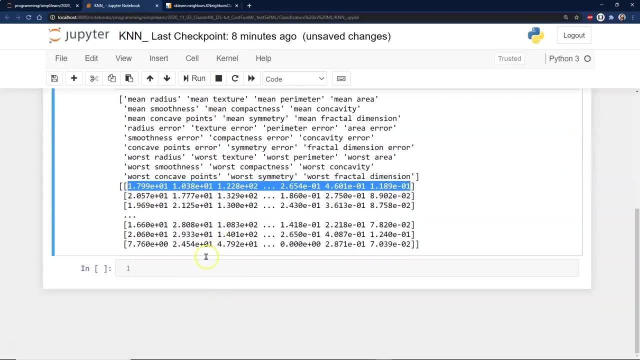 Remember, we are only going to use two features off of here Just to make it a little easier to follow. And here is the actual data And you can see that this is just this massive stream of data coming in here. It is going to just skip around because there is so much in there to set up. 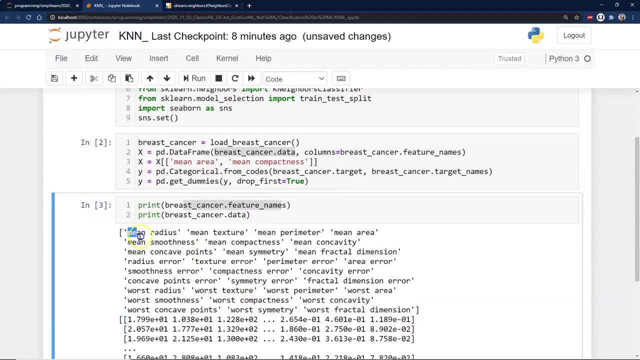 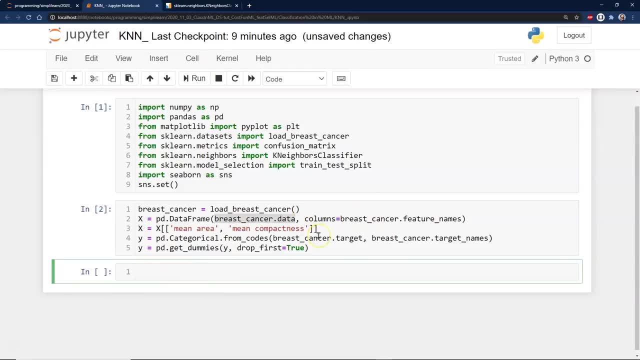 I think there is like 500, if I remember correctly, And you can see here is all the different measurements they take. But we don't really need to see that on here. We are just going to take a look at just the two columns. 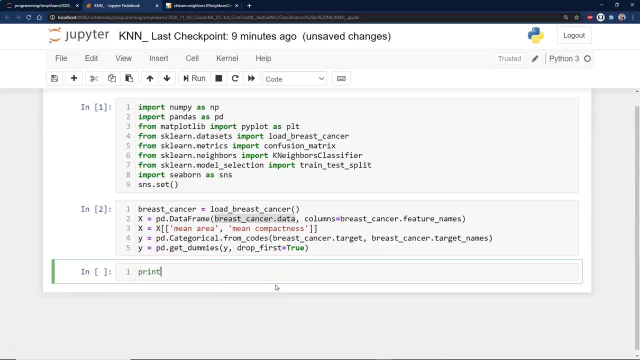 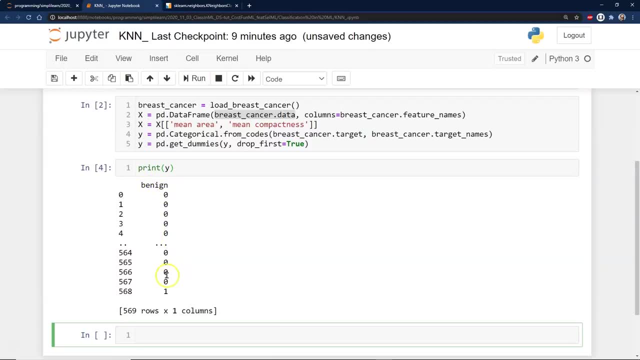 And then also our solution. We will go ahead and just do a quick print Y on here so you can see what the y looks like, And it is simply just 0, 0, 0, b9, 0, 0, 0, 1.. 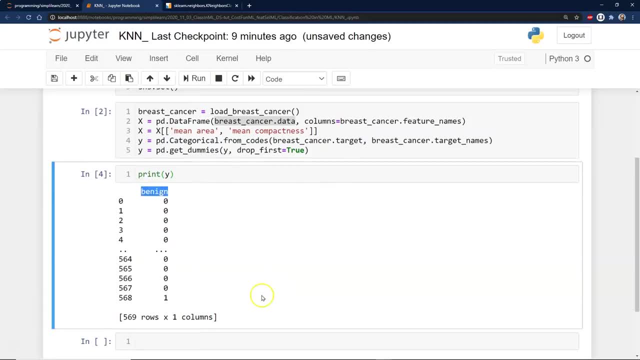 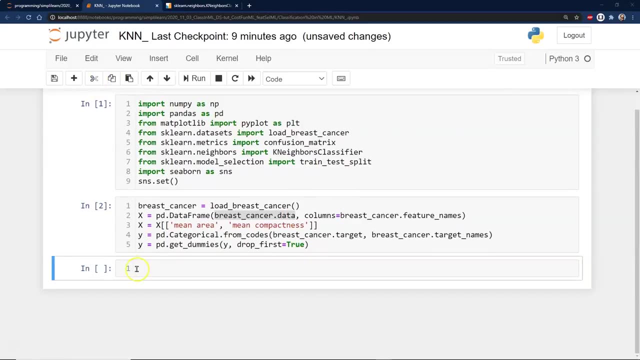 So a 1 means it is b9 and a 0 means it is malignant. That is what we are looking at on that. Go ahead and cut that out of there. The next stage is to go ahead and split our data. I mentioned that earlier. 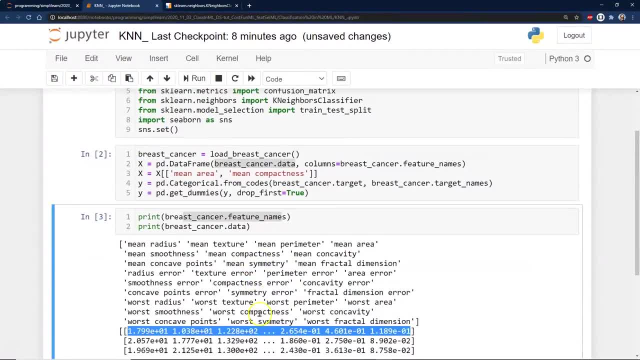 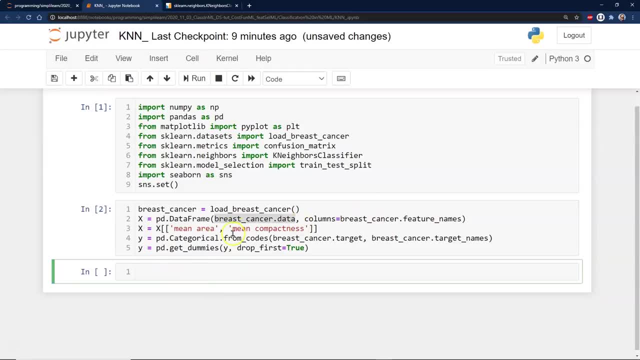 to set up. I think there's like 500, if I remember correctly, And you can see. here's all the different measurements they take. But we don't really need to see that on here. We're just going to take a look at just the two columns And then also our solution. We'll go ahead and just do a quick. 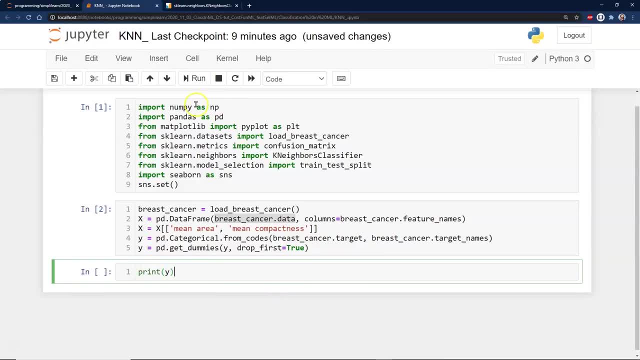 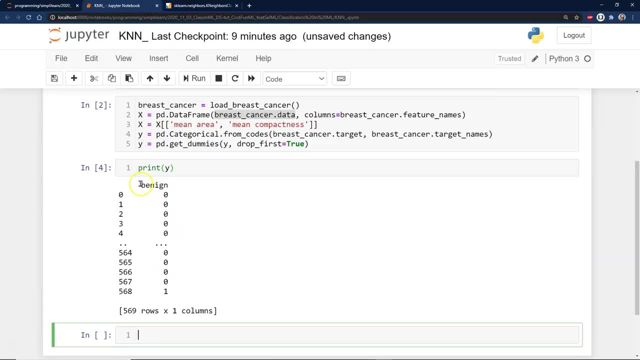 print Y on here so you can see what the Y looks like. And it is simply just 000,. you know B9, 0001.. So one means it's B9.. Zero means it's malignant. is what we're looking at on that. Cut that out of there. The next stage. 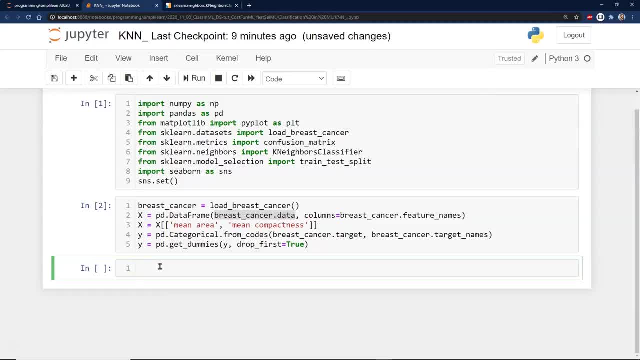 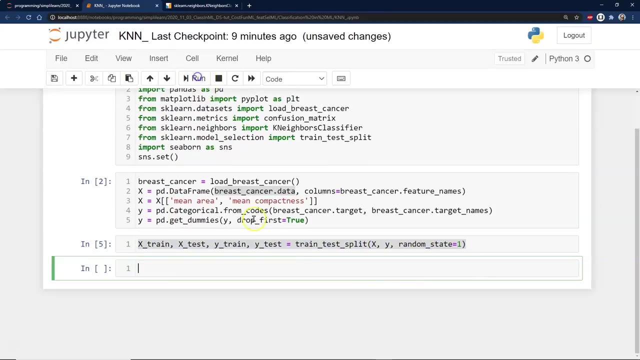 is to go ahead and split our data. I mentioned that earlier. We'll just go ahead and let them do the splitting forest for us. We have X train, X test, Y train, Y test, And so we go ahead and train test, split XY. random state equals one. It makes it nice and easy for us. We'll go and run. 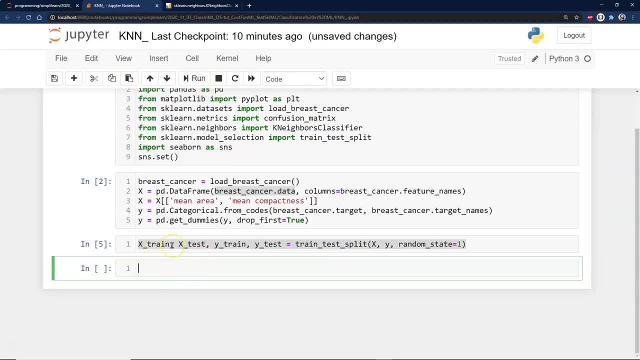 that, And so now we have our training and our testing. Train means we're going to use that to train the model, And then we're going to go ahead and split our data. And so we're going to go ahead and split our data And then we're going to use the test to test to see how good our model does. 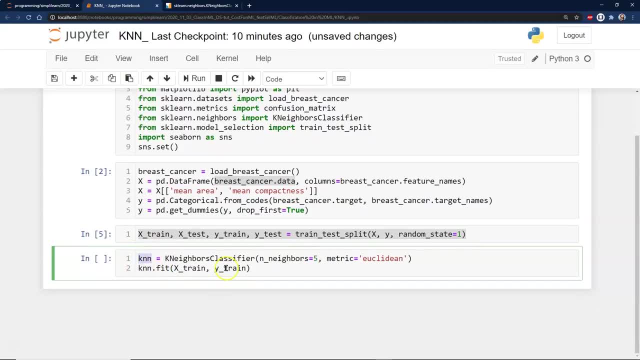 And then we'll go ahead and create our model. Here's our KNN model. the K neighbors classifier N neighbors equals five. The metrics is Euclidean. Remember I talked about Euclidean? This is simply your C squared equals A squared plus B squared plus A squared equals B squared plus C squared. 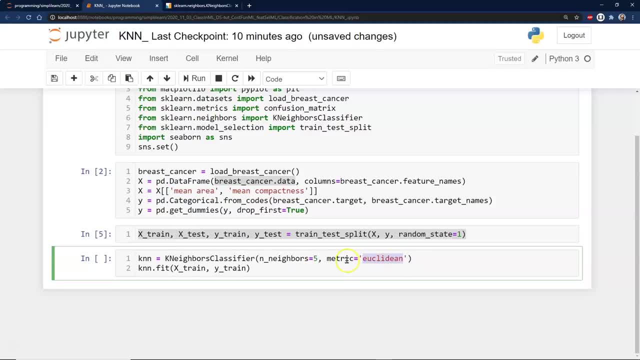 plus C squared, plus D squared, And then you take the square root of all that. That's what they're talking about here. It's just the length of the hypotenuse of a triangle, But you can actually do that in multiple dimensions, just like you do in two dimensions with a regular triangle, And 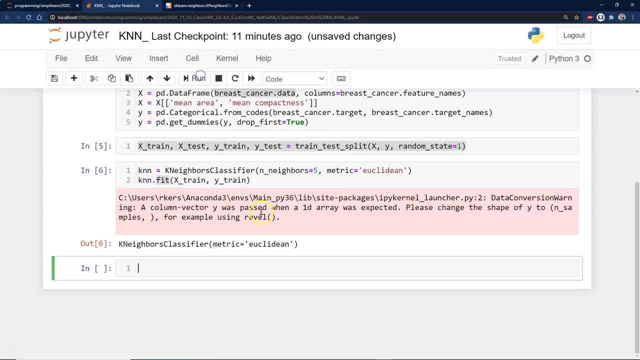 here we have our fit. This should start to look familiar, since we already did that in our last example. That's very standard for scikit and any other one, Although sometimes the fit algorithms look a little bit more complicated because they're doing more things on there, especially when you 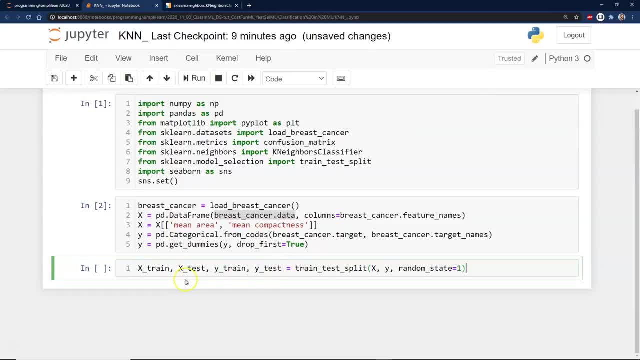 We will just go ahead and let them do the splitting for us. We have x train, x test, y train, y test, And so we go ahead and train test. split x, y, random state equals 1.. It makes it nice and easy for us. 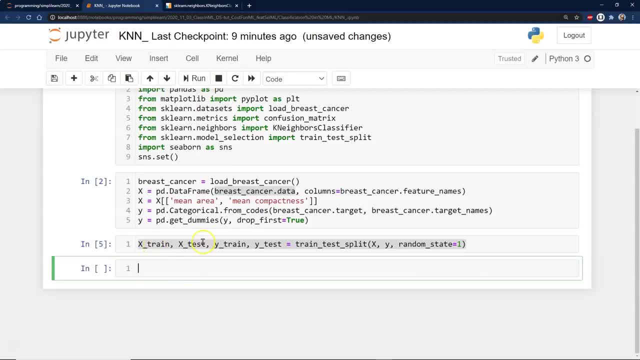 We will go ahead and run that, And so now we have our training and our testing. Train means we are going to use that to train the model, And then we are going to use the test to test to see how good our model does. 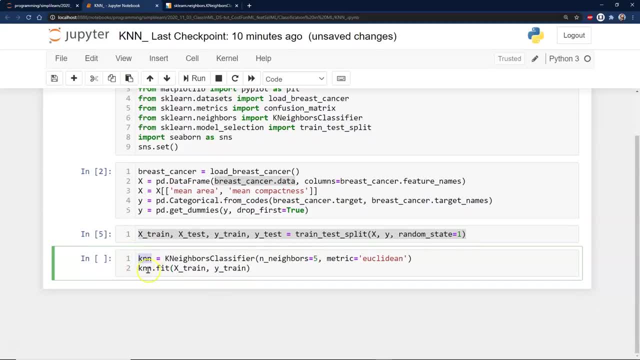 And then we will go ahead and create our model. Here is our KNN model. The K- neighbors classifier, N neighbors equals 5.. The metrics is Euclidean. Remember I talked about Euclidean? This is simply your c squared equals a squared plus b squared plus. 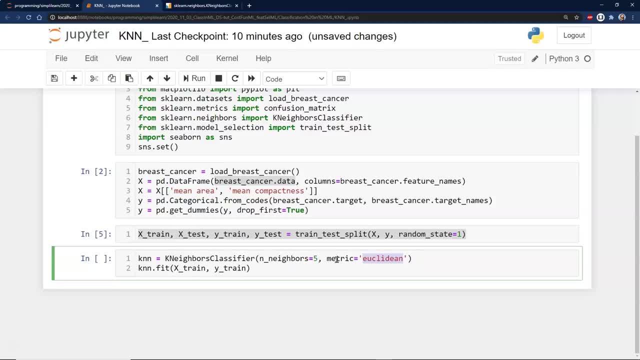 a squared equals b squared plus c squared, plus c squared plus d squared, And then you take the square root of all that. That is what they are talking about here. It is just the length of the hypotenuse of a triangle, But you can actually do that in multiple dimensions. 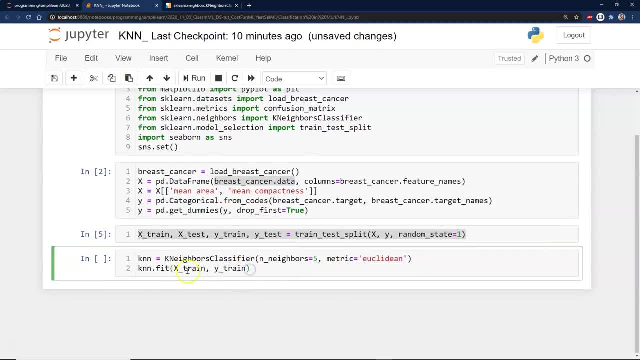 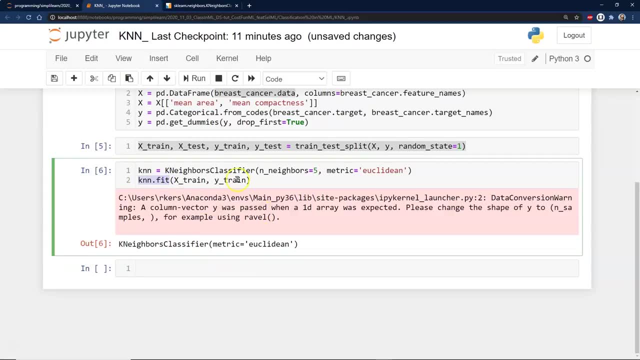 Just like you do in two dimensions with a regular triangle, And here we have our fit. This should start to look familiar, since we already did that in our last example. That is very standard for scikit And any other one, Although sometimes the fit algorithms look a little bit more complicated. 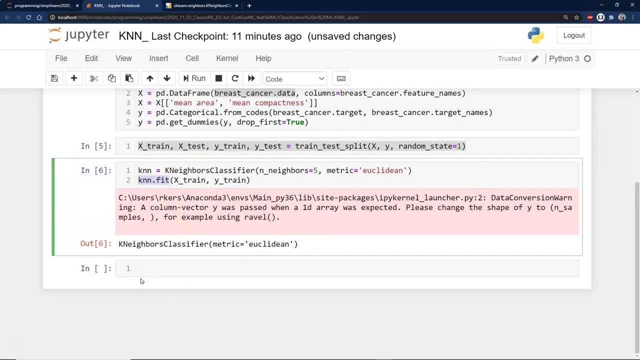 because they are doing more things on there, especially when you get into neural networks And then you have your k neighbors. We have created a k neighbors setup. They kind of wanted us to reformat the y, but it is not that big of a deal for this. 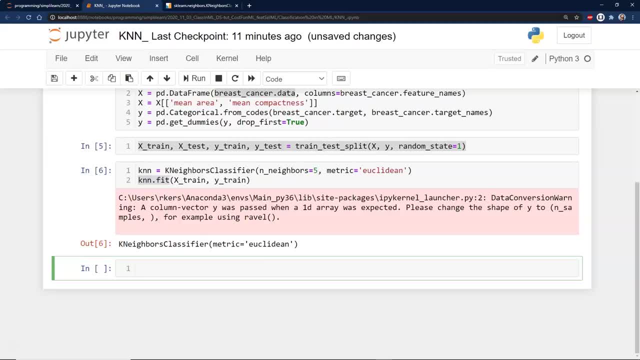 And it comes out and shows you that we are using the Euclidean metric for our measurement. So now we have created a model. Here is our live model. We have fitted the data to it. We say, hey, here is our training data. 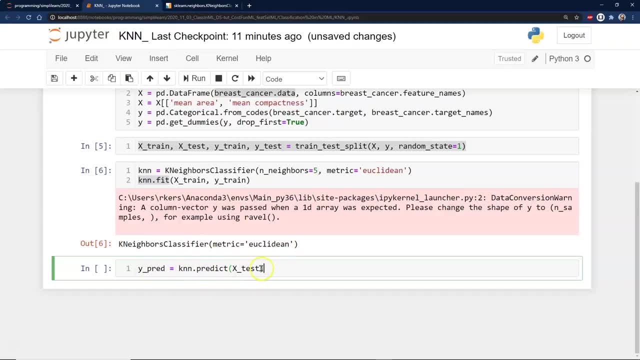 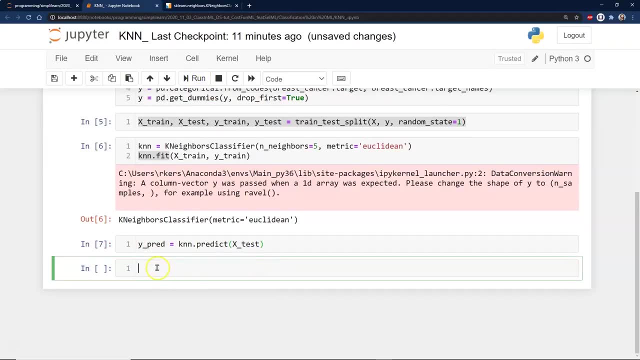 Let us go ahead and predict it. So we are going to take our y predict equals k and n predict y test. So this is data we have not, this model has not seen this data, And so we are going to create a whole new set of data options. 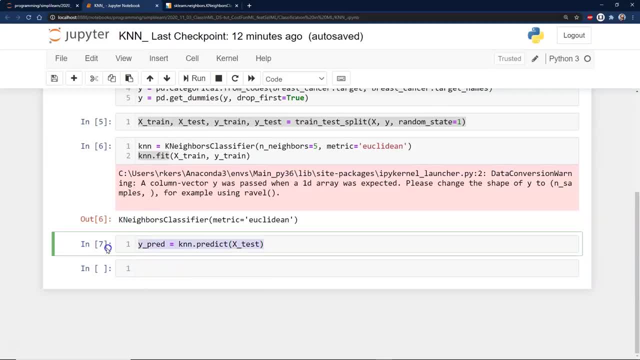 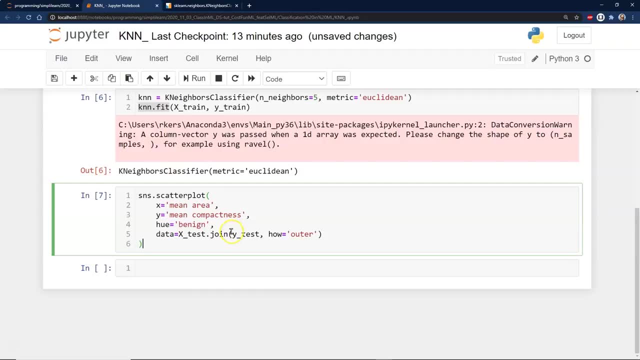 Now, before we look at our prediction- in fact, I am going to bring this down and put it back in here later- Let us take a look at our x test data. versus the y test, What does it look like? And so we have our mean area. 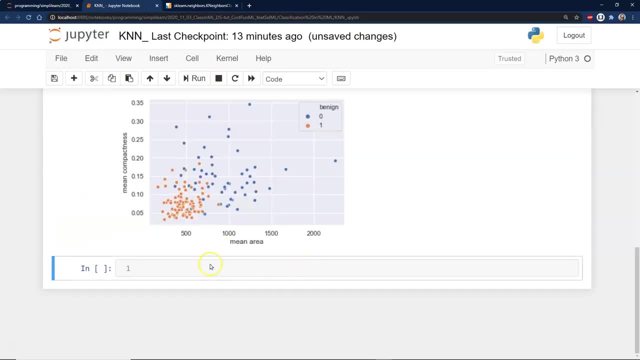 We are going to compare it to our mean compactness. We are going to go ahead and run that And we can see here the data. if you look at this, just eyeballing it, We put it in here. We have a lot of blue here. 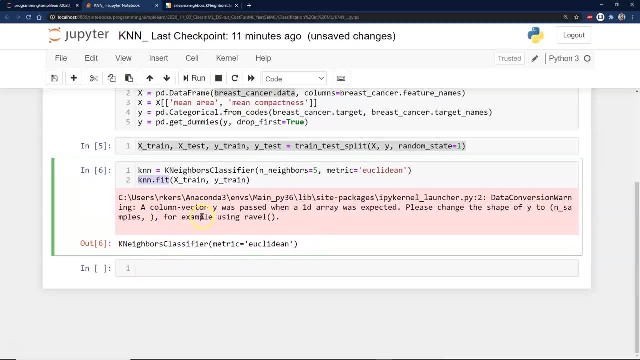 get into neural networks And then you have your K neighbors. It just tells you: we created a K neighbors setup. They kind of wanted us to reformat the Y, but it's not that big of a deal for this. It comes out and shows you that we're using the Euclidean metric for our measurement. So now we've. 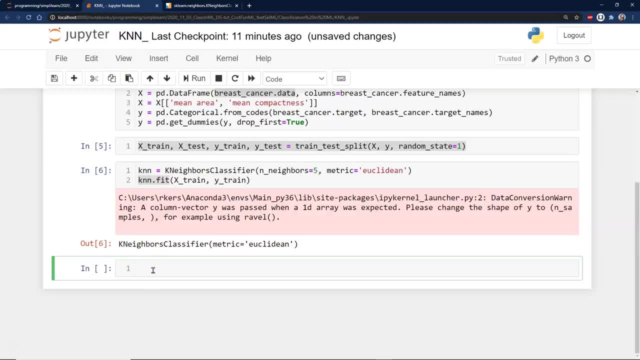 created a model. Here's our live model. We fitted the data to it. We say: hey, here's our training data, Let's go ahead and predict it. So we're going to take our Y predict equals KNN predict Y test. So this is data. we have not. this model has not seen this data, And so we're going to. 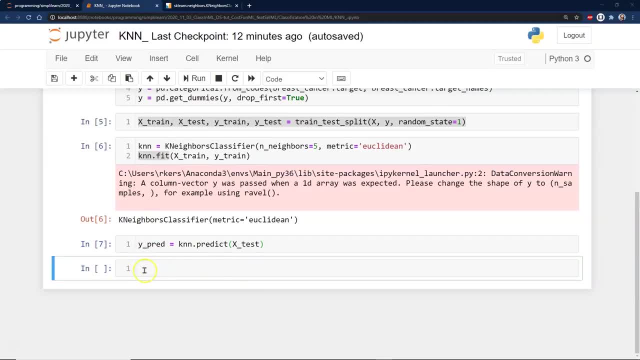 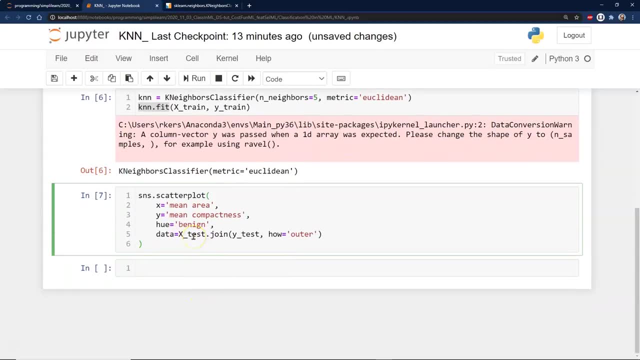 create a whole new set of data off of there. Now, before we look at our prediction- in fact, I'm going to bring this down and put it back in here later- Let's take a look at our X test data versus the Y test. What does it look like? And so we have our. 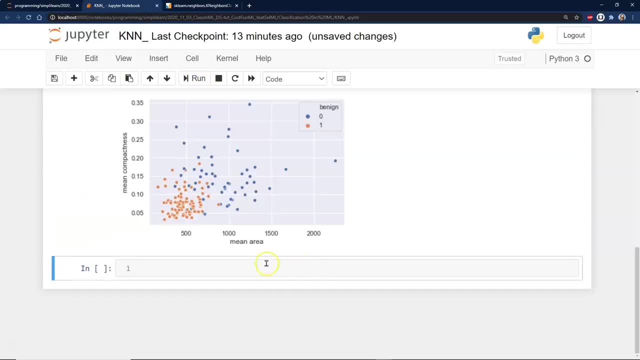 mean area. We're going to compare it to our mean compactness. We're going to go ahead and run that And we can see here the data. If you look at this, just eyeballing it, we put it in here. We have a. 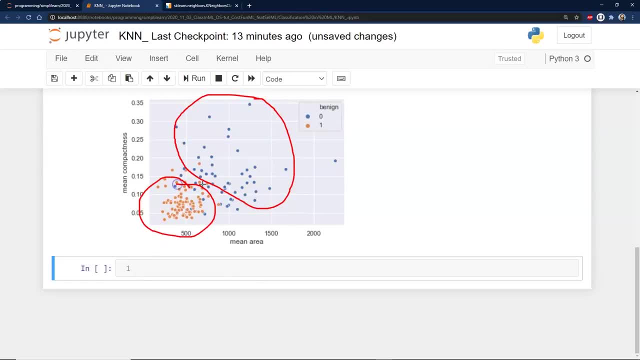 lot of blue here and we have a lot of orange here, And so these dots in the middle, especially like this one here and these here, these are the ones that are going to give us false negatives, And so we should expect. this is your noise. This is where we're not sure what it. 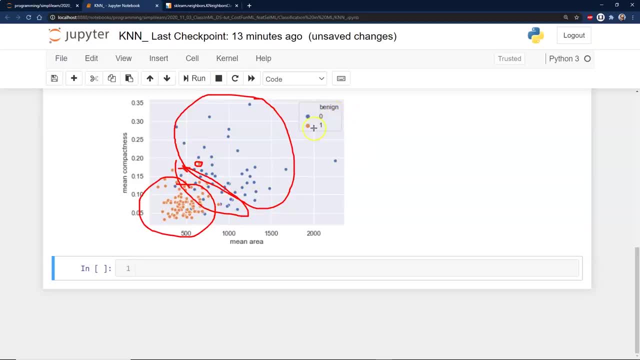 is, And then B9 is, in this case, is done in blue and malignant is done in one. So, if you look at it, there's two points based on these features, which makes it really hard to have 100% where the 100%. 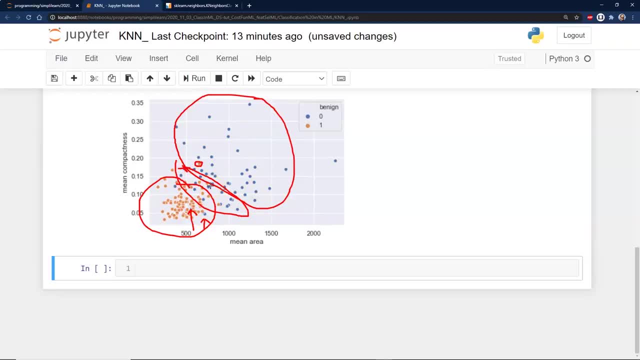 is down here or up here. That's kind of the thing I'd be looking for when we're talking about cancer and stuff like that, where you really don't want any false negatives, You want everything false positive. great, You're going to go in there and have another setup in there where you 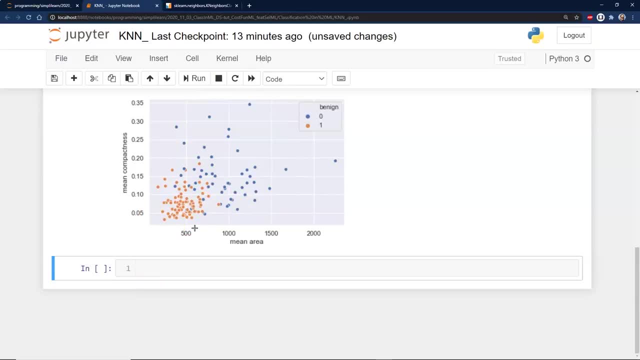 might get a, get an autopsy or something like that done on it. Again, that's very data specific on here. So now let's go ahead and pull in and get our prediction in here and we'll create our Y prediction. We'll go and run that. So now this is loaded with what we think the unknown data is. 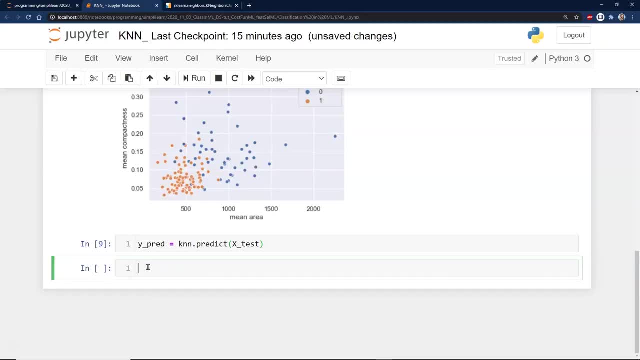 going to be, And we can go ahead and take that and go ahead and plot it, because it's always nice to have some pretty pictures And when we plot it we're going to have some pretty pictures. And when we plot it we're going to have some pretty pictures. And when we plot it, we're going to have 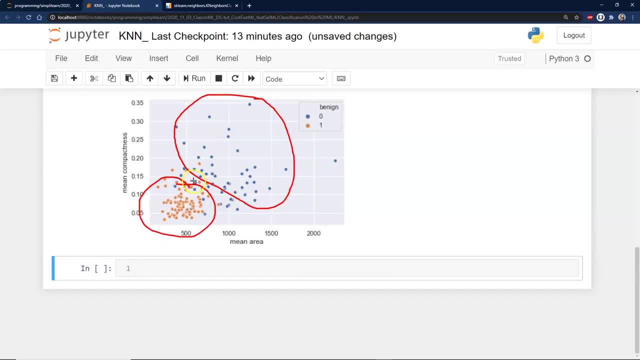 And we have a lot of orange here, And so these dots in the middle, especially like this one here and these here, these are the ones that are going to give us false negatives, And so we should expect. this is your noise. This is where we are not sure what it is. 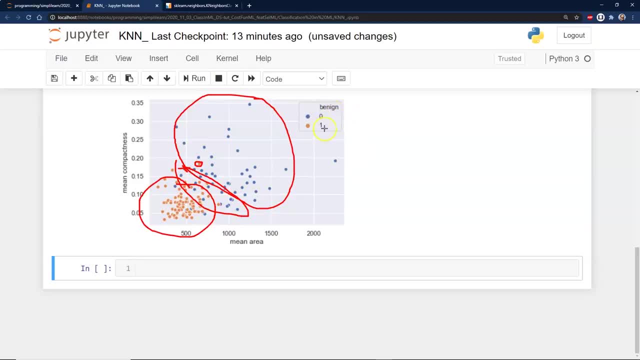 And then b9, in this case, is done in blue And malignant is done in one. So if you look at it, there are two points based on these features, which makes it really hard to have 100% where the 100% is down here or up here. 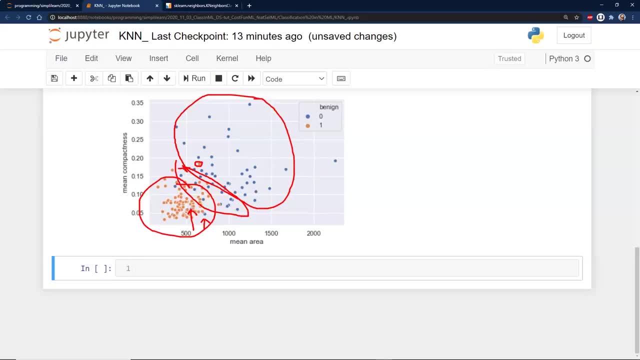 That is kind of the thing I would be looking for when we are talking about cancer and stuff like that, where you really do not want any false negatives, You want everything false positive. great, You are going to go in there and have another setup in there. 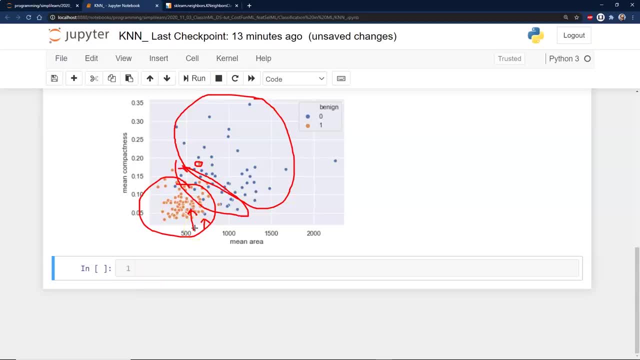 where you might get an autopsy or something like that done on it. Again, that is very data specific on here. So now let us go ahead and pull in and get our prediction in here And we will create our Y prediction. We will go ahead and run that. 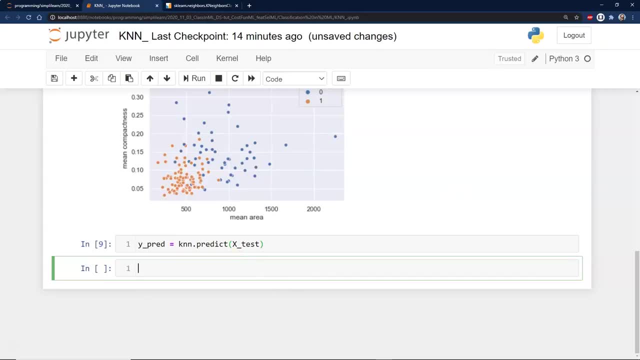 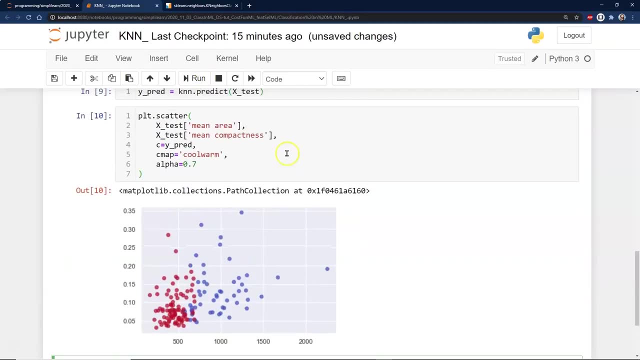 So now this is loaded with what we think the unknown data is going to be, And we can go ahead and take that and go ahead and plot it, because it is always nice to have some pretty pictures And when we plot it we are going to do the mean area versus mean compactness. 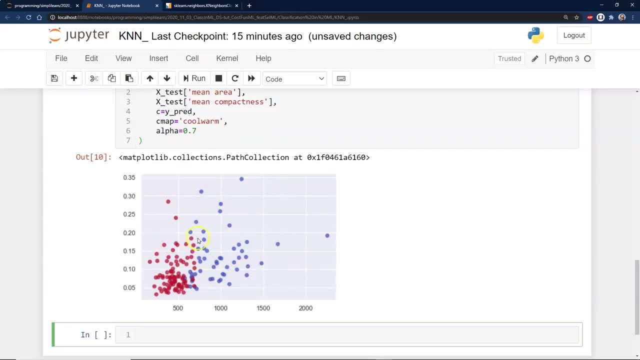 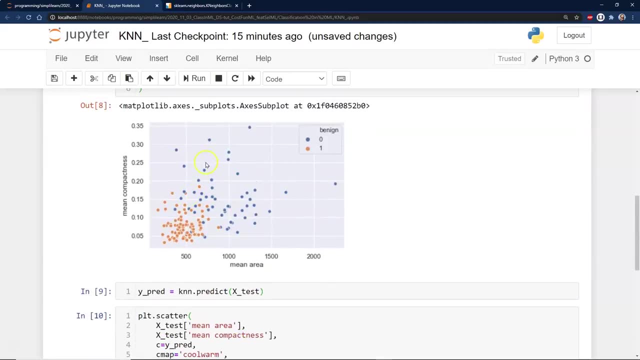 Again, you look at this map and you can see that there is some clear division here. We can clearly see on some of this stuff that our Y prediction- if we look at this map up here and this map down here, we probably got some pretty good deal. 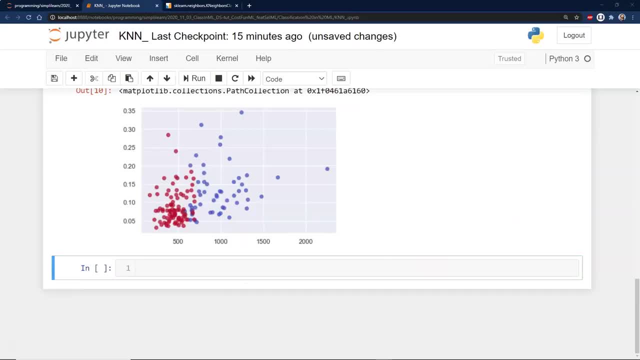 It looks pretty good, like they match a lot. This is, of course, just eyeballing it. Obviously you do not want to eyeball these things. You want to show people the pictures so that they can see it and you can say, hey, this is what it looks like. 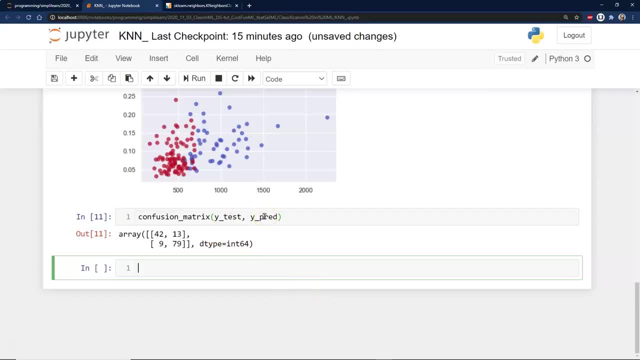 But we really want the confusion matrix And when we do the Y test and the Y predict, we can see in the confusion matrix here it did pretty good And we will just go ahead and point that out real quick. Here is our 42,. 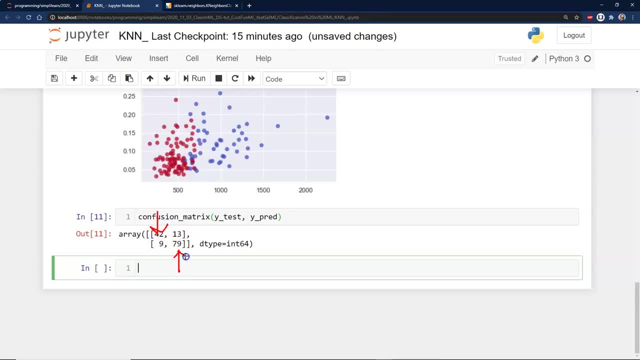 which is positive, And our 79. And if I remember correctly- I would have to look at the data- which one of these is a false negative 99. That is scary. I would not want to be one of those nine people. 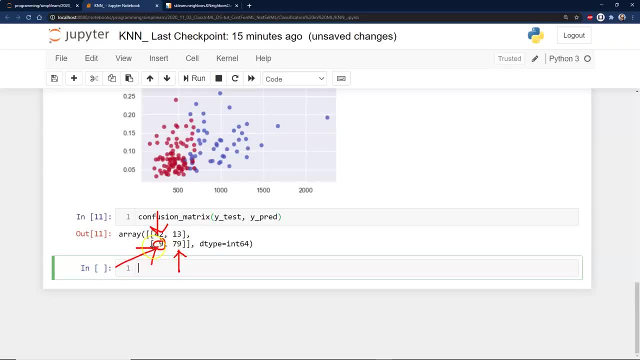 told that I do not have cancer and then suddenly find out I do. So we would need to find a way to sort this out, And there is different ways to do that. A little bit past this, but you can start messing with the actual Euclidean geometry. 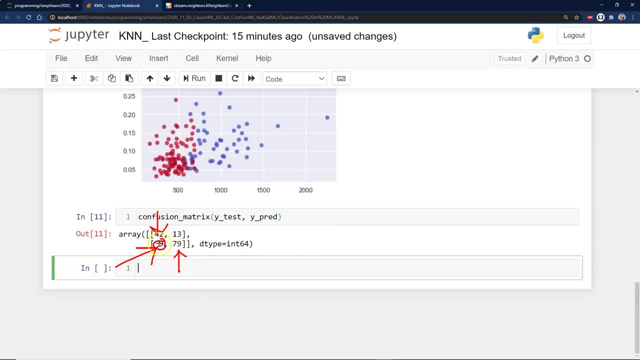 and the activation measurements and start changing those and how they interact. But that is very advanced. There is also other ways to classify them or to create a whole other class right here. Those are just a couple of the solutions you might use for that, But for a lot of things this works out great. 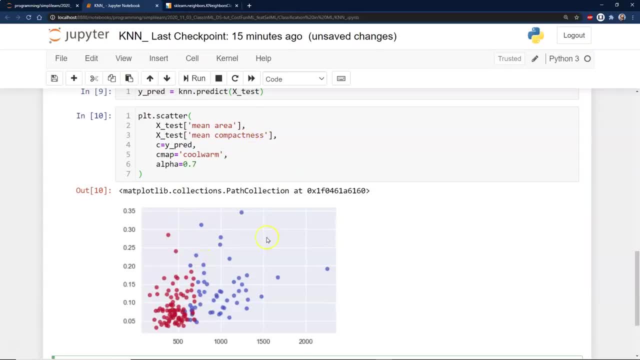 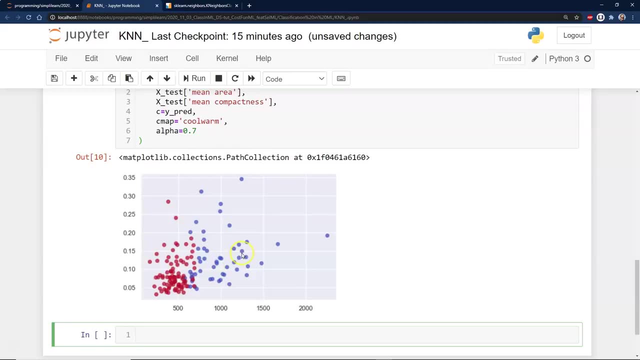 some pretty pictures And when we plot it, we're going to have some pretty pictures And we're going to do the mean area versus mean compactness. Again, you look at this map and you can see that there's some clear division here. We can clearly say on some of this stuff that our Y 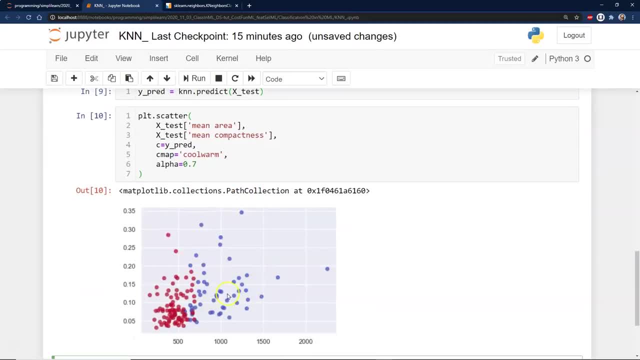 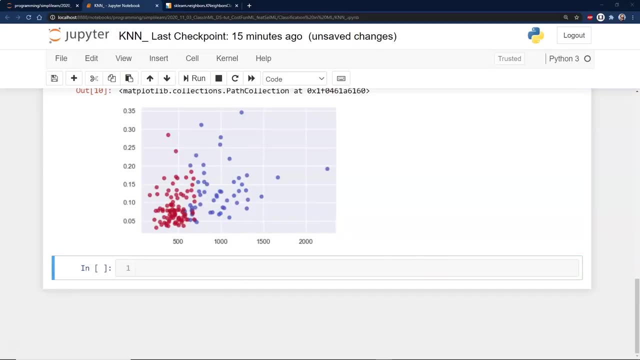 prediction. if we look at this map up here and this map down here, we probably got some pretty good deal. It looks pretty good like they match a lot. This is, of course, just eyeballing it. Really, you don't want to eyeball these things. You want to show people the pictures so that they 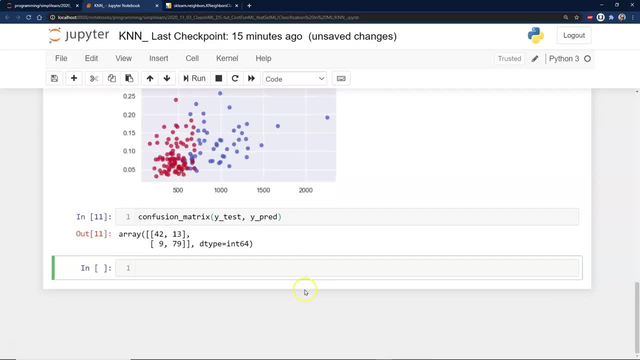 can see it. You can say, hey, this is what it looks like. but we really want the confusion matrix and we do the y test and the y predict. we can see in the confusion matrix here it did pretty good and we'll just go ahead and point that out real quick. here's our 42, which is positive, and our 79. 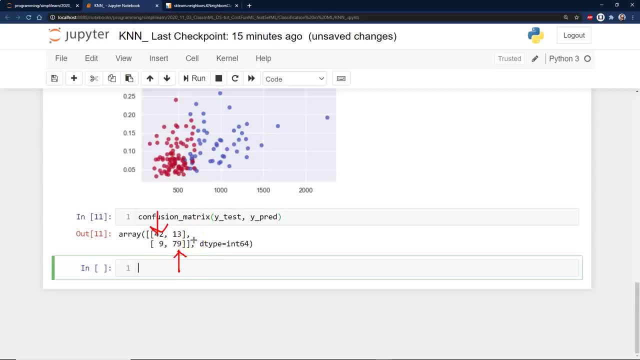 and, if i remember correctly, i'd have to look at the data. which one of these is a false negative? i believe it's the nine. that's scary. i would not want to be one of those nine people told that i don't have cancer and then suddenly find out i do. so we would need to find a way to sort this out. 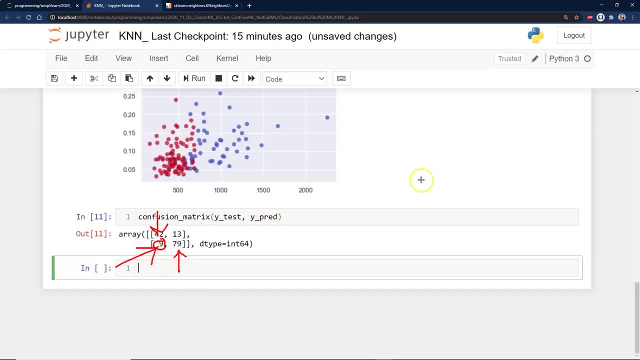 and there is different ways to do that a little bit past this, but you can start messing with the actual euclidean geometry and the activation measurements and start changing those and how they interact, but that's very advanced. there's also other ways to classify them or to create. 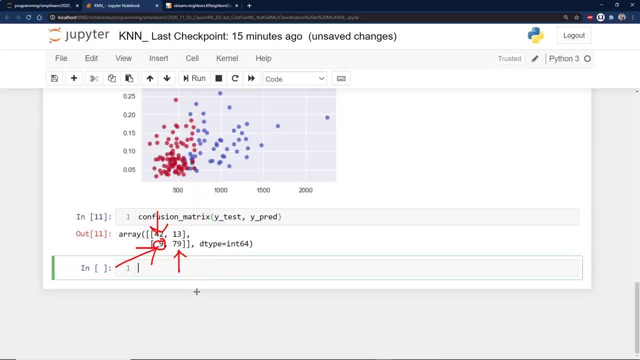 a whole nother class right here of we don't knows. those are just a couple of the solutions you might use for that, but for a lot of things this works out great. you can see here, you know, maybe you're trying to sell something. well, if this was not life dependent. 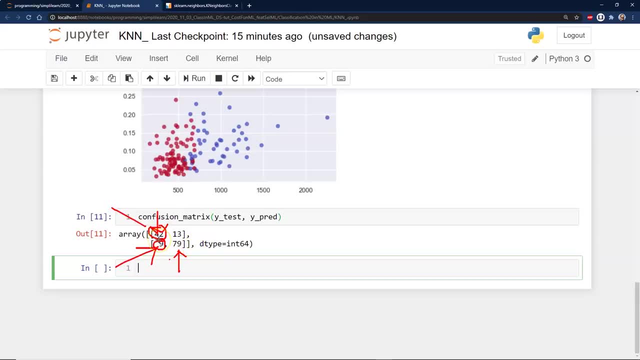 and this was: if i display this ad, 42 of these people are going to buy it, and if i display this other ad- if i don't display it- 79 people are going to go a different direction or whatever it is. so maybe you're trying to display whether they're going to buy something if you add it on to the 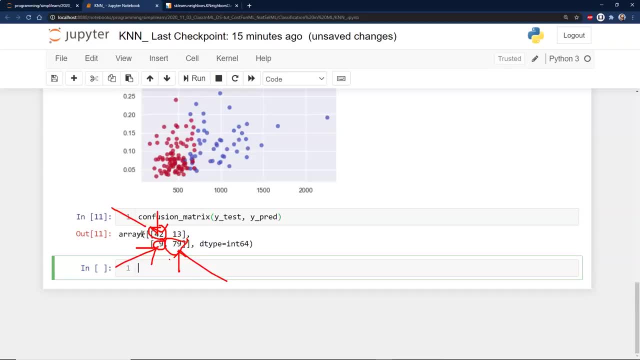 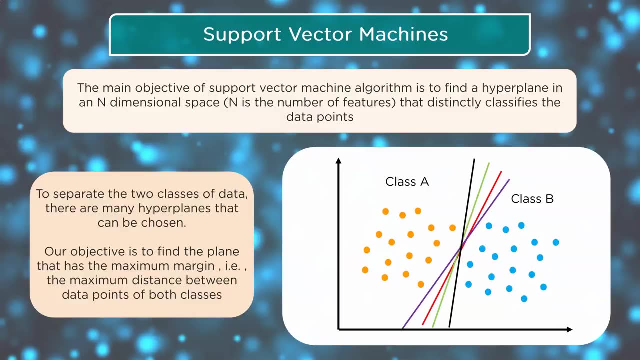 website, in which case that's really a good numbers. you've just added a huge number of cells to your company. so that was our k nearest neighbors. let's see, here we go. let's go ahead and take a look at support vector machines. so support vector machines is the main. 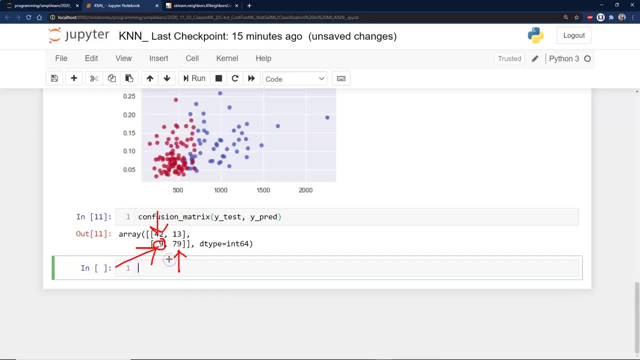 You can see here, maybe you are trying to sell something. Well, if this was not life dependent- and this was, if I display this ad, 42 of these people are going to buy it. And if I display this other ad, if I do not display it, 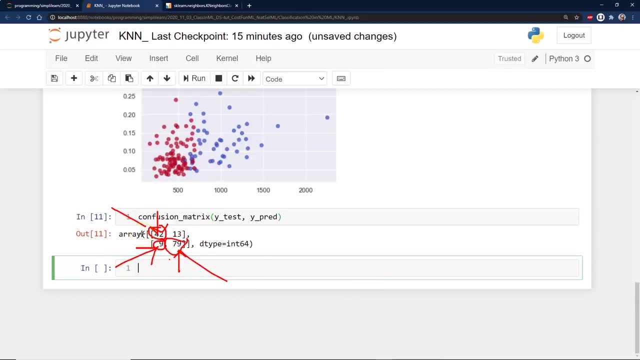 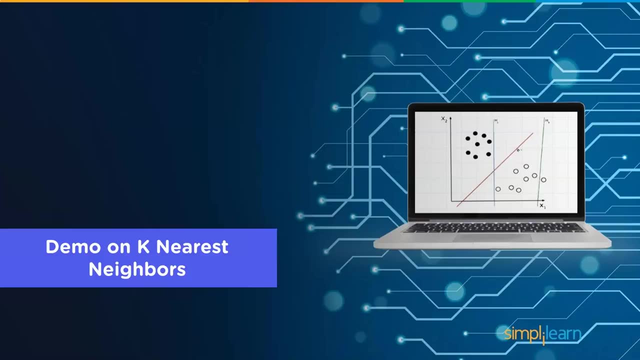 79 people are going to go a different direction or whatever it is. So maybe you are trying to display whether they are going to buy something or whether they are going to sell something to your company. So that was our k nearest neighbors. Let us go ahead and take a look at. 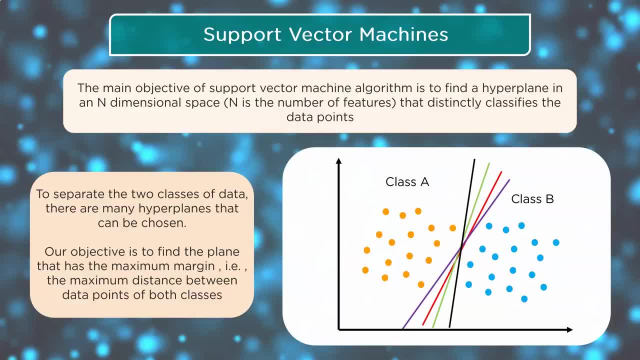 support vector machines. So support vector machines is. the main objective of a support vector machine algorithm is to find a hyperplane in an n-dimensional space. n is the number of features that distinctly classifies the data points. If you remember, we were just looking at. 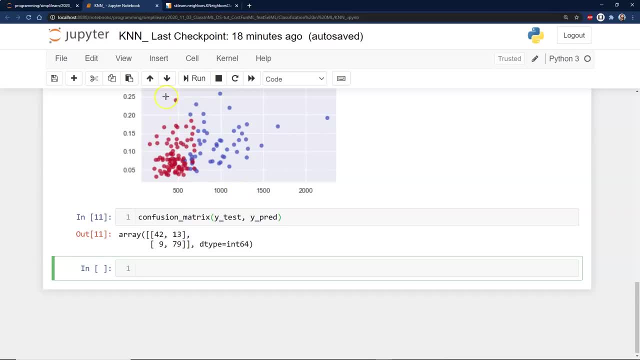 those nice graphs we had earlier. In fact, let me go ahead and flip back on over there. We might want to try to find a nice line through the data, And that is what we are talking about with this next setup. So the main objective of a 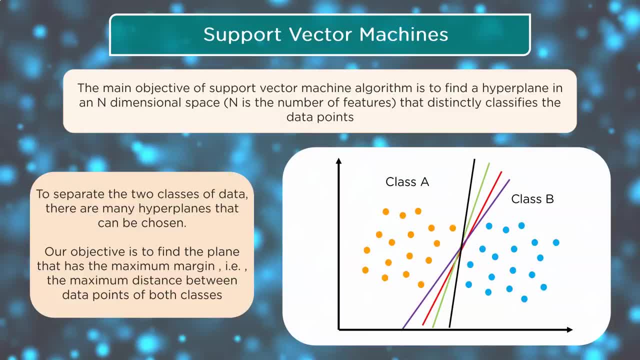 support vector machine algorithm is to find a hyperplane in an n-dimensional space. n is the number of features that distinctly classifies the data points To separate the two classes of data. there are many hyperplanes that can be chosen. Our objective is to find the plane. 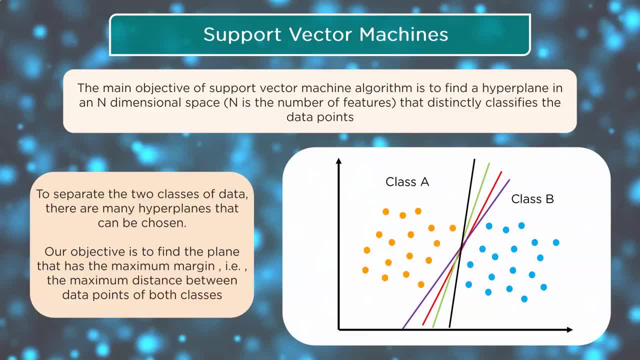 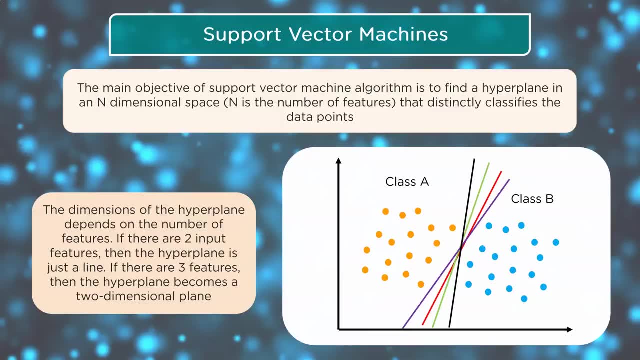 that has the maximum margin, ie the maximum distance between the data points of both classes. The dimensions of the hyperplane depends on the number of features. If there are two input features, then the hyperplane is just a line. If there are three features, 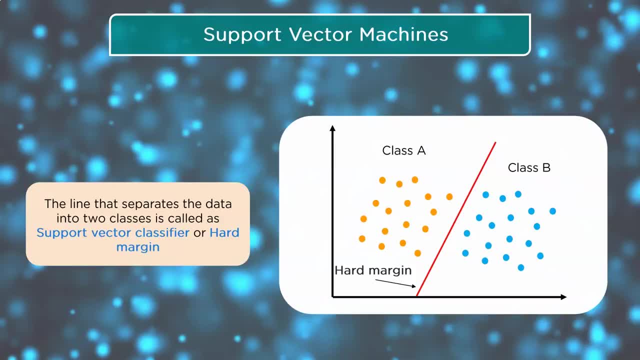 then the hyperplane becomes a two-dimensional plane. The line that separates the data into two classes is called as support vector classifier or hard margin. That is why I just showed you on the other data you can see here we look for a line that splits the data evenly. 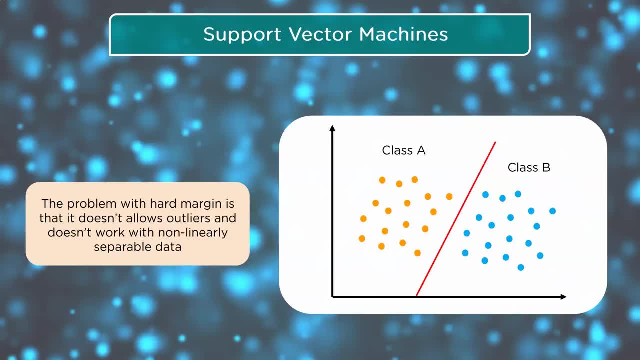 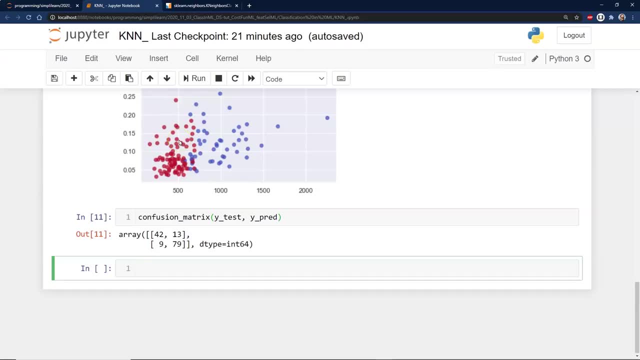 The problem with hard margin is that it allows outliers and doesn't work with non-linearly separable data. We just were looking at that. let me flip back on over here, and when we look at this setup in here and we look at this data here, we go: look how many outliers are in here. 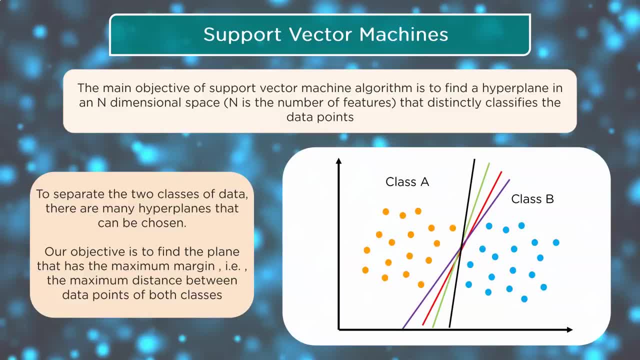 objective of a support vector machine algorithm is to find a hyper plane in an n dimensional space. in is the number of features that distinctly classifies the data points. if you remember, we were just looking at those nice graphs we had earlier, in fact, let me go and flip back on over. 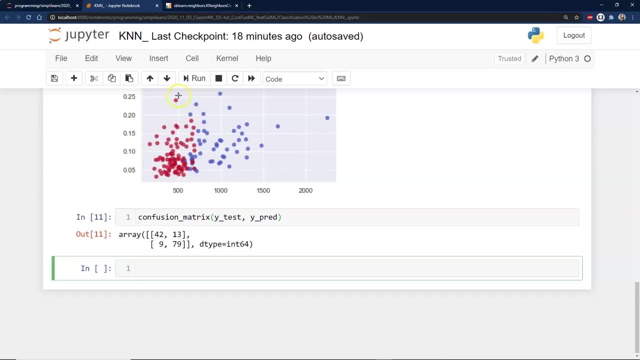 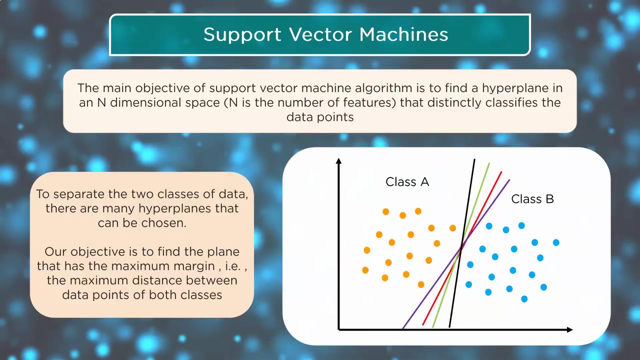 there. if we were looking at this data here we might want to try to find a nice line through the data. so the main objective of support vector machine algorithm is to find a hyper plane in an n dimensional space. in is the number of features that distinctly classifies the data. points to separate the two. 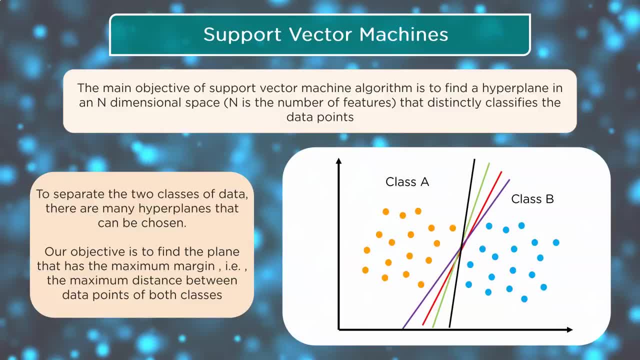 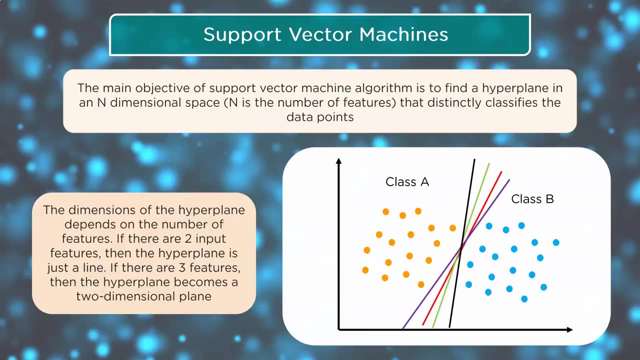 classes of data. there are many hyper planes that can be chosen. our objective is to find the plane that has the maximum margin, ie the maximum distance between data points of both classes. the dimensions of the hyper plane depends on the number of features. if there are two input features, then the hyper plane is just a. 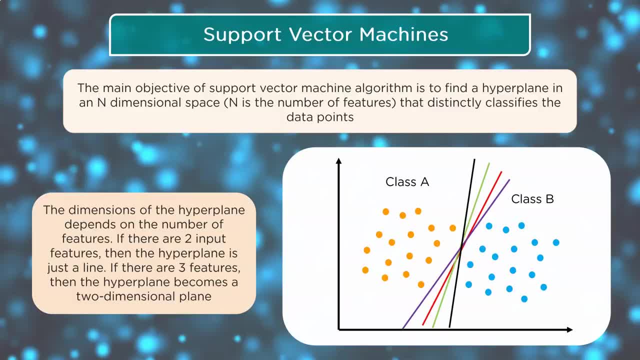 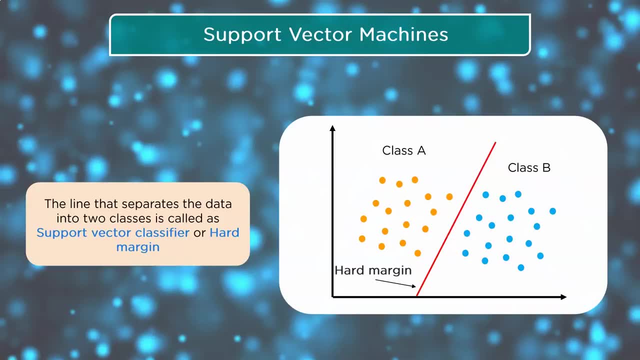 line. if there are three features, then the hyper plane becomes a two dimensional plane. the line that separates the data to two classes is called as support vector, classifier or hard margin. that's why I just showed you on the other data you can see here we look for a line that splits the data. 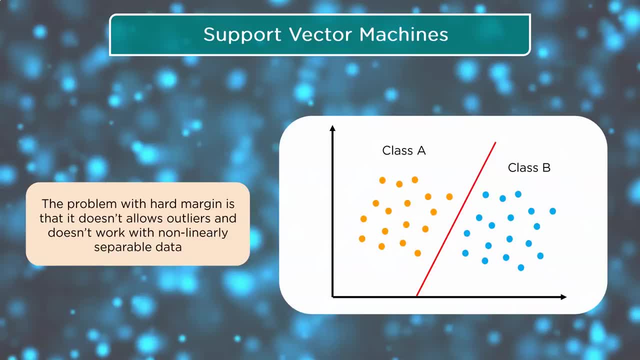 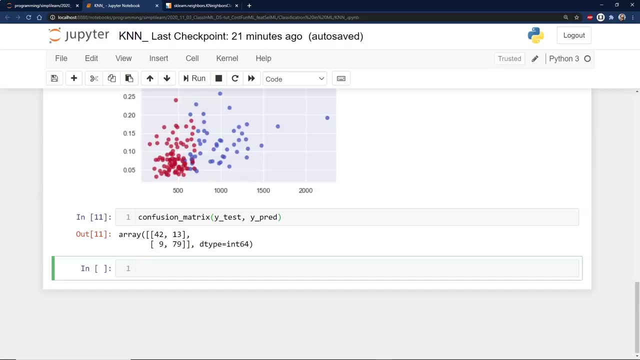 evenly. the problem with hard margin is that it doesn't allow outliers and doesn't work with non-linearly separable data. We just were looking at that and we flip back on over here and when we look at this setup in here and we look at this data here, we go: look how many outliers are in here. 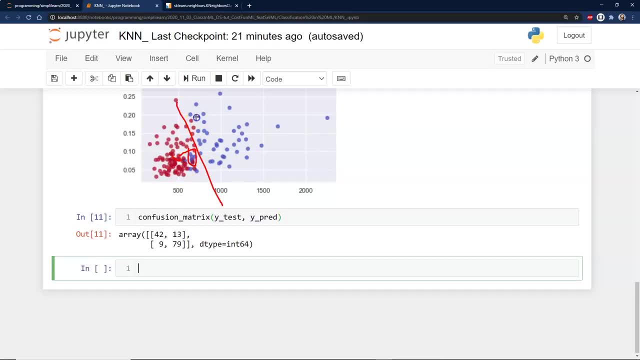 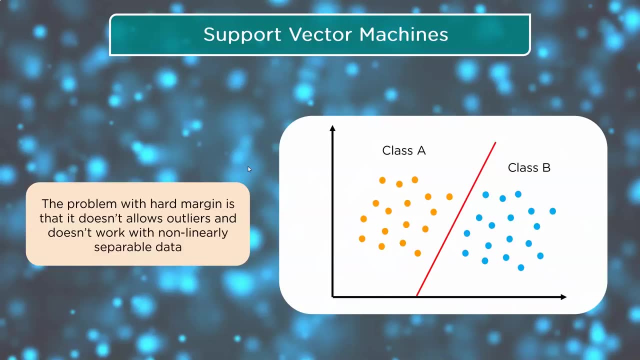 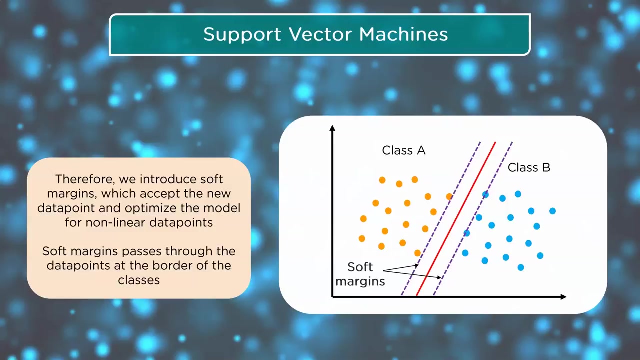 These are all, with all these blue dots on the wrong side of the line would be considered an outlier, and the same with the red line, and so it becomes very difficult to divide this data unless there's a clear space. There we go. Therefore, we introduce soft margins which accept the new data point and optimize a model for nonlinear data points. 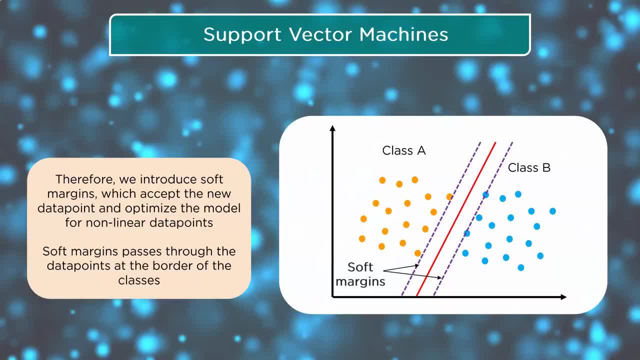 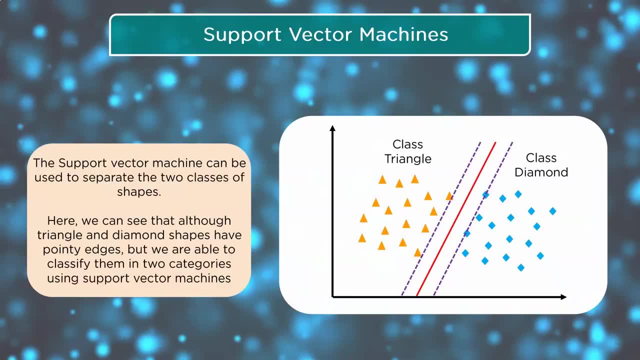 Soft margins pass through the data points at the border of the classes. The support vector machine can be used to separate the two classes of shapes. Here we can see that although triangles and diamond shapes have pointy edges, but we are able to classify them in two categories using a support vector machine. 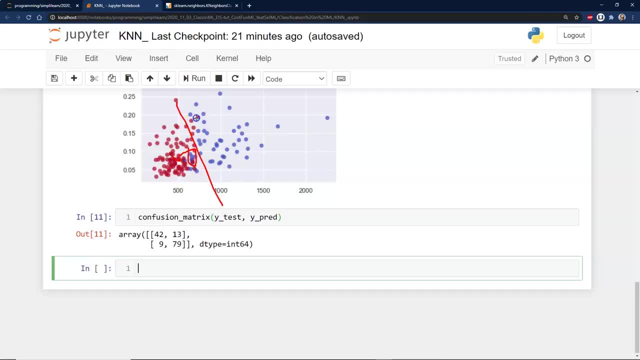 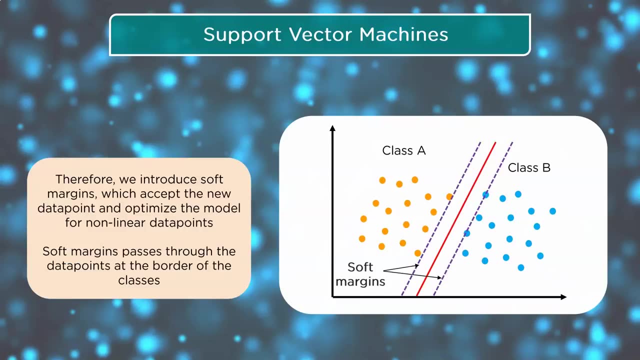 all these blue dots on the wrong side of the line would be considered an outlier, and the same with the red line. It becomes very difficult to divide this data unless there is a clear space. Therefore we introduce soft margins which accept the new data points. 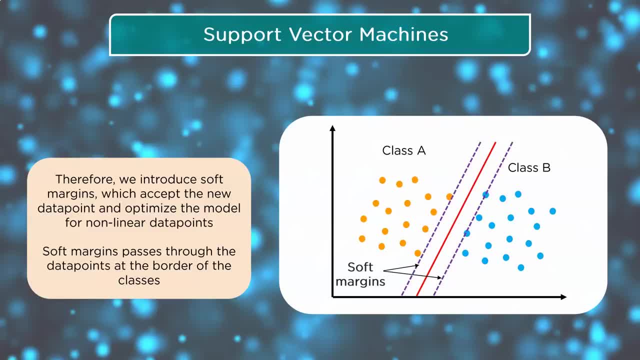 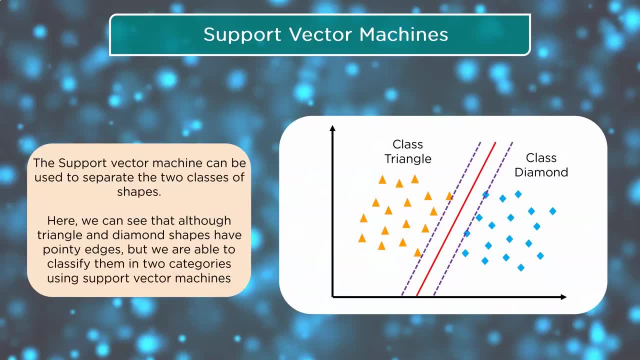 and optimize a model for non-linear data points. Soft margins pass through the data points at the border of the classes. The support vector machine can be used to separate the two classes of shapes. Here we can see that although triangles and diamond shapes have pointy edges, but we are able 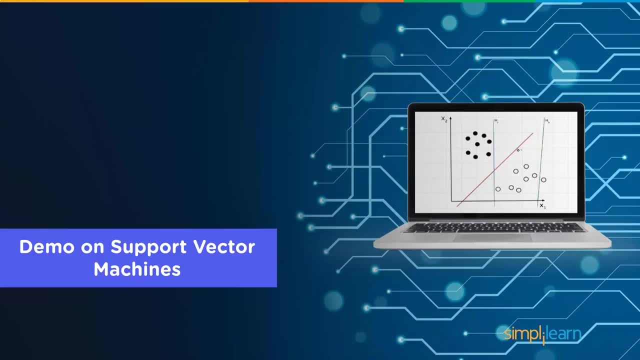 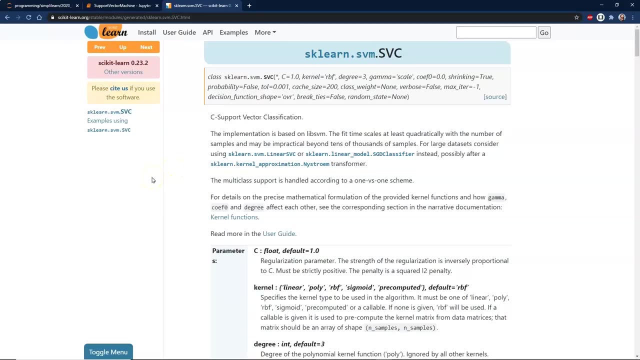 to classify them in two categories using a support vector machine. Let's go ahead and see what that looks like in a demo. Flip back on over to our Jupyter notebook. We always want to start with taking a look at the learn API, in this case the SVM-SVC. 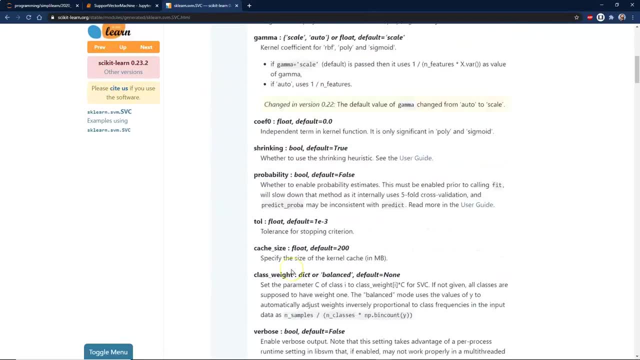 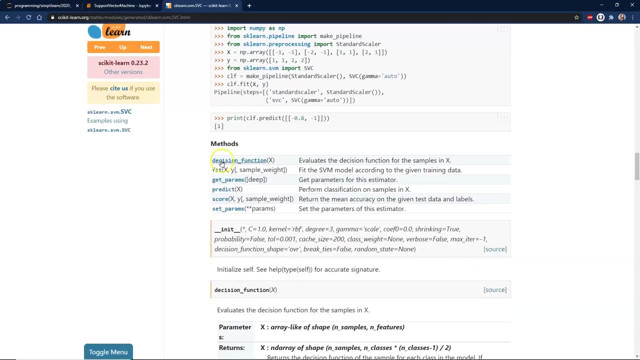 There is a significant number of parameters because the SVM has been in a lot of development in the recent years and has become very popular. If we scroll all the way down to methods, you'll see right here is our fit and our predict. that's what you should see. 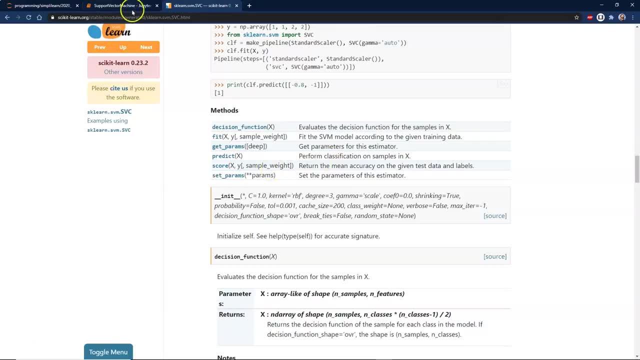 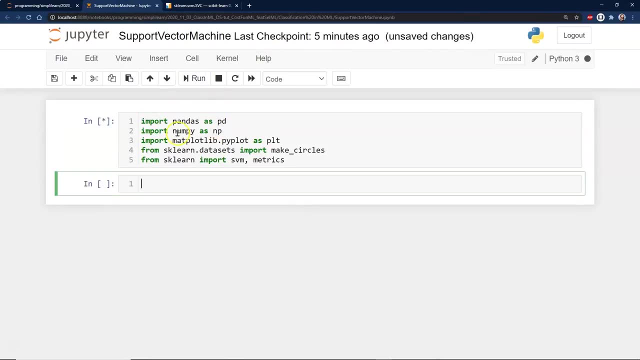 in most of the scikit-learn packages. So this should look very familiar to what we've already been working on And we'll go ahead and bring in our import and run that We should already have pandas numpy, our matplot library, which we're. 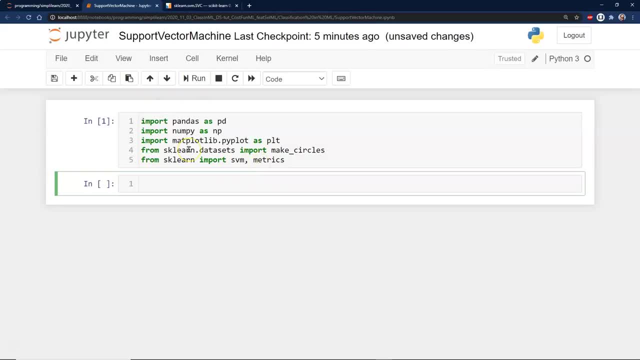 going to be using to graph some of the things A little bit different. right here you'll see that we're going to go ahead and bring in. one of the fun things you can do with test data is make circles. Circles are really hard to classify. 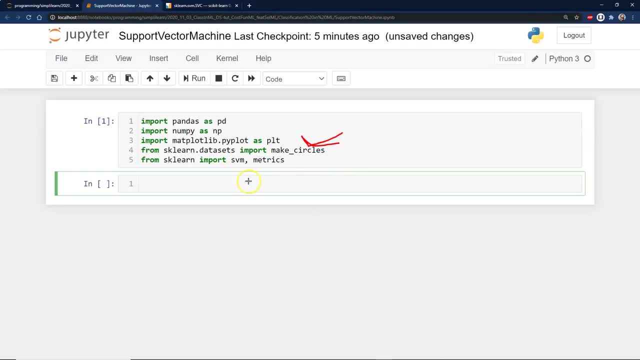 You have a ring on the inside and a ring on the outside and you can see where that can cause some issues. We'll take a look at that a little closer in a minute. Here's our SVM setup on there, and then, of course, our metrics, because we're going to use that to. 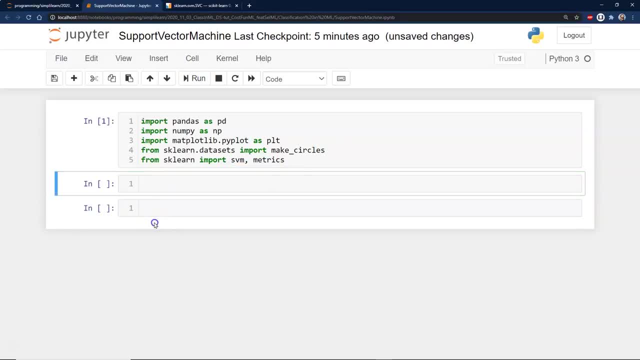 take a closer look at things. So we go ahead and run this. Once we've gone ahead and done that, we're going to go ahead and start making ourselves some data, And this part is probably a little bit more complicated than we need. I'm not going to go too much in. 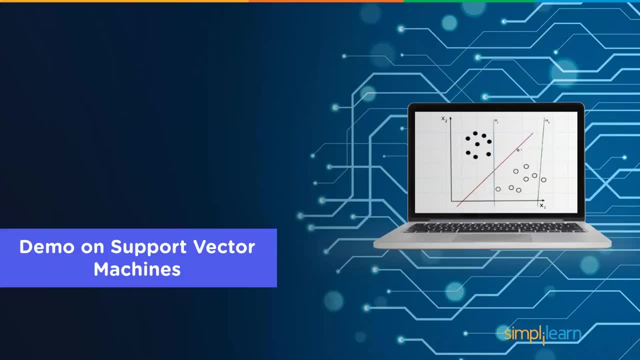 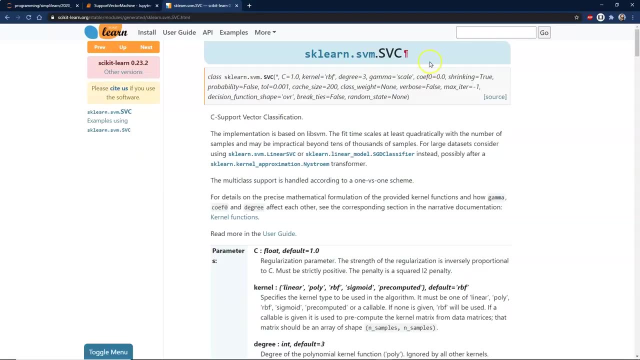 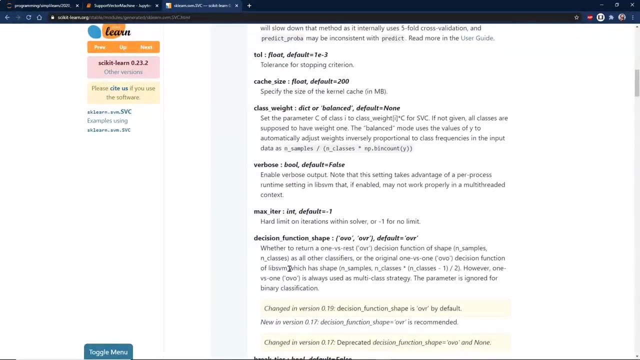 Let's go ahead and see what that looks like in a demo. We'll flip back on over to our Jupyter notebook. We always want to start with taking a look at the sklearn API, In this case the SVM. There is a significant number of parameters because the SVM has been a lot of development in the recent years and has become very popular. 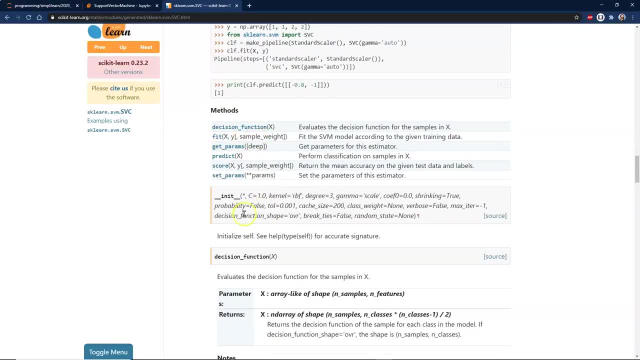 If we scroll all the way down to methods, you'll see right here is our fit and our predict. That's what you should see in most of the scikit-learn packages, So this should look very familiar to what we've already been working on. 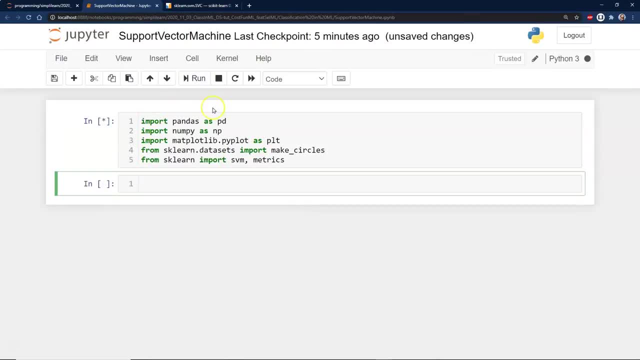 And we'll go ahead and bring in our import and run that. We should already have pandas, numpy, our matplotlib. We should already have a library which we're going to be using to graph some of the things a little bit different right here. 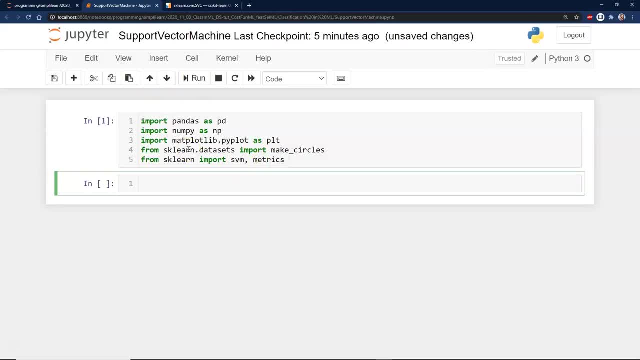 You'll see that we're going to go ahead and bring in. one of the fun things you can do with test data is make circles. Circles are really hard to classify. You have a ring on the inside and a ring on the outside and you can see where that can cause some issues. 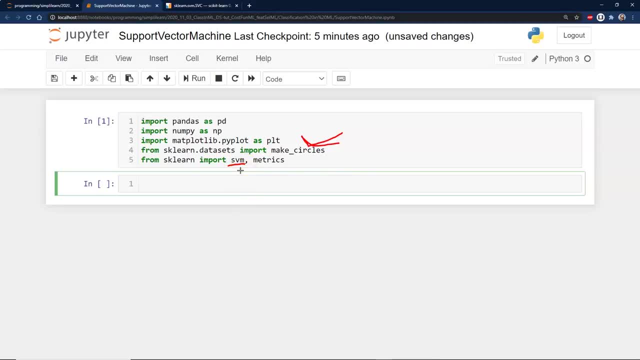 And we'll take a look at that a little closer in a minute. Here's our SVM set up on there And then, of course, our metrics, because we're going to use that to take a closer look at things. So we go and run this. 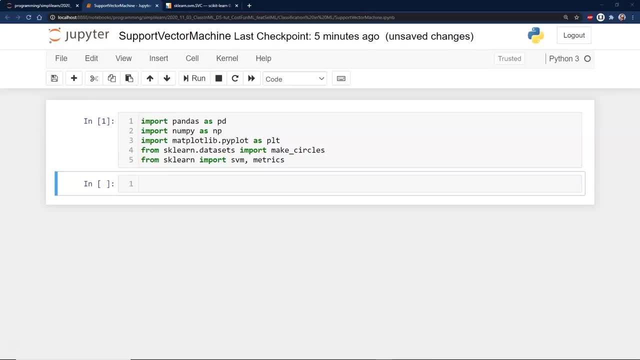 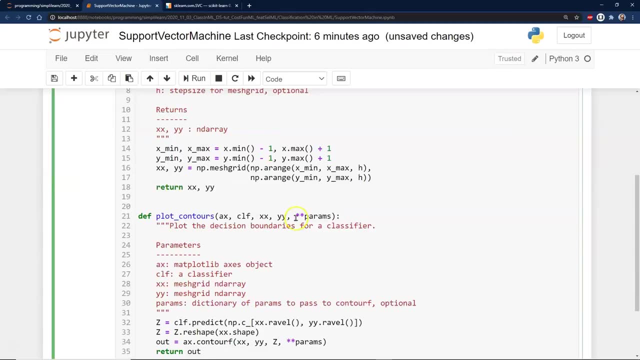 Whoops already did Once. we've gone ahead and done that, we're going to go ahead and start making ourselves some data And this part probably a little bit more complicated than we need. I'm not going to go too much in detail on it. 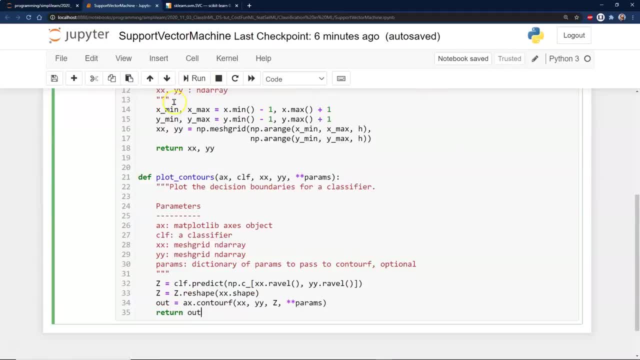 We're going to make a mesh grid and we'll see what that looks like in a minute. We're defining the minimums You can see in here. create a mesh grid of points. Here's our parameters of x, y and h. 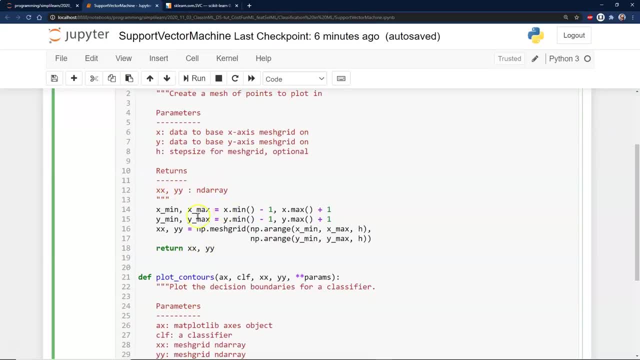 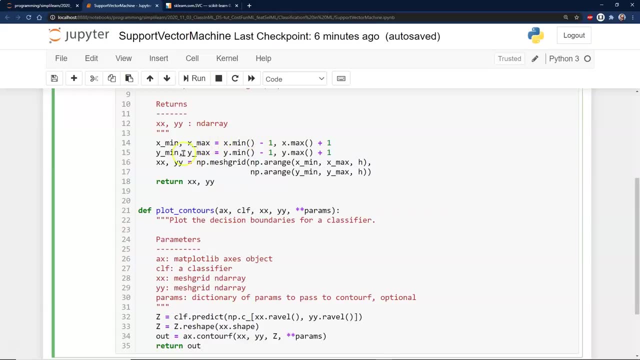 It's going to return x, x, y, y. You can also send a note to us. Make sure you get a copy of this if you want to dig deeper, Deeper into this particular code, especially- And we have a ymin ymax, ymin ymax plus 1.. 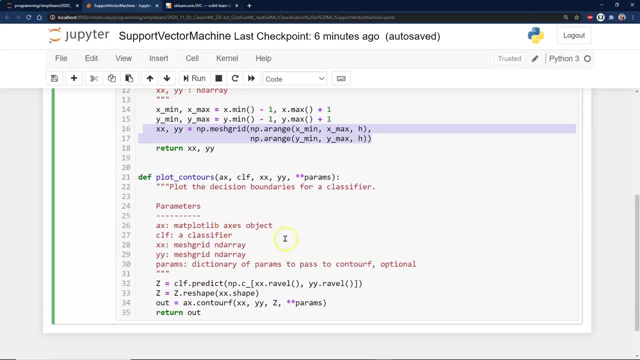 Here's our mesh grid. we're actually going to make x, x and y- y, Plot the contours all the way through, And this is just a way of creating data. It's kind of a fun way to create some data. 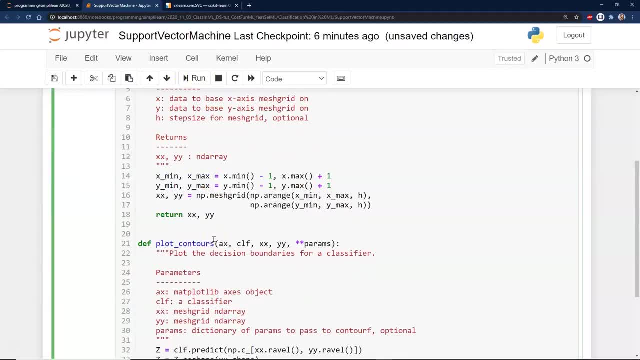 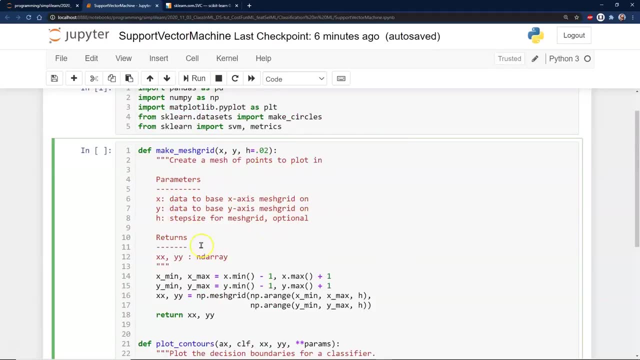 detail on it. We're going to make a mesh grid and we'll see what that looks like in a minute. We're defining the minimums You can see in here. create a mesh grid of points. Here's our parameters of x, y and h. It's going to 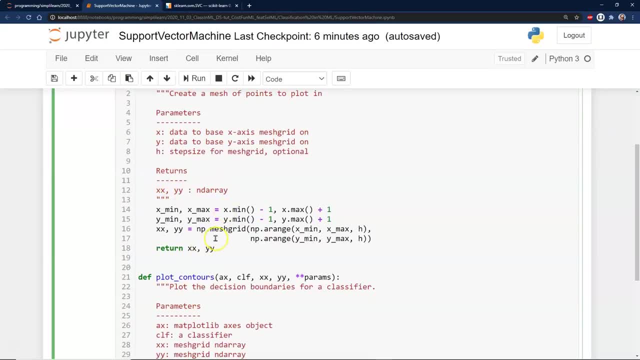 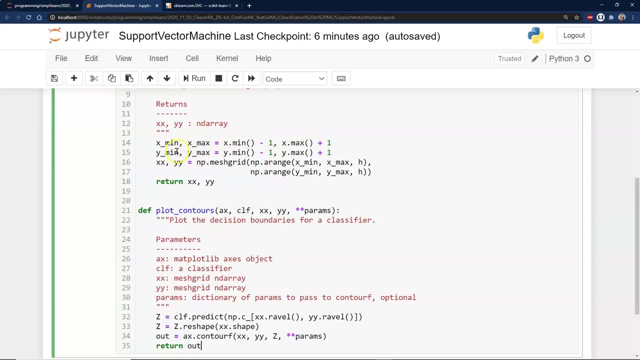 return x, x, y, y. You can also send a note to us. Make sure you get a copy of this if you want to dig deeper into this particular code especially. And we have a ymin ymax, ymin ymax plus 1.. Here's our mesh. 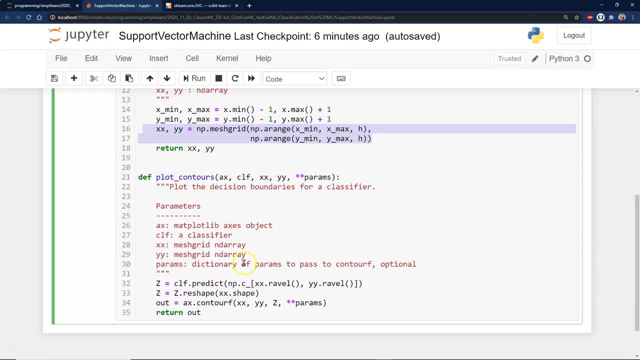 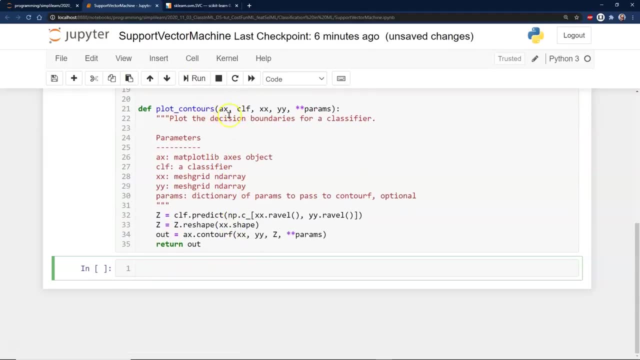 grid. we're actually going to make x, x and y, y, Plot the contours all the way through And this is just a way of creating data. It's kind of a fun way to create some data. We go plot contours ax, clf, x, x, y, y. 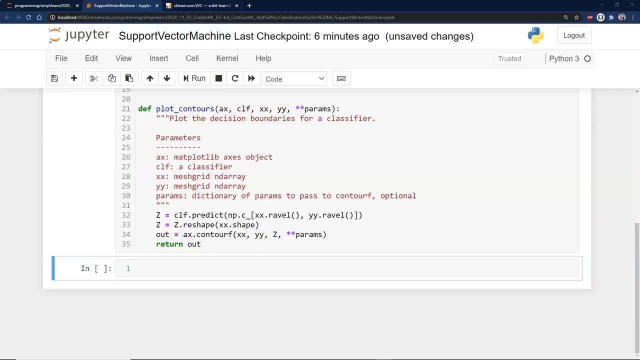 And return it out. Add some perimeters here so that when we're doing it we have our setup on there- Train property- And then we'll go ahead and make our data. Just throw that right in there too, in the same setup. 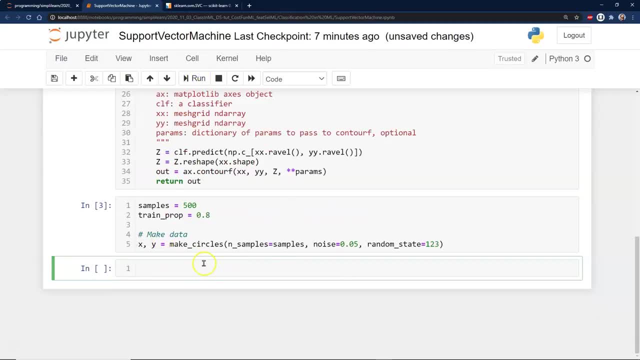 And run that. So now we have x and y. We're going to make our circles. We have nsamples, equals samples. In this case, we're going to have 500 samples. We went ahead and gave it noise of .05, random state of. 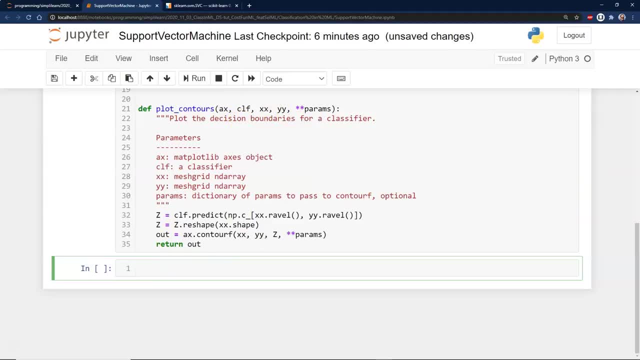 We go plot contours ax, clf, x, x, y, y And return it out. Add some perimeters here so that when we're doing it we have our setup on there- Train property- And then we'll go ahead and make our data. 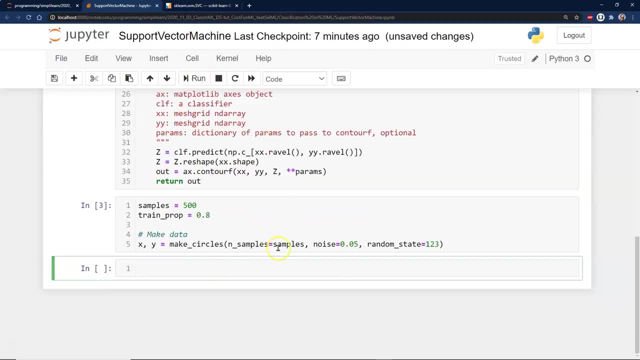 Just throw that right in there too in the same setup And run that. So now we have x and y. We're going to make our circles. We have n samples, equals samples. In this case, we're going to have 500 samples. 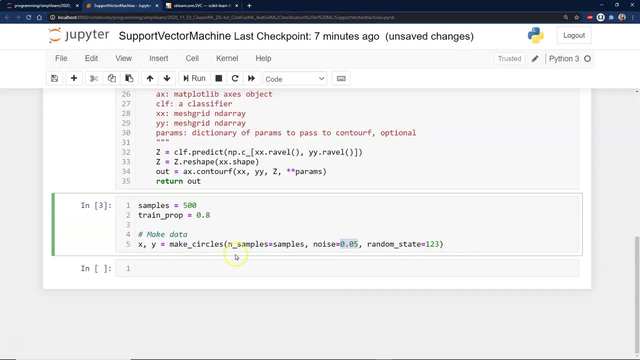 We went ahead and gave it noise of 0.05.. Random state 123.. These are all going into. oops, let's go back up. Here we go Make our mesh grid, Make circles. There it is, So this is going into our make circles. 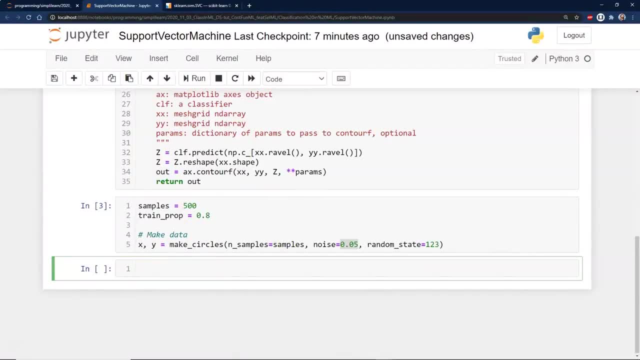 And this is part of that setup on this- And then, once we've gone ahead and make the circle, let's go ahead and plot it. That way you can see we're talking about. right now. what I'm saying is really confusing, because without a visual it doesn't really mean very much what we're actually doing. 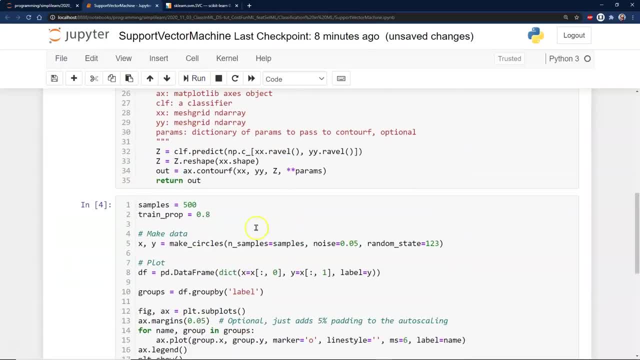 So let me go ahead and run this with the plot. Let's go back up here and just take a look. We've made our circle. We have our n samples, equals samples. We're going to have 500.. We're going to have training, property 0.8.. 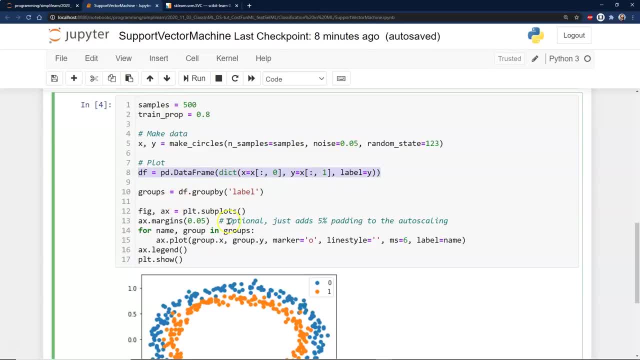 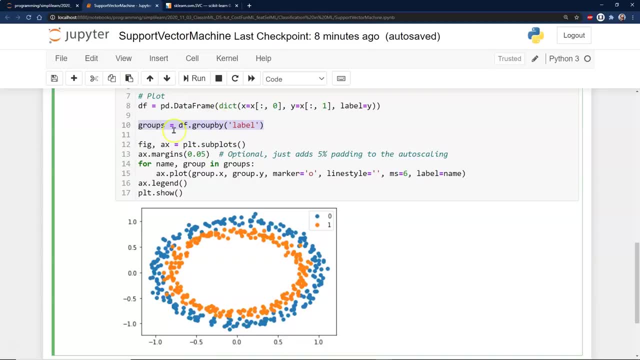 Here's our data frame. We go and load it into the data frame So we can plot it. Groups, df, group by label. This is kind of a fun way. if you have multiple columns you can really quickly pull whatever setup is in there. 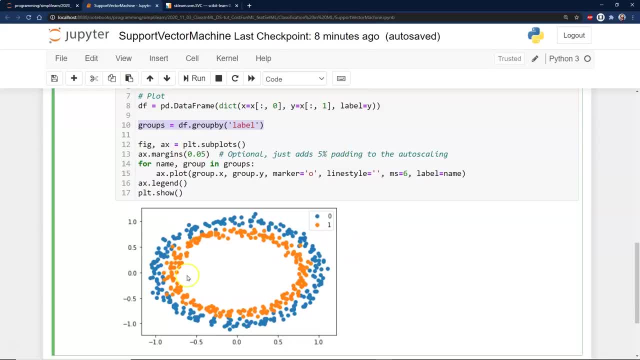 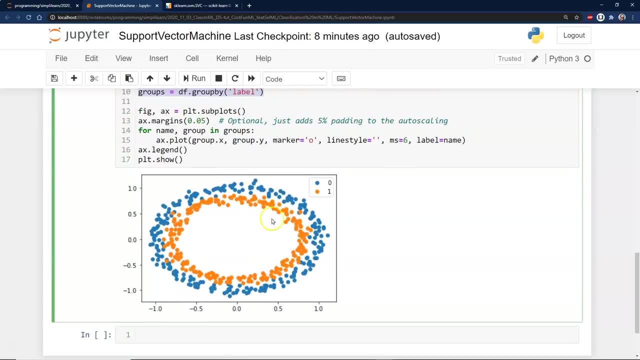 And then we go ahead and plot it And you can see, here we have two rings that are formed, And that's all this is doing is just making this data for us. This is really hard data to figure out. A lot of programs get confused in this because there's no straight line or anything like that. 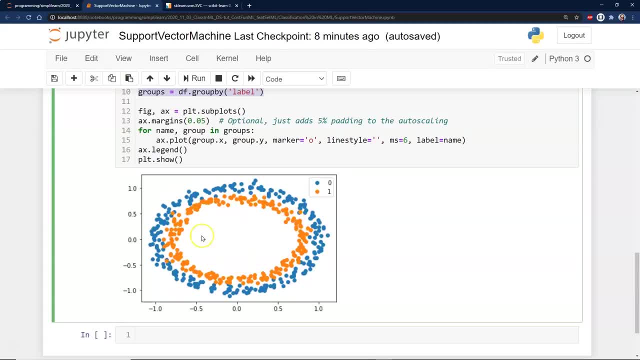 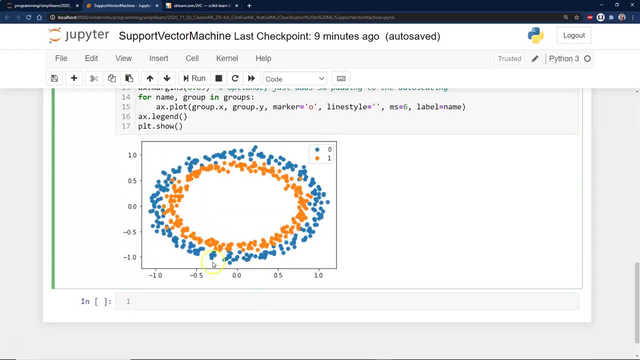 But we can add planes and different setups on here, And so you can see we have some very Interesting data. we have our zeros in blue and our ones in the yellow in the middle, And the data points are an x- y coordinate plot on this. 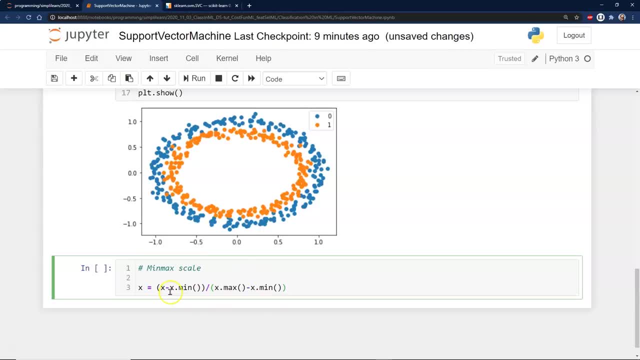 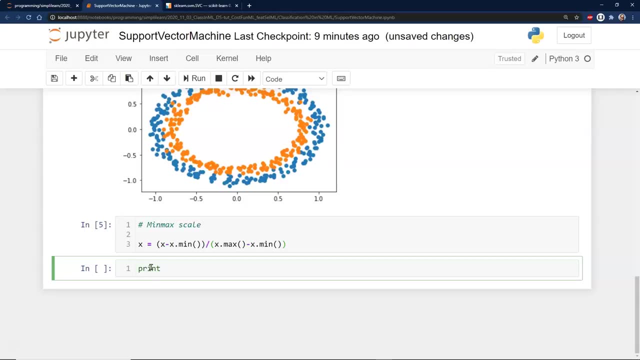 One of the things we might want to do on here is go ahead and find the min to max ratio set up in there, And we can even do this. just do a print x. You can see what the data looks like that we're producing on this. 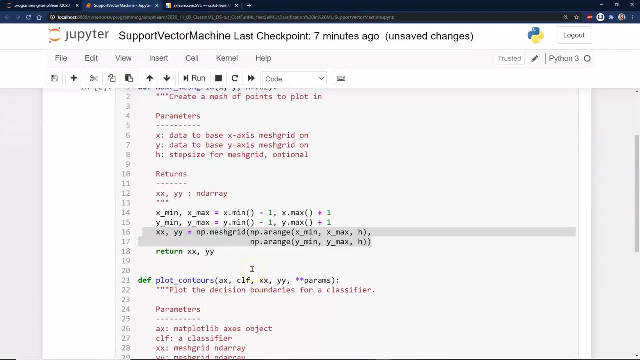 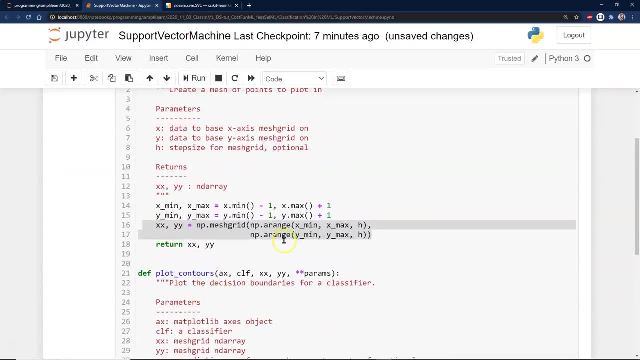 123.. These are all going into oops, let's go back up. Here we go, Make our mesh grid, Make circles. There it is. So this is going into our make circles up here And this is part of that setup on this. 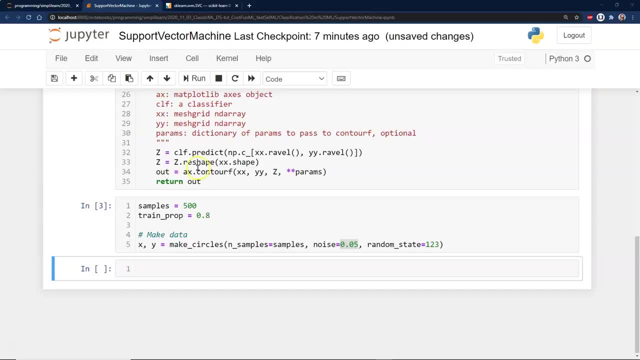 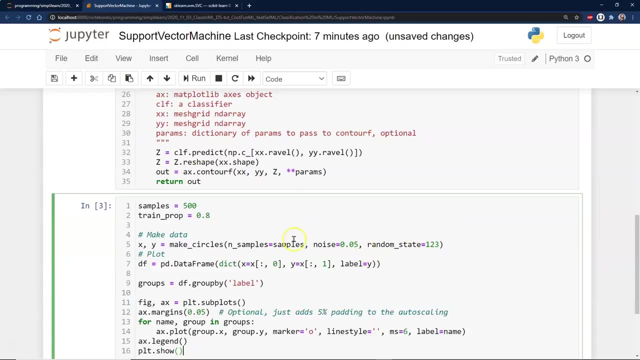 And then, once we've gone ahead and make the circle, let's go ahead and plot it. That way you can see what we're talking about. Right now. what I'm saying is really confusing, because without a visual it doesn't really mean very much. 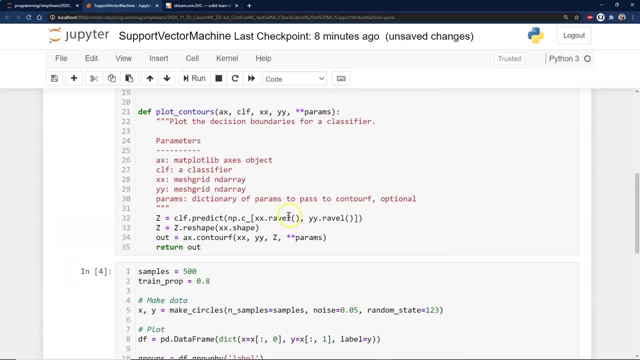 what we're actually doing. So I'm going to go ahead and run this with the plot. Let's go back up here and just take a look. We've made our circle. We have our nsamples- equals samples. We're going to have 500.. We're going to have 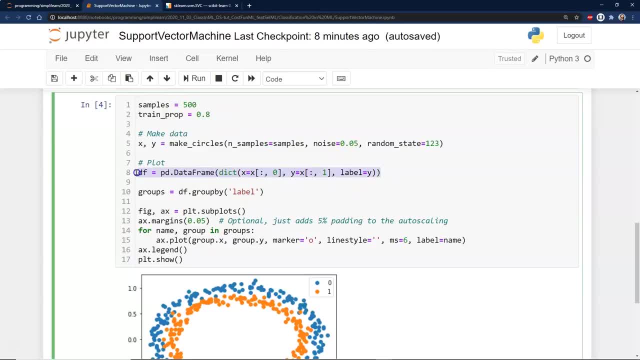 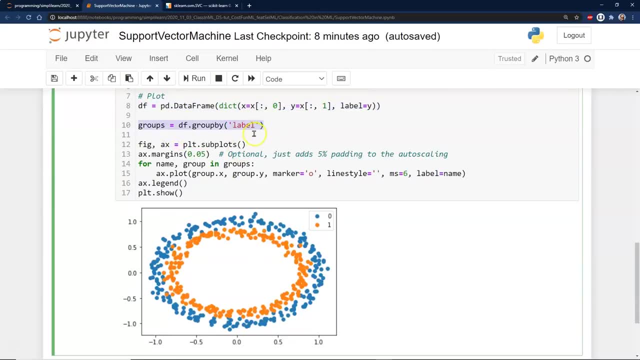 training: property .8.. Here's our data frame. We go ahead and load it into the data frame so we can plot it. Groups df: group by label. This is kind of a fun way. if you have multiple columns you can really quickly pull whatever setup. 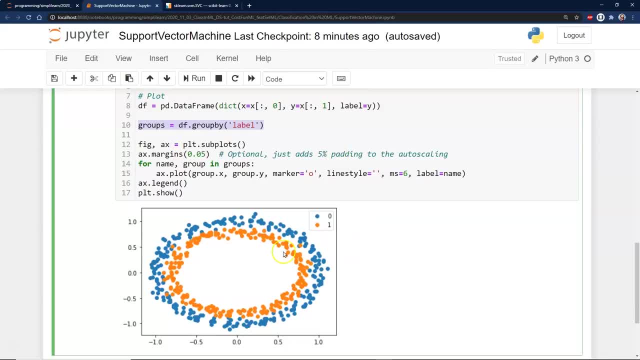 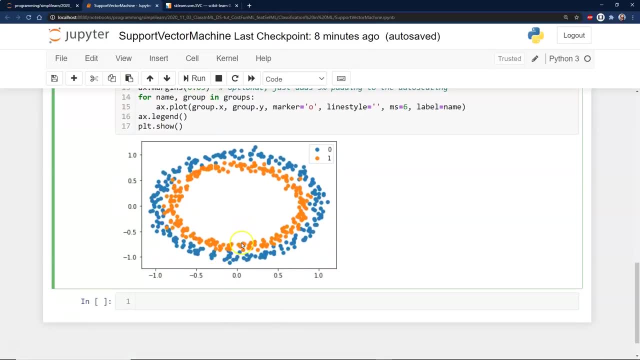 is in there, And then we go ahead and plot it And you can see, here we have two rings that are formed, And that's all this is doing is just making this data for us. This is really hard data to figure out. A lot of programs get. 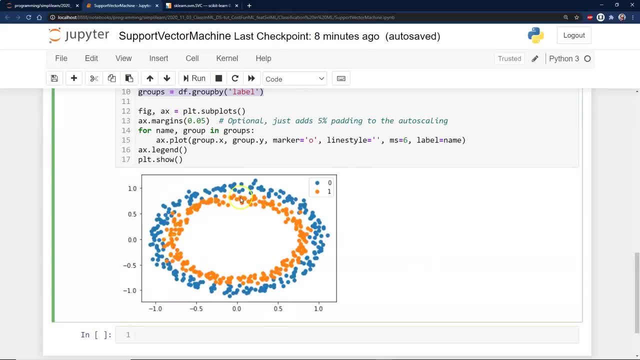 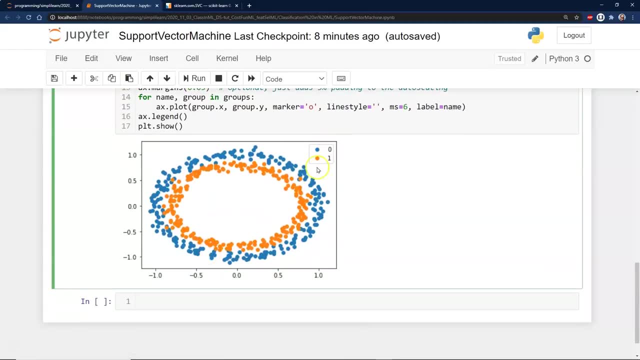 confused in this because there's no straight line or anything like that, But we can add planes and different setups on here, And so you can see we have some very interesting data. We have our zeros in blue and our ones in the yellow in the middle, And the data. 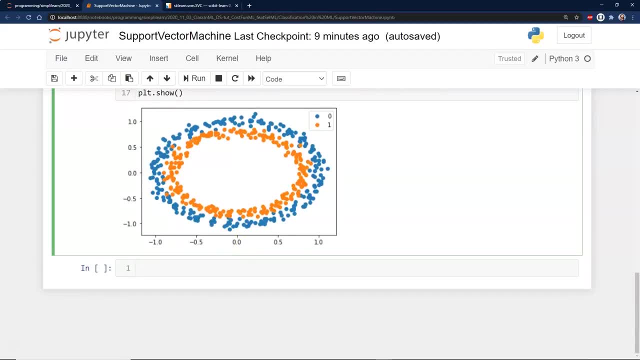 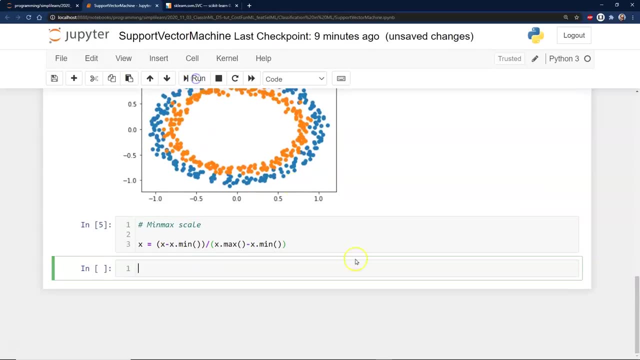 points are an xy coordinate plot on this. One of the things we might want to do on here is go ahead and find the min to max ratio setup in there, And we can even do- let's just do a print x so you can see what the data looks like. 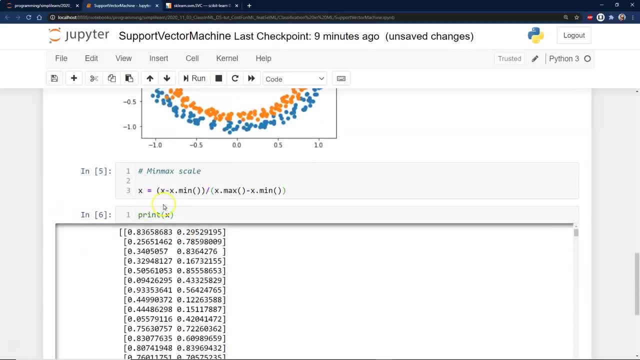 that we're producing on this. There we go. So x equals x minus x min. over x max minus x min. All we're doing is putting this between zero and one. Whatever this data is, we want a zero to one setup on here. And if you look at this: 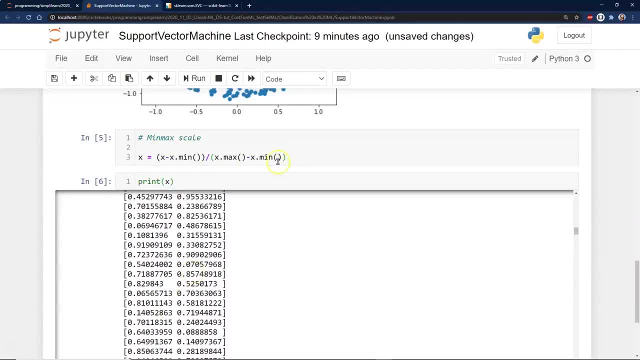 all our data is 0.8, 0.5.. That's what this particular line is doing. That's a pretty common thing to do in processing data, especially in neural networks. Neural networks don't like big numbers. They create huge biases. 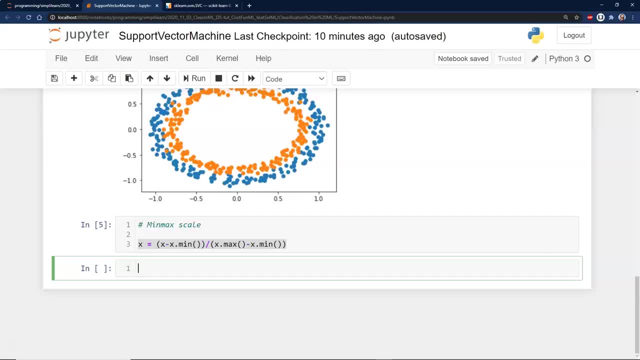 and cause all kinds of problems. And that's true in a lot of our models, Some of the models. it doesn't really matter, But when you're doing enough of these, you just start doing them, You just start putting everything between zero and one. 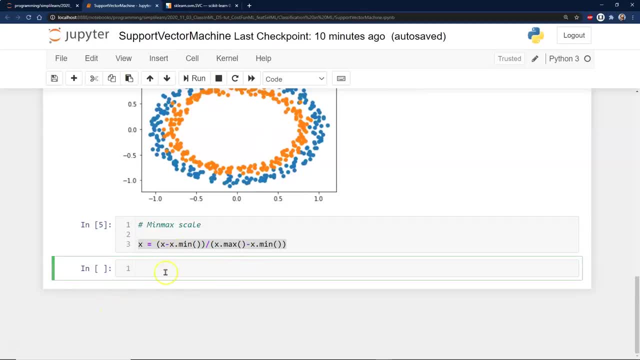 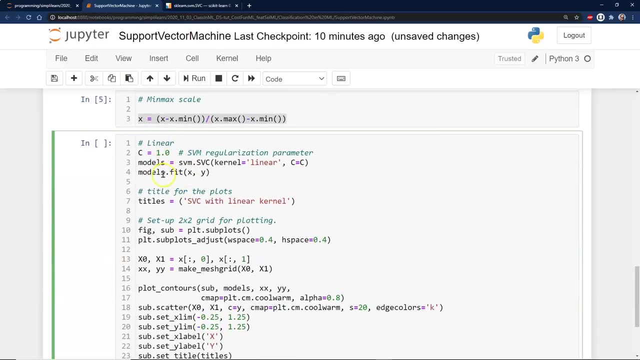 There's even some algorithms to do that in the sklearn, although, as you can see, it's pretty easy to do it here. So let's go ahead and jump into the next thing, which is a linear kind of setup. C equals 1.0.. This is the SVM. 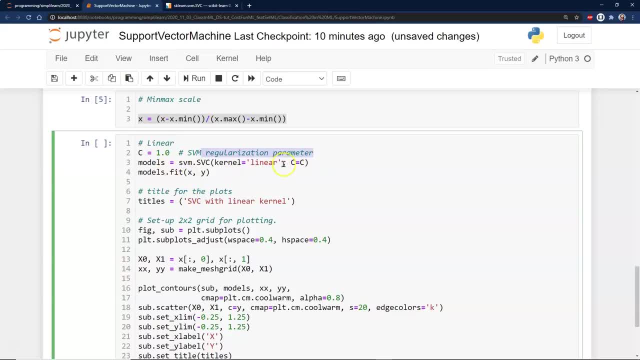 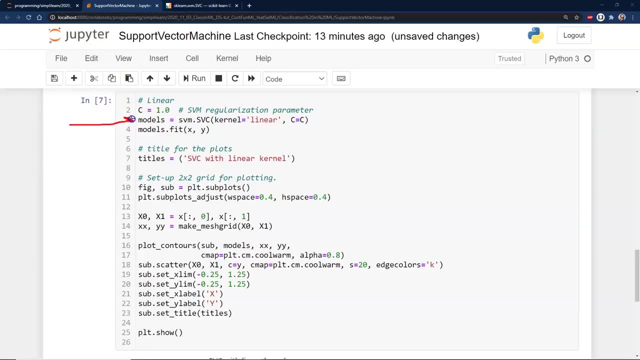 regularization parameter. we're going to use Models. here's our SVM. Let's go ahead and scroll up just a notch. There we go. So here we are with our model. We're going to create the setup with the SVM. SVC Kernel is linear. 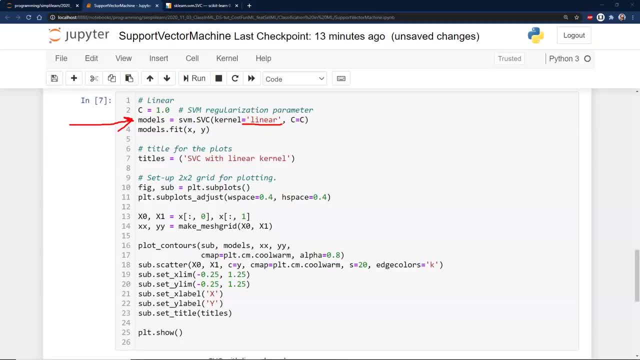 And we'll come back to that because that's an important setup in there as far as what our kernel is, And you'll see why that's so important here in a minute, Because we're going to look at a couple of these, And so this one. 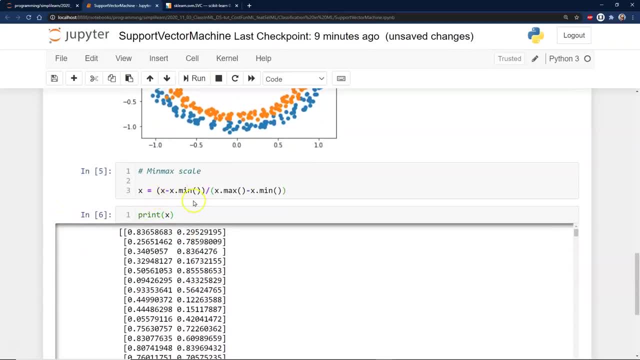 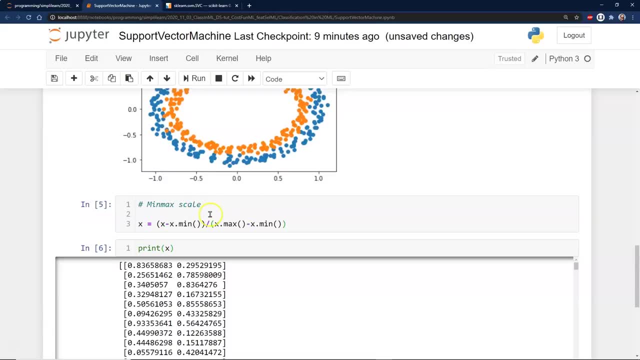 There we go. So x equals x minus x min over x max minus x min. All we're doing is Putting this between zero and one. Whatever this data is, we want a zero to one set up on here And if you look at this, all our data is 0.8, 0.5.. 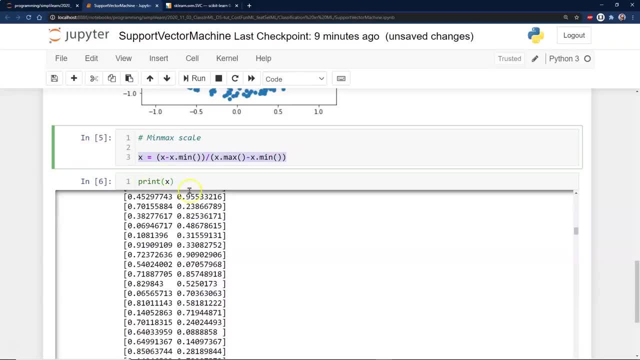 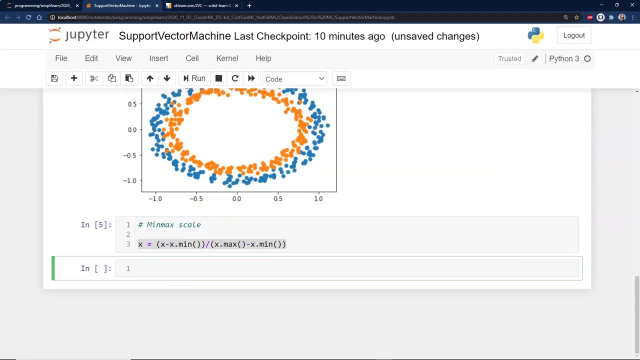 That's what this particular line is doing. That's a pretty common thing to do in processing data, especially in neural networks. Neural networks don't like big numbers. They create huge biases and cause all kinds of problems, And that's true in a lot of our models. 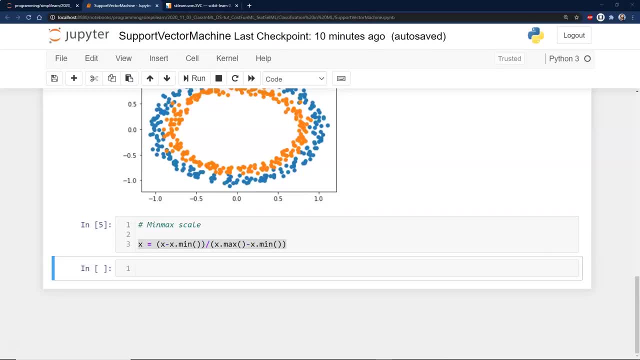 Some of the models. it doesn't really matter, But when you're doing enough of these, you just start doing them. You just start putting everything between zero and one. There's even some algorithms to do that in the SK learn. Although it's pretty as you can see, it's pretty easy to do it here. 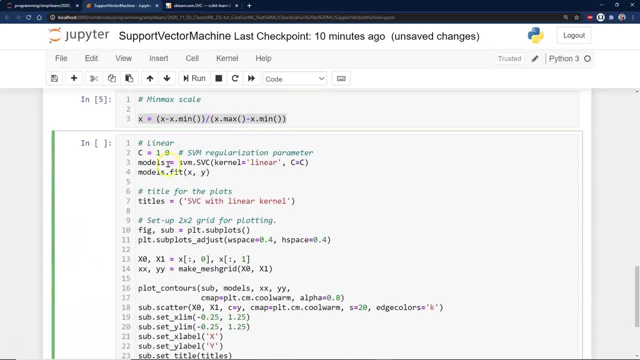 So let's go ahead and jump into the next thing, which is a linear kind of set up. C equals 1.0.. This is the SVM regularization parameter. we're going to use Models. Here's our SVM, and this one scroll up just a notch. 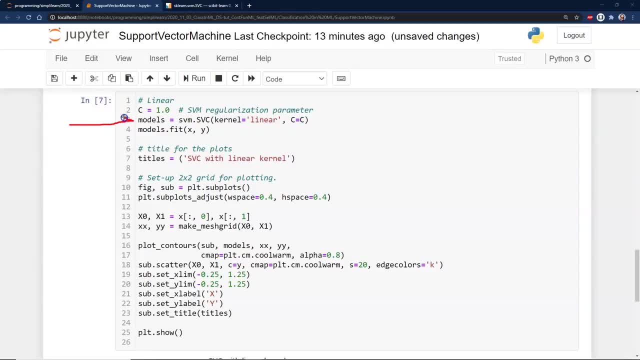 There we go. So here we are with our model We're going to create. the setup with the SVC kernel is linear and we'll come back to that because that's an important setup in there as far as what our kernel is, And you'll see why that's so important here in a minute because we're going to 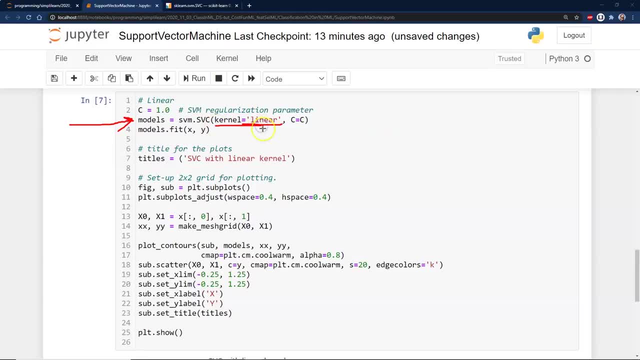 look at a couple of these, And so this one is: we're actually going to be changing how that processes it. And then our C, here's our 1.0, and then the rest of this is plotting. We're just adding titles, making the contours, so it's a pretty graph. 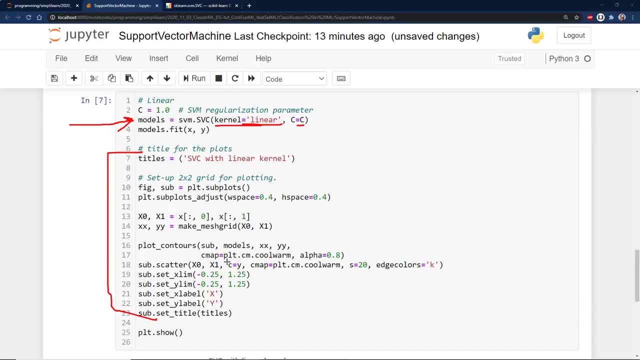 You can actually spend. this would be a whole class just to do all the cool things you can do with scatter plots and regular plots and colors like that. In this case, we're going to create a graph with a nice white line down the middle so that you can see what's going on here. 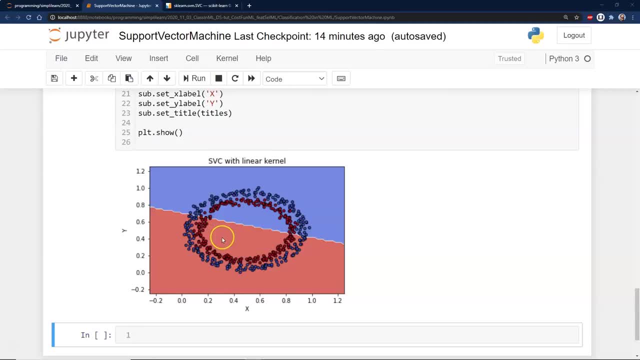 And when we do this, you can see that, as it is a split, the data, the linear- did just that: it drew a line through the data and it says this is supposed to be blue and this is supposed to be red, and it doesn't really fit very well. 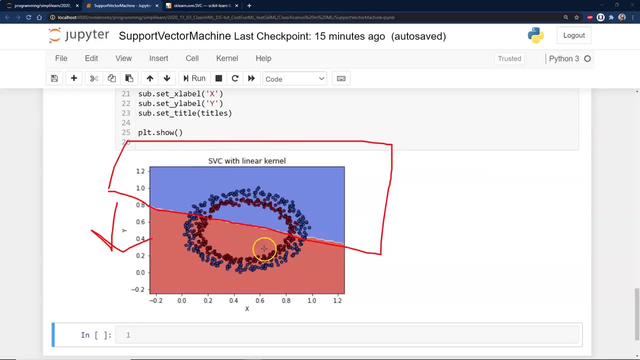 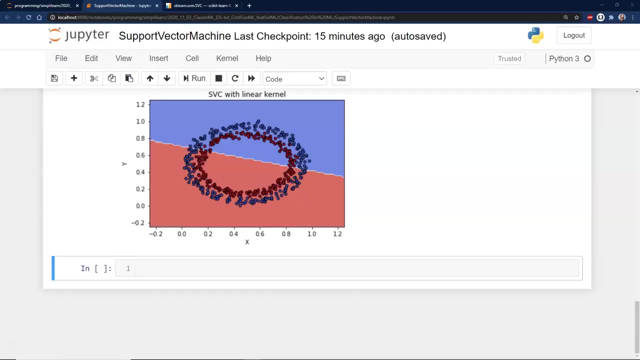 That's because we used a linear division of the data and it's not very linear data. It's anything but linear. So if you look at that, it's like, well, OK, that didn't work. What's the next option? Well, there's a lot of choices in here. 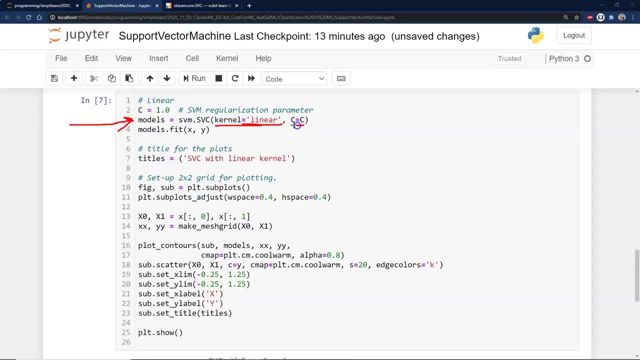 is we're actually going to be changing how that processes it. And then our C, here's our 1.0.. And then the rest of this is plotting. We're just adding titles, making the contours. so it's a pretty graph. 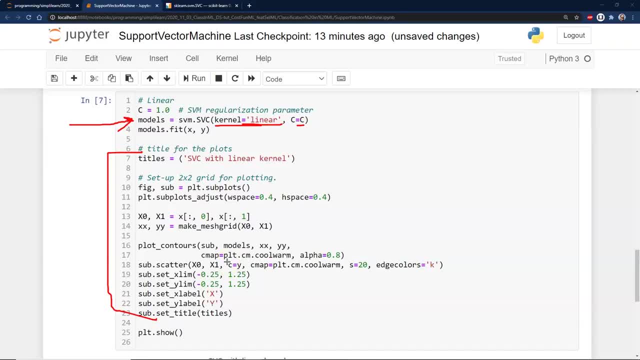 You can actually spend. this would be a whole class just to do all the cool things you can do with scatter plots and regular plots and colors and things like that. In this case, we're going to create a graph with a nice white line down the middle so that you 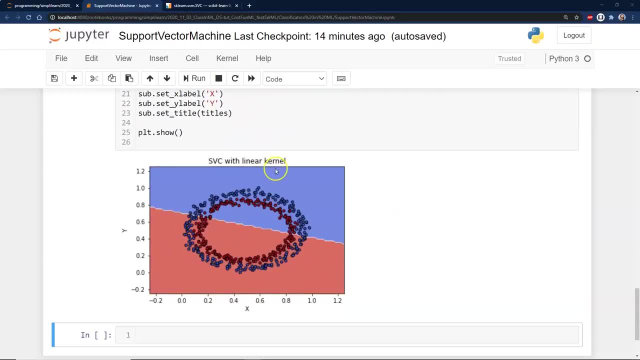 can see what's going on here And when we do this, you can see that as it split the data, the linear did just that. It drew a line through the data and it says this is supposed to be blue and this is supposed to be red, And it doesn't really fit. 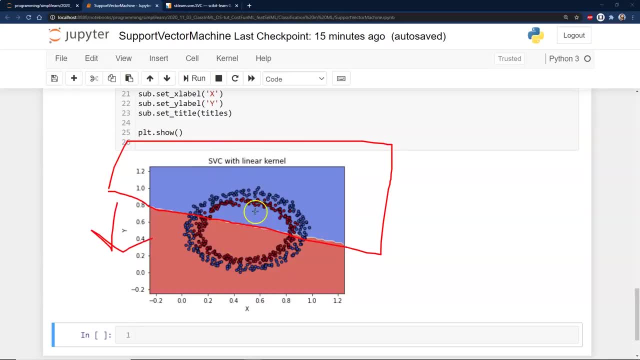 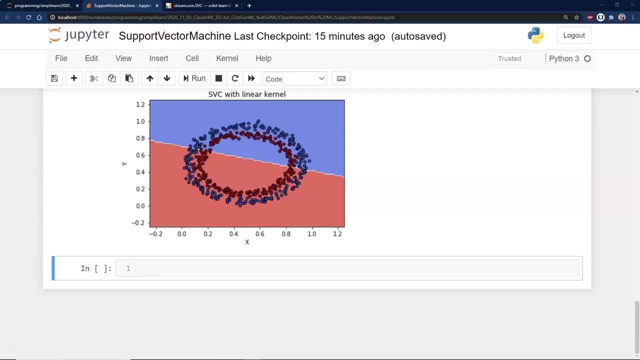 very well. That's because we used a linear division of the data and it's not very linear data, It's anything but linear. So when we look at that, it's like, well, okay, that didn't work. What's the next option? Well, there's a lot of choices. 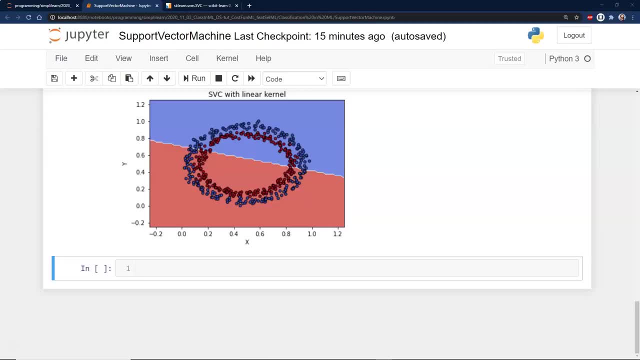 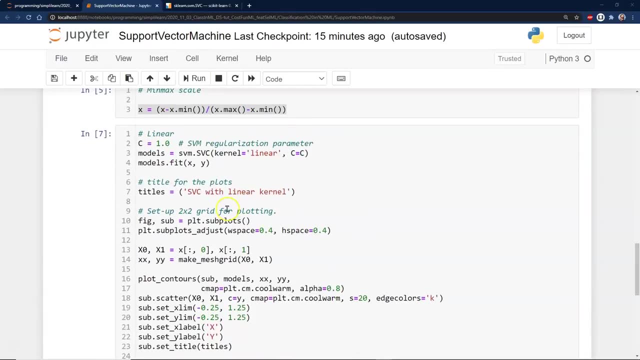 in here. One of them is just simply: we can change this from the kernel being linear to poly, And we'll just go back up here and use the same chart. Oops, here we go. So here we go: Linear kernel- We'll change this to poly. 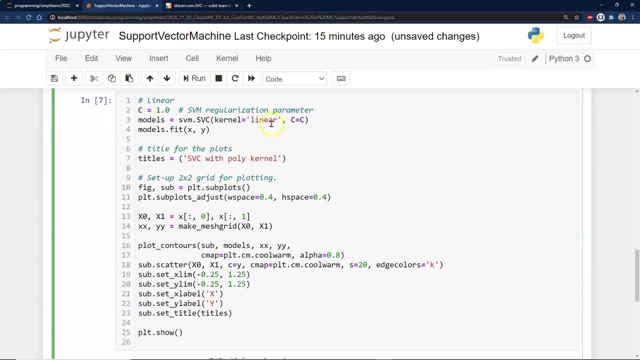 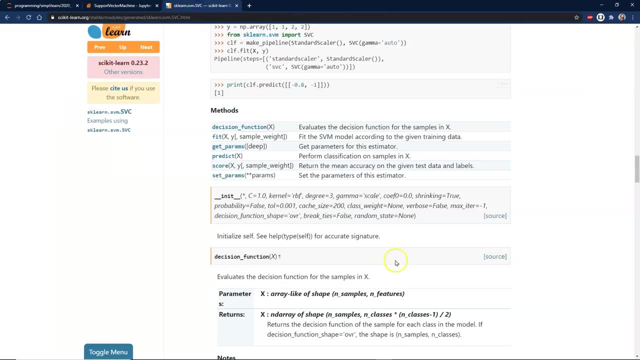 And then when we come in here and create our model- here's our model up here, linear- We can actually just go right in and change this to the poly model And, if you remember, when we go back over here to the SVC and let's scroll back up here- 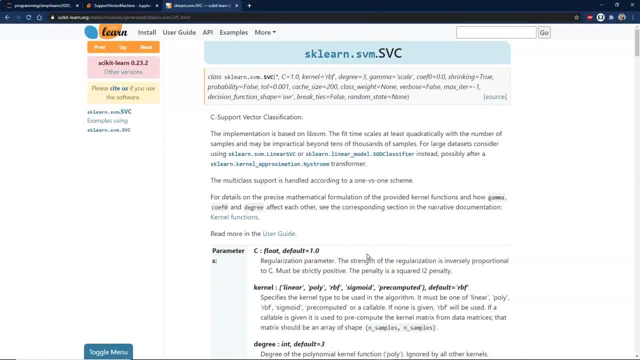 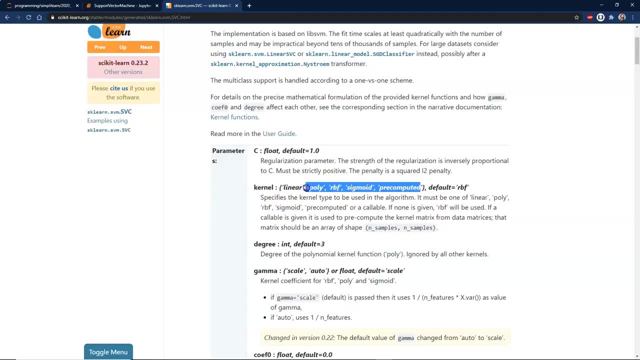 there's a lot of different options. Oops, even further. Okay, So we come up here and we start talking about the kernel. Here's the kernel. There's linear, there's poly, RBF, sigmoid, pre-computed. There's a lot of different. 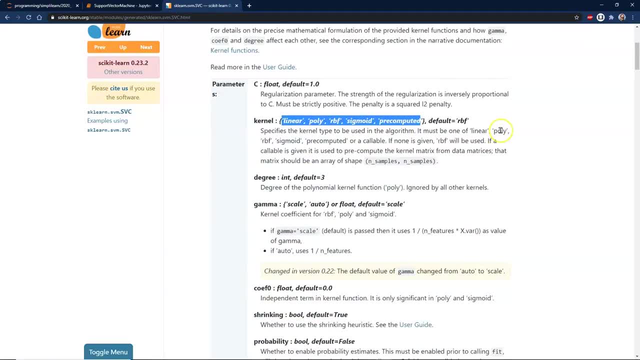 ways to do this setup And their actual default is RBF. Very important to note that. So when you're running these models, understanding which parameter really has a huge effect on what's going on. In this particular one, with the SVM, the kernel is so important. 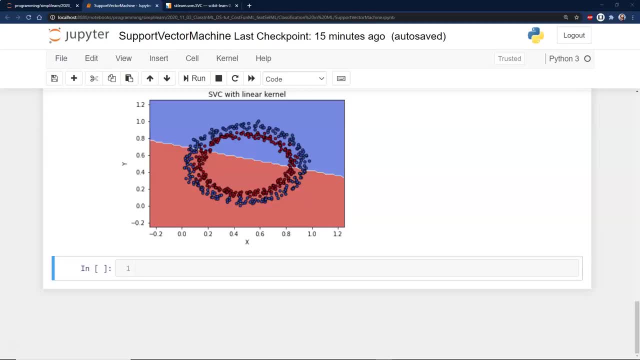 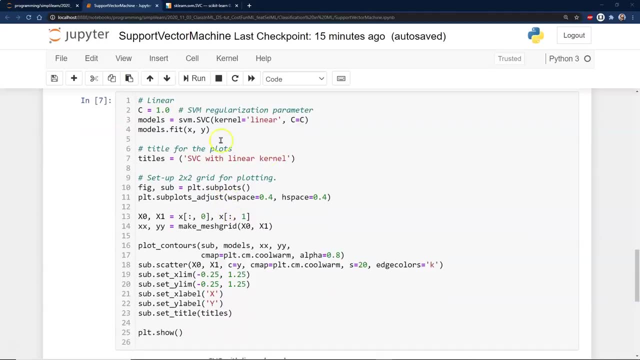 One of them is just simply, we can change this from the kernel being linear to poly, And we'll just go back up here and use the same chart Here we go. So here we go: Linear kernel will change this to poly, And then when we come in here and create our model, here's our model, up here, linear. 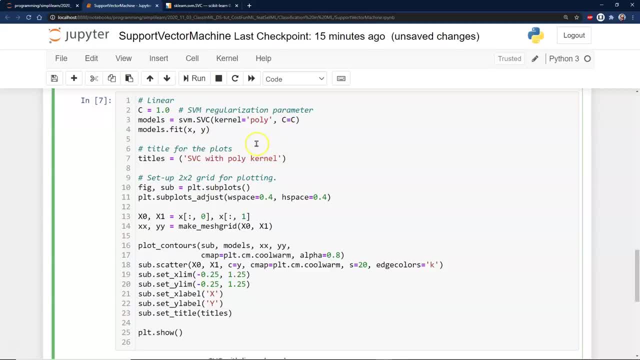 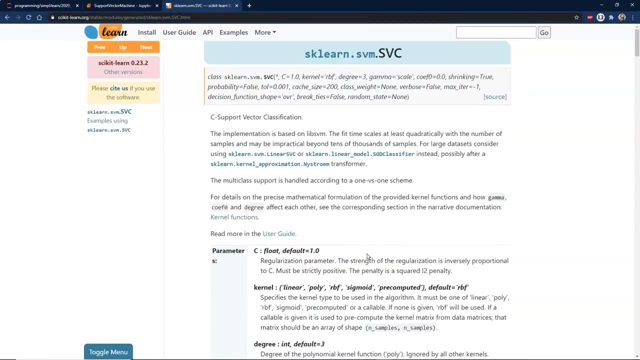 We can actually just go right in and change this to the poly model And, if you remember, we go back over to the SVC And let's scroll back up here. There's a lot of different options even further. OK, so we come up here, we start talking about the kernel. 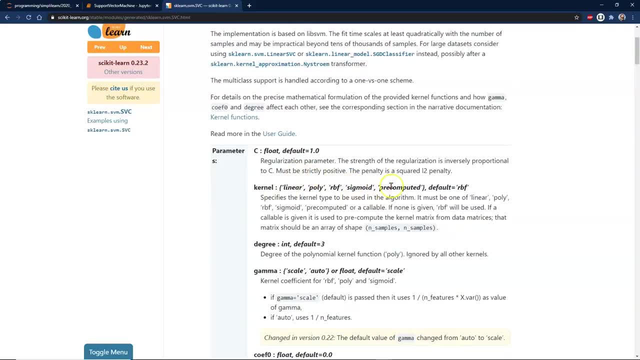 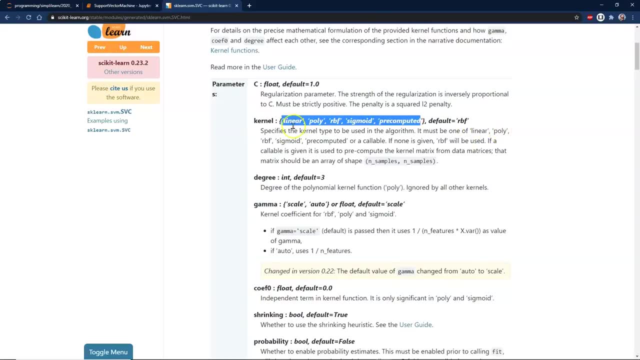 Here's the kernel. there's linear, there's poly, RBF, sigmoid, precomputed. There's a lot of different ways to do this setup and their actual default is RBF. Very important to note that. So, when you're running these models, understanding which parameter is really has a huge effect on what's going on. in this particular one, with the SVM. 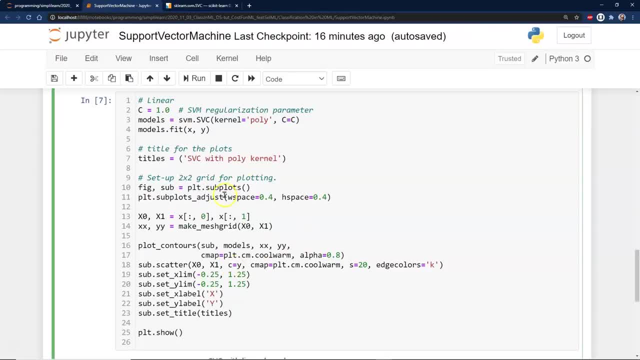 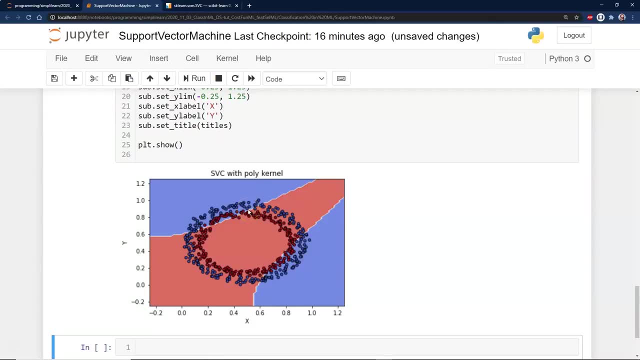 The kernel is so important. you really need to know that. And we switched our kernel to poly and when we run this you can see it's changed a little bit. We now have a quite an interesting looking diagram And you can see on here. it now has these classifications, correct. 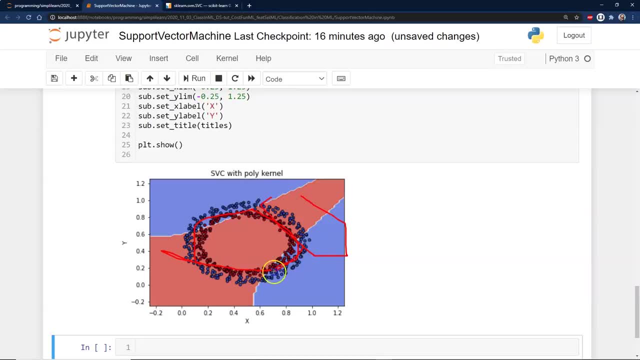 But it messes up in this blue up here and it messes up on this blue is correct and this blue is supposed to be red. You can see that it still isn't quite fitting on there, And so that is. we do a poly. 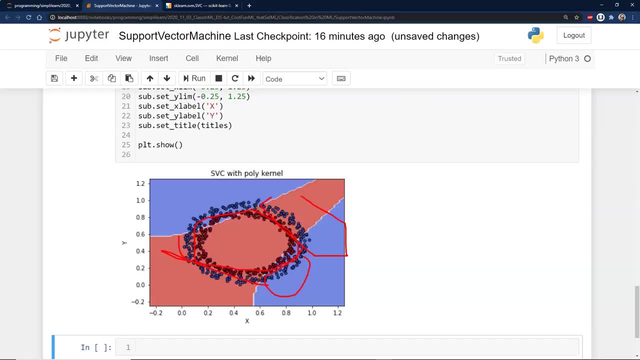 Fit, you can see if you have a split in data where there's a group in the middle, This one kind of data- and the groups on the outside are different. The poly fit or the poly kernel is what's going to be fit for that. 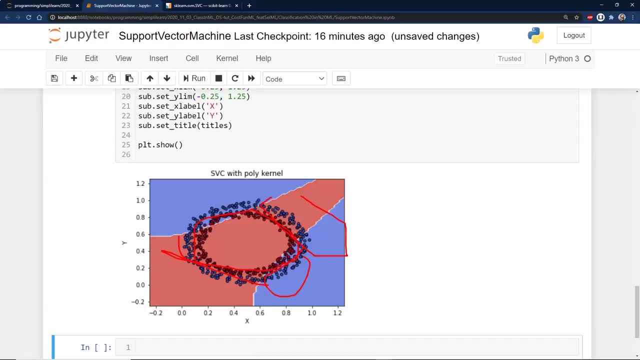 So if that doesn't work, then what are we going to use? Well, they have the RBF kernel and let's go ahead and take a look and see what the RBF looks like And let me go and turn there. we go, Turn my drawing off and the RBF kernel. 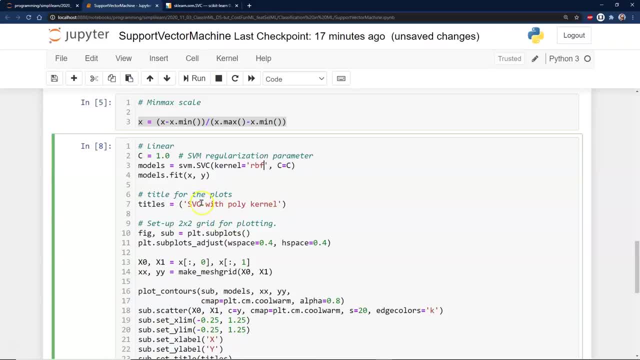 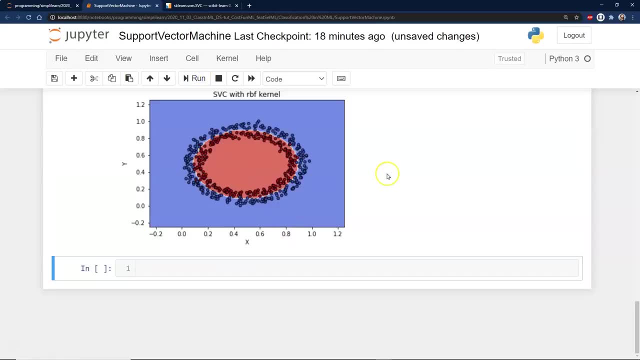 There we go, RBF, And, of course, for our title, it's always nice to have it match with the RBF kernel. Let me go ahead and run this and you can see that the RBF kernel does a really good job. It actually has divided the data up on here and this is the kind of what you expect. here was that ring. 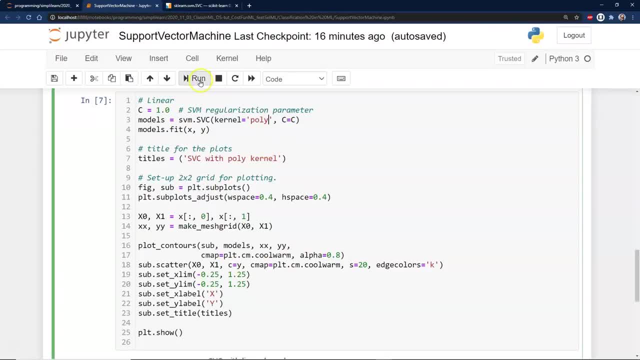 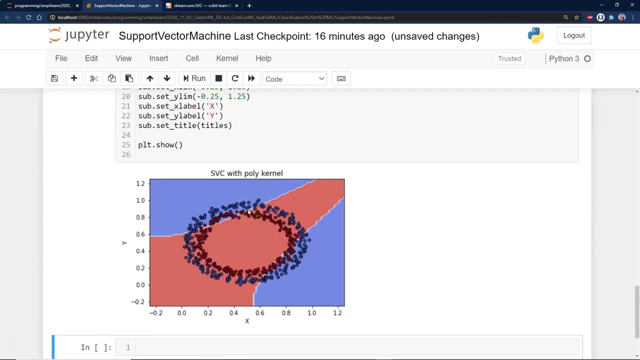 You really need to know that. And we switched our kernel to poly and when we run this you can see it's changed a little bit. We now have quite an interesting looking diagram and you can see on here. it now has these classifications correct, but it messes up in this. 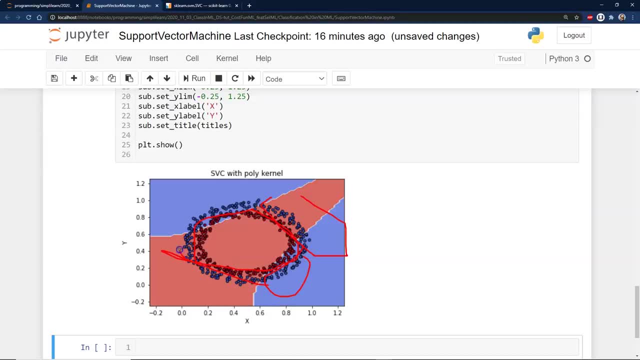 blue up here and it messes up on. this blue is correct and this blue is supposed to be red. You can see that it still isn't quite fitting on there, And so that is when we do a poly fit. you can see if you have a split in data. 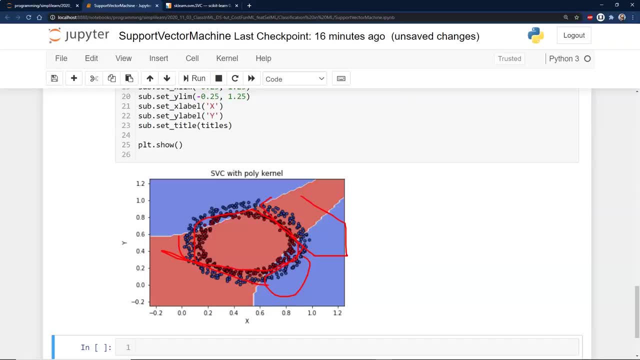 where there's a group in the middle- that's one kind of data- and the groups on the outside are different. the poly fit or the poly kernel is what's going to be fit for that. So if that doesn't work, then what are we going to use? 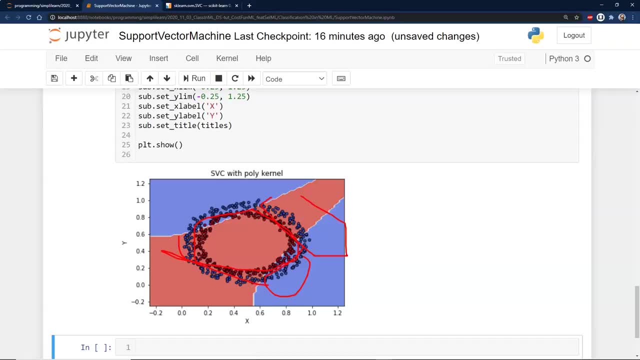 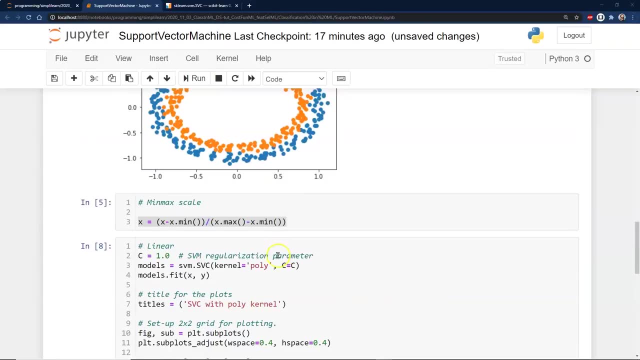 Well, they have the RBF kernel And let's go ahead and take a look and see what the RBF looks like, And let me go and turn my drawing off And the RBF kernel, oops, there we go- RBF. 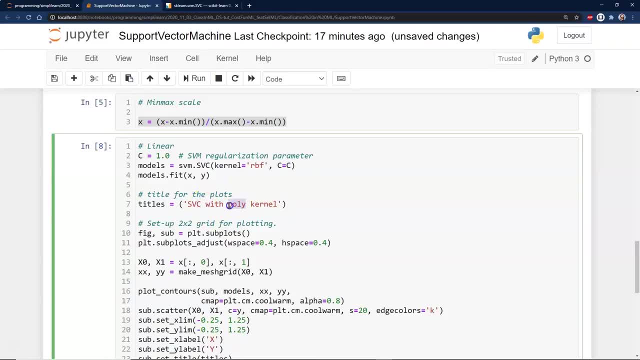 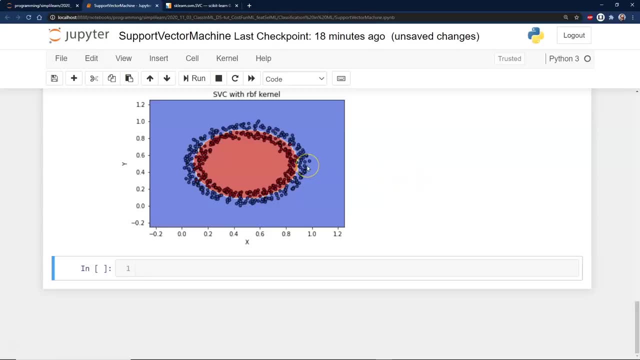 and then, of course, for our title. it's always nice to have it match with the RBF kernel. Let me go ahead and run this, And you can see that the RBF kernel does a really good job. It actually has divided the data up on here. 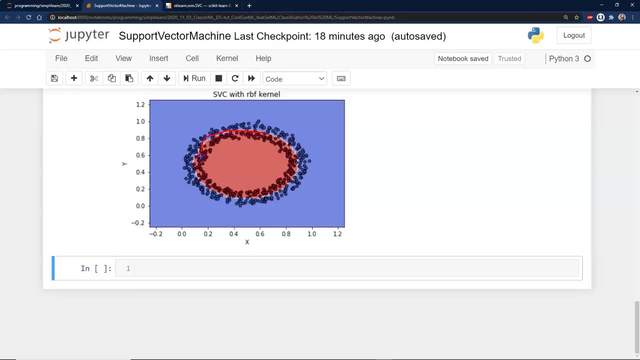 and this is the kind of what you expect. here was that ring. Here's our inner ring and an outer ring of data, So the RBF fits this data package quite nicely And that, when you're talking about SVM, it really is. 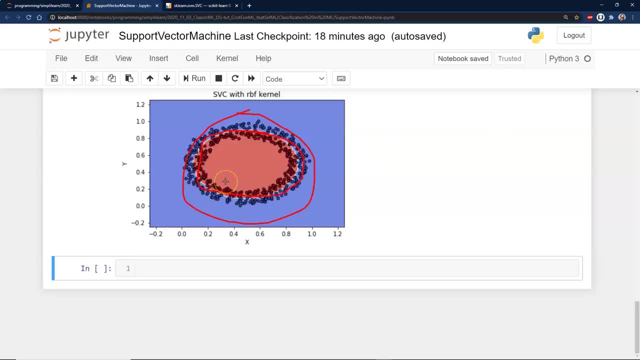 powerful in that it has this kind of sorting feature to it in its algorithms. This is something that is really hard to get the SK means to do or the K-means setup, And so when you start looking at these different machine learning algorithms, 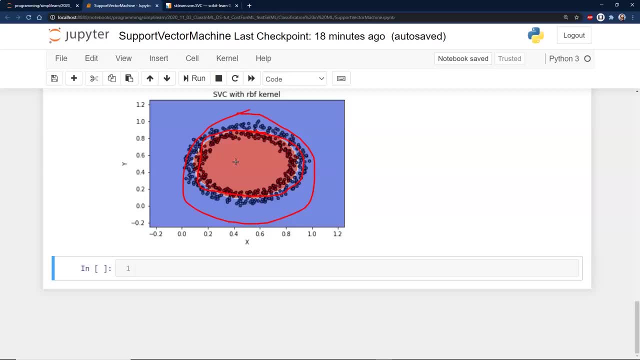 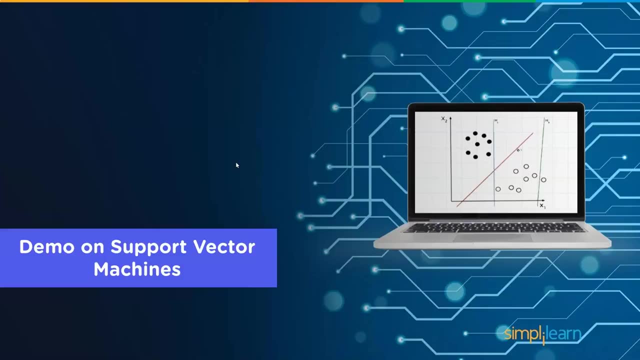 understanding your data and how it's grouped is really important. It makes a huge difference as far as what you're computing and what you're doing with it. So that was a demo on the support vector. Certainly you could have done continued on that and done like a confusion. 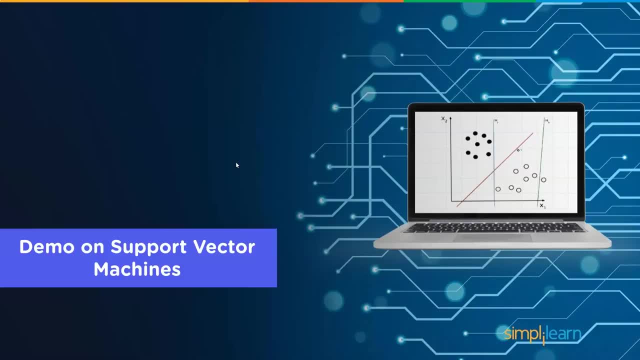 matrix and all that kind of fun stuff to see how good it was and split the data up to see how it vectorizes. The visual on that is so important. It makes a big difference just to see what it looks like and that giant donut and why it does. 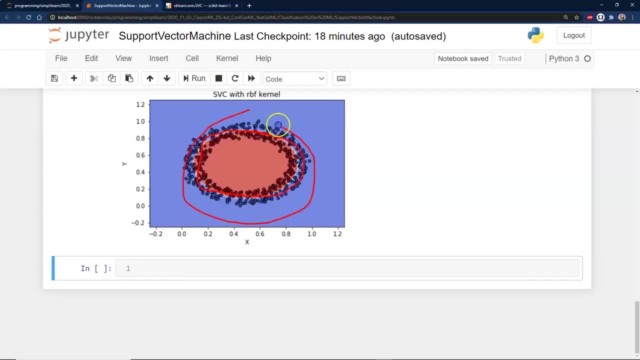 Here's our inner ring and an outer ring of data, So the RBF fits this data package quite nicely and that we're talking about SVM. It really is powerful in that it has this sorting feature to it in its algorithms. This is something that is really hard to get. the SK means to do, or the K means set up. 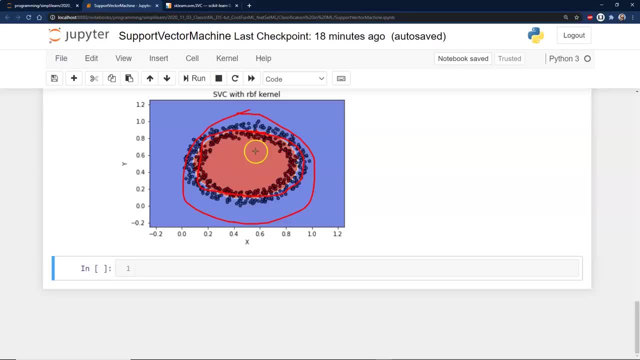 And so when you start looking at these different machine learning algorithms, understanding your data and how it's grouped is really important. It makes a huge difference as far as what you're computing and what you're doing with it. So that was a demo on the support vector. 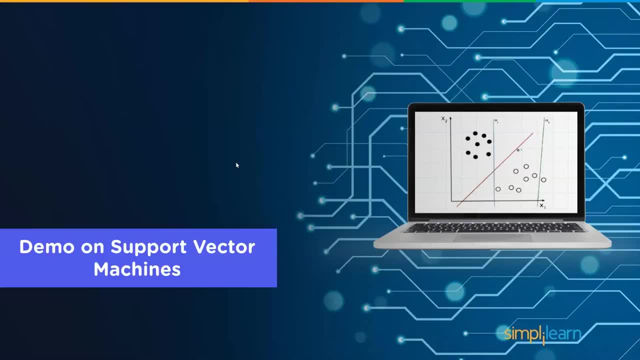 Certainly you could have done, continued on that and done like a confusion matrix and all that kind of fun stuff to see how good it was, and split the data up to see how it vectorizes the visual. and that's so important. It makes a big difference just to see what it looks like and that giant donut. 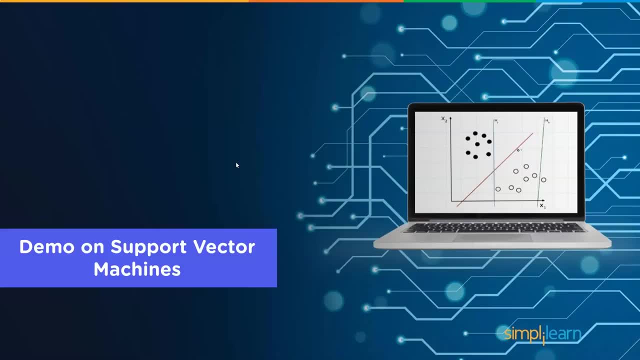 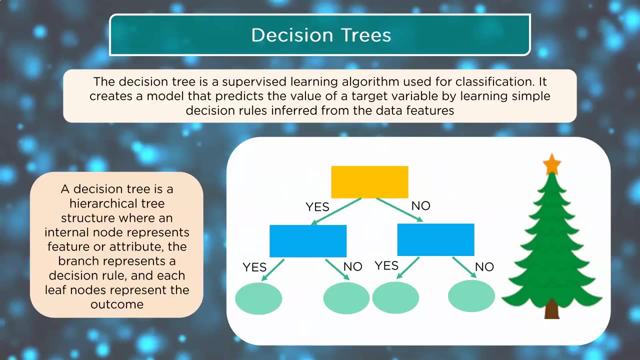 and why it does circle so well, or your poly version or your linear version. So we've looked at some very numerical kind of setups where there's a lot of math involved- Euclidean geometry, that kind of thing. a totally different machine learning algorithm for approaching this is the decision trees. 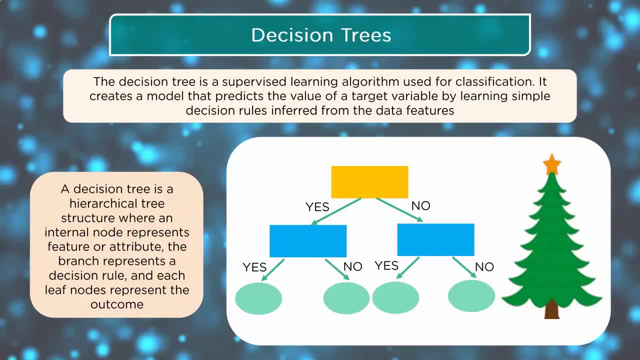 And there's also forest To go with. the decision trees are based on multiple trees combined. The decision tree is a supervised learning algorithm used for classification. It creates a model that predicts the value of a target variable by learning simple decision rules inferred from the data. 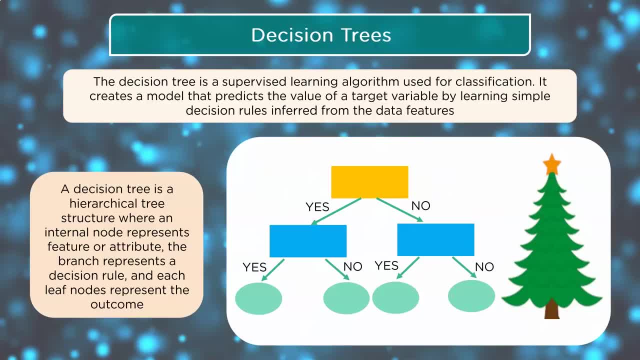 features. A decision tree is a hierarchical tree structure where an internal node represents features or tribute, The branch represents a decision rule and each leaf node represents the outcome. And you can see here where they have the first one, Yes or no- And then you go either left or right, and so forth. 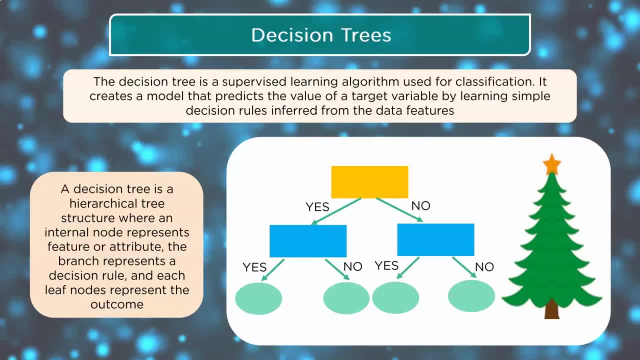 One of the coolest things about decision trees is- and I'll see people actually run a decision tree, even though their final model is different- because the decision tree allows you to see what's going on. you can actually look at it and say: why did you go right or left? What was the choice? 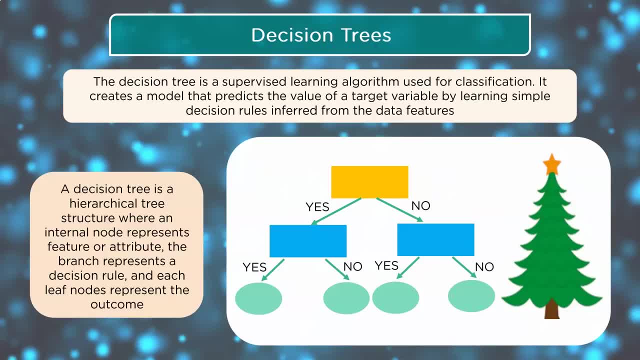 Where's that break? And that is really nice if you're trying to share that information with somebody else as to why, When you start getting into the why this is happening, decision trees are very powerful, So the topmost node of a decision tree is known as the root node. 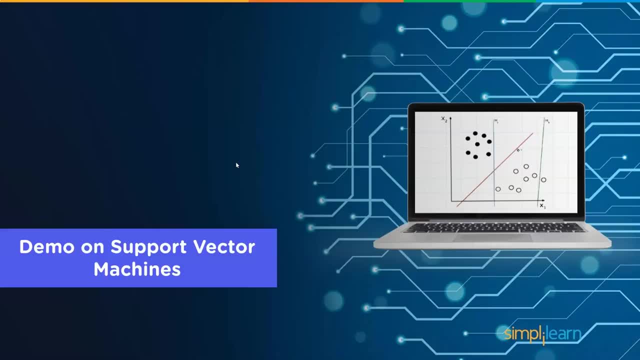 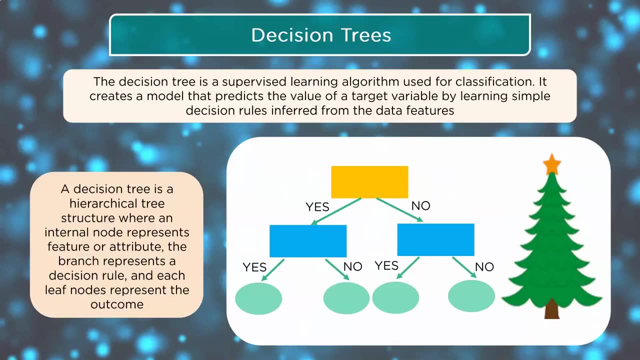 circle. so well, or your poly version, or your linear version. So we've looked at some very numerical kind of setups where there's a lot of math involved: Euclidean geometry, that kind of thing. A totally different machine learning algorithm for approaching this is the. 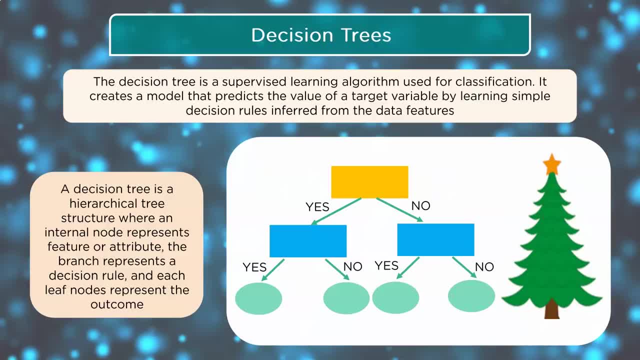 decision trees And there's also forests that go with the decision trees. They're based on multiple trees combined. The decision tree is a supervised learning algorithm used for classification. It creates a model that predicts the value of a target variable by learning simple decision rules. 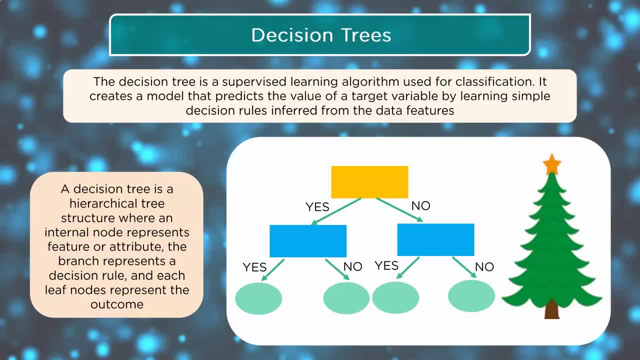 inferred from the data features. A decision tree is a hierarchical tree structure where an internal node represents features or attribute, The branch represents a decision rule and each leaf node represents the outcome. And you can see here where they have the first one, yes or no, and then you go either left or 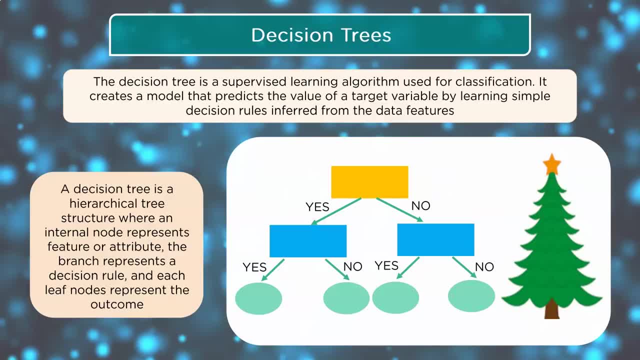 right and so forth. One of the coolest things about decision trees is- and I'll see people actually run a decision tree, even though their final model is different- Because a decision tree allows you to see what's going on. You can actually look at it and say: why did you go? 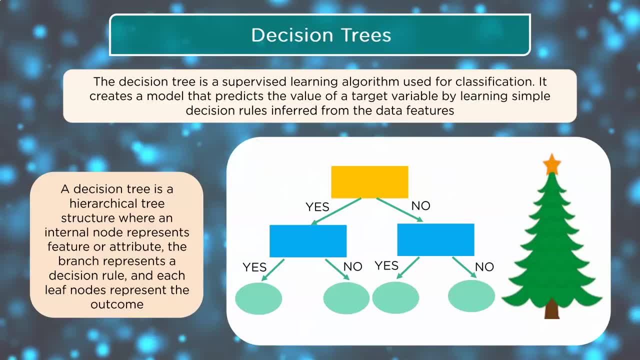 right or left? What was the choice? Where's that break? And that is really nice if you're trying to share that information with somebody else as to why, When you start getting into the why this is happening, decision trees are very powerful. So the topmost node of a 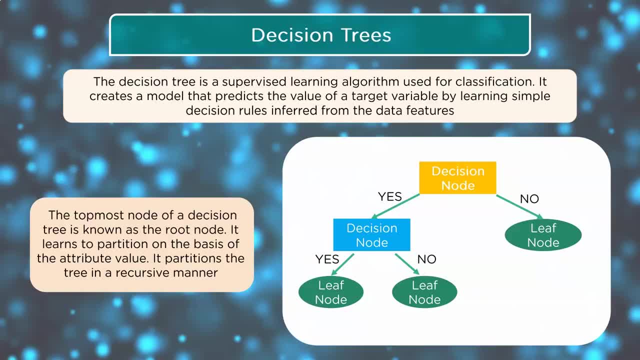 decision tree is known as the root node. It learns to partition on the basis of the attribute value. It partitions the tree in a recursive manner, So you have a decision node. If you get yes, you go down to the next node. That's a. 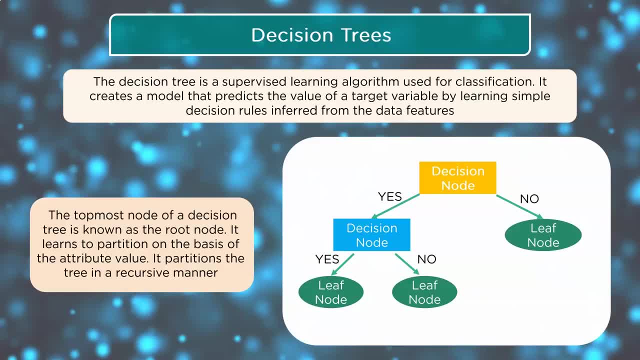 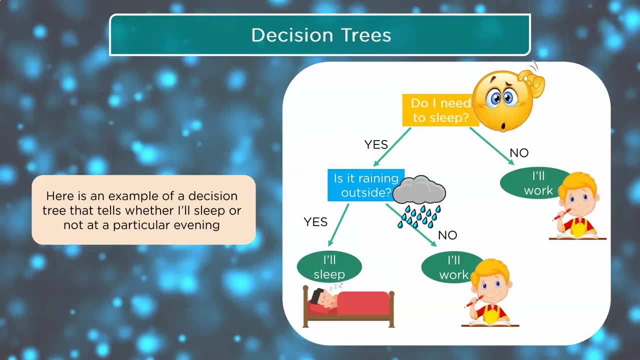 decision node And either yes, you go to. if it ends on a leaf node, then you know your answer, which is yes or no. So there's your end classification set up on there. Here's an example of a decision tree that tells whether I'll sleep or not. 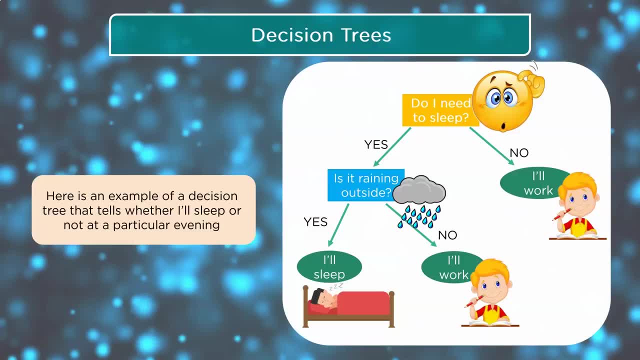 at a particular evening. Mine would be, depending on whether I have the news on or not. Do I need to sleep? No, Okay, I'll work. Yes. is it raining outside? Yes, I'll sleep. No, I'll work, So I guess. 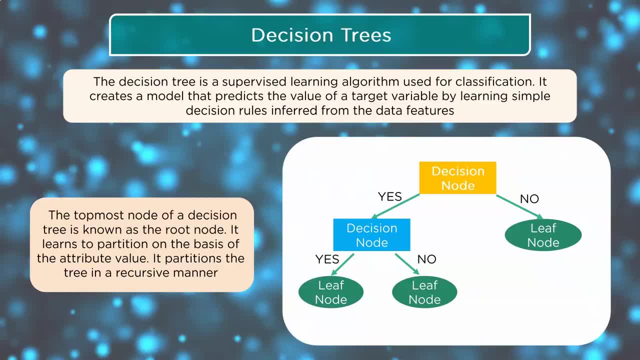 It learns to partition on the basis of the attribute value. It partitions the tree in a recursive manner. So you have your decision node. If you get yes, you go down to the next note. That's a decision note. And either yes, you go to if it ends on a leaf node. 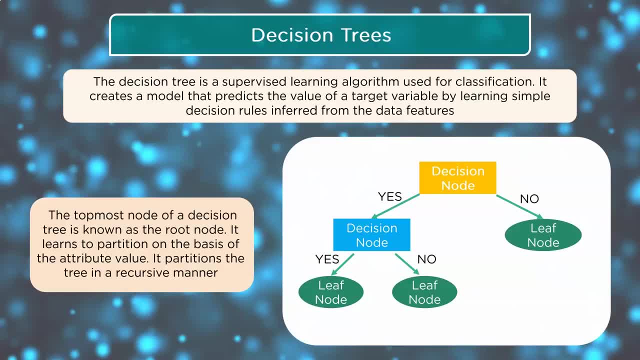 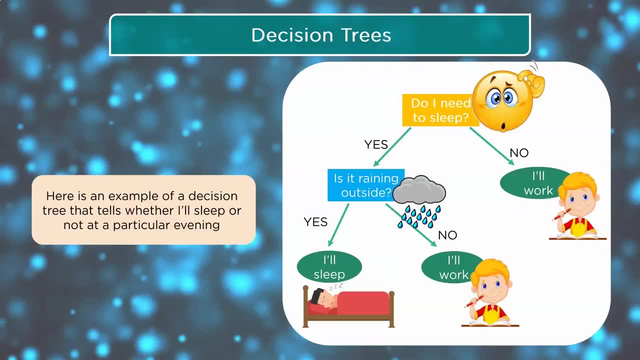 then you know your answer, which is yes or no. So there's your. there's your end classification set up on there. Here's an example of a decision tree that tells whether I'll sleep or not at a particular evening. Mine would be depending on whether I have the news on or not. 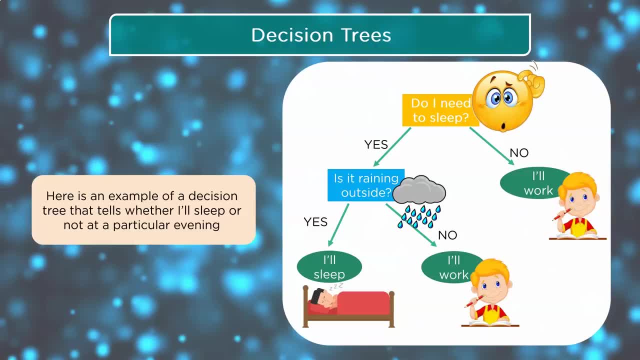 Do I need to sleep? No, OK, I'll work, Yes. Is it raining outside? Yes, I'll sleep. No, I'll work. So I guess if it's not raining outside, it's harder to fall asleep where you have that nice rain coming in. 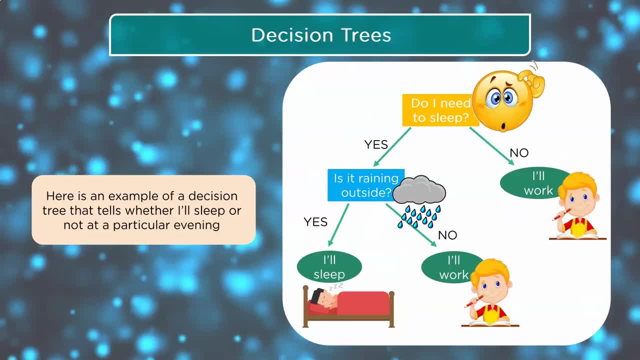 And again, this is really cool about a decision tree is I can actually look at it and go, oh, I like to sleep when it rains outside. So you're looking at all the data. You can say, oh, this is where the switch comes in. 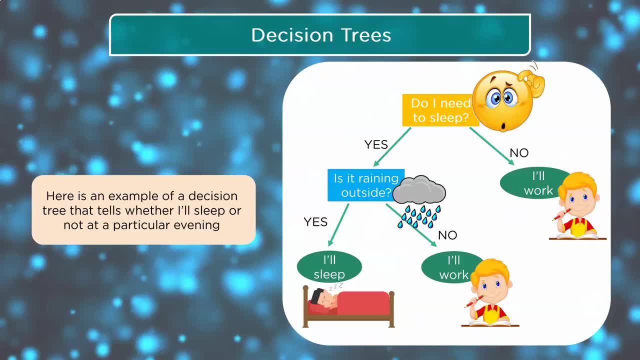 When it rains outside, I'll sleep really good. If it's not raining, or if I don't need sleep, then I'm not going to sleep. I'm going to go work. So let's go ahead and take a look at that. 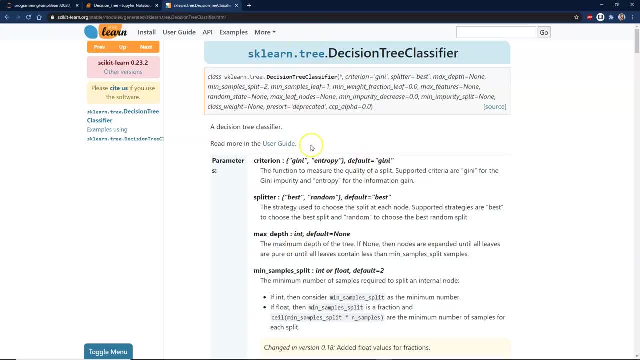 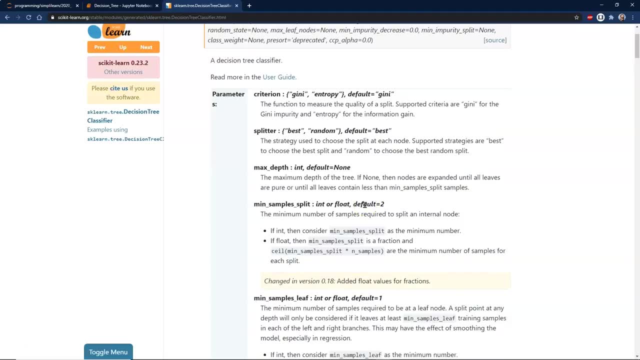 That looks like in the code, just like we did before We go ahead and open up the site kit set up just to say what the decision tree classifier has. you have your parameters, which we'll look a little bit more in depth at as we write the code, but it has different ways of splitting it. 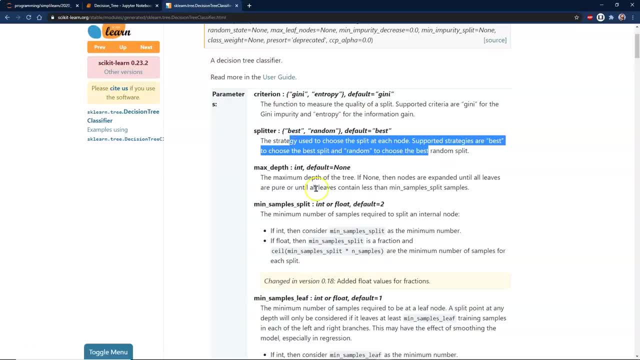 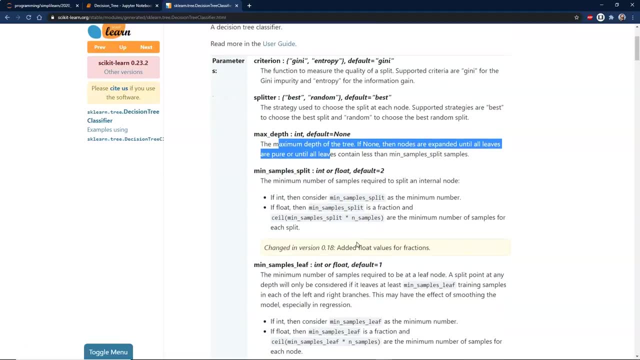 The strategy used to choose a split at each node. criterion: max depth. Remember the tree. How far down Do you want it? Do you want to take up the space of your whole computer with and map every piece of data? or the smaller that number is, the smaller the level of the tree is? 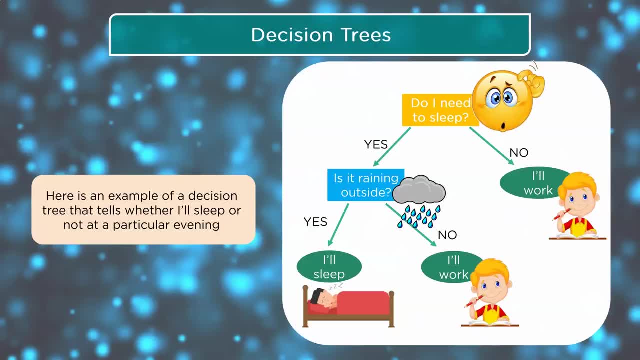 if it's not raining outside it's harder to fall asleep where you have that nice rain coming in. And again, this is really cool about a decision tree is I can actually look at it and go: oh, I like to sleep when it rains outside. 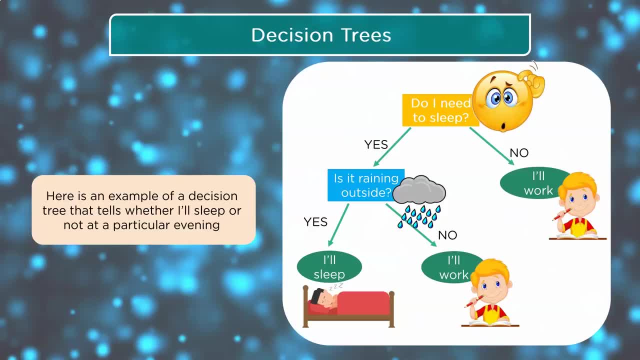 So when you're looking at all the data, you can say: oh, this is where the switch comes in. When it rains outside, I'll sleep really good. If it's not raining, or if I don't need sleep, then I'm not going to sleep, I'm going to go work. 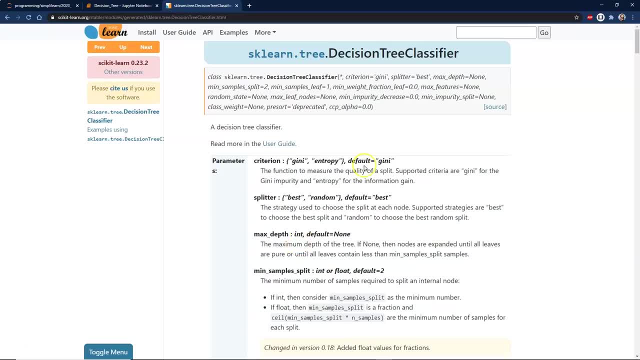 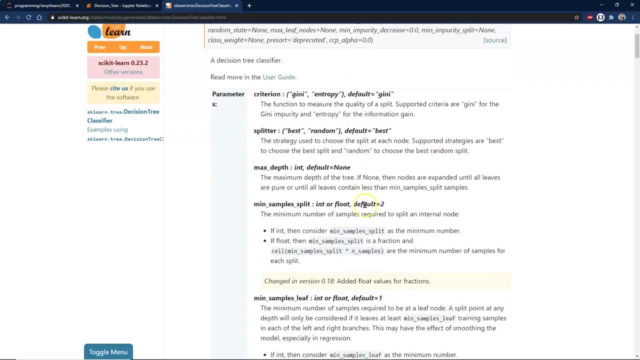 So let's go ahead and take a look at what that looks like in the code, Just like we did before we go ahead and open up the site kit set up, just to tell you what the decision tree classifier has. You have your parameters, which we'll look a little. 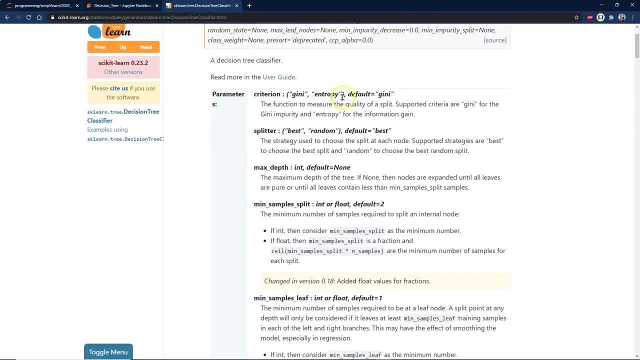 bit more in depth at as we write the code. It has different ways of splitting it. the strategy used to choose a split at each node. criterion: max depth: Remember the tree. how far down do you want it? Do you want it to take up the space of your whole? 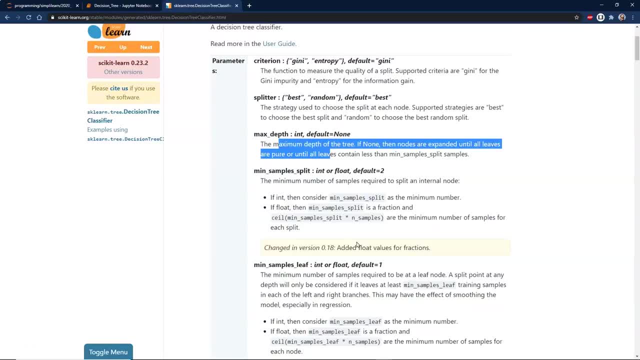 computer and map every piece of data, Or the smaller that number is, the smaller the level of the tree is and the less processing it takes. But it's also more general, so you're less likely to get as in-depth an answer. And then, of course, 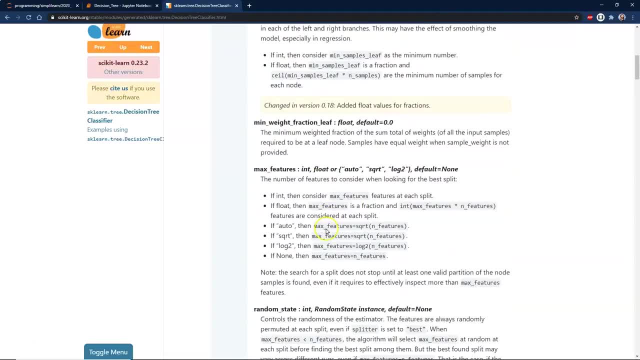 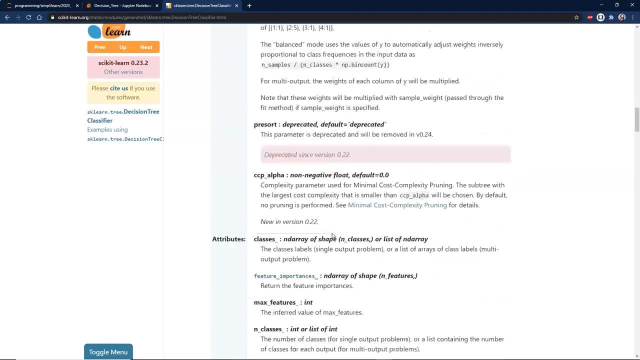 minimal samples you need for it to split samples for the leaves. There's a lot of things in here as far as how big the tree is and how to define it and when do you define it and how to weight it, And they have their different. 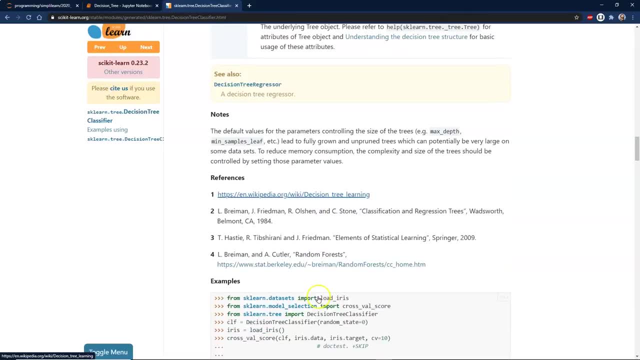 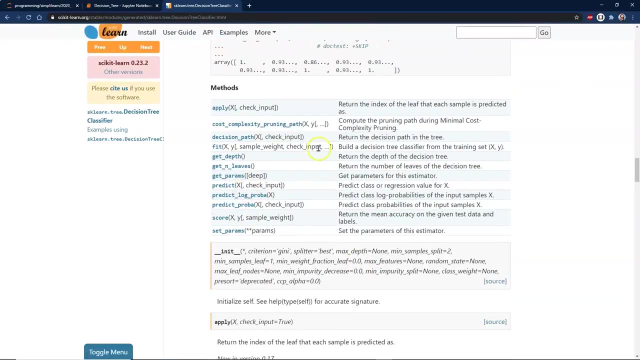 attributes which you can dig deeper into. That can be very important if you want to know the why of things. And then we go down here to our methods and you'll see, just like everything else, we have our fit method- very important- and our predict. 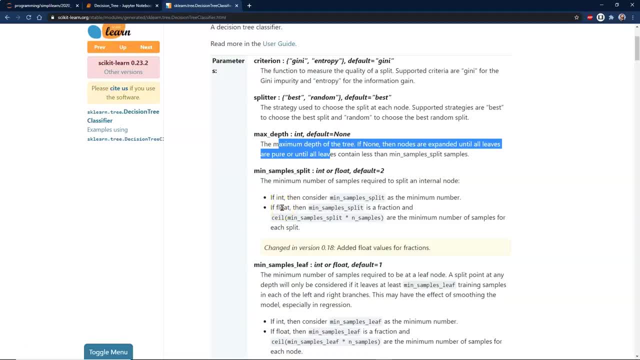 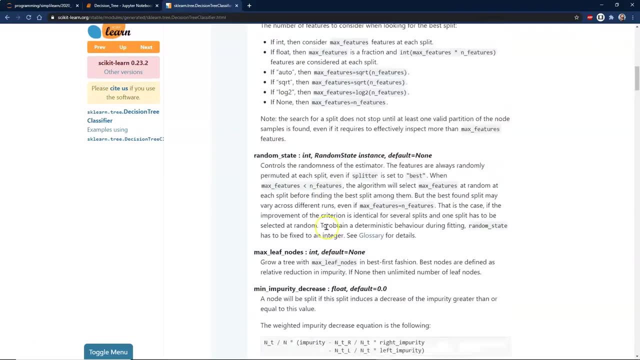 and the less processing it takes, but is also more general, So you're less likely to get as in depth an answer. And then, of course, minimal samples you need for to split samples for the leaves. There's a lot of things in here as far as what, how big the tree is and how 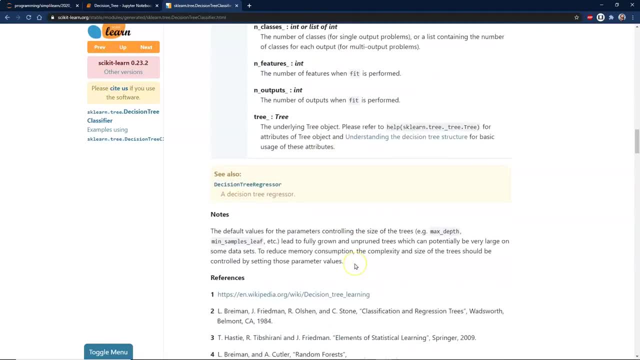 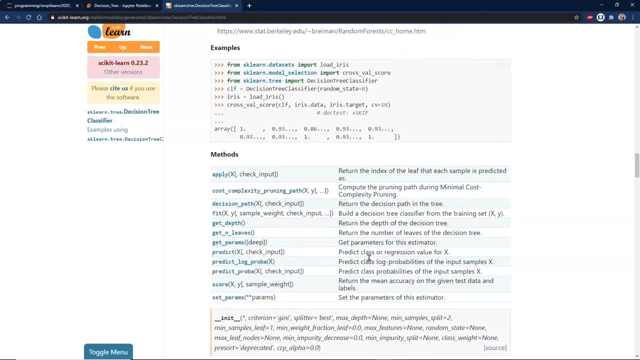 to define it and when do you define it and how to weight it, And they have their different attributes which you can dig deeper into. That can be very important if you want to know the why of things. And then we go down here to our methods and you'll see, just like everything else. 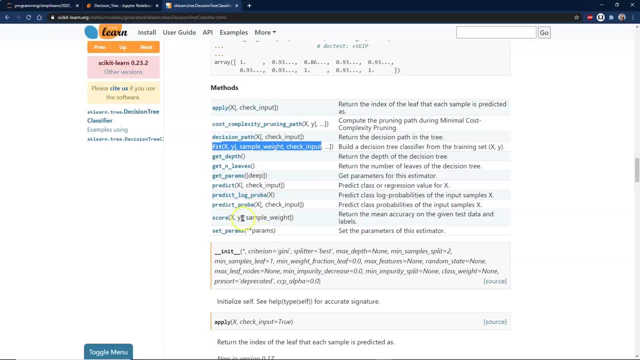 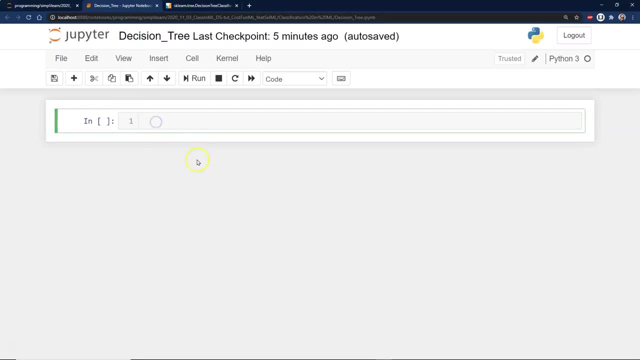 we have our fit method- very important- and our predict the two main things that we use. what is what we're going to predict our X to be equal to? We'll go ahead and go up here and start putting together the code We're going to import our numpy, our pandas. 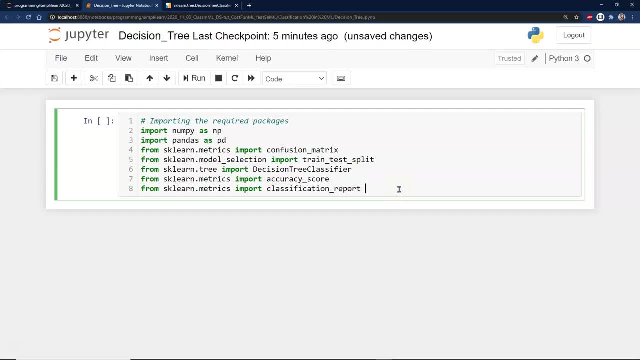 There's our confusion matrix, our train test split decision tree classifier. That's the big one that we're actually working with. That's the line right here where we're going to be. Oops, Decision tree. There it is. Decision tree classifier. 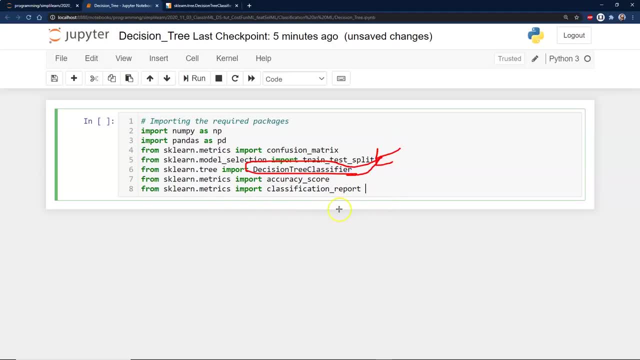 That's the one I was looking for And of course we want to know the accuracy and the classification report on here And we're going to do a little different than we did in the other examples, And there's a reason for this. 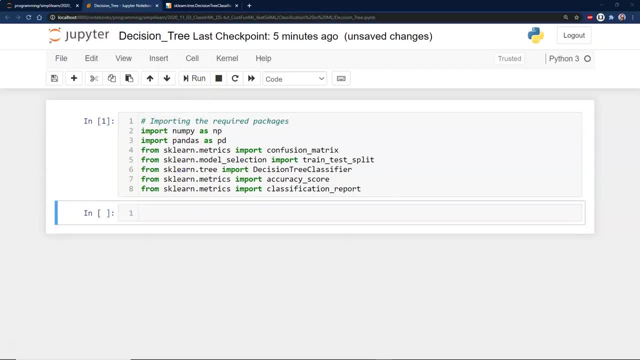 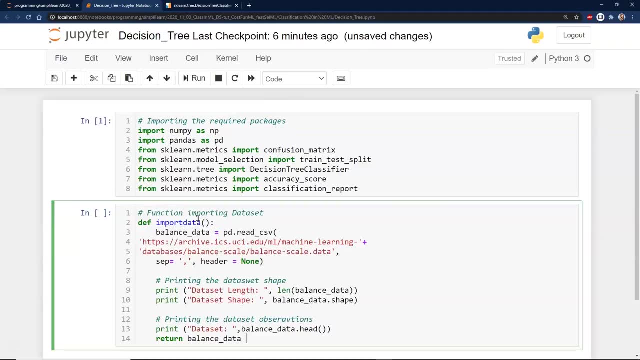 Let me go and run this and load this up here. We're going to go ahead and build things on functions, And this is when you start splitting up into a team. This is the kind of thing you start seeing a lot more, Both in teams and for yourself, because you might want to swap one data. 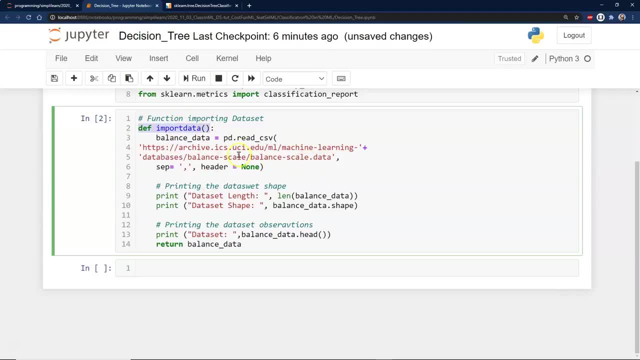 to test it on a different data depending on what's going on. So we're going to have our import data here, The data set, length, the balance and so forth. This just returns balance data. Let me just go ahead and print some curious as to what this looks like. 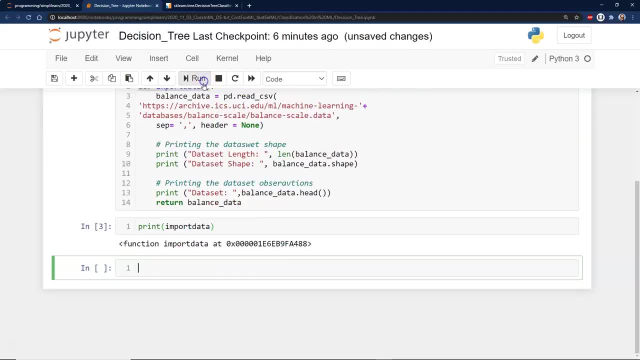 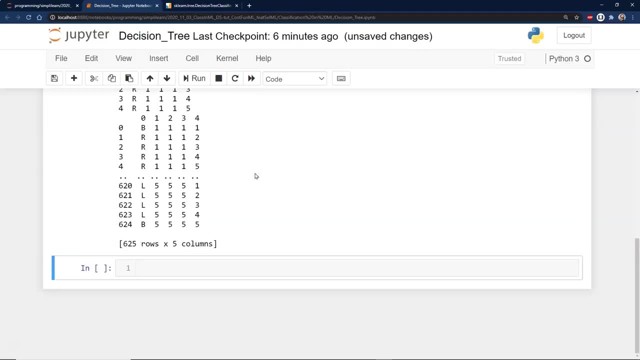 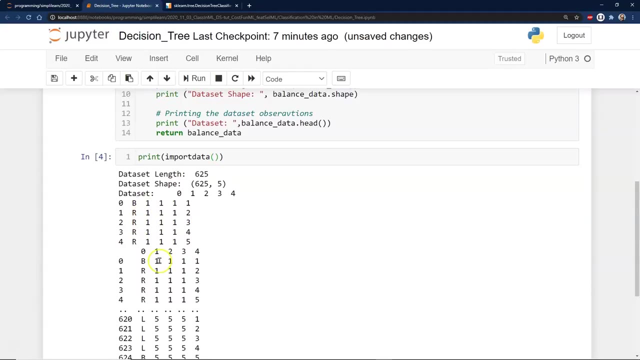 Import data and it's going to return the balance data. So if I run that, if we go ahead and print this out here and run that, you can see that we have a whole bunch of data that comes in there and some interesting set up on here has- let's see BRR. 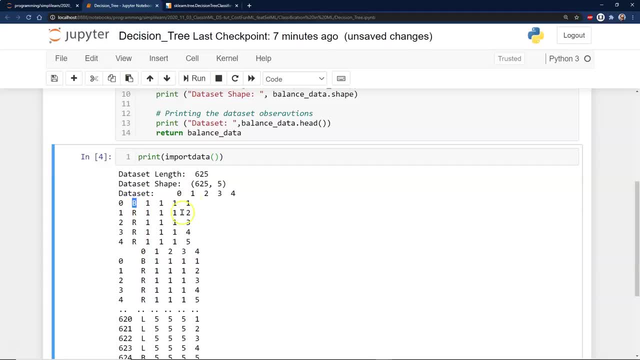 I'm not sure exactly what that represents on here: One one, one, one one two and so forth. So we have a different set of data here. The shape is five columns: one, two, three, four, five. 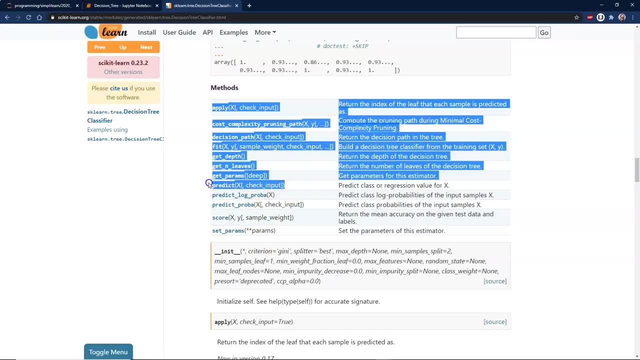 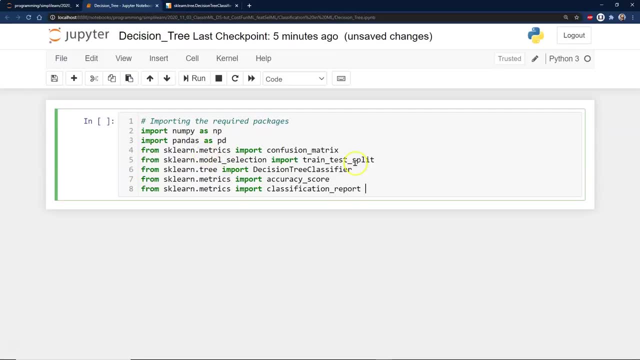 The two main things that we use. what we're going to predict our x to be equal to. We'll go ahead and go up here and start putting together the code. We're going to import our numpy, our pandas. there's our confusion. 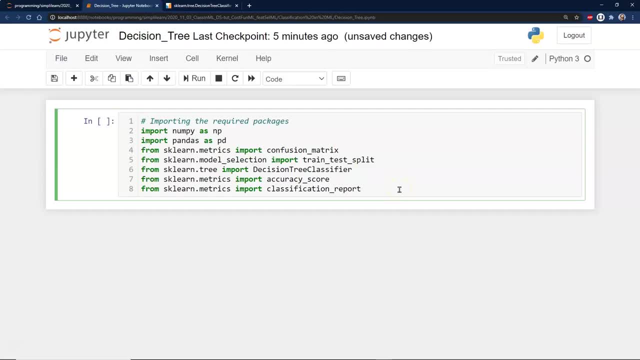 matrix, our train test split. decision tree classifier. that's the big one that we're actually working with. That's the line right here where we're going to be- oops, decision tree. there it is. decision tree classifier. that's the one I was looking for. 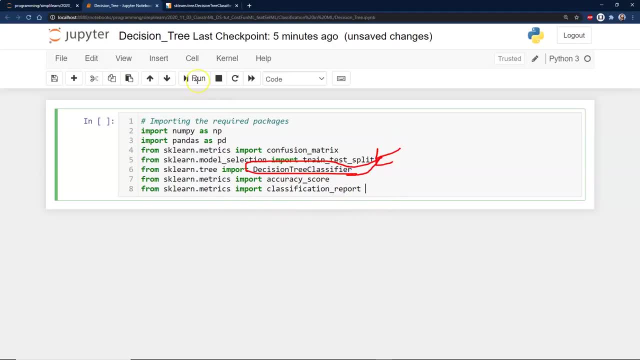 And of course, we want to know the accuracy and the classification report on here And we're going to do a little different than we did in the other examples, And there's a reason for this. Let me go ahead and run this and load this up here. We're going to 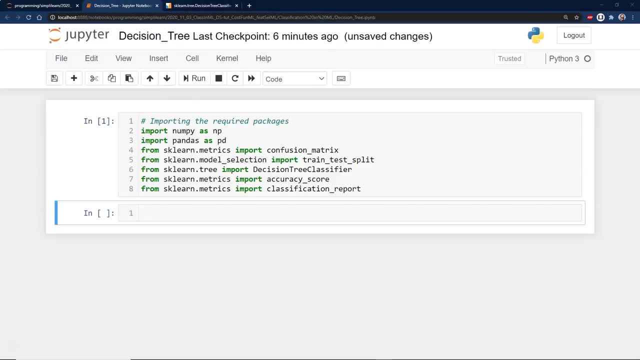 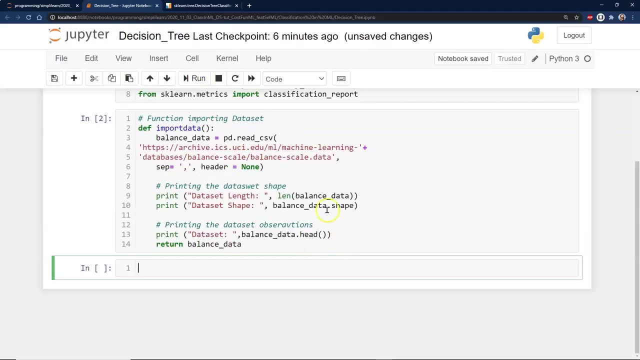 go ahead and build things on functions, And this is when you start splitting up into a team. this is the kind of thing you start seeing a lot more, both in teams and for yourself, because you might want to swap one data to test it on a different data. 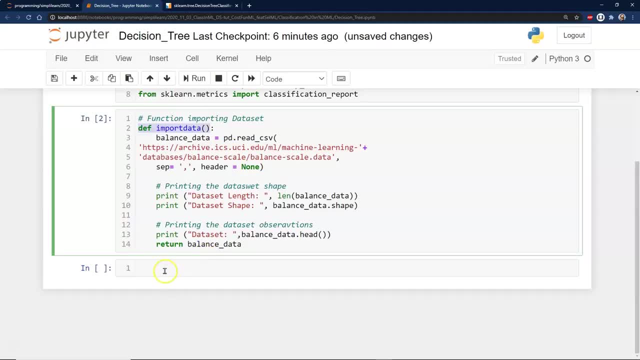 depending on what's going on. So we're going to have our import data here: the data set, length, the balance and so forth. This just returns balance data. Let me just go ahead and print, because I'm curious as to what this looks like. 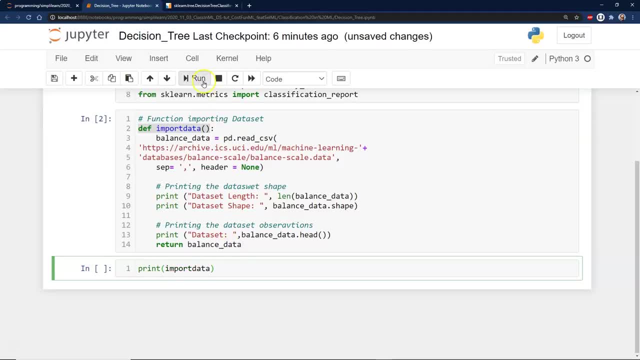 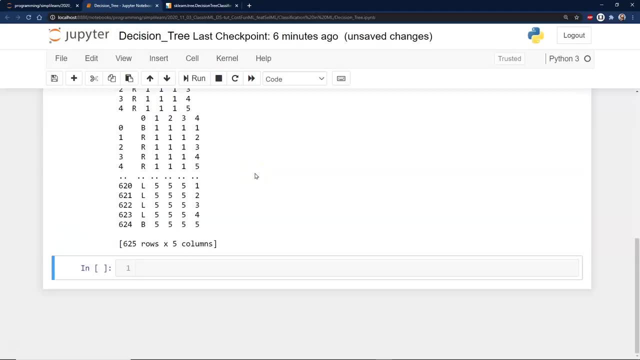 Import data And it's going to return the balance data. So if I run that, if we go ahead and print this out here and run that, you can see that we have a whole bunch of data that comes in there and some interesting setup on here has. 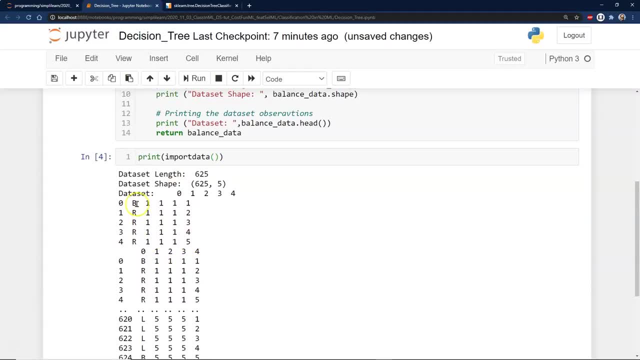 let's see BRR- I'm not sure exactly what that represents on here 111,, 112, and so forth. So we have a different set of data here. The shape is five columns: 1,, 2,, 3,, 4, 5.. 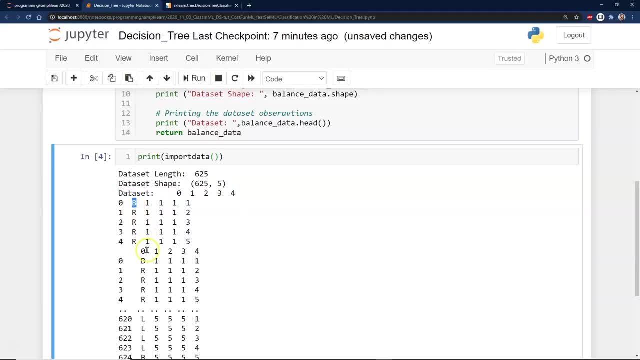 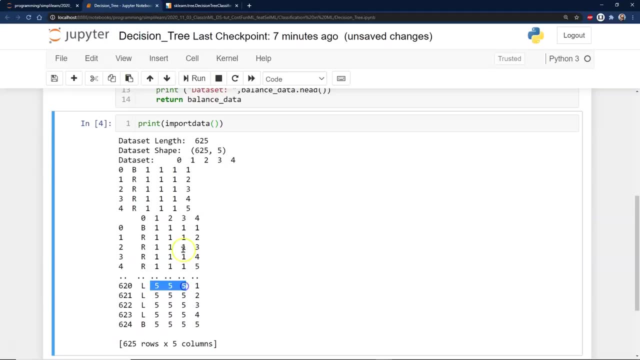 Seems to have a number at the beginning which I'm going to guess- BRL, a letter I mean- And then a bunch of numbers in there: 1111.. Let's see down here we've got 555.. Setup on this And let's see. 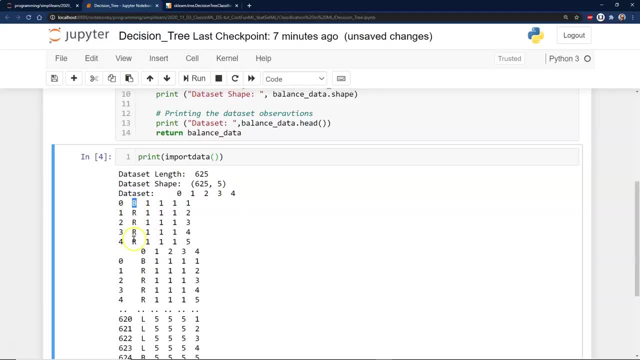 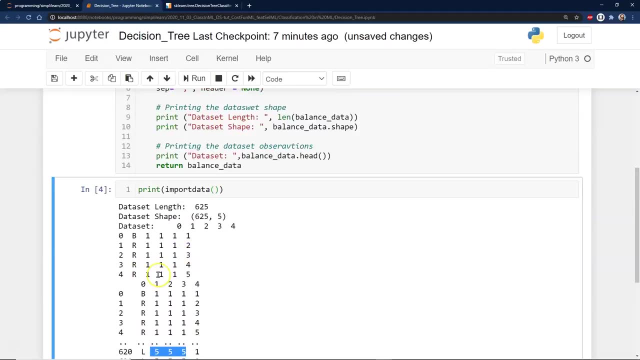 Seems to have a number at the beginning, which I'm going to guess BRL, a letter, I mean, and then a bunch of numbers in there, One, one, one, one. Let's see down here Five set up on this and let's see balance data. 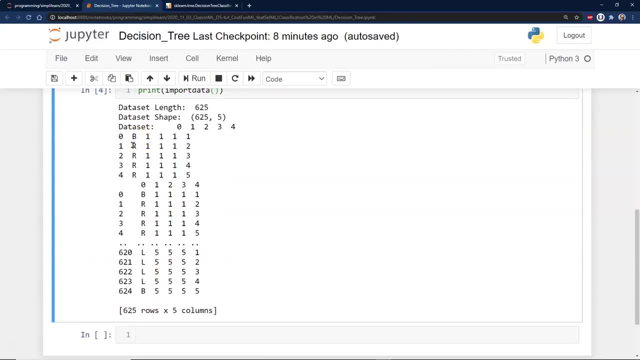 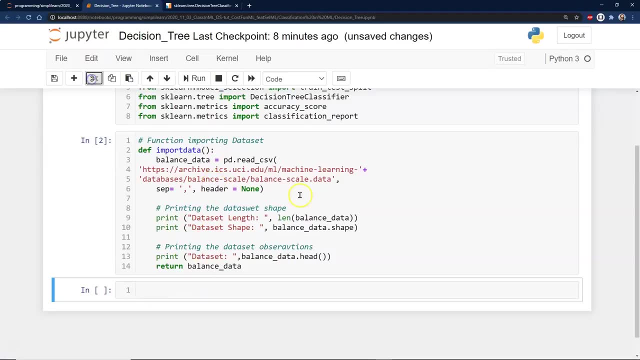 And since it said balance data, I'm going to guess that B means balanced, R means you need to move it right And L means it needs to be moved left or skewed to the left. I'm not sure which one. Let's go and close that out and we'll go. 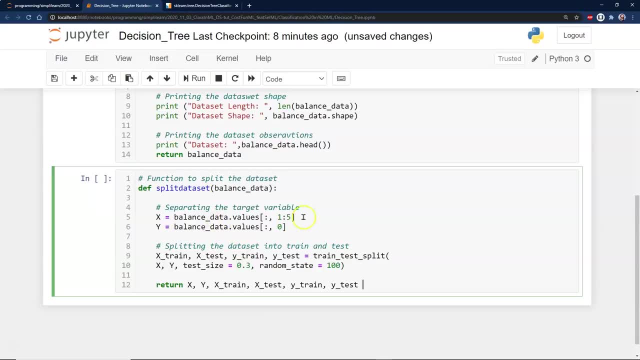 ahead and create a function to split the data set. X balance- data equals data values. Y balance equals data values of zero. There's that letter number- left, right and balance, And then we're looking for the values of one through five And we go ahead and split it just like you would. 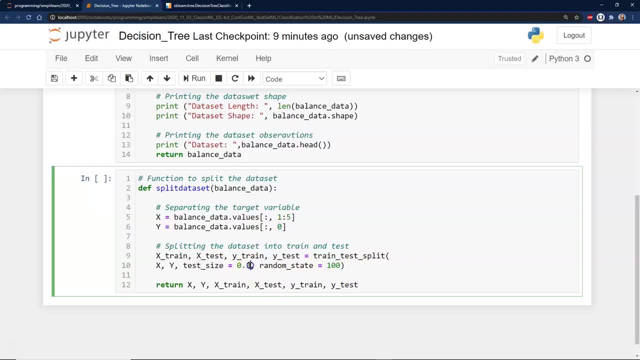 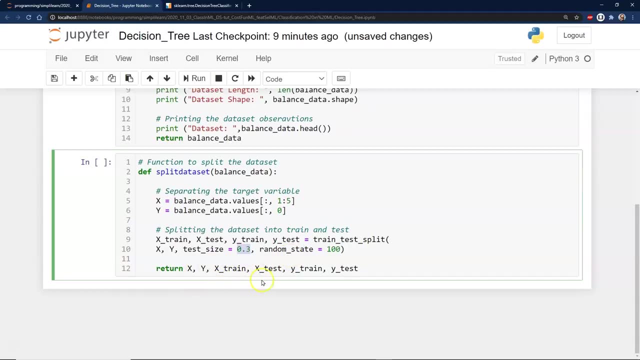 X train Y train set: random state 100, test size is 0.3. So we're taking 30 percent of the data and it's going to return your X, your Y, your Y train, your X train your X test, your Y train your Y test. 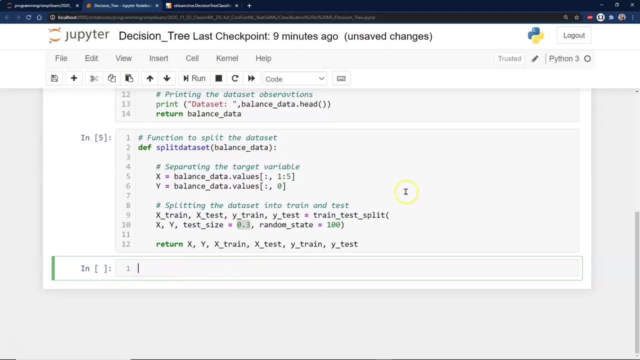 Again, we do this because if you're running a lot of these, you might want to switch how you split the data and how you train it. I tend to use a bifold method. I'll take a third of the data and I'll train it on the other two thirds and test it on that third. 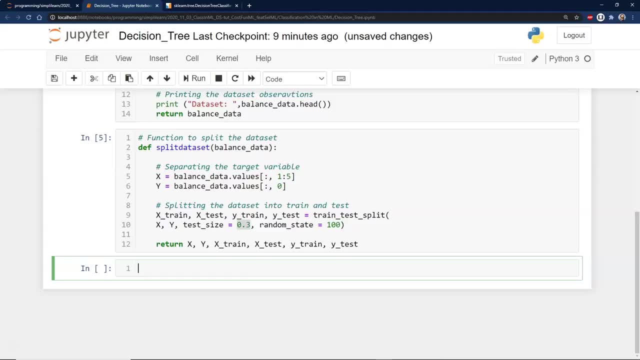 And then I'll switch it. I'll switch which third is a test data, And then I can actually take that information and correlate it And it gives me a really robust package for figuring out what the complete accuracy is. But in this case we're just going to go ahead. 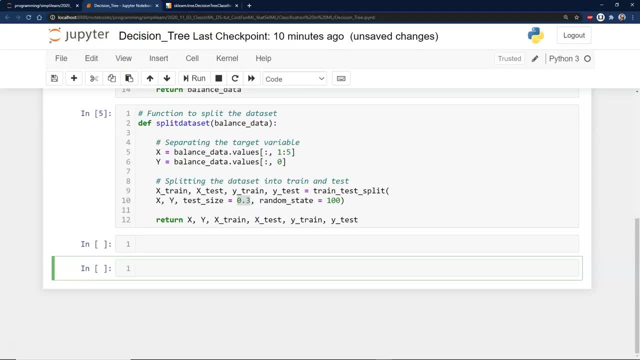 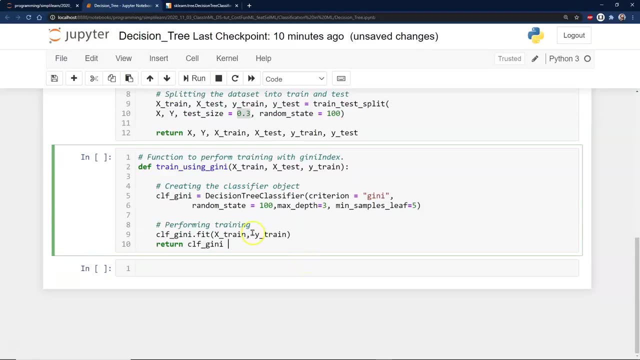 This is our function for splitting data, And this is where it kind of gets interesting, because remember we were talking a little bit about the different settings in our model, And so in here we're going to create a decision tree, but we're going to use the genie set up. 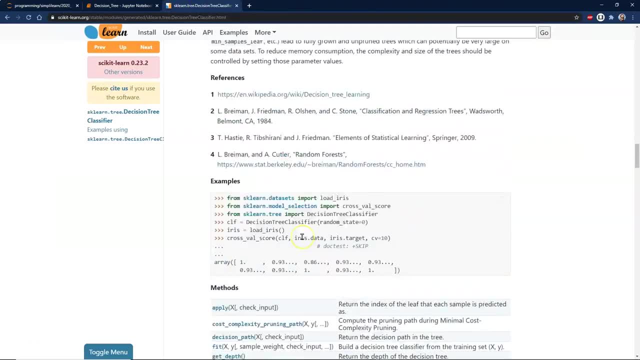 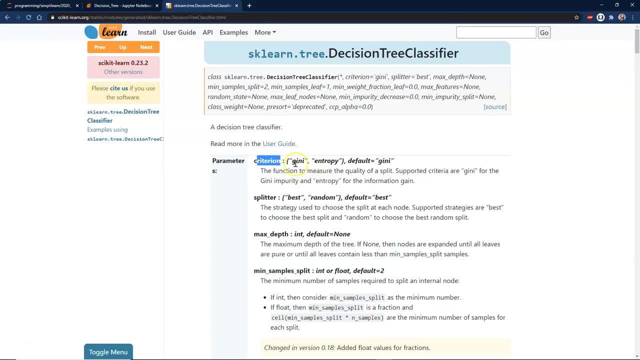 And where did that come from? What's the genie on here? So if we go back to the top of their page and we have, what criterion are we going to use? We're going to use genie. They have genie and entropy. Those are the two main ones that they use for the decision tree. 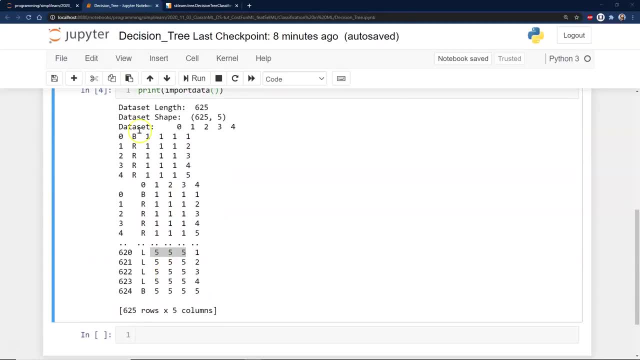 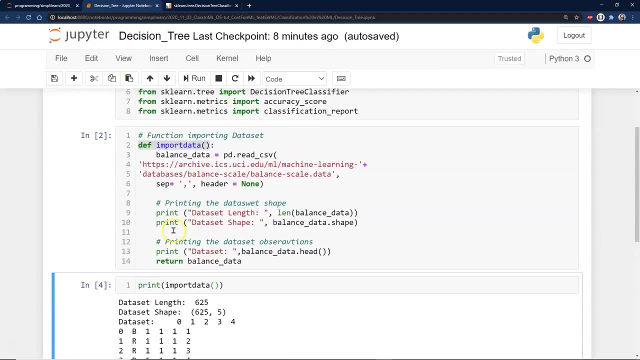 Balance data. And since it said balance data, I'm going to guess that B means balanced, R means you need to move it right and L means it needs to be moved left or skewed to the left. I'm not sure which one Let's go, and. 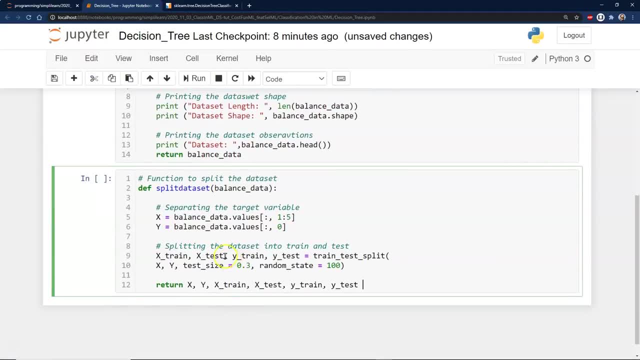 close that out And we'll go ahead and create a function to split the data set. X balance- data equals data values. Y balance equals data values of zero. There's that letter, Remember: left, right and balance. Then we're looking for the values of 1 through 5.. 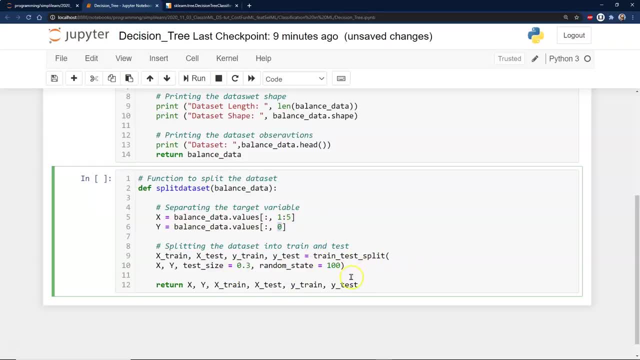 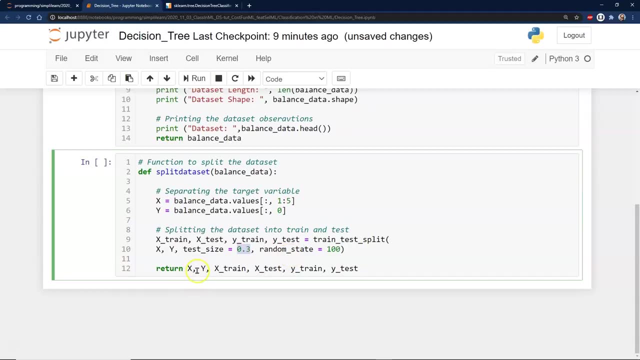 And we go ahead and split it just like you would. X train, Y train set. random state 100.. Test size is .3, so we're taking 30% of the data And it's going to return your X, your Y, your Y train. 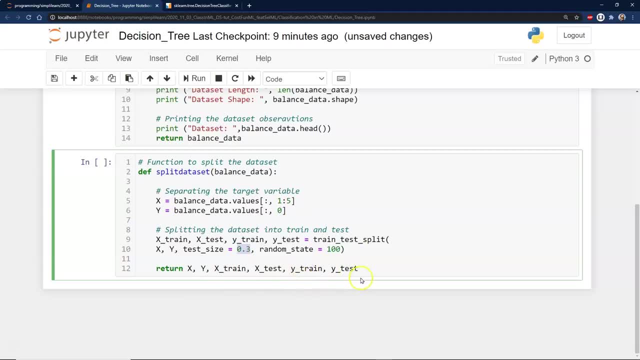 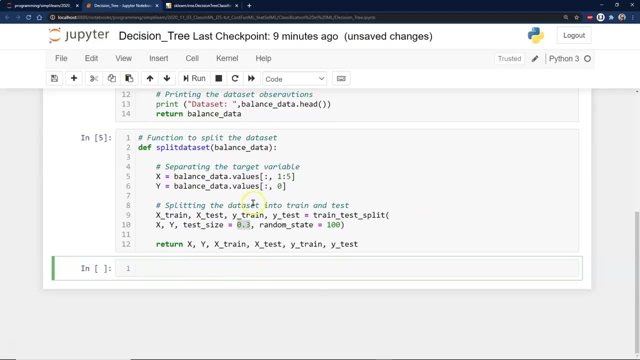 your X, train your X test your Y train your Y test Again. we do this because if you're running a lot of these, you might want to switch how you split the data and how you train it. I tend to use a bifold method. 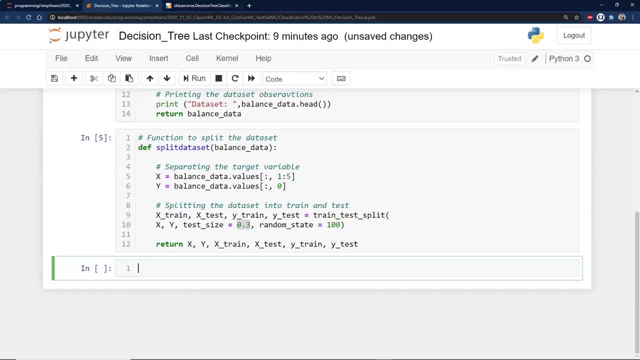 I'll take a third of the data and I'll train it on the other two thirds and test it on that third And then I'll switch it. I'll switch which third is the test data And then I can actually take that information and correlate. 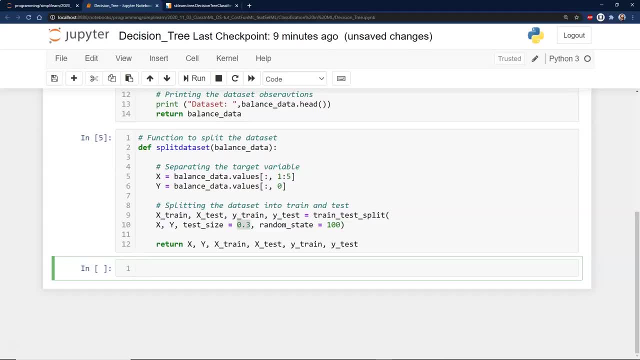 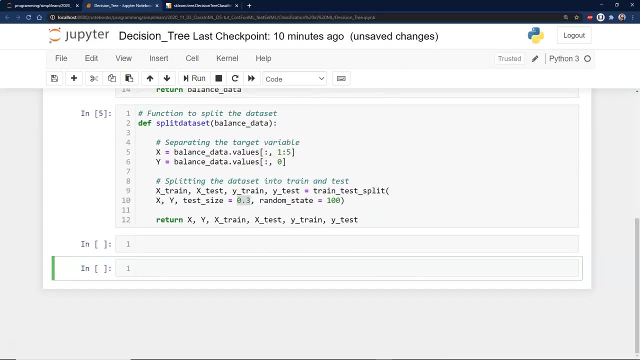 it and it gives me a really robust package for figuring out what the complete accuracy is. But in this case we're just going to go ahead. This is our function for splitting data, And this is where it kind of gets interesting, Because, remember, we were talking a little bit about. 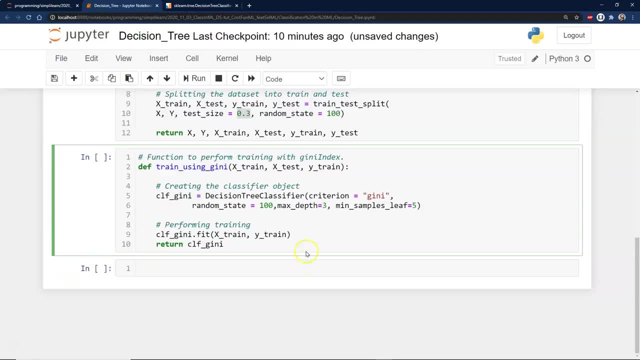 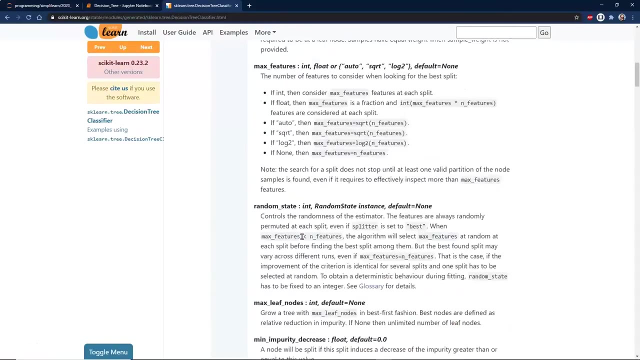 the different settings in our model. And so in here we're going to create a decision tree, but we're going to use the genie setup. And where did that come from? What's the genie on here? So if we go back to the top of their page, 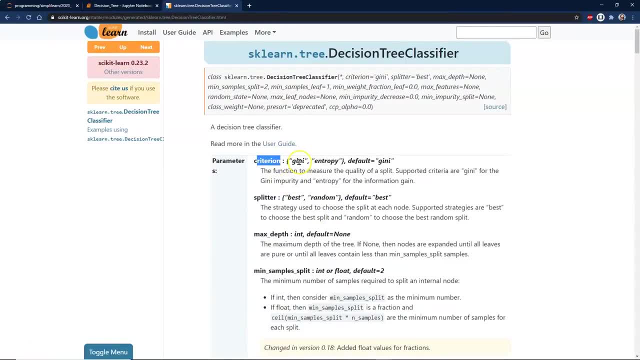 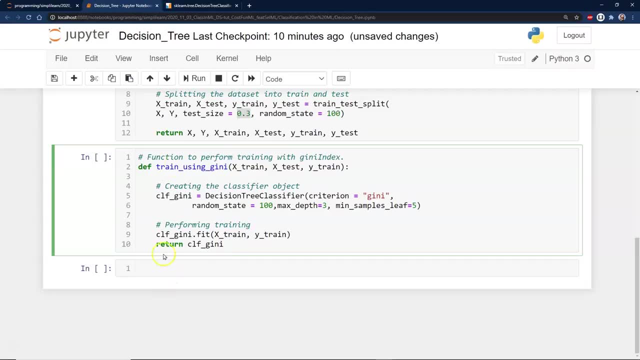 and we have. what criterion are we going to use? We're going to use genie. They have genie and entropy. Those are the two main ones that they use for the decision tree. So this one's going to be genie, And if we're going to have 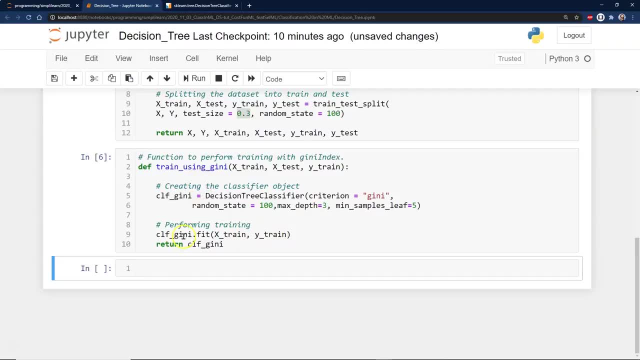 a function that creates the genie model and it even goes down here, And here's our fit train of the genie model. We'll probably also want to create one for entropy. Sometimes I even- just I- might even make this just one function with the different setups. 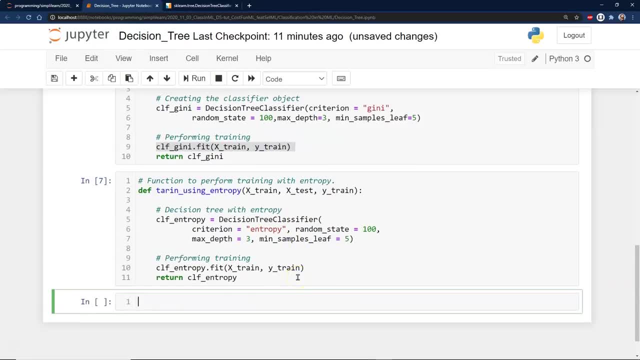 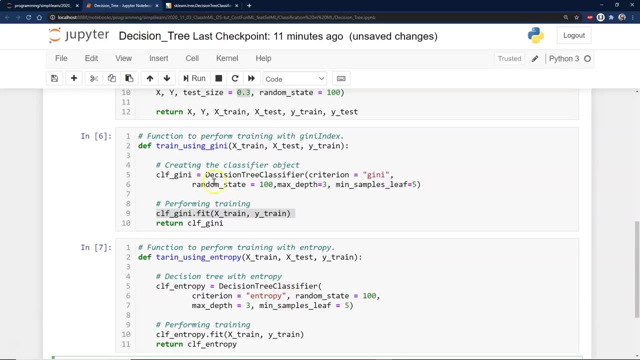 And I know one of my, one of the things I worked on recently. I had to create one that tested across multiple models, And so I would send the parameters to the models, or I would send this part right here where it says decision tree classifier. 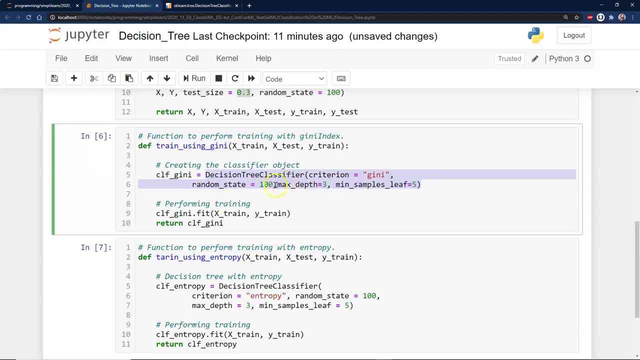 That whole thing might be what I send to create the model, And I know it's going to fit. We're going to have our x train and we're going to have our predict and all that stuff is the same, So you can just send. 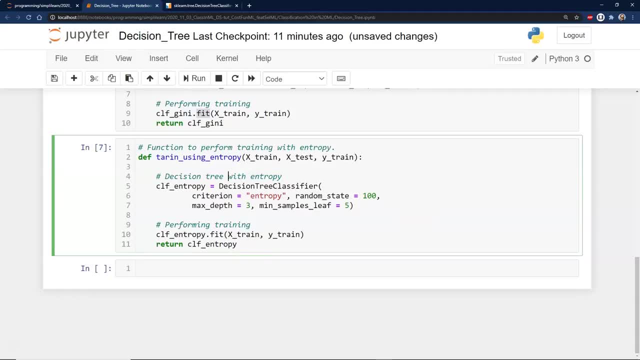 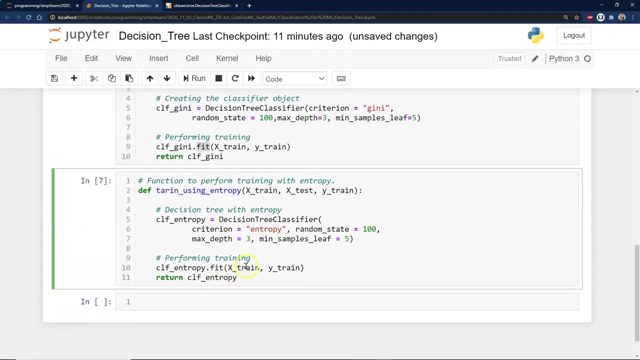 that model to your function for testing different models. Again, this just gives you one of the ways to do it And you can see, here we're going to train with the genie and we're also going to train with the entropy to see how that works. 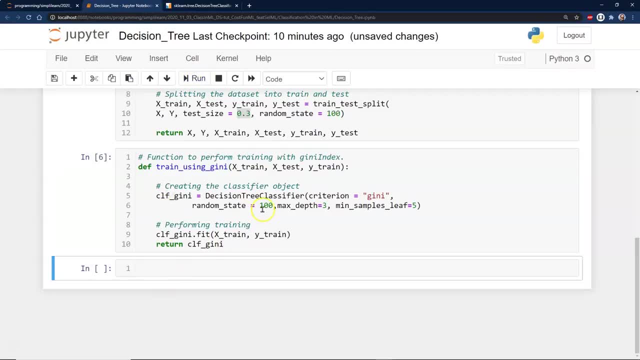 So this one's going to be genie, And if we're going to have a function that creates the genie model- and it even goes down here and here's our fit train to the genie model- we'll probably also want to create one for entropy. 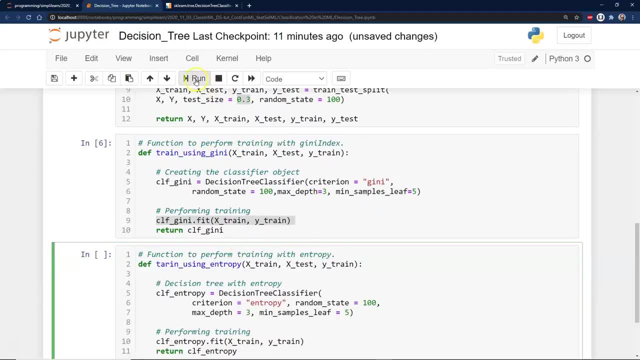 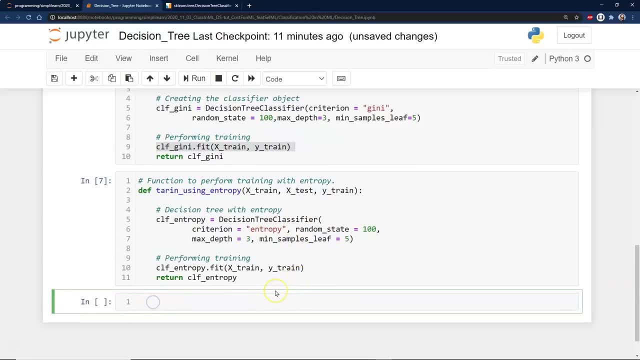 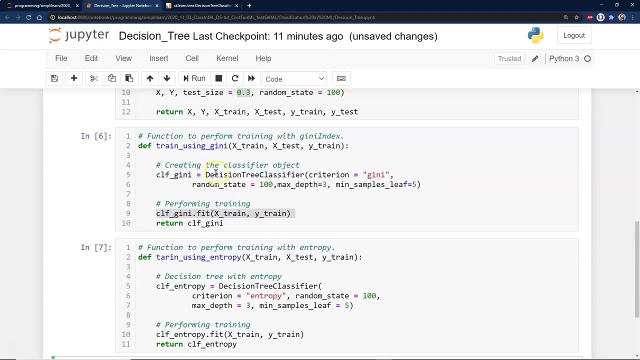 Sometimes I even just I might even make this just one function with the different setups, and I know one of my- one of the things I worked on recently- I had to create a one that tested across multiple models, And so I would send the parameters to the models, or I would send this part right. 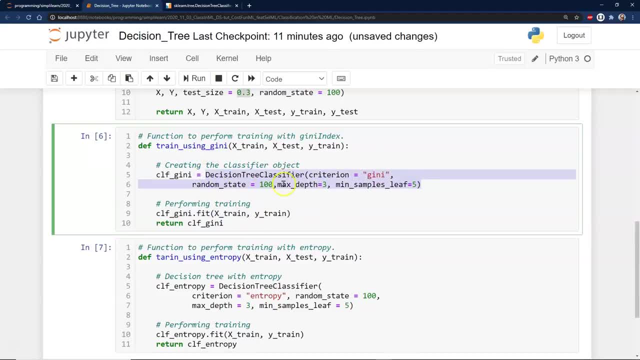 here, which is decision tree classifier. that whole thing might be what I send to create the model And I know it's going to fit. We're going to have our X train and we're going to have a predict and all that stuff is the same. 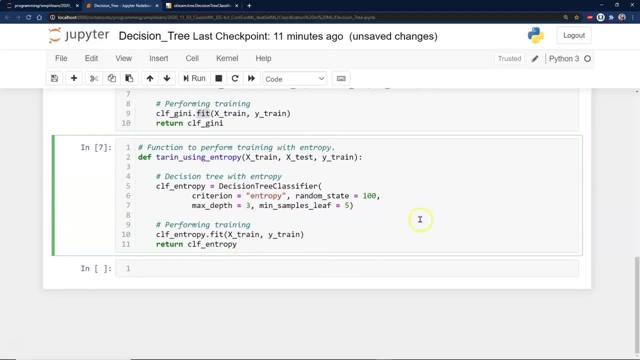 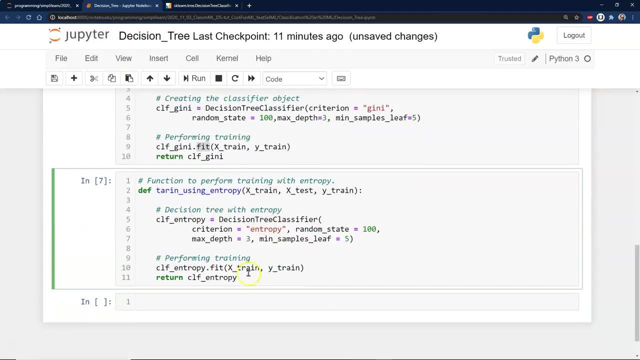 So you can just send that model to your function for testing different models Again, this just gives you one of the ways to do it And you can see, here we're going to train with the genie and we're also going to train with the entropy to see how that works. 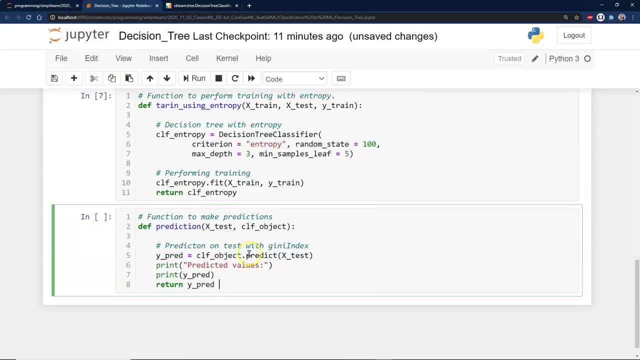 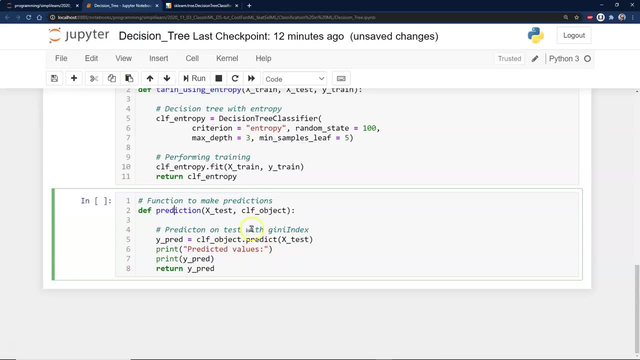 And if you're going to have your models going, two separate models you're sending there- we'll go and create a prediction. This simply is our Y predict equals our whatever object we sent, whatever model we sent here, the CLF object, and predict against our X test. 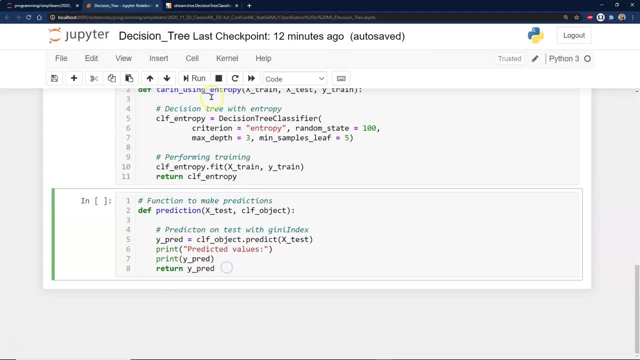 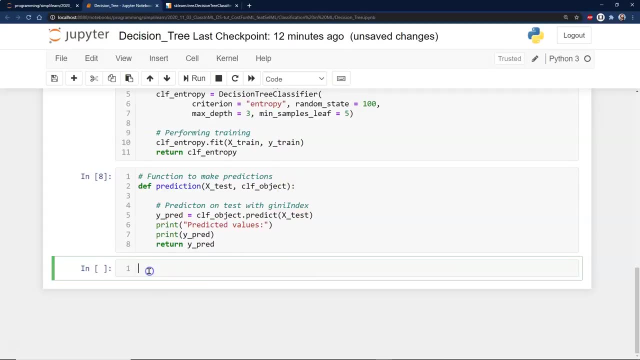 And you can see here: print Y predict and return Y predict set up on here. We'll load that definition up And then, if you're going to have a function that runs a predict and print some things out, we should also have our accuracy function. So here's our: calculate the accuracy. 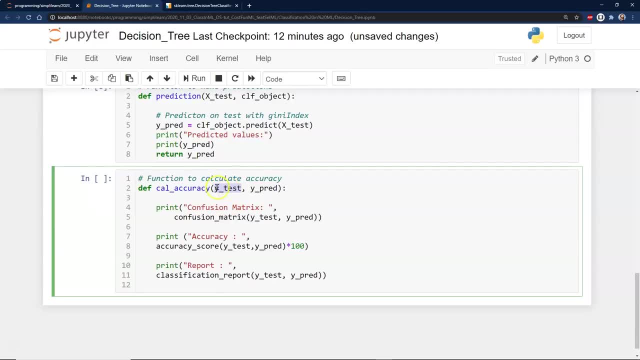 What are we sending? We're sending our Y test data. This could also be Y actual And then Y predict, And then we'll print out a confusion matrix. Then we'll print out the accuracy of the score on here and print a report, classification report. 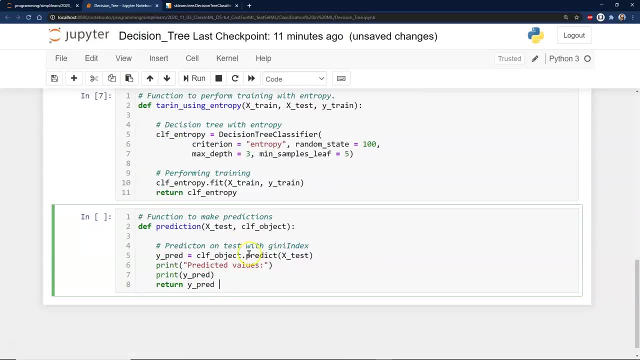 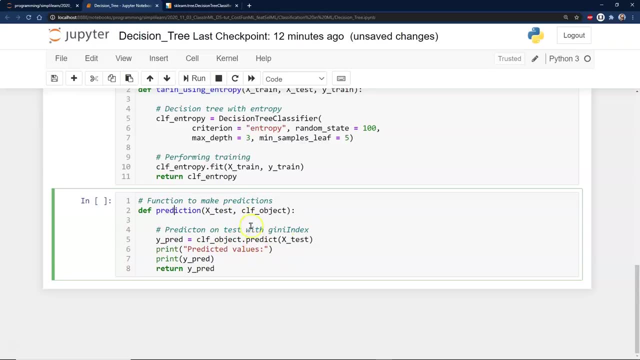 And if you're going to have your models going, two separate models you're sending there- we'll go ahead and create a prediction. This simply is our y predict equals our: whatever object we sent, whatever model we sent here, the CLF object. 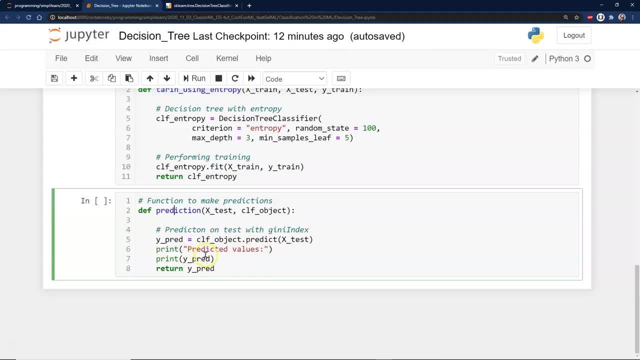 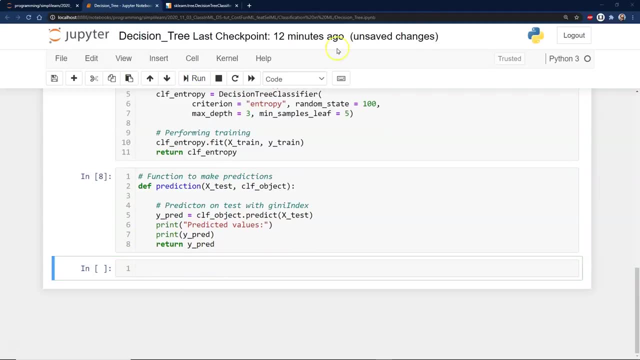 and predict against our x test And you can see here: print y predict and return y predict, set up on here And we'll load that definition up And then if you're going to have a function that runs a predict and prints some things out, 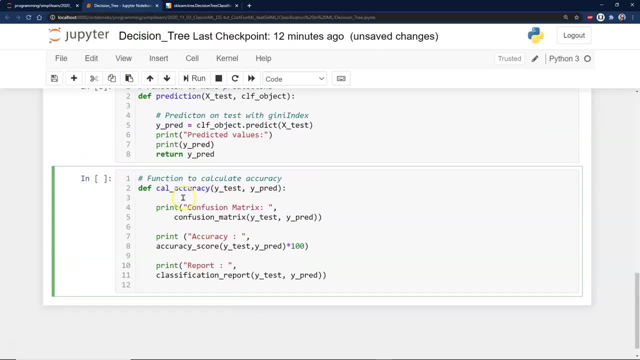 we should also have our accuracy function. So here's our: calculate the accuracy. What are we sending? We're sending our y test data. This could also be y actual and y predict- And then we'll print out a confusion matrix. Then we'll 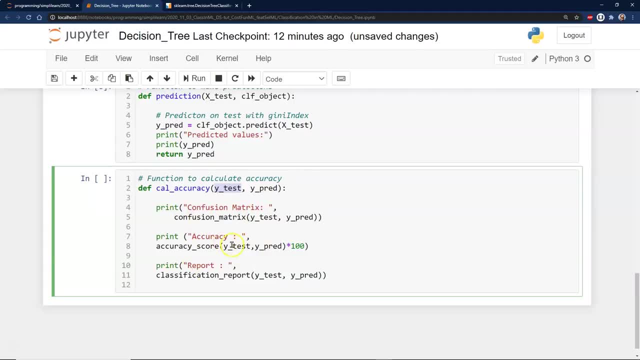 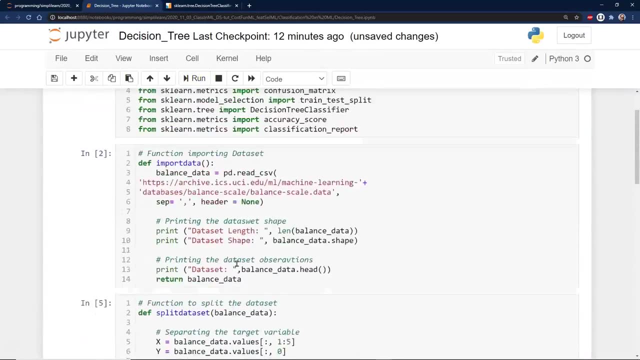 print out the accuracy of the score on here and print a report, classification report, Bundle it all together there. So if we bring this all together, we have all the steps we've been working towards, which is importing our data. By the way, you'll spend 80% of 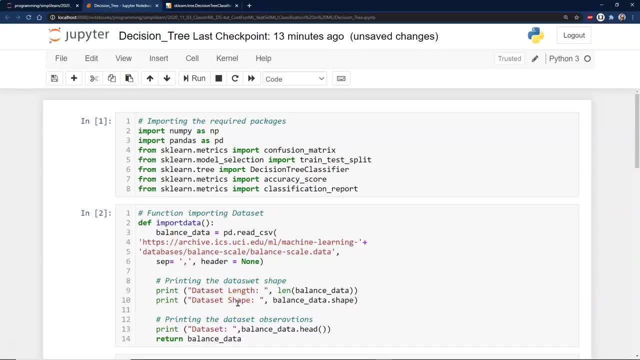 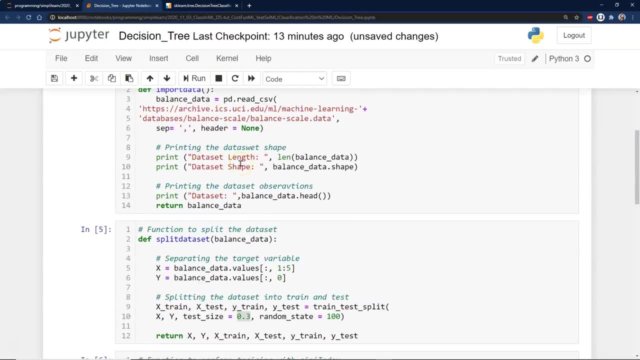 your time importing data in most machine learning setups and cooking it and burning it and getting it formatted so that it works with whatever models you're working with. The decision tree has some cool features in that if you're missing data, it can actually pick that up and just skip that, It says. 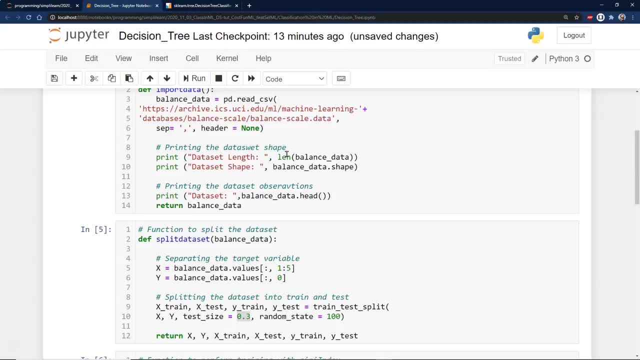 I don't know how to split this. There's no way of knowing whether it rained or didn't rain last night, so I'll look at something else, like whether you watched TV after 8 o'clock. You know that blue screen thing. So we have. 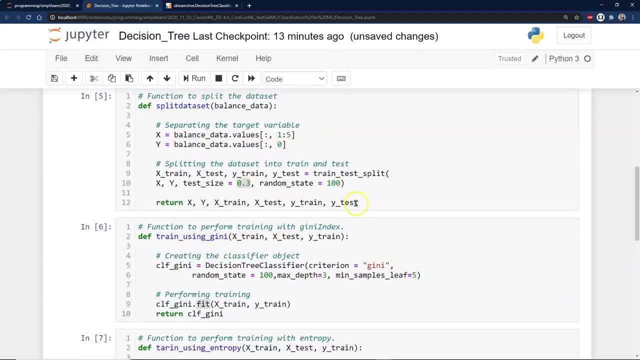 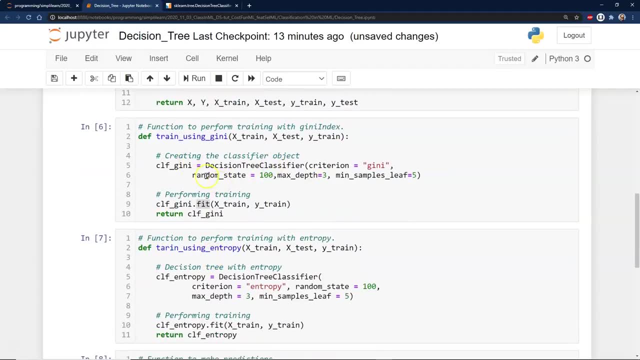 our function, importing our data set. We bring in the data, We split the data so we have our x test and y train And then we have our different models, Our CLF Genie. so it's a decision tree classifier using the Genie setup, And then we can also. 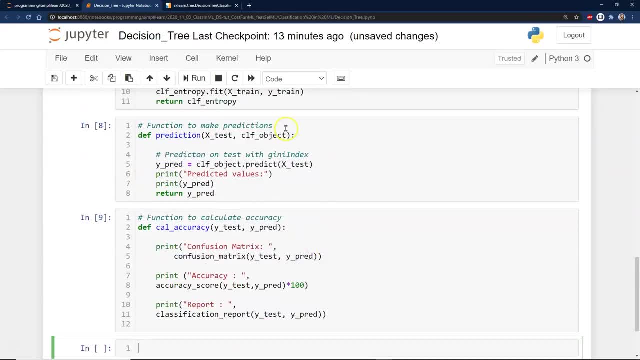 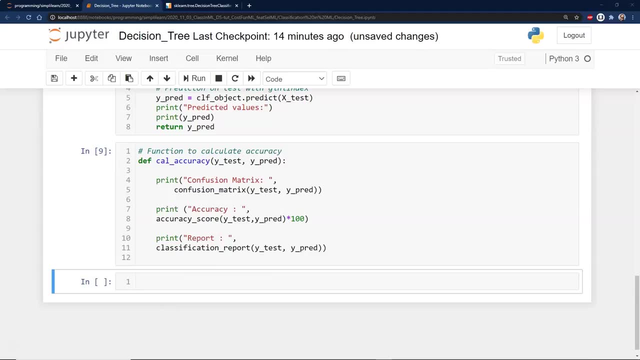 create the model using entropy And then, once we have that, we have our function for making the prediction And we have our function for calculating the accuracy, And then, if we're going to have that, we should probably have our main code involved here. This probably looks more. 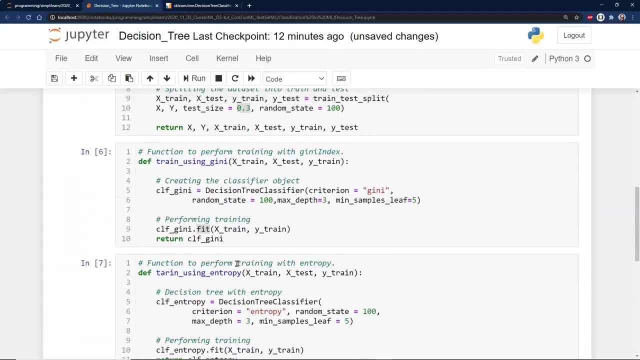 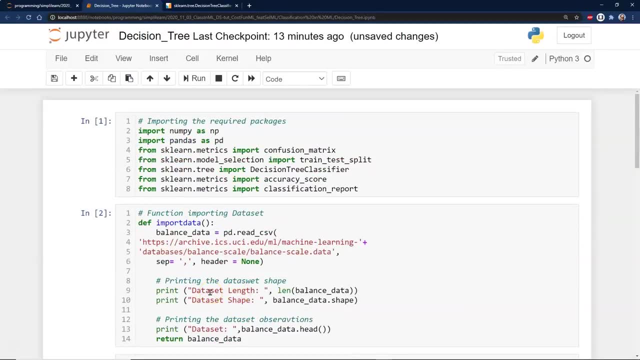 Bundle it all together there. So if we bring this all together, we have all the steps we've been working towards, which is importing our data. by the ways, you'll spend 80 percent of your time importing data and most machine learning setups and cooking it and burning it, and 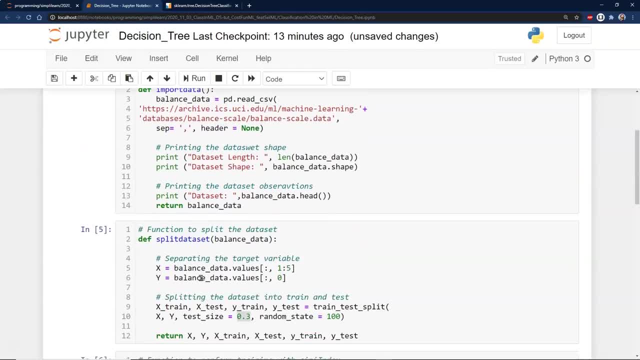 getting it formatted so that it works with whatever models you're working with. The decision tree has some cool features in that if you're missing data, it can actually pick that up and just skip that and says: I don't know how to split this. 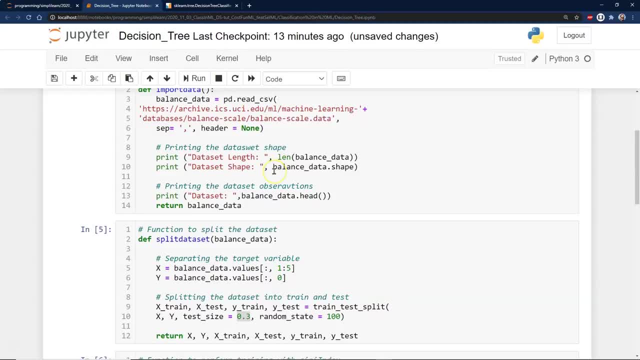 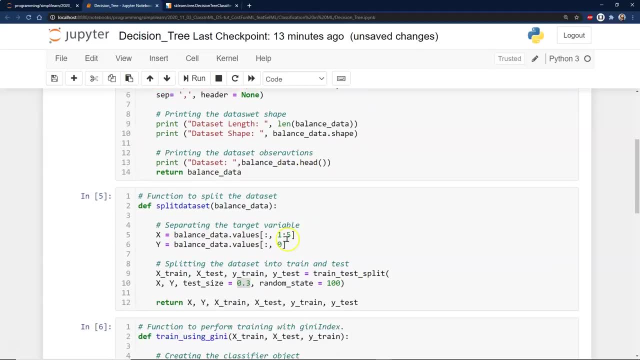 There's no way of knowing whether it rained or didn't rain last night, So I'll look at something else, like whether you watched TV after 8 o'clock. you know that blue screen thing. So we have our function: importing our data set. 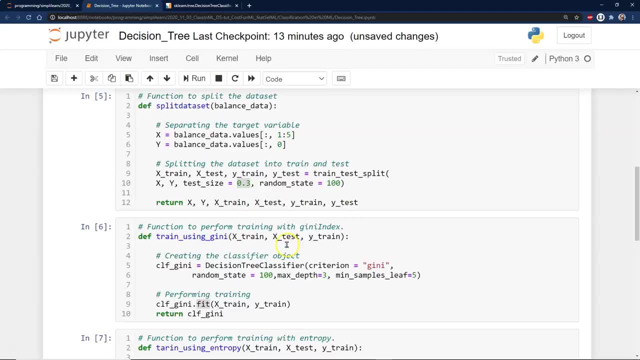 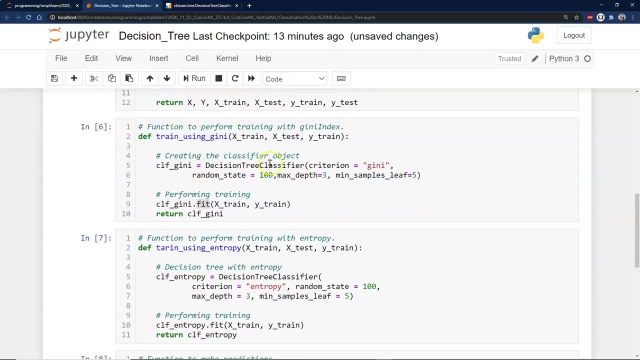 We bring in the data, We split the data, So we have our X test and Y train And then we have our different models, our CLF Genie. So it's a decision tree Classifier using the Genie setup And then we can also create the model using entropy. 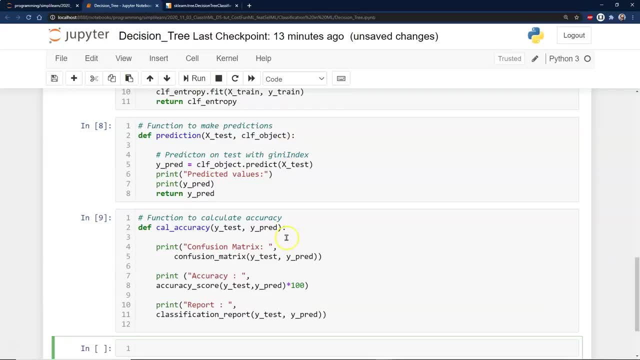 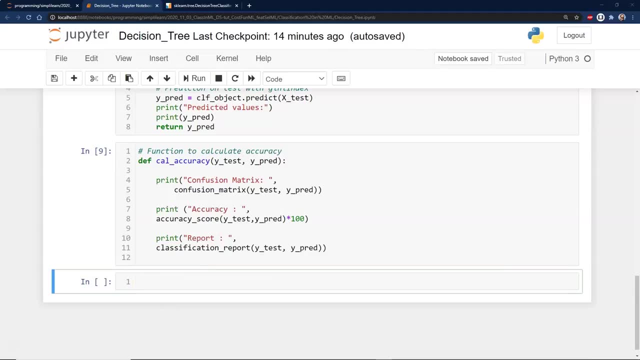 And then, once we have that, we have our function for making the prediction and we have our function for calculating the accuracy, And then, if we're going to have that, we should probably have our main code involved here. This probably looks more familiar if you're depending on what you're working on. 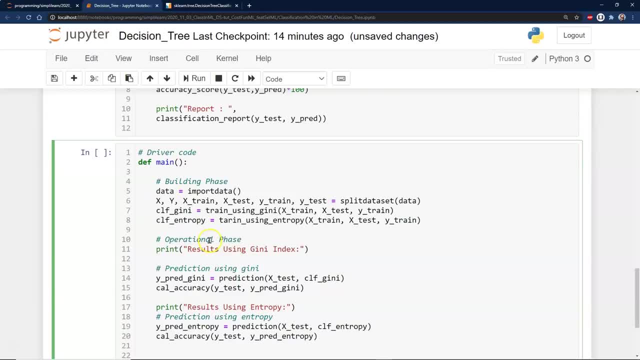 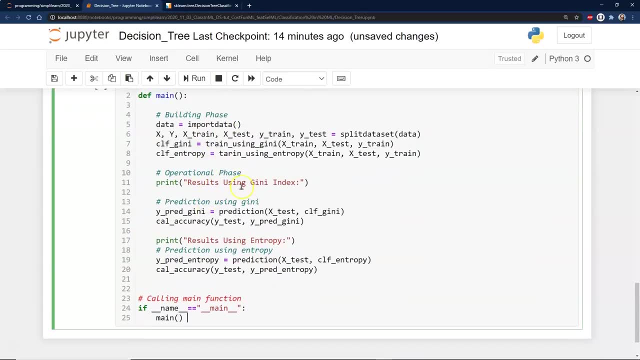 If you're working on like a pie charm, then you would see this in throwing something up real quick in Jupyter Notebook. So here's our main data import, which we've already defined. We get our split data, We create our Genie. 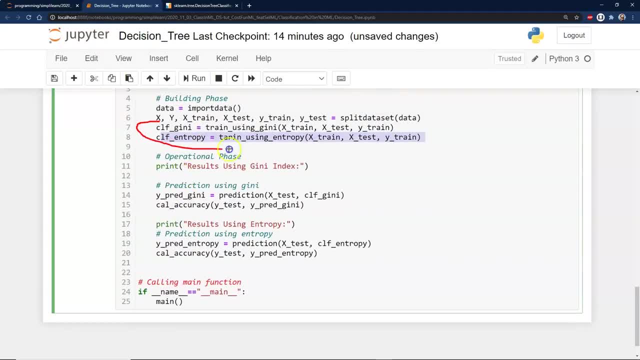 We create our entropy. So there's our two models going on here. There's our two models. So these are two separate data models. We've already sent them to be trained. Then we're going to go ahead and print the results using Genie index. 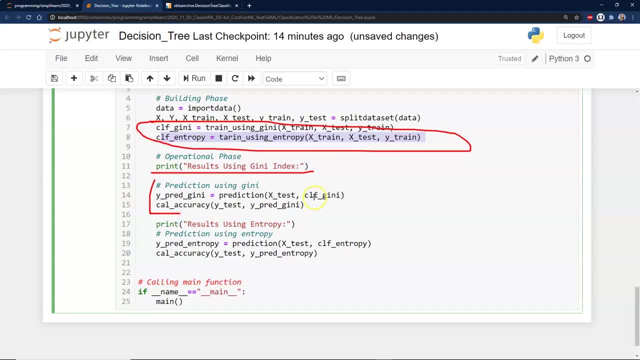 So we'll start with the Genie and we want to go ahead with the Genie and print our predictions- Y, X, test to the Genie and calculate the accuracy on here, And then we want to print the results using Genie. So this is just the same thing coming down like we did with the Genie. 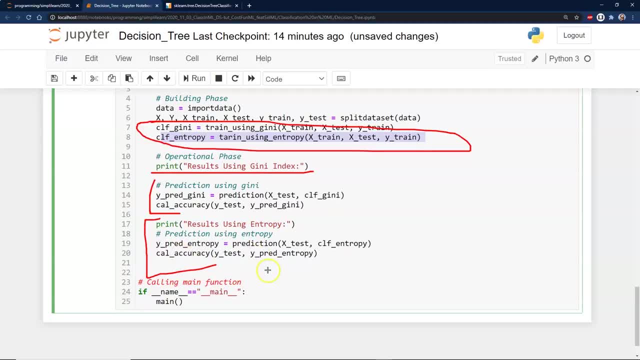 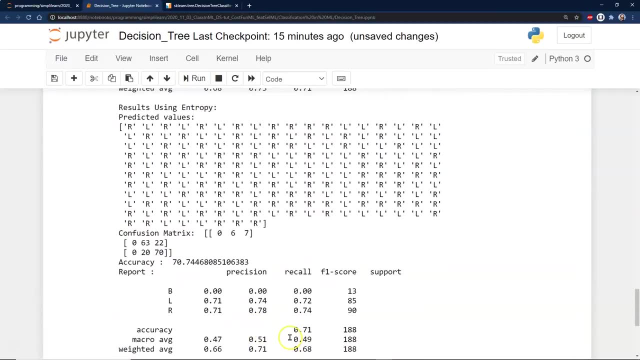 We're going to put out our Y predict entropy and our calculations, So let's go ahead and run that and just see what this piece of code does. We do have, like, one of our data needs to be getting a warning on there. There's nothing major because it's just a simple warning. 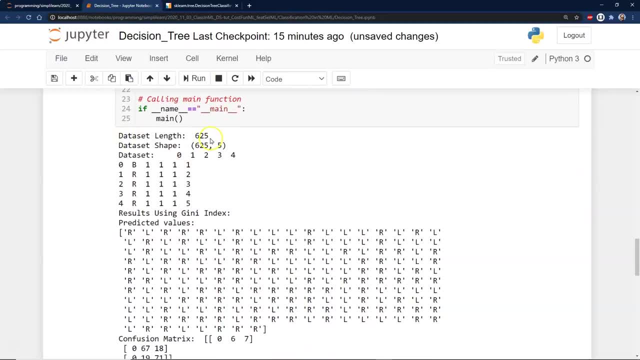 Probably an update of a new versions coming out. And so here we are. We have our data set. It's got 625.. You can actually see an example of the data set B, meaning balanced, I guess. And here's our five data points. 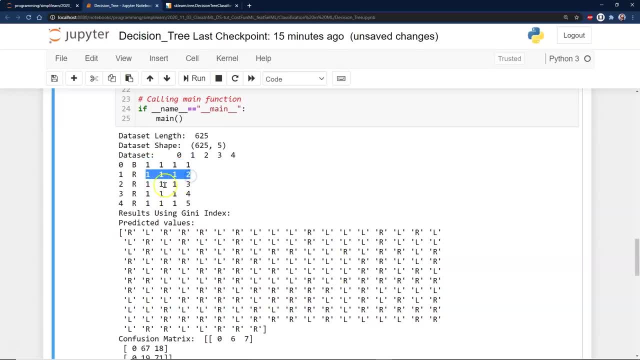 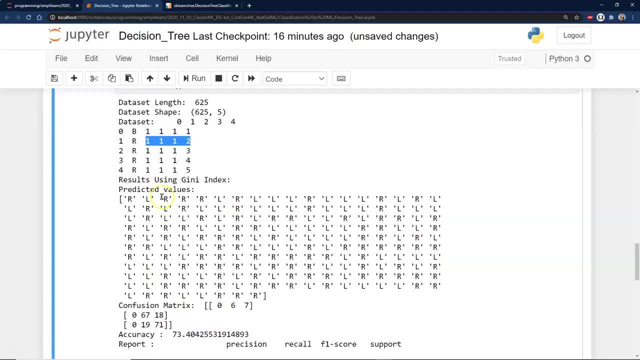 1111 means it's balanced, It's skewed to the right with 1112 and so forth on here, And then we're going to go ahead and predict from our prediction whether it's to the right or to the left. you can think of a washing machine, that's. 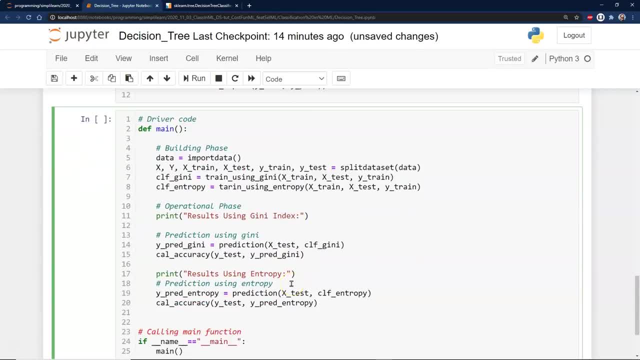 familiar if you're depending on what you're working on. if you're working on like a PyCharm, then you would see this in throwing something up real quick in Jupyter Notebook. So here's our main data import, which we've already defined. 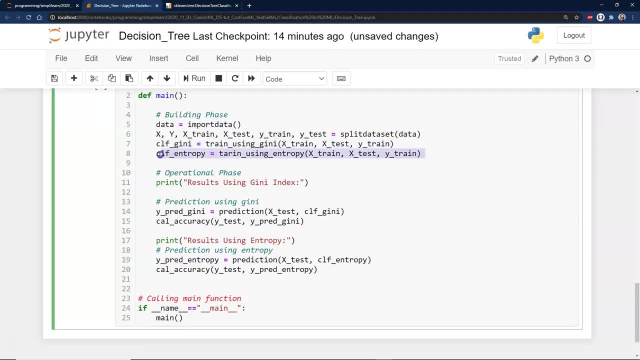 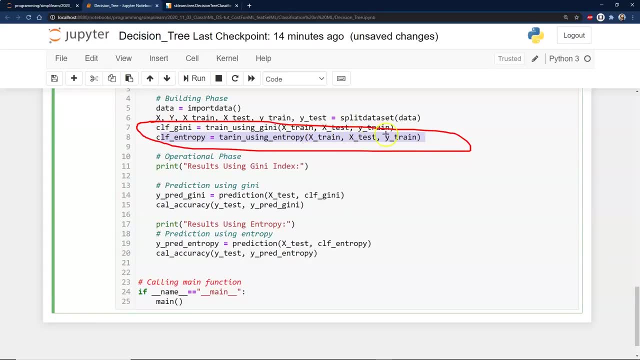 We get our split data, We create our Genie, We create our entropy. So there's our two models going on here. There's our two models. So these are two separate data models. We've already sent them to be trained. Then we're. 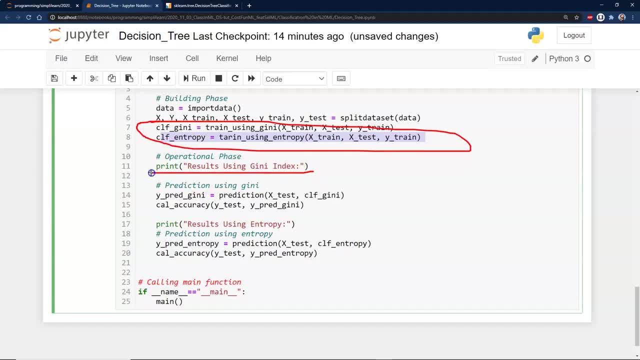 going to go ahead and print the results using Genie index. So we'll start with the Genie And we want to go ahead with the Genie and print our predictions Y, x, test to the Genie And calculate the accuracy on here. 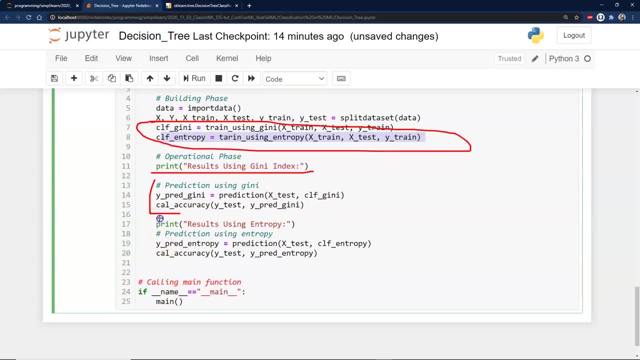 And then we want to print the results using entropy. So this is just the same thing coming down. like we did with the Genie, We're going to put out our Y, predict entropy and our calculations. So let's go ahead and run that and just see. 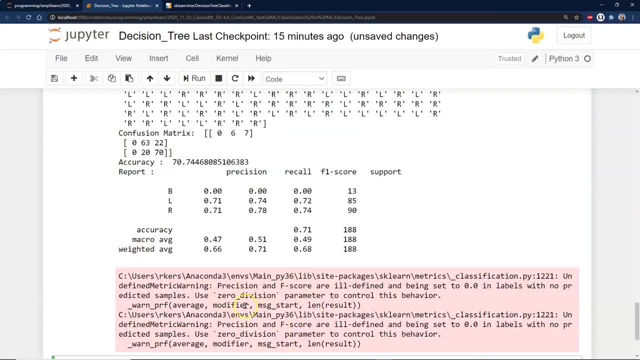 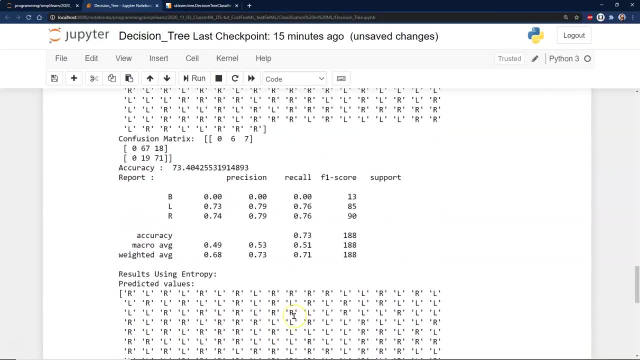 what this piece of code does. We do have, like, one of our data needs to be getting a warning on there. That's nothing major because it's just a simple warning. Probably an update of a new version is coming out, And so here we are. 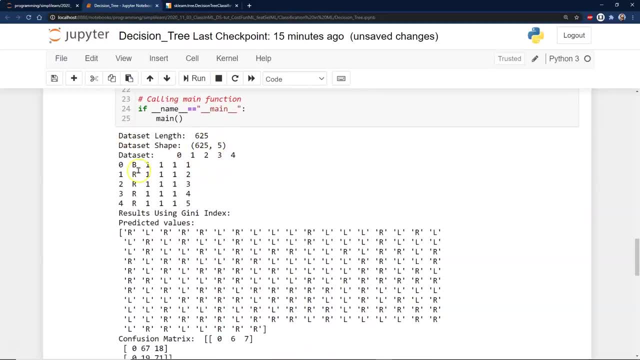 We have our data set. It's got 625.. You can actually see an example of the data set B meaning balanced, I guess. And here's our five data points: 1111 means it's balanced, It's skewed to the right. 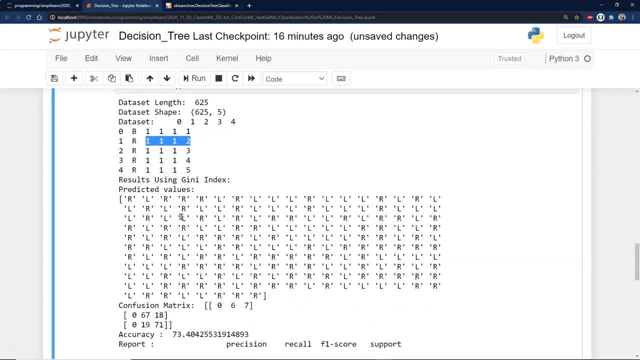 with 1112 and so forth on here, And then we're going to go ahead and predict from our prediction whether it's to the right or to the left. You can think of a washing machine that's banging on one side of the thing, or 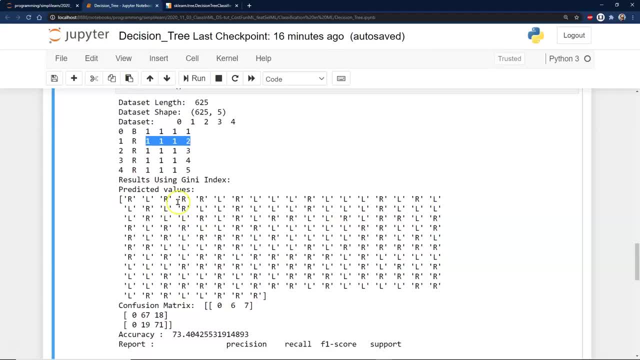 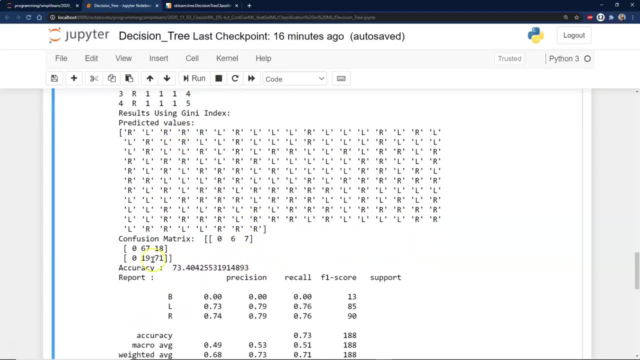 banging on one side of the thing, or maybe it's an automated car, or down the middle of the road that's in balance and it starts going veering to the right. So we need to correct for it. And when we print out the confusion matrix, we have three different variables: R, L and B. 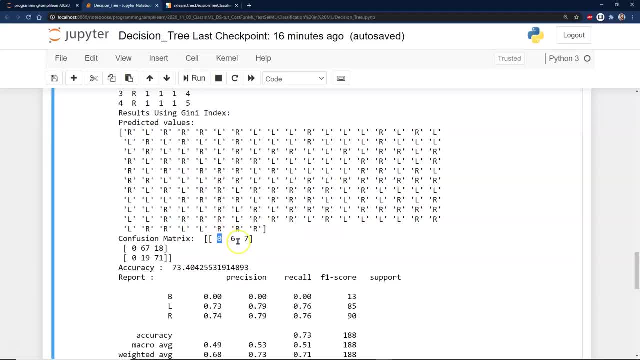 So we should see the three different variables on here and you have, as far as whether it predicts, in this case, the balance. there's not a lot of balanced loads on here And didn't do a good job guessing whether it's balanced or not. 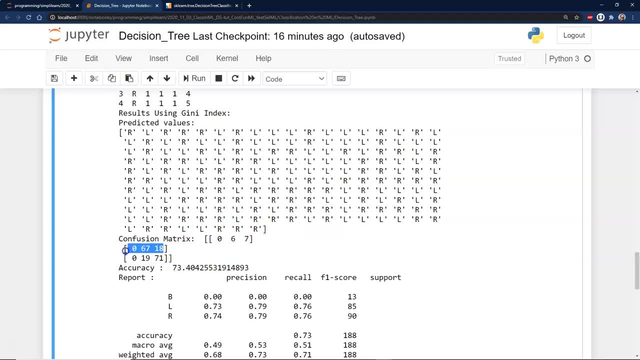 That's what I took from this first one. The second one I'm guessing is the right, So it did a pretty good job guessing the right balance. You can see that a bunch of them came up left unbalanced- Probably not good for an automated car, as it tells you 18 out of the 18 missed things. 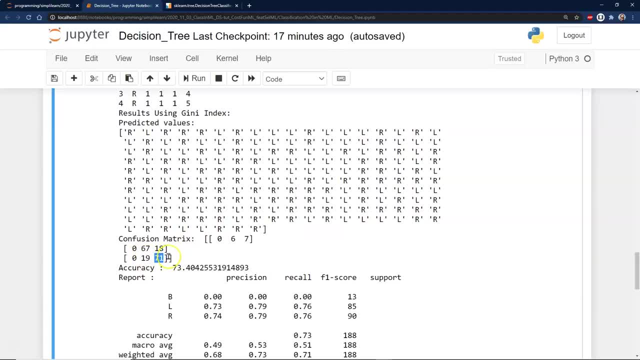 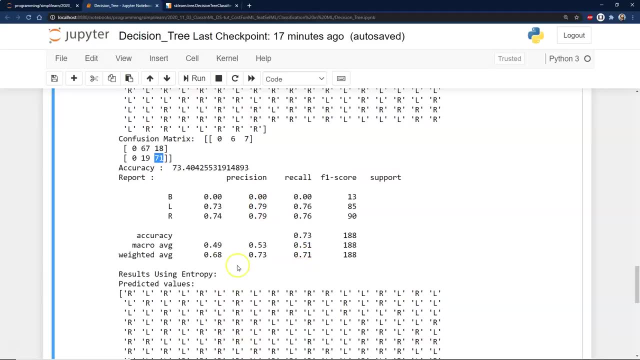 to go the wrong direction, And here we are going the other way. 19 to 71.. And of course we can back that up with an accuracy report on here And you can see the precision, how well the left and right balance is. 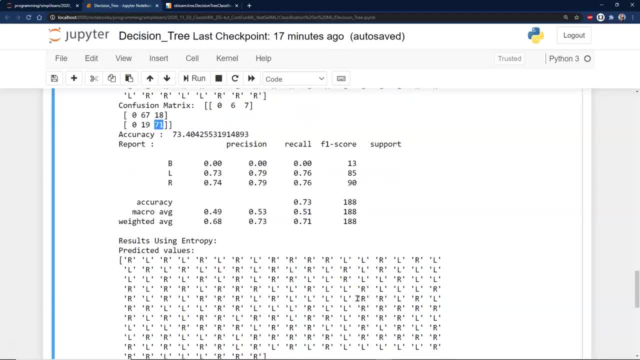 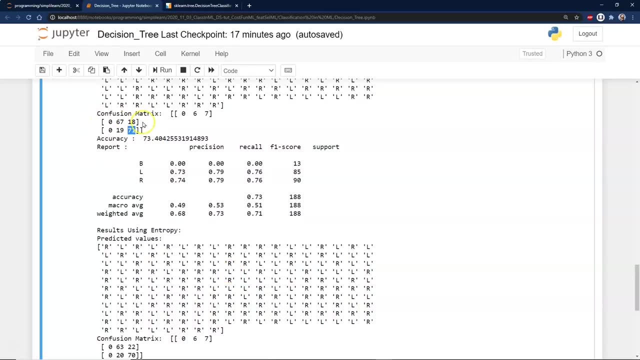 Seventy nine percent, 79 percent precision and so forth. And then we went and used the entropy And let me just see if we can get, so we can get them both next to each other. Here's our entropy of our, the first setup, our first model, which is the Genie model. 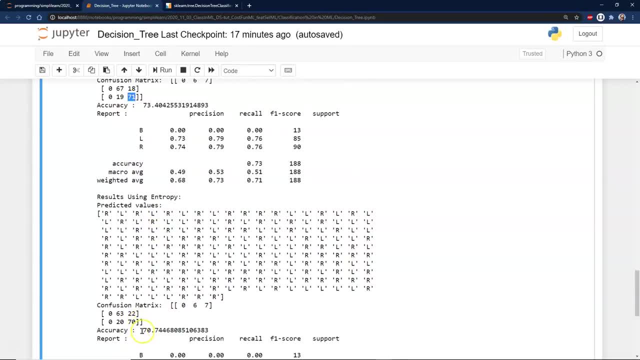 67,, 18,, 19,, 71., 63,, 22,, 20,, 70, pretty close The two models. you know that's not a huge difference in numbers. This second, one of entropy, did slightly- it looks like slightly- worse because it. 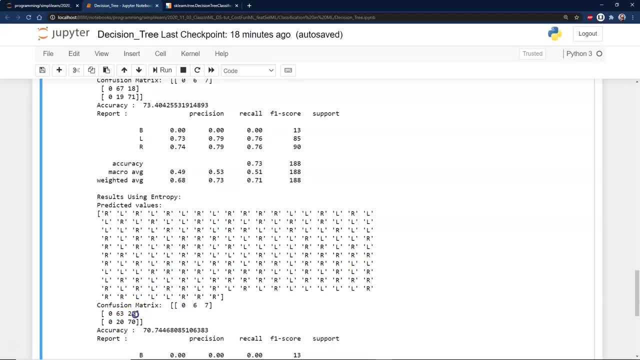 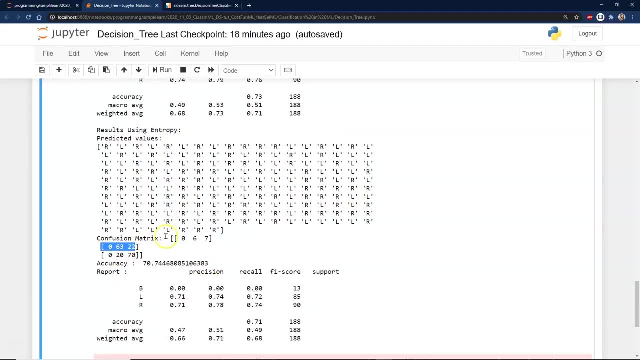 did one better as far as the right balance and did what is this for worse on the left balance or whatever, so slightly worse. if I was guessing between these, I'd probably use the first one. They're so close, though that wouldn't be. 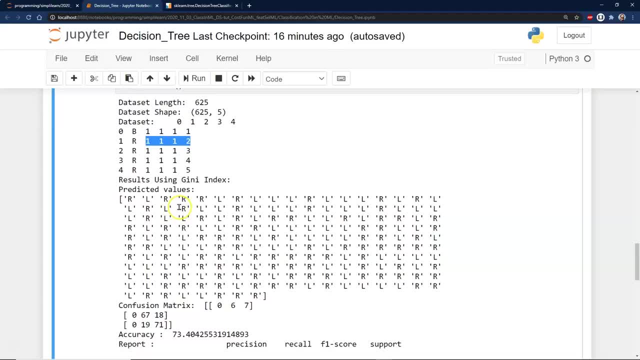 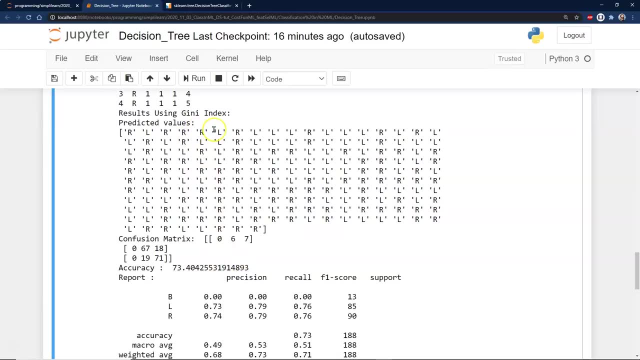 maybe it's an automated car, where we're down the middle of the road That's in balance and it starts veering to the right, So we need to correct for it. And when we print out the confusion matrix, we have three different variables- R, L and B- So we should. 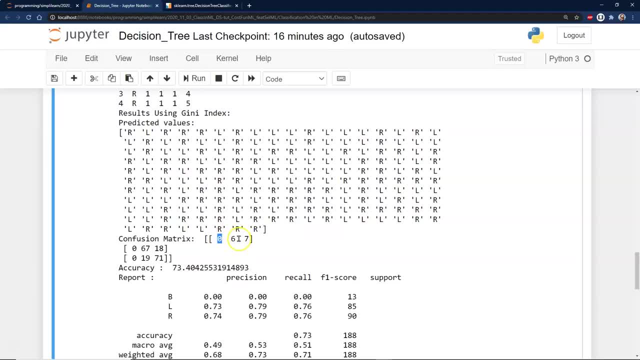 see the three different variables on here And you have as far as whether it predicts, in this case, the balance. There's not a lot of balanced loads on here And it didn't do a good job guessing whether it's balanced or not. That's what I took from. 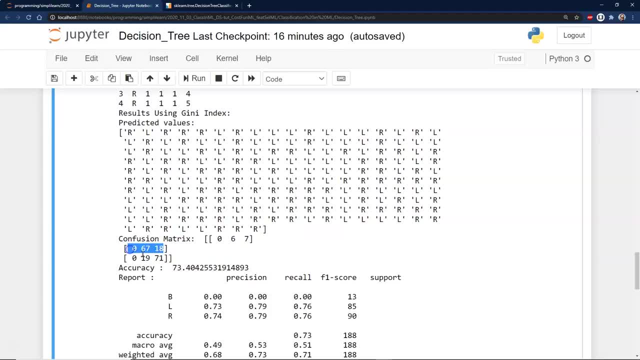 this first one. The second one I'm guessing is the right. So it did a pretty good job guessing the right balance. You can see that a bunch of them came up left unbalanced. Probably not good for an automated car, as it tells you 18 out of. 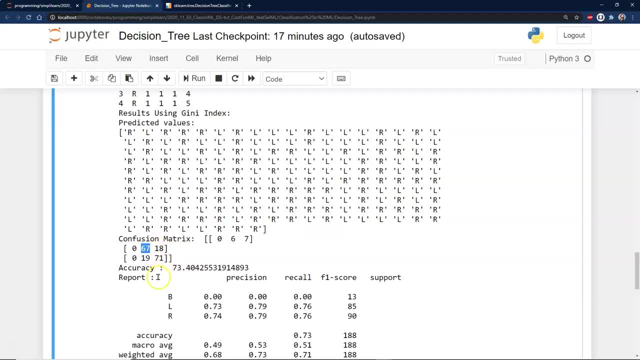 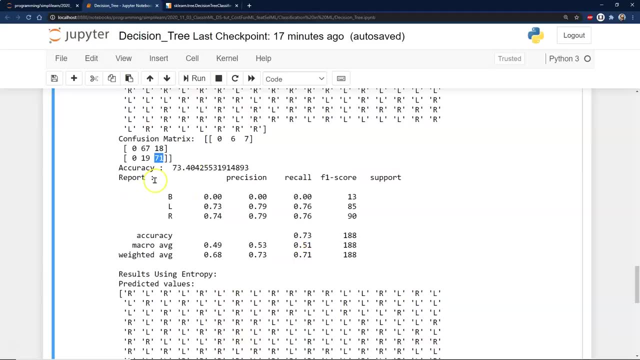 the 18 missed things and tells you to go the wrong direction. And here we are going the other way. 19 to 71. And of course we can back that up with an accuracy report on here And you can see the precision How well the left. 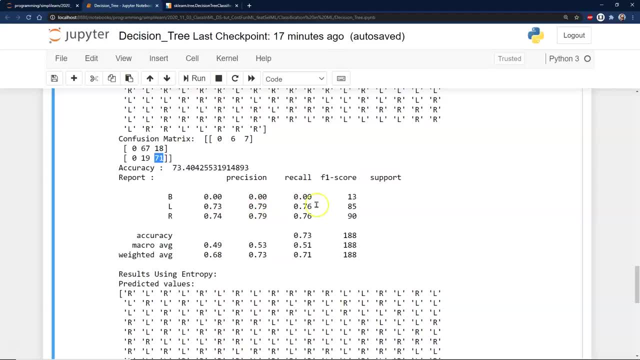 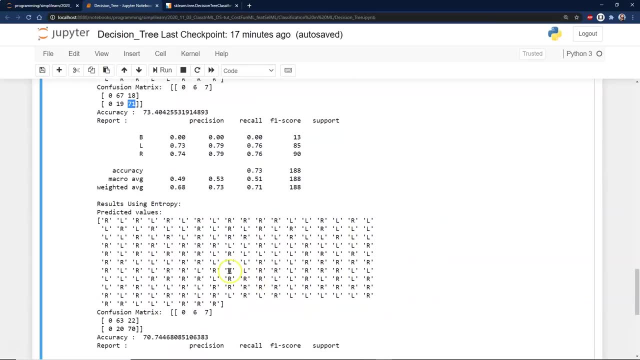 and right balance is 79 percent, 79 percent precision and so forth. And then we went and used the entropy And let me just see if we can get them both next to each other. Here's our entropy of the first setup, Our first model, which is the Genie model. 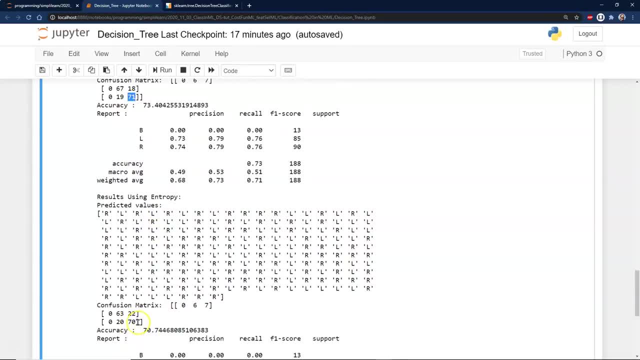 67,, 18,, 19,, 71.. 63,, 22,, 20,, 70. Pretty close, The two models. you know that's not a huge difference in numbers. This second, one of entropy, did slightly- it looks like slightly. 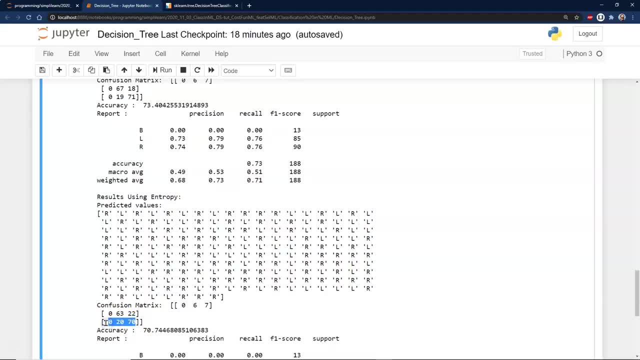 worse because it did one better as far as the right balance and did 4 worse on the left balance or whatever, So slightly worse. If I was guessing between these, I'd probably use the first one. They're so close, though that wouldn't be. 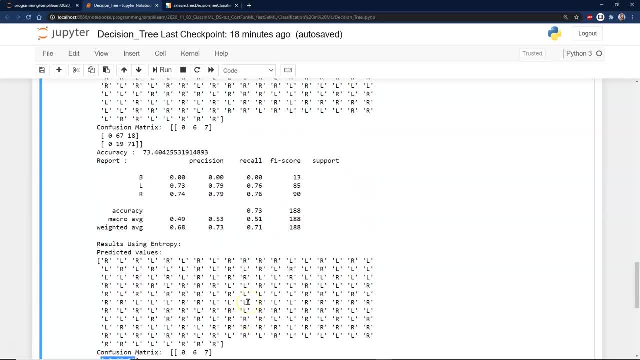 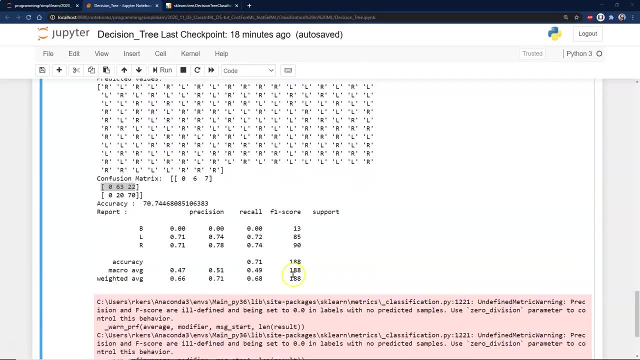 it wouldn't be a clear choice as to which one worked better, And there's a lot of numbers you can play with here which might give better results, depending on what the data is going in. Now, one of the takeaways you should have from the different 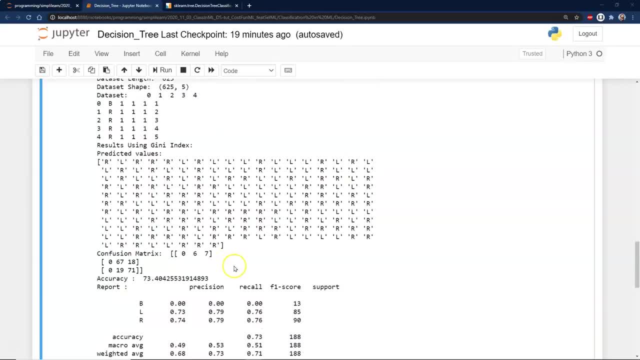 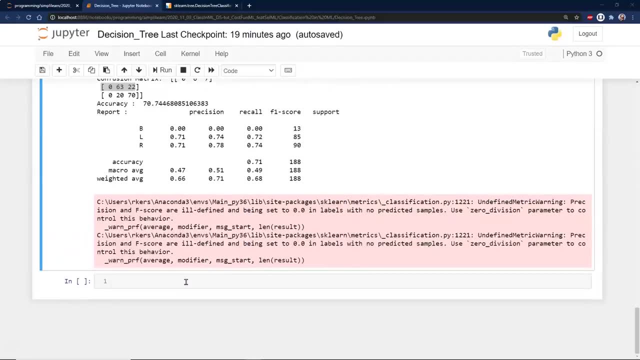 category routines we ran is that they run very similar. You certainly change the perimeters in them as to whether you're using, what model you're using and how you're using it, and what data they get applied to, But when you're talking about the 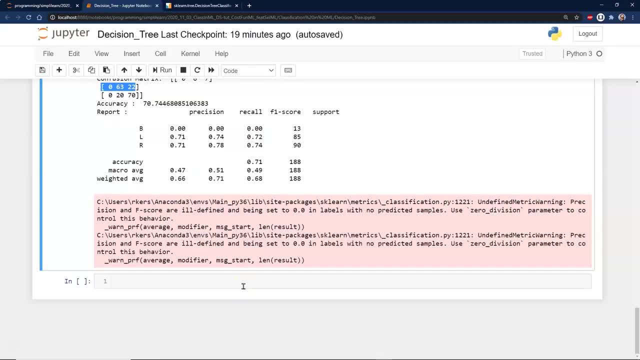 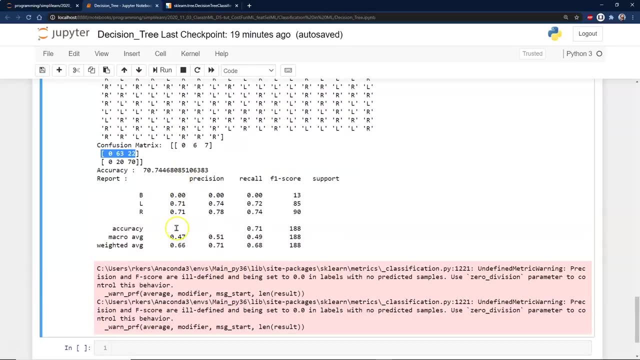 Scikit-Learn package. it does such an awesome job of making it easy. You split your data up, you train your data and you run the prediction and then you see what kind of accuracy, what kind of confusion matrix it generates. So we 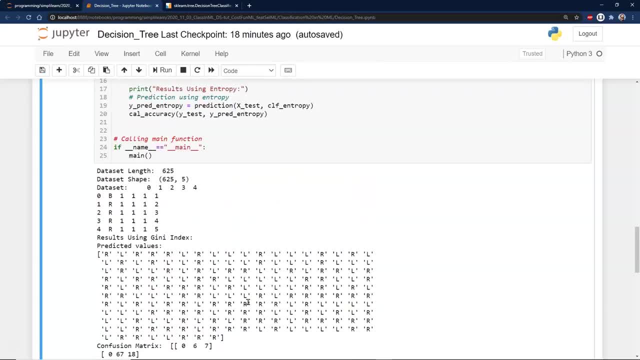 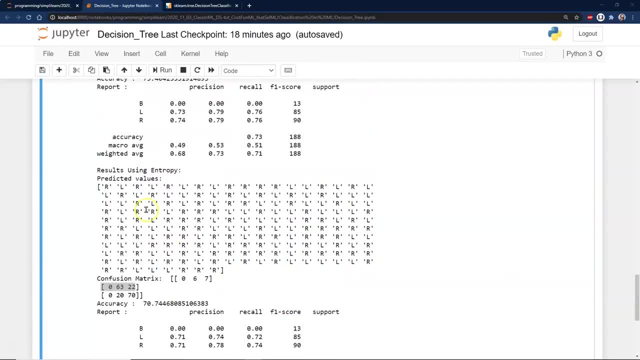 It wouldn't be a clear choice as to which one worked better, And there's a lot of numbers you can play with here which might give better results, depending on what the data is going in Now, one of the takeaways you should have: 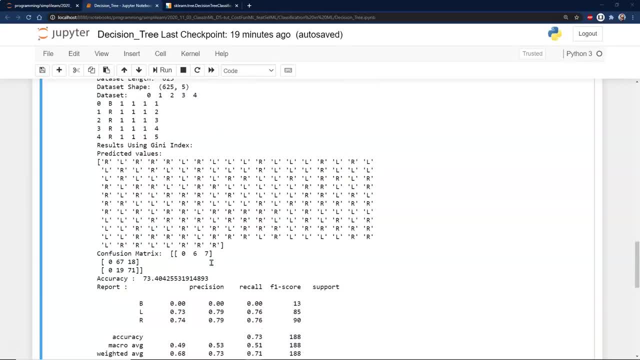 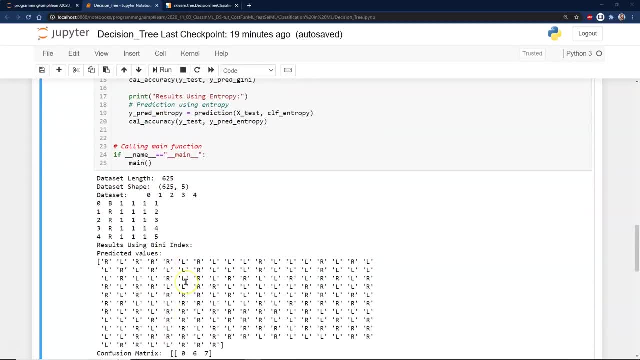 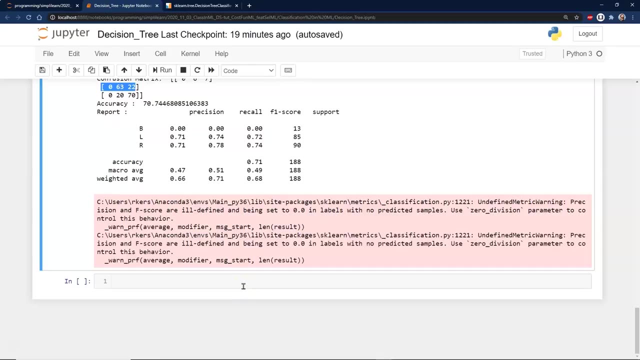 from the different category routines we ran is that they run very similar. You certainly change the perimeters in them as to whether you're using what model you're using and how you're using it and what data they get applied to, But when you're talking about the scikit learn package, it does such an awesome job. 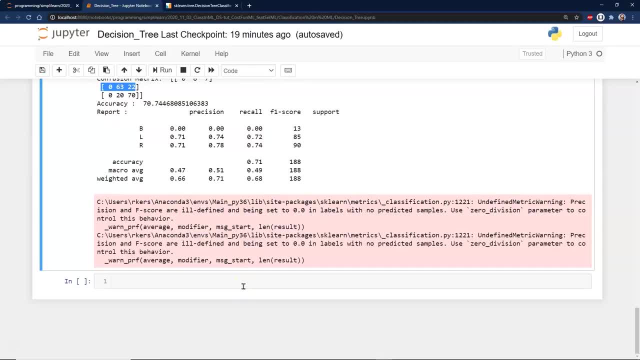 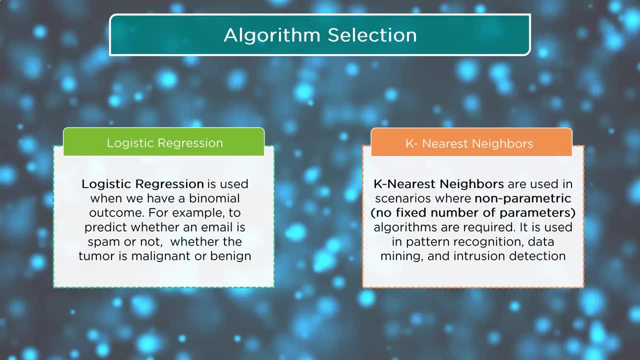 of making it easy. You split your data up, you train your data and you run the prediction and then you see what kind of accuracy, what kind of confusion, matrix it generates. So we talk about algorithm selection, logistic regression, k- nearest neighbors. 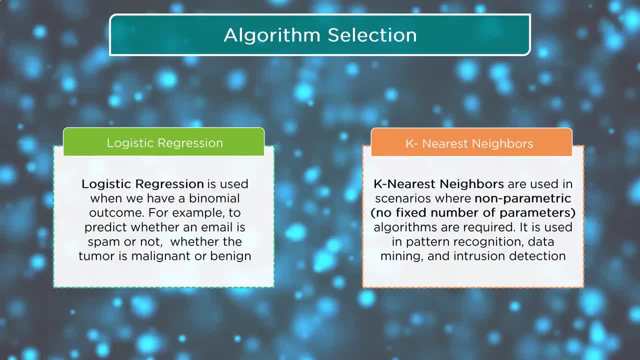 Logistic regression is used when we have a binomial outcome, for example, to predict whether an email spam or not, whether the tumor is malignant or not. The logistic regression works really good on that. You can do it in a K nearest neighbors. 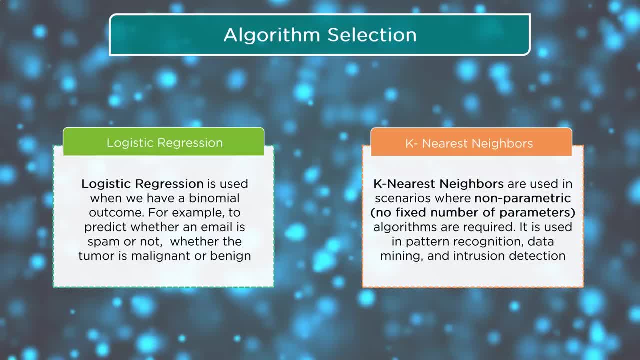 Also, the question is, which one will it work better in? I find the logistic regression models work really good in a lot of raw numbers. So if you're working with, say, the stock market, is this a good investment or a bad? 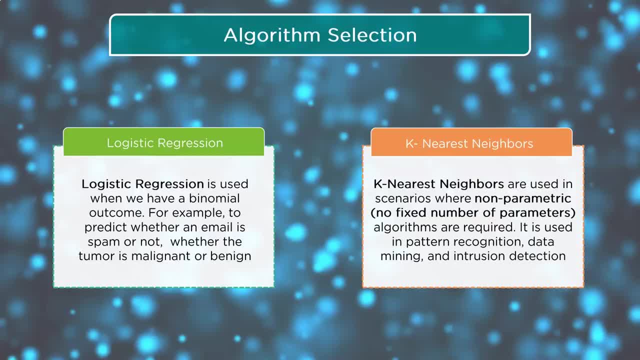 investment. So that's one of the things that it handles the numbers better. K- nearest neighbors are used in scenarios where non parametric- no fixed number of perimeters- algorithms are required. It is used in pattern recognition, data mining and intrusion detection. 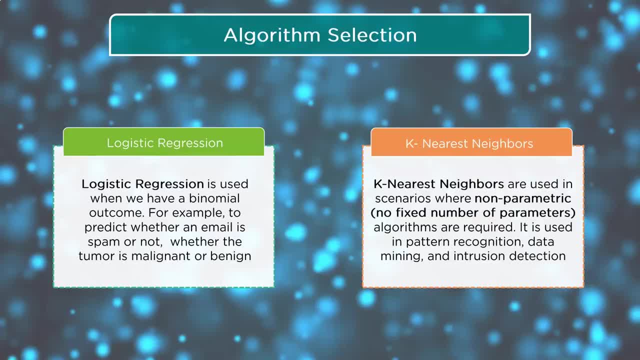 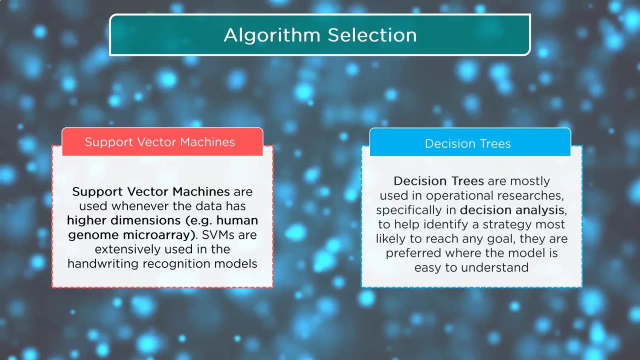 So K means really good in finding the patterns. I've seen that as a preprocessor to a lot of other processors where you use the k- nearest neighbors to figure out what data groups together Very powerful package Support vector machines. Support vector machines are used whenever the data has higher dimensions. 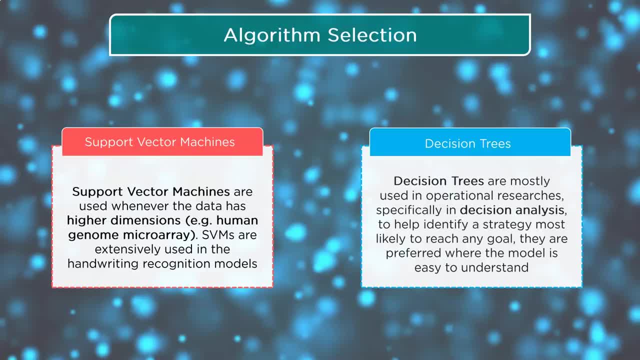 The human genome microarray. SVMs are extensively used in the hard handwriting recognition models And you can see that we were able to switch between the parabolic and the circular setup on there, where you can now have that donut kind of data and be able to filter that out with the support vector. 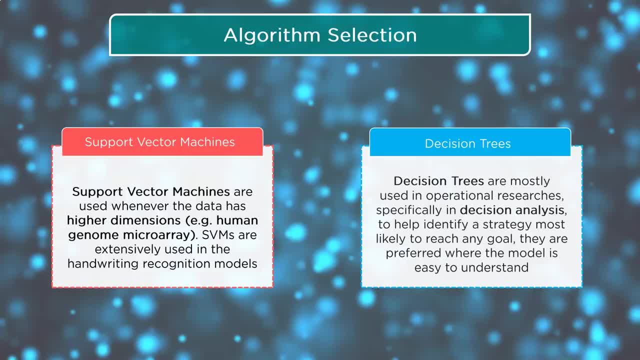 machine and then decision trees are mostly used in operational researches, specifically decision analysis, to help identify a strategy most likely to reach any goal. They are preferred where the model is easy to understand. I like that last one. It's a good description. 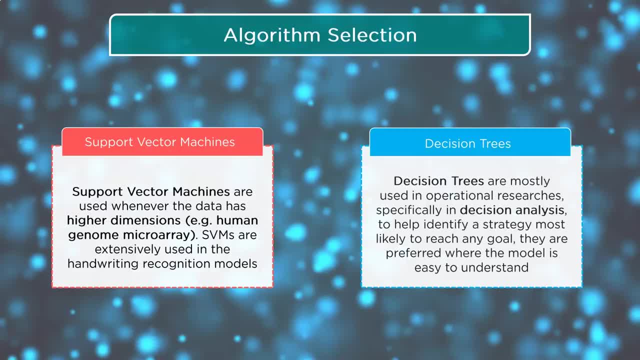 Is it easy to understand. So you have data coming in. When am I going to go to bed? You know was it raining outside? You can go back and actually look at the pieces and see those different decision modes. takes a little bit more to dig in there and figure out what they're doing. 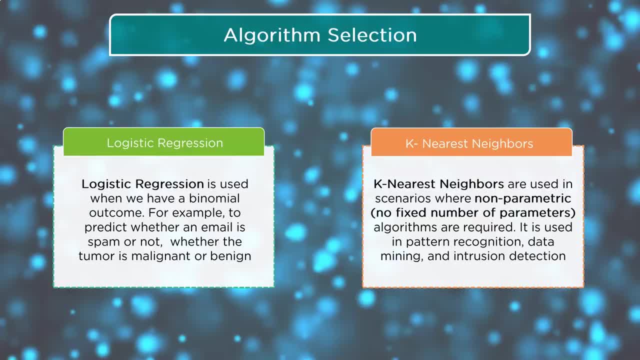 talk about algorithm selection. Logistic regression k-nearest neighbors. Logistic regression is used when we have a binomial outcome, For example, to predict whether an email is spam or not, whether the tumor is malignant or not. The logistic regression works really good on that. You can do. 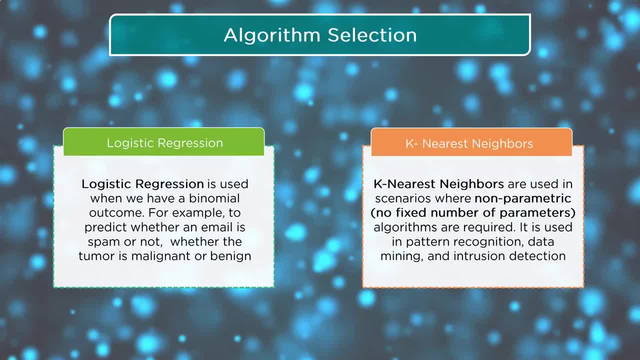 it in a k-nearest neighbors. also, The question is, which one will it work better in? I find the logistic regression models work really good in a lot of raw numbers. So if you're working with, say, the stock market, Is this a good investment or a bad? 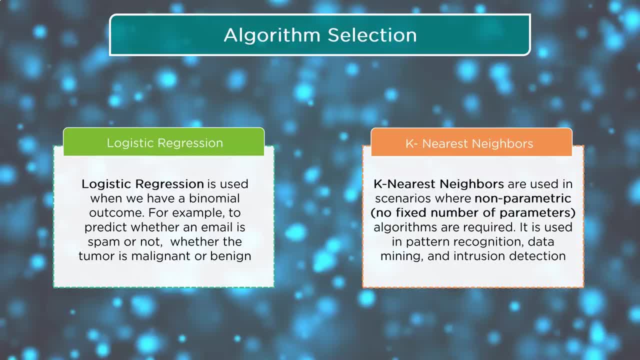 investment. So that's one of the things. it handles the numbers better. K-nearest neighbors are used in scenarios where non-parametric- no fixed number of perimeters- algorithms are required. It is used in pattern recognition, data mining and intrusion detection. So k means 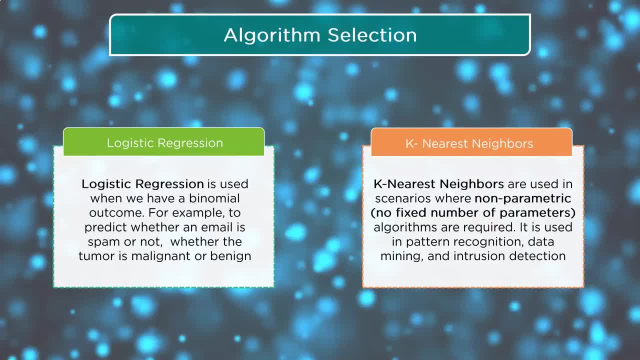 really good in finding the patterns. I've seen that as a pre-processor to a lot of other processors where you use the k-nearest neighbors to figure out what data groups together. Very powerful package Support vector machines. Support vector machines are used whenever the data 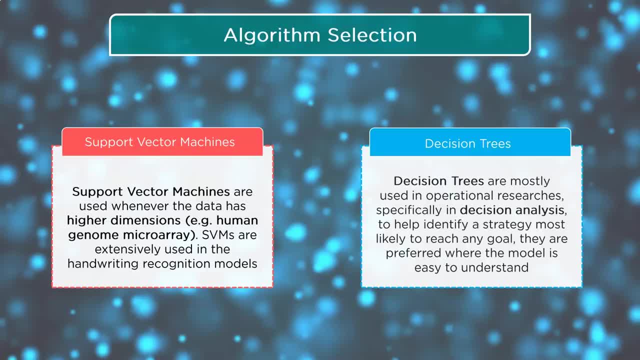 has higher dimensions, The human genome microarray SVMs are extensively used in the hard handwriting recognition models And you can see that we were able to switch between the pair of the parabolic and the circular setup on there where you can now have that donut kind of data. 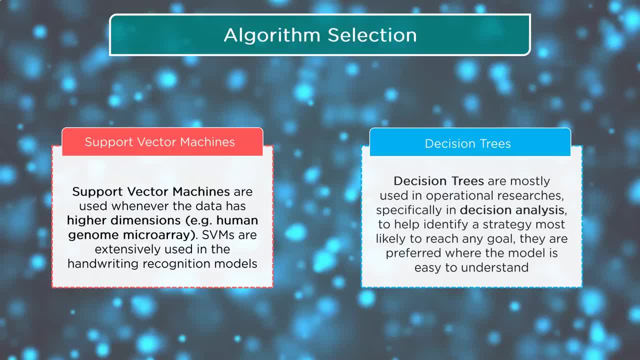 and be able to filter that out with the support vector machine. And then decision trees are mostly used in operational researches, Specifically decision analysis, to help identify a strategy most likely to reach any goal. They are preferred where the model is easy to understand. 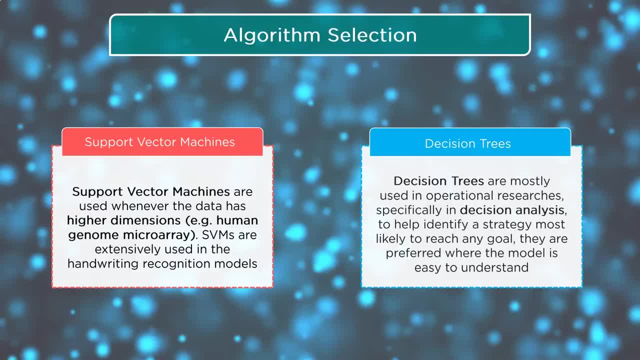 I like that last one. It's a good description. Is it easy to understand? So you have data coming in. When am I going to go to bed? You can go back and actually look at the pieces and see those different decision modes. 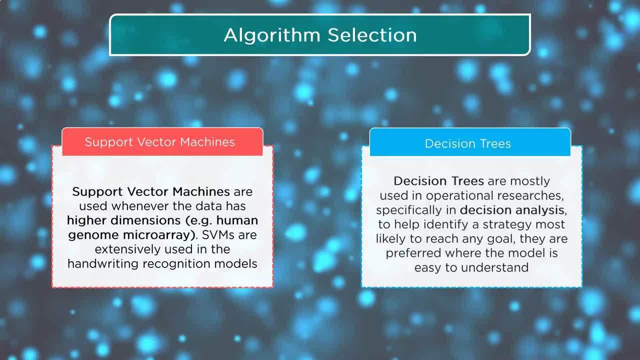 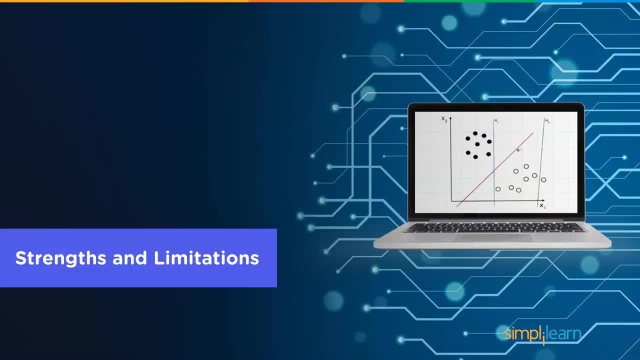 It takes a little bit more to dig in there and figure out what they're doing, But you can do that and you can actually help. you figure out why People love it for the why factor So strengths and limitations? Big one on all of these. 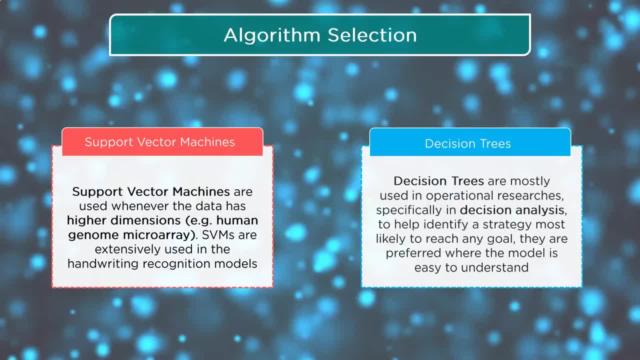 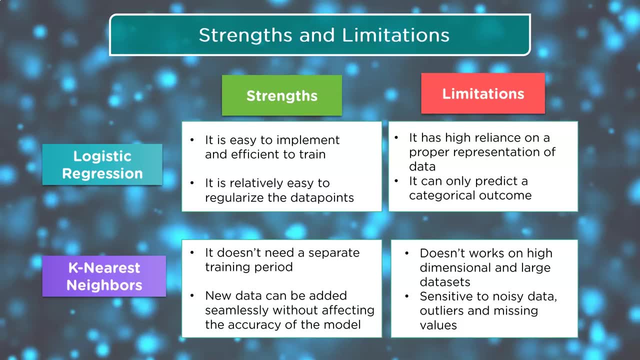 But you can do that and you can actually help you figure out why people love it for the Y factor. So strengths and limitations, Big one on all of these, The strengths and limitations. We talk about logistic regressions. The strengths are: it is easy to implement and efficient to train. 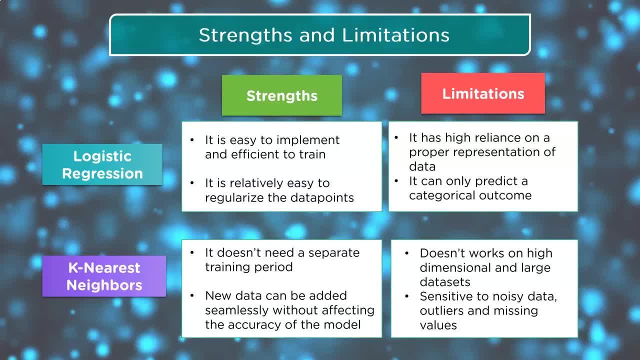 It is relatively easy to regularize The data points. remember how we put everything between zero and one. When you look at logistic regression models, you don't have to worry about that. as much limitations as a high reliance on proper representation of data that can only predict a categorical outcome. 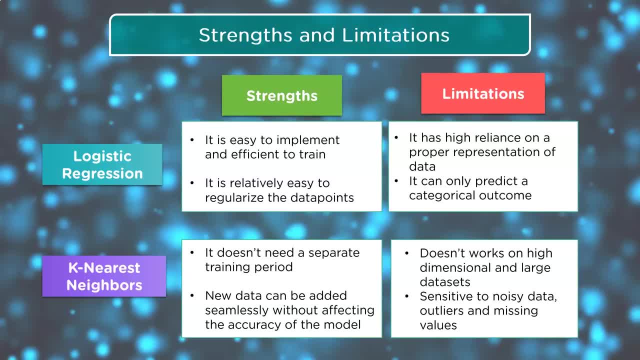 with the K nearest neighbors. it doesn't need a separate training period. New data can be added seamlessly without affecting the accuracy of the model. Kind of an interesting thing because you can do partial training. that can become huge If you're running across a really large data sets or the data is coming in. 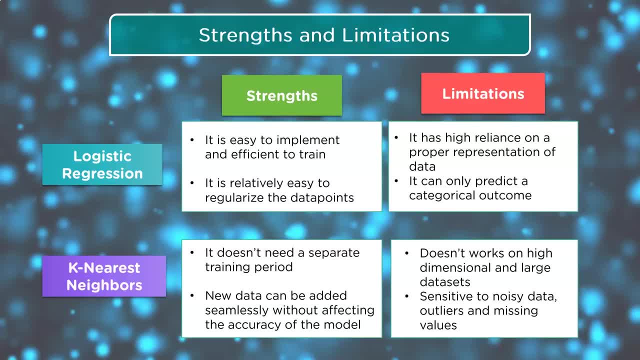 you can continually do a partial fit on the data with the K nearest neighbors and continue to adjust. that data doesn't. doesn't work on high dimensional and large data sets. We were looking at the breast cancer: 36 different features. What happens when you have one hundred twenty seven features or a million features? 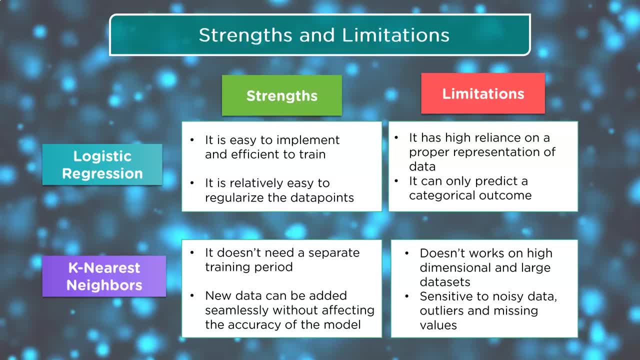 And you say: well, what do you have? a million features in. Well, if I was analyzing logic, I would have a million features. And if I was analyzing the legal documents, I might have a tokenizer that splits the words up to be analyzed, and that tokenizer might create one million. 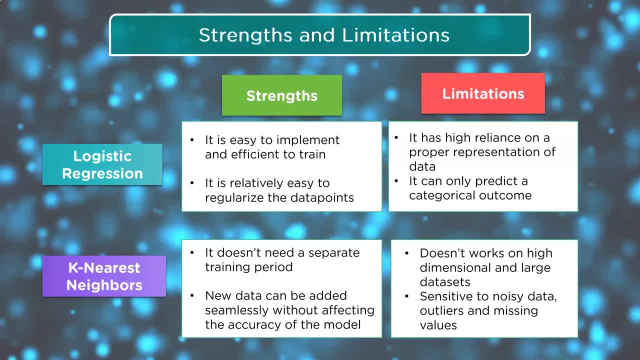 different words available that might be in the document for doing weights sensitive to noisy data outliers and missing values. That's a huge one with K nearest neighbors. They really don't know what to do with the missing value. How do you compute the distance if you don't know what the value is? 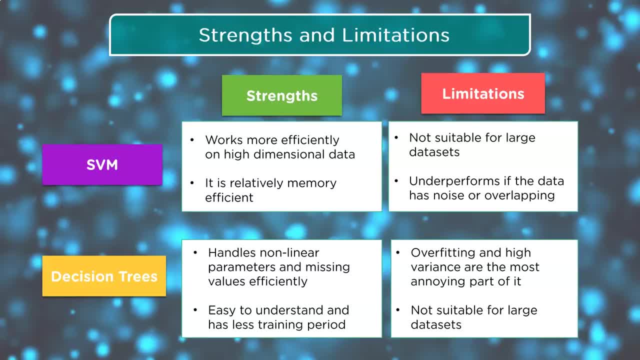 The SVM works more efficiently on high dimensional data. It's relatively memory efficient, so it's able to create those planes with only a few different variables in there, as opposed to having to store a lot of data for different features and things like that. It's not suitable for a large data sets. 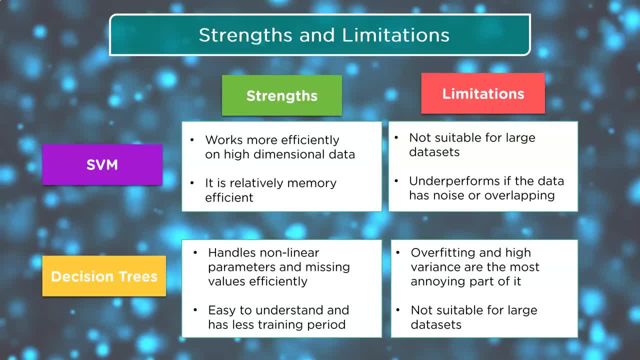 The SVM, you start running this over gigabytes of data causes some huge issues, Underperforms, if the data has noise or overlapping. That's a big one. We were looking at that where the SVM splits it and it creates a soft buffer. 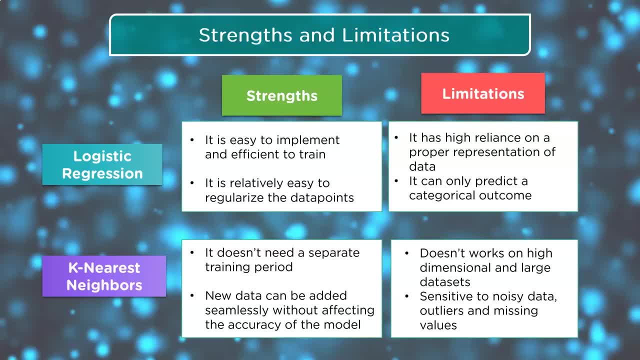 The strengths and limitations We talk about logistic regressions. The strengths are: it is easy to implement and efficient to train. It is relatively easy to regularize. Remember how we put everything between zero and one When you look at logistic regression models. you don't have to worry about that as much. 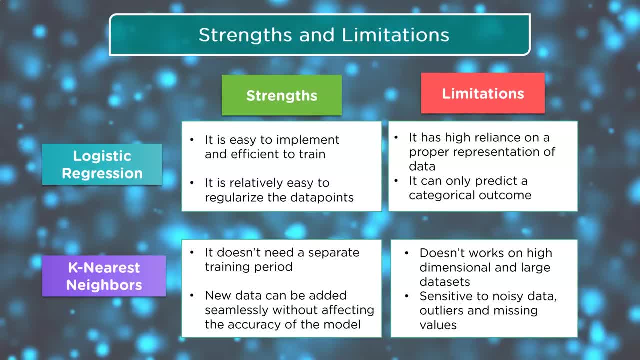 Limitations. as a high reliance on proper representation of data, It can only predict a categorical outcome With the K nearest neighbors. it doesn't need a separate training period. New data can be added seamlessly without affecting the accuracy of the model. Kind of an interesting thing, because 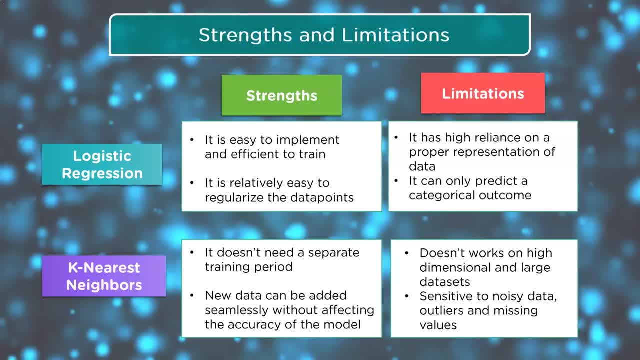 you can do partial training. That can become huge if you're running across data sets or the data is coming in. You can continually do a partial fit on the data with the K nearest neighbors and continue to adjust that data. It doesn't work on high dimensional. 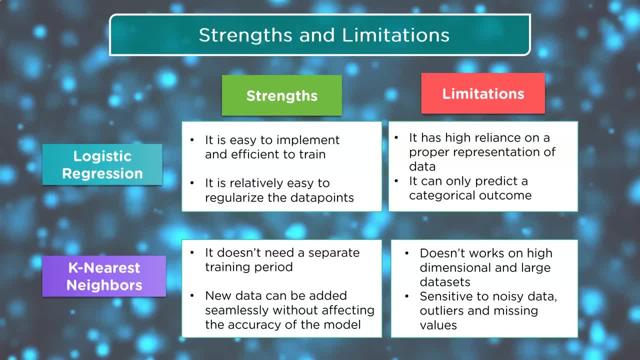 and large data sets. We were looking at the breast cancer: 36 different features. What happens when you have 127 features or a million features, And you say, well, what do you have a million features in? Well, if I was analyzing the legal documents, 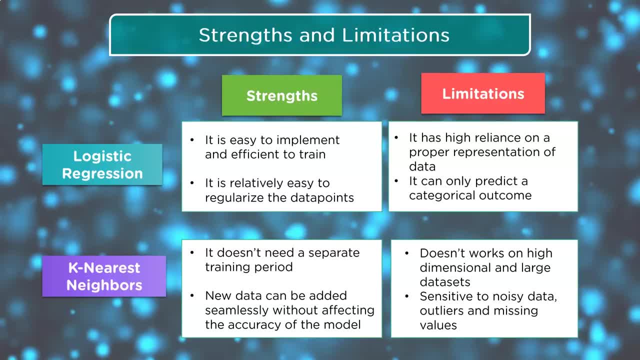 I might have a million features. I might have a tokenizer that splits the words up to be analyzed and that tokenizer might create one million different words available that might be in the document for doing weights Sensitive to noisy data outliers and missing values. 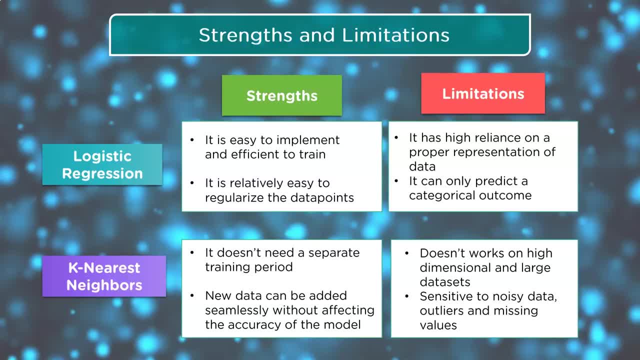 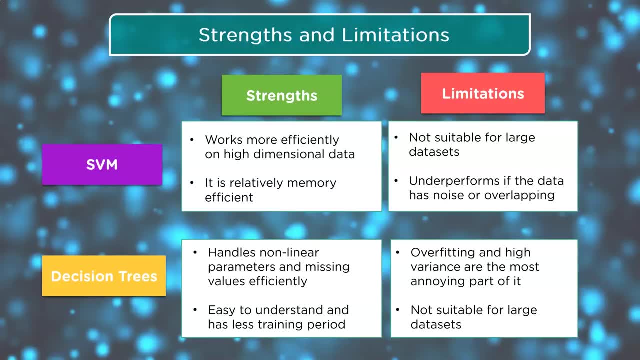 That's a huge one with K nearest neighbors. They really don't know what to do with a missing value. How do you compute the distance if you don't know what the value is? The SVM works more efficiently on high dimensional data, So it's able to create those planes. 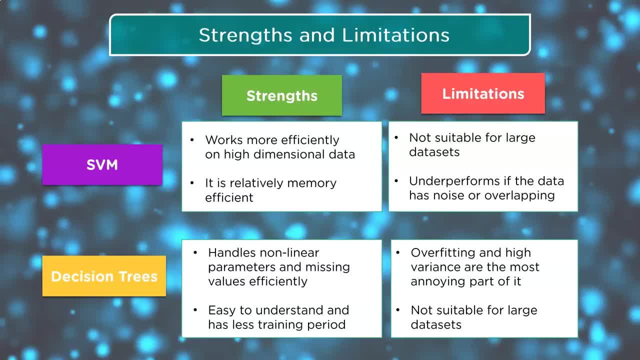 with only a few different variables in there, as opposed to having to store a lot of data for different features and things like that. It's not suitable for large data sets. The SVM you start running this over gigabytes of data causes some huge issues. 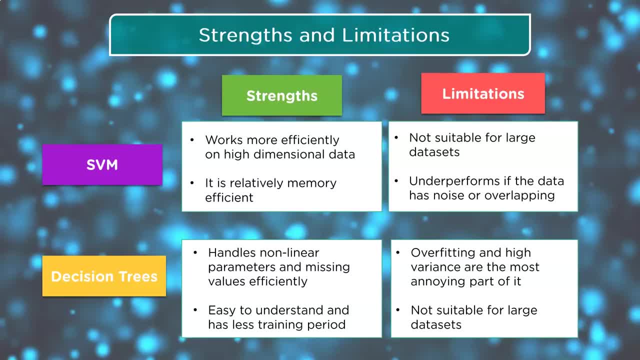 Underperforms if the data has noise or overlapping. That's a big one. We were looking at that where the SVM splits it and it creates a soft buffer. but what happens when you have a lot of stuff in the middle? that's hard to sort out.